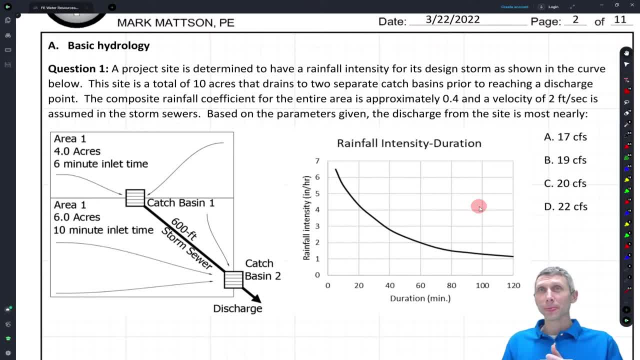 question number one says is a hydrology question. So hydrology has to do with water falling right and running off a site. So obviously the big concern here with hydrology is: before development you got a bunch of trees, grass and you have a lot more room for that site. 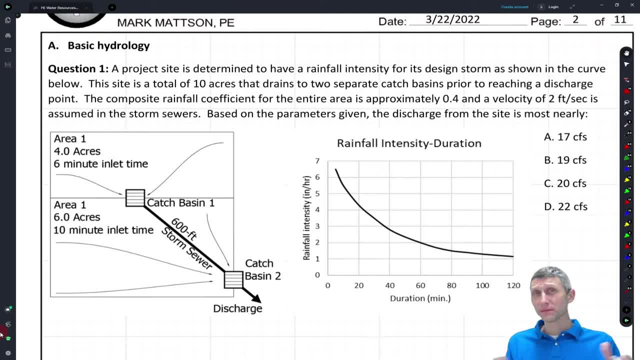 to retain water And after development, where you get a lot more pavement, maybe develop space and there's going to be more runoff. So one of the ways of getting runoff is is by using Q equals CIA. So the rational, the rational method, And here we have a project site determined. 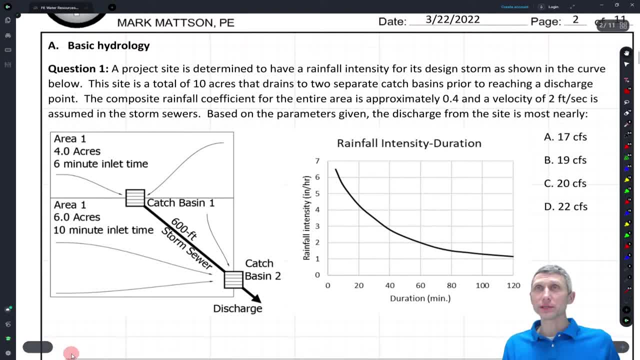 to have rainfall intensity for its design storm, as shown in the curve below. So this is a rainfall intensity duration curve right. So generally you might get that really quick blast and you get a bunch of rain right away, but it doesn't last as long versus a long. 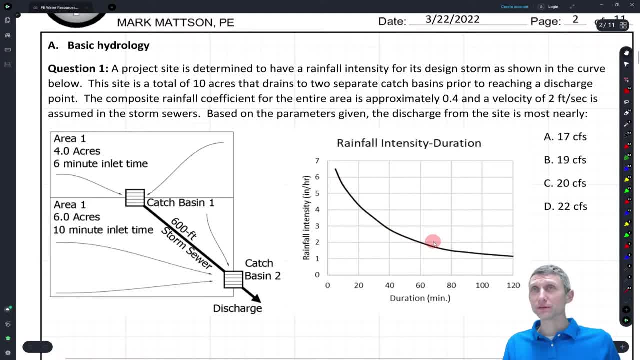 slow drizzle right, We have our intensity duration curve And the total site has 10 acres. So we have two areas, two catchments here: area one and that should say area 2.. So if you guys were in, I'll repost this with area 2.. So that's one other correction that I have to make. 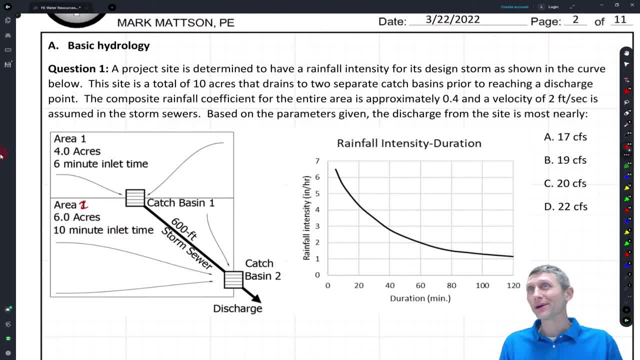 So we have area one, area two. one area has 4 acres, 1 area 6 acres and area one. everything in area one is going to drain to this catch basin, Okay, And then everything in area 2 is drained to area 2.. Everything in area 2 is going to drain. to this catch basin, Okay, And then everything in area 2 is going to drain to this wetland. So then you can see that these areas change. So you can see that here's a lot of different things over the area of soil you can see. So we can see all of the areas change over the. 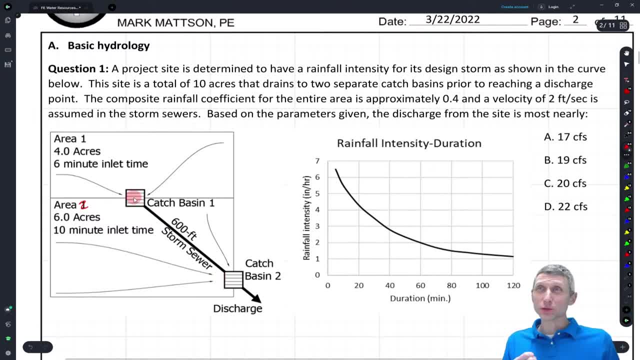 is going to drain to this catch basin and in between the flow goes from catch basin 1 to catch basin 2. so that's kind of the way this site is set up and the come in and what we see here is the composite rainfall coefficient for the. 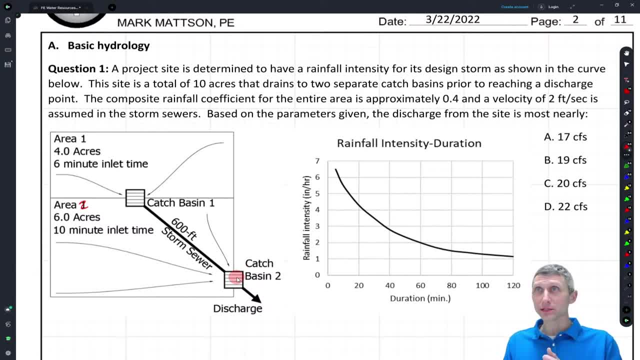 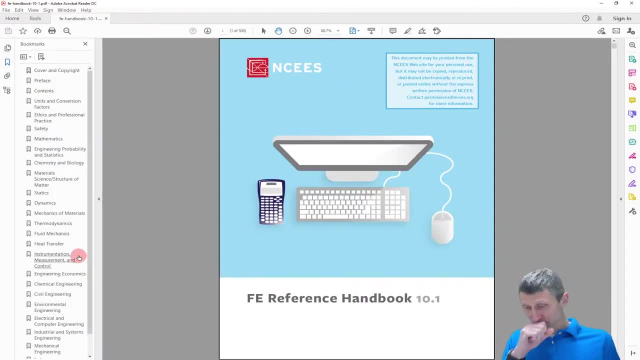 entire area is about 0.4. velocity to 2 feet per second is assumed in the storm sewers and, based on the parameters given, the discharge from this site is most nearly so. this is where, again, when we take a look at our reference handbook here, we're gonna be in this civil engineering section. I hope, I believe, and 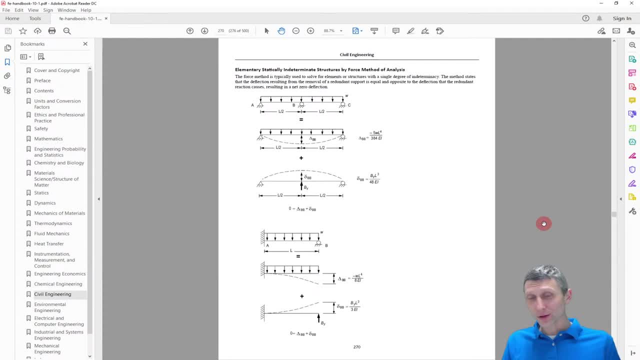 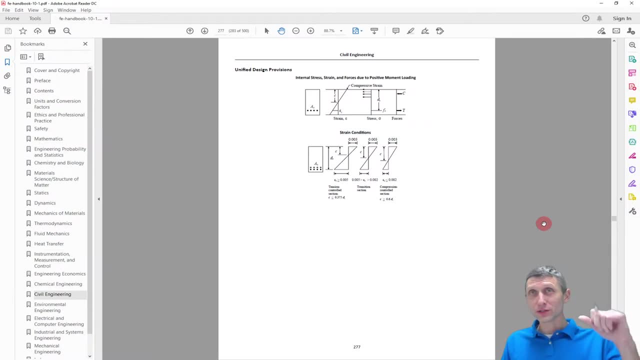 what we're gonna be doing here is we're gonna be taking a look, is we're gonna go past the structures, past geotech, and I like sort of scrolling through this a little bit, so you can kind of- and maybe you should do this too when you, as 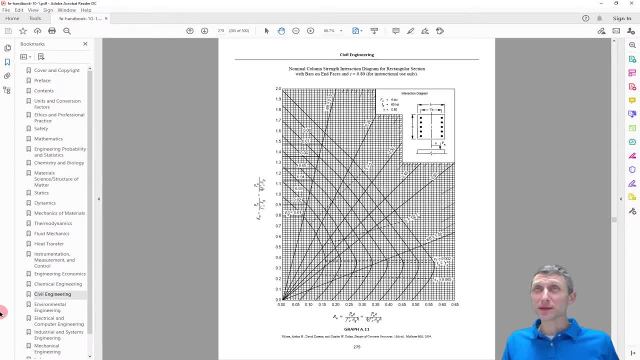 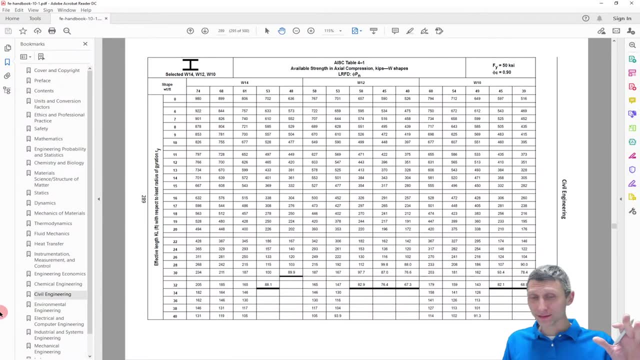 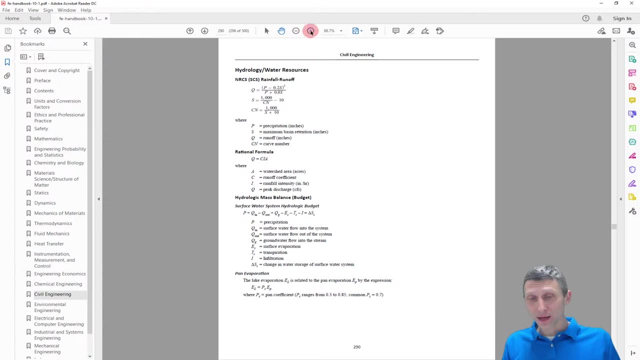 you're studying for the FE. but the nice thing about scrolling through these: sometimes you get kind of used to where things are okay and eventually you get past steel right in past steel. we get there, getting there and we get the hydrology water resources right. so we have the NRCS method and we 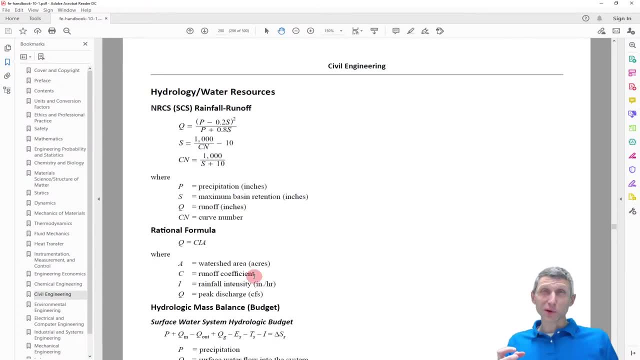 have the rational formula here, and anytime you're gonna write runoff coefficient, typically you're gonna be using this: Q equals CIA, so the- I mean that sounds easy enough. all we need is the rock coefficient intensity at the watershed and the peak discharge right. so that's the formula we're gonna use. 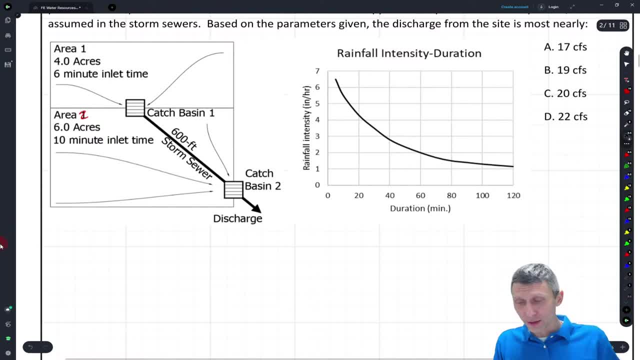 here. so we know that we're gonna say, right, Q equals CIA. but then what we have to do is we have to figure out: well, okay, we know the area, that's already ten acres, so we know the area. but in, we know, see, right, so we know. 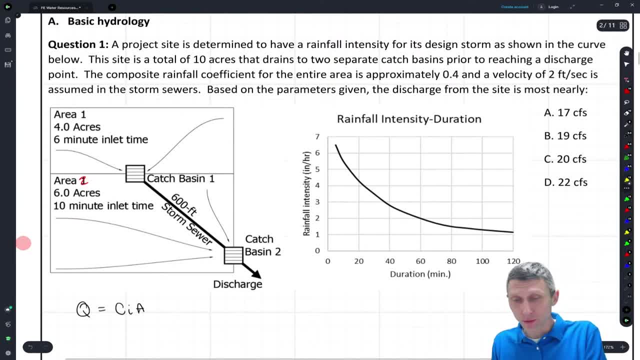 the area. we're actually given these two parameters. right, we're giving, we're given the area of a, we're given C a point, for really, the only thing that we have to do here is is find the intensity, and some of you are probably gonna be tempted to come here and, just you know, pick a number. and I'm just reading this: 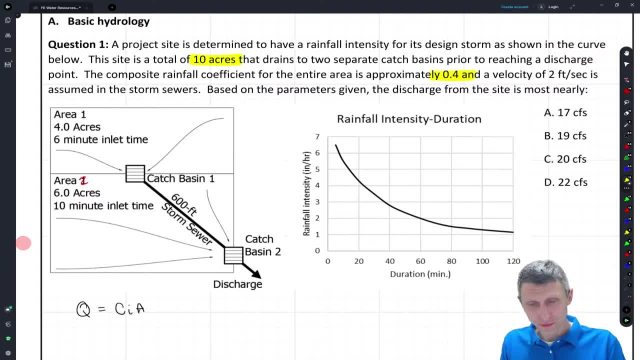 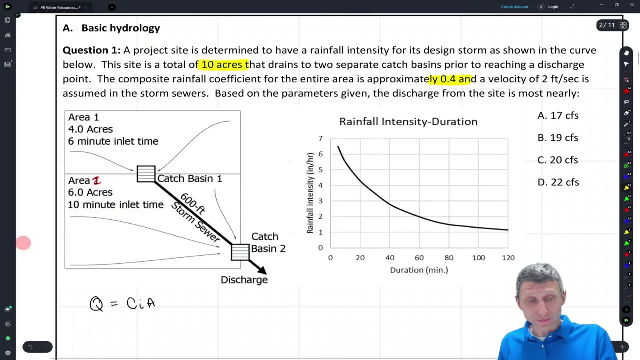 for a second too, but I think this is a good way to kind of figure out where to go. oh no, i think we're good. oh sorry, so, um. so, as we go through here, what we're going to do is we have to find that intensity. and to find the intensity, um, what we're going to do is: 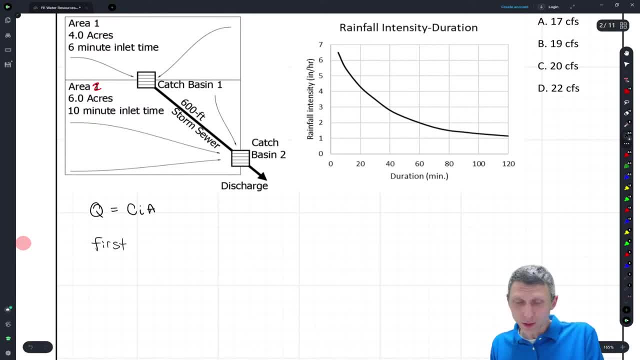 we have to first um solve for the time of concentration. so what's the time of concentration? the time of concentration is essentially the time until you have all of the water kind of concentrated at your, at your outflow, right. so with what we have here is it's like i i have a house that's next to a stream and it might start raining. 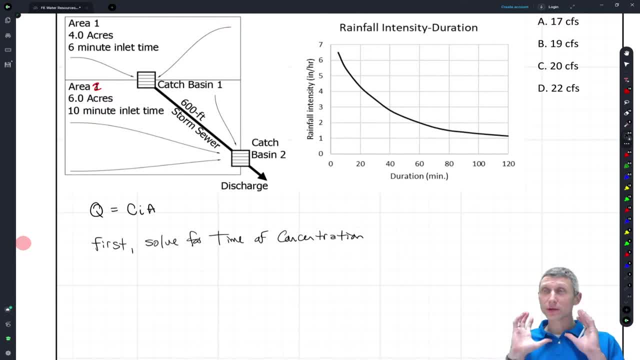 and then about 20 minutes later, that storm- that's that stream- is really rushing. well, what happened it? it took 20 minutes for that that stream to start raining and then about 20 minutes later to get really full with all the runoff from all the different areas hitting that stream. so kind. 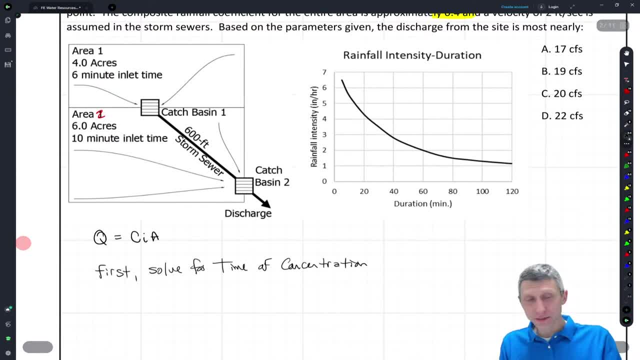 of the same thing is going to happen here. right, what we have is we have two different areas, right, we have area one and we're bringing water in from area one. it comes down to this catch basin and then it goes through the storm sewer and goes out. so what we want to do is we want to find the 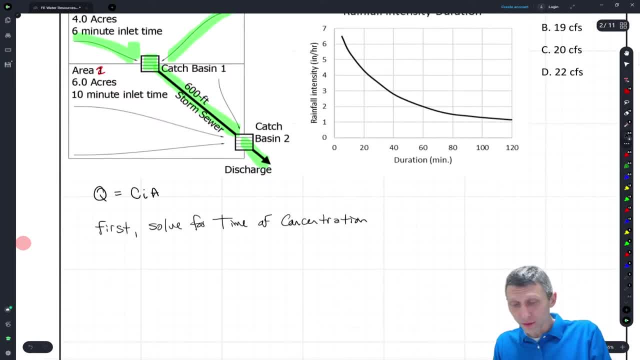 time of concentration for that area. so we're going to start with, like, i'm just going to call this tc1 and that's going to be our time of concentration for that area. so all that we, all that we have to do here is we'll we say: well, we know that it takes six minutes to go from the most remote point, the catch basin. 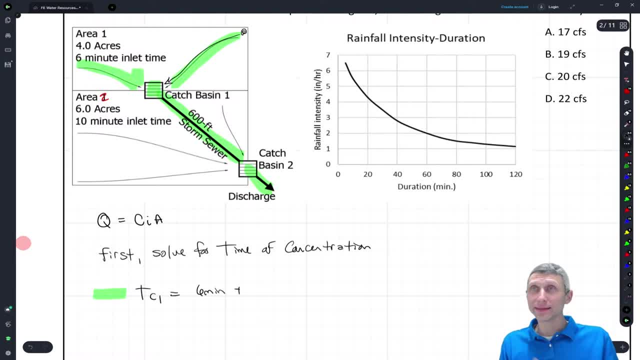 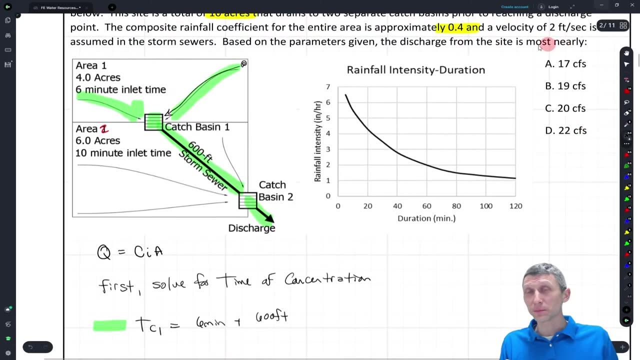 so we're going to start with six minutes and then we're going to add the amount of time it takes in the storm sewer. so in the storm sewer, um, we know the sewer is 600 feet right, so 600 feet. and um, we're told in the problem that we have um two feet per second, so velocity: two feet per second. so how? 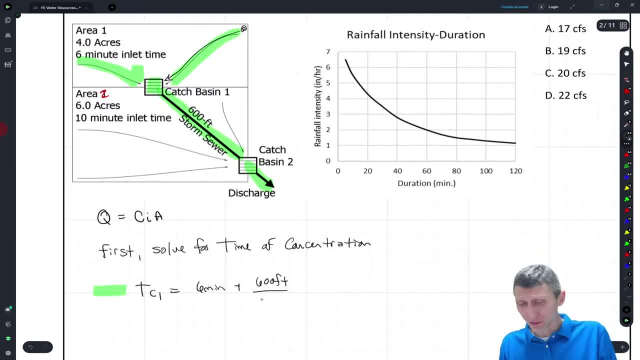 long is it in that sewer? well, to get the time, we're going to divide by two feet per second. but you'll see here that the the units aren't the same, so we have minutes and seconds. um, we need to do some conversions here. our duration, um for our curve here, is in minutes. so we are going to go. 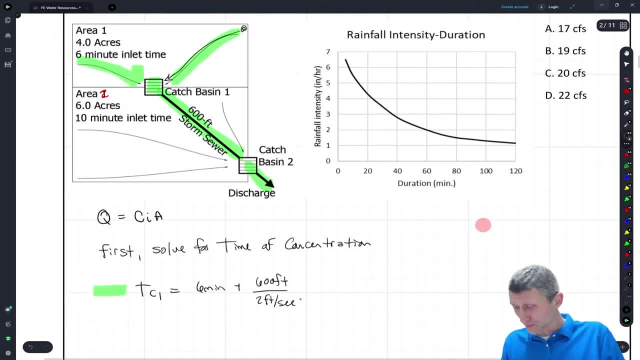 with um, with minutes. so what we want to do is we want to multiply by on the bottom here i'm just going to extend this a little bit- but we're going to multiply by um 60 seconds per minute and this time of concentration. if we do that out, um, we do. what do we do? 600 divided by two divided. 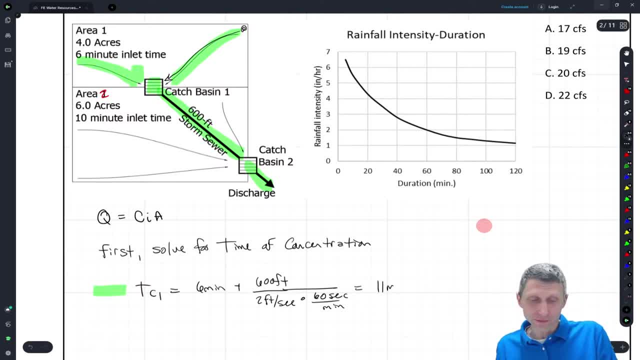 is going to be five minutes, so this is a total time of concentration of 11 minutes. so when you know the rain starts falling, it takes 11 minutes to go from the most hydrologic, hydrologically distant point on that watershed to the catch base and through the catch basin and out of the sewer. 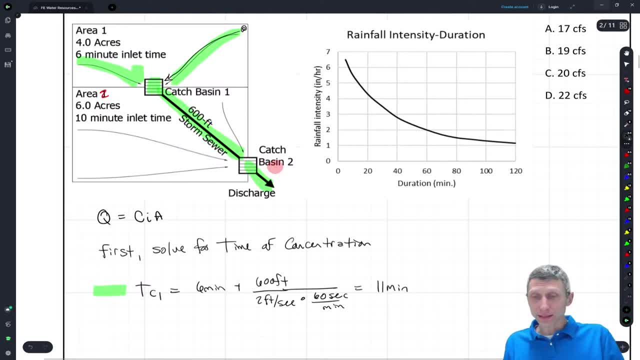 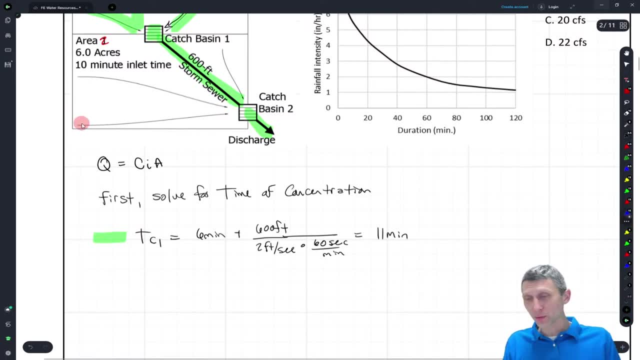 okay, out of discharge off the site. so then let's look at time of concentration too. in in what we see here is: um, this one's actually a little bit easier, because what we're doing with this one is we're saying, okay, we're starting on a hydrologically most distant point and we're 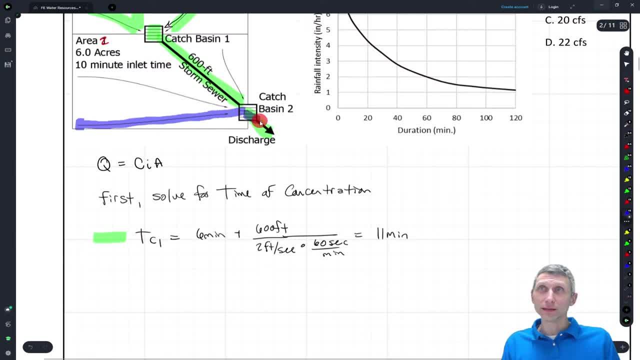 going to go to catch basin two and then we're going to go off the site, okay, so. so with this, we actually don't head through the storm sewer at all. and for this one, um, we're just told that, you know, time of concentration two is 10 minutes, so all that we're going to do here is we're just 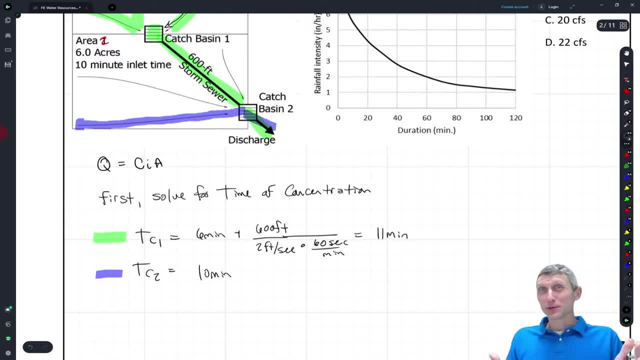 going to say: well, this one's 10 minutes. and now comes the question: well, what's the time of concentration? is it 10, is it 11, or is it 21? well, again, let's think. when rain starts falling, it starts falling at the same. you know time of concentration: it starts falling at the same time. 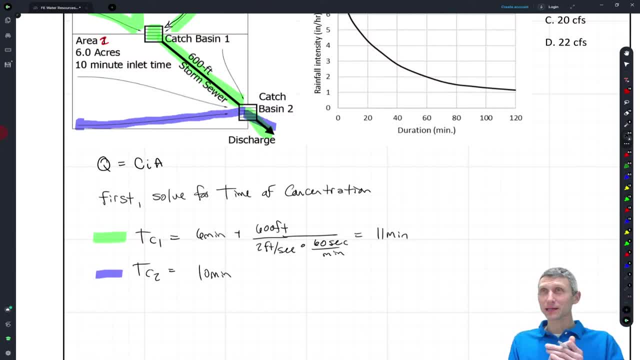 you know, this whole 10 acre site all at the same time, roughly within you know, a couple seconds probably. so what we're doing is we're trying to say the time of concentration is the time, from the most distant part, to all hit the discharge point at the same time. so we're going to take the longest. 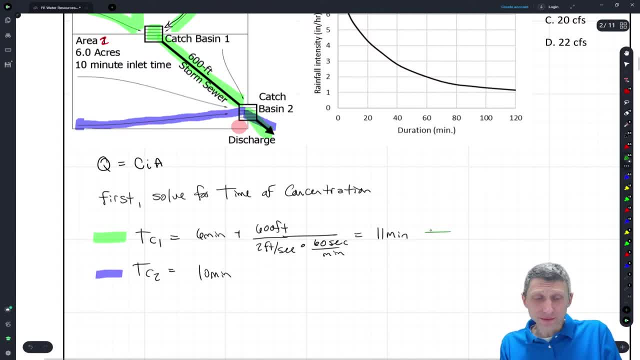 time of concentration here and we're going to say that the 11 minutes um controls right. so this is going to be um the worst case for for your intensity. essentially, once you hit that 11 minutes, all the water's flowing from all over the site. that's going to be, uh, your worst case. so that's the the storm, you know intensity. 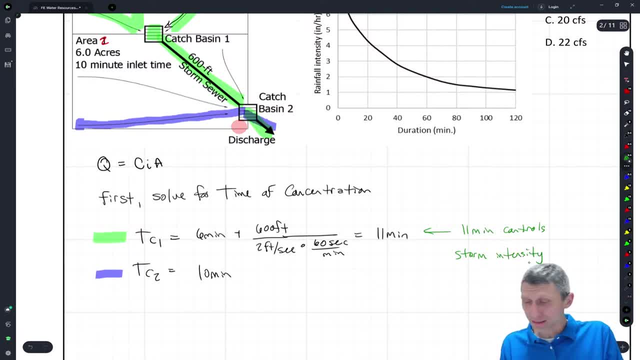 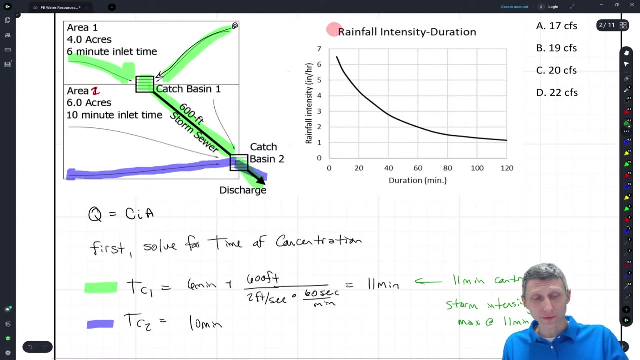 is going to be the max essentially is going to be um. the storm intensity is going to be the max at 11 minutes. so, um, if we have that, we can come back up here now and we can use our rainfall intensity intensity duration curve and we can take a look at this right. so i'm just going to 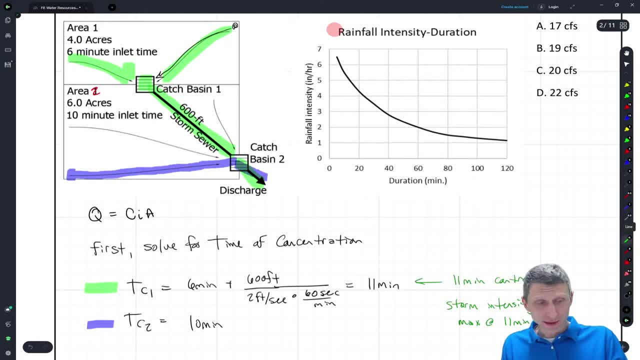 get a line here, and if i take a look at a line, essentially, um, let's take a look at a line here, let's take this here. so i'm going to come in at 11 minutes, which is right around here. i don't know if you can see that. yeah, you can, you can see it. well, enough, right, and then what i'm going to do. 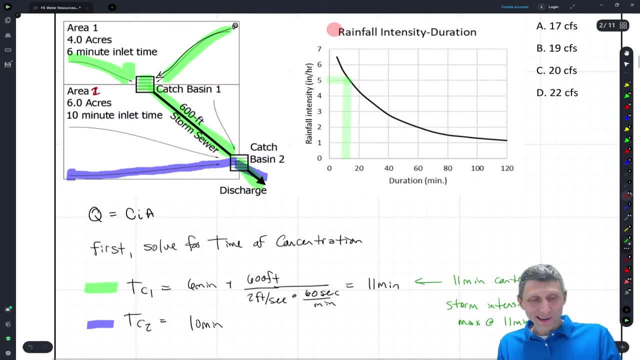 is until i hit this curve, and then i'm going to come over. so what we see is this curve is, you know, we hit this curve somewhere around on that point, okay, which is roughly five inches per hour. so what we've just done is we've gone and we've gotten our eye, so this is our eye value. 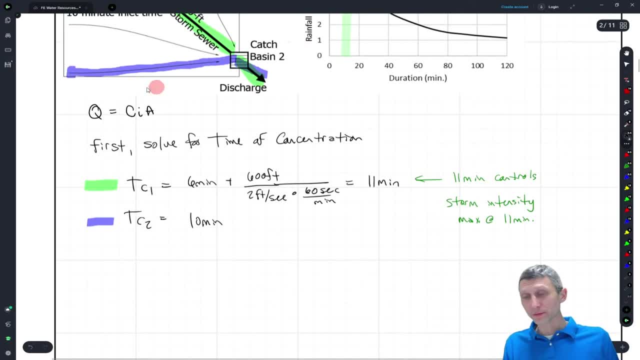 of of five inches per hour. so when we come back and solve our formula now, um, essentially all that we have to do is we have to say: well, q equals c, which is going to be that 0.4. that was given times what? five inches per hour times 10 acres. and some of you are looking at this and saying: 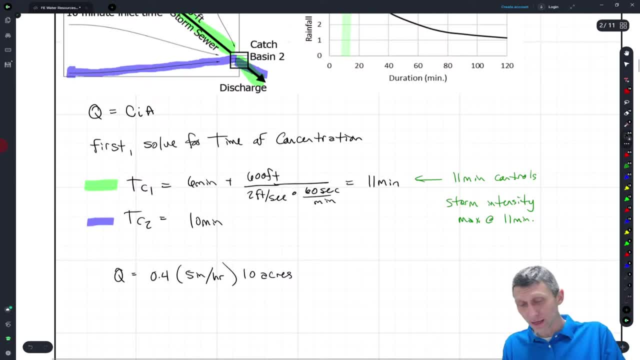 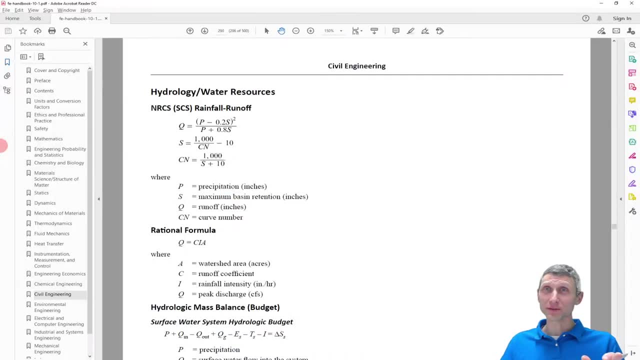 like man. those units are really nasty and, um, to be honest, they are nasty, but that's okay, because when we look at the rational formula and the handbook, right. so in the handbook, what are we? what are we given? we're given a watershed area and acres. we're given the runoff coefficient, which is unitless. it, well, isn't really unitless. 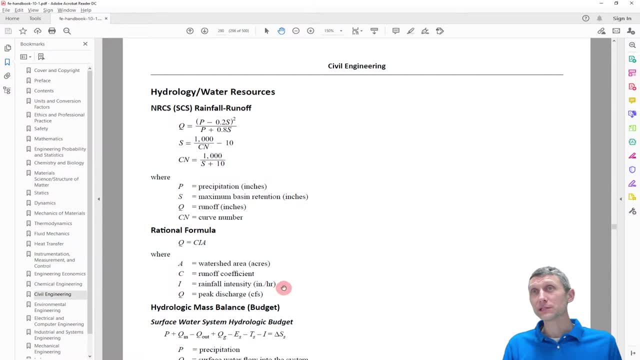 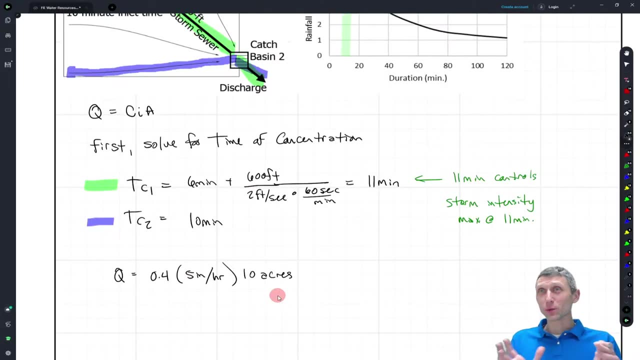 but it takes all those conversions into account. we have rainfall in inches per hour and we have peak discharge and cfs, so the beautiful thing about this equation is our units actually work out for themselves and we don't actually have to do any conversions, right? so we get. what do we get? 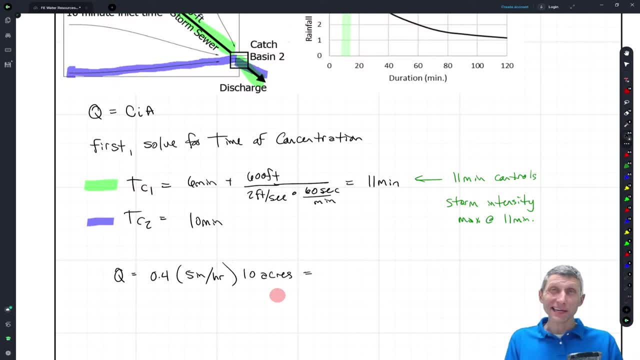 we get 0.4 times five inches per hour times 10 acres, and we get 0.4 times 10 acres and we get 20 cfs, so 20 um cubic feet per second. so that's kind of the first. the first step here is just to. 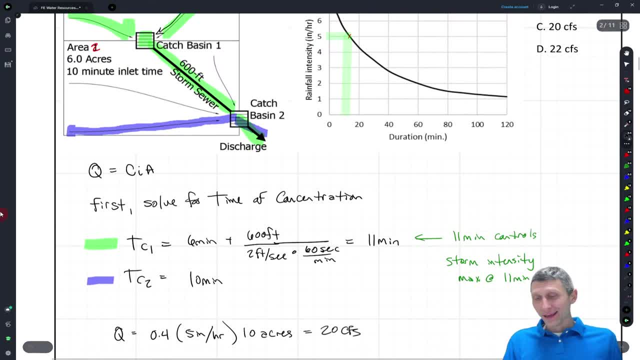 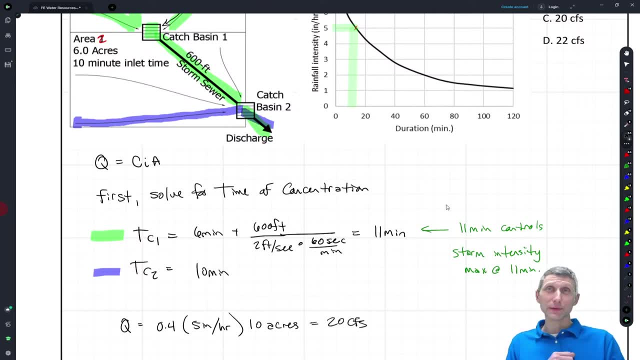 take a look at uh flow from a site and you know you might be given a duration um intensity curve. you might be given uh some catchments you might have to solve for the time of concentration. but again, what we're looking for is the maximum time of concentration, the peak intensity at this for 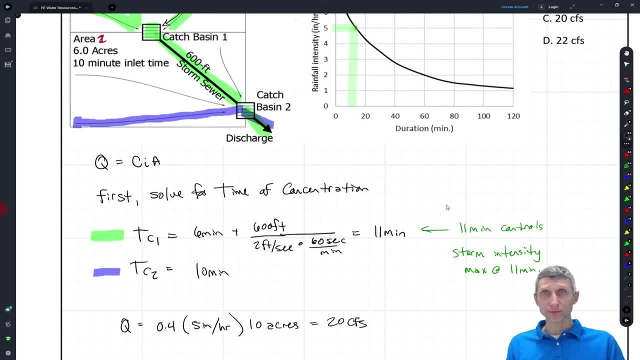 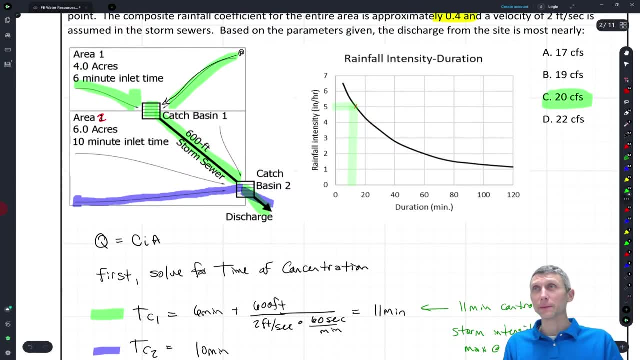 this storm, you know, and that's going to give us, um, the wrong answer, so we're going to have to run off before that for that design storm. okay, so we can come back up here. uh, we got our 20 cubic feet per second, uh, so we're pretty good, all right, so that's pretty cool and, uh, hopefully, uh, that. 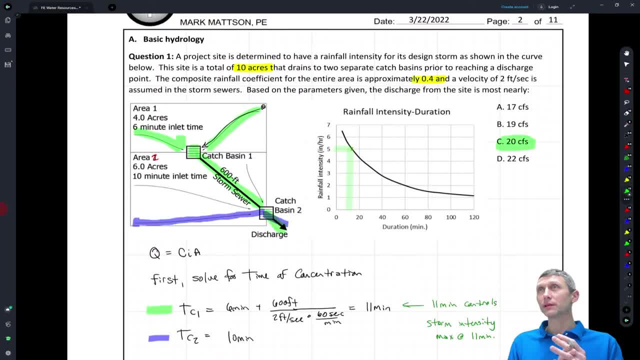 works for you. if you do have questions, feel free to drop um any comments. so the live. i am trying to monitor the live uh chat as well. so, um, or, if you're watching this video later, you can put comments down below and i will do my best to respond to those as well. so, um. 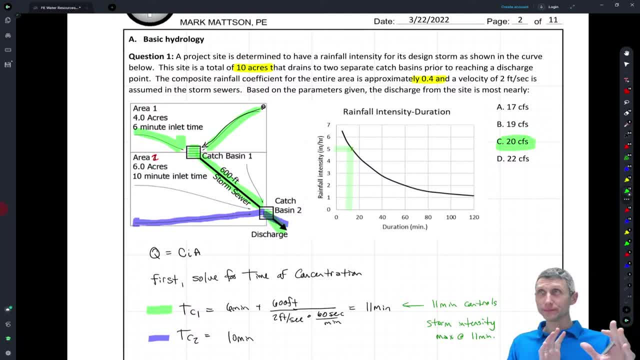 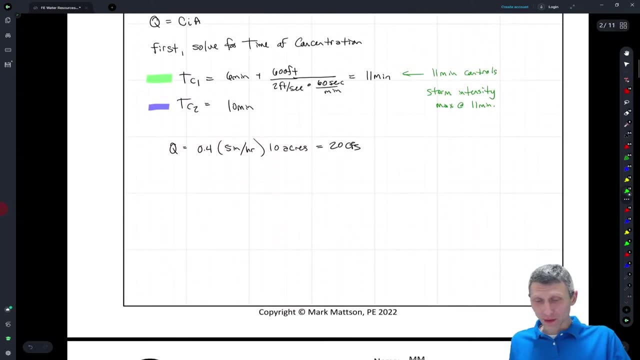 with. that said, there is a slight delay between um, i think, for buffering, for what goes live and and what's on the chat. so, uh, if i don't see you right away, um, let me know and i will try to try to get to it. all right? so as we keep going, uh, let's go to question two. so question two is another. 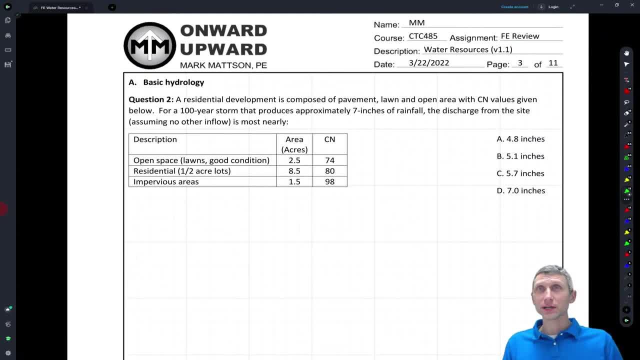 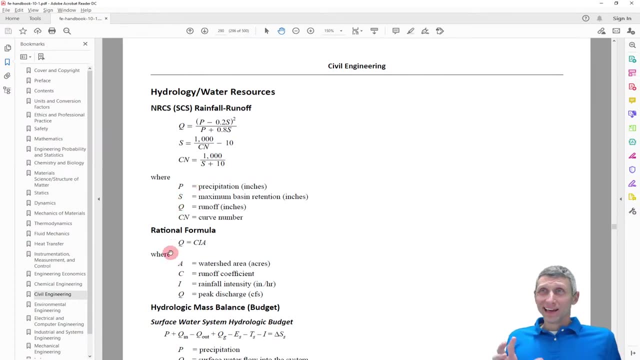 hydrology question, and this uses an alternate method, right. so this uses a method uh for uh. this is the scs method, right? or nrcs. and as we look at the handbook again, there's two methods kind of for predicting run, runoff, and the rational formula gets a lot of use. um, the scs rainfall, uh runoff method does as well. so 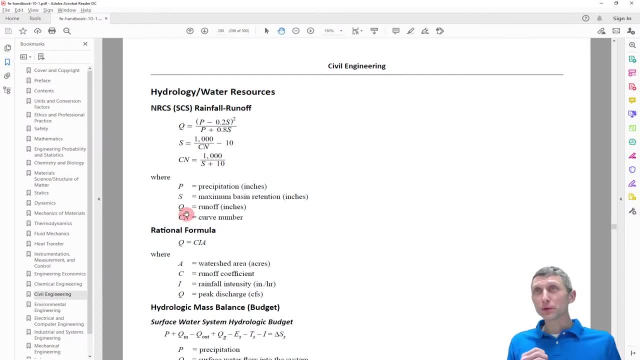 they're both good to know that. but they produce different things. they both produce q. so at the, you know, they both have these equations for q. but it's interesting to note here that this, the, the rational formula, gives a peak discharge in cfs. but what does the nrcs method do? it gives a peak. 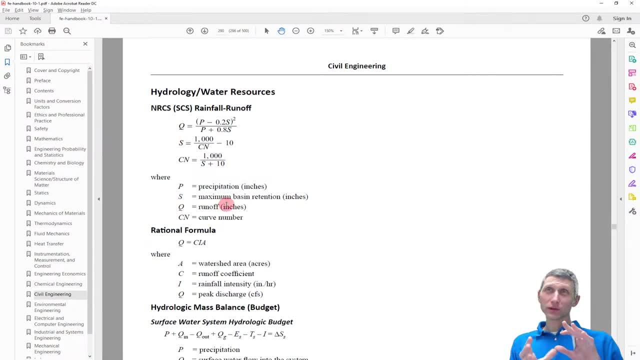 q in inches. so the, the nrcs method, um it's, it's based on ncr 55 and maybe you've seen that before, but there's a. there's like a bunch of forms. these forms get played out in in programs, uh, like water type um resources, programs with that, like a hydro cab, for example, so you can plug these in um and 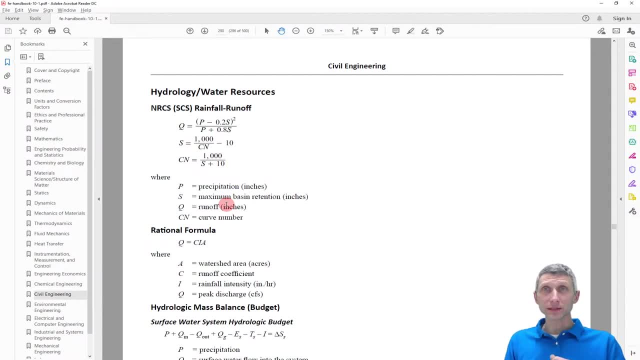 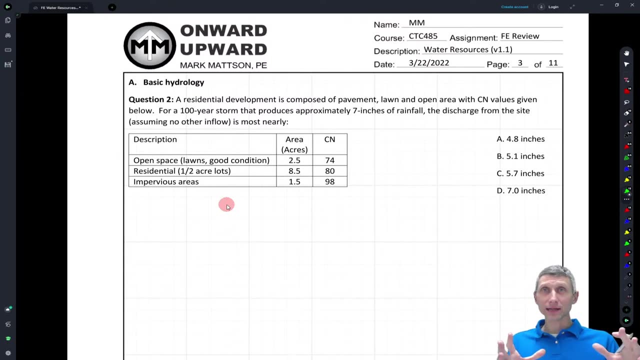 use them there, but it's good to kind of understand, uh, both methods a little bit as well, so we're going to go over this one and this is- this is the way this works- is, um, the. the land system is essentially broken up into curve numbers and what the curve number is. 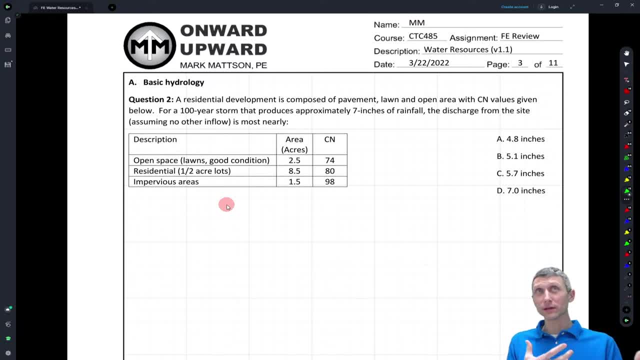 is. it's a reflection of how much runoff will come off of that site. so an impervious area like pavement will have a lot of runoff. it's. it's not a curve number of 100, because even though you know the the pavement um will will pretty much take all of that water and and shed it off. okay, it's. 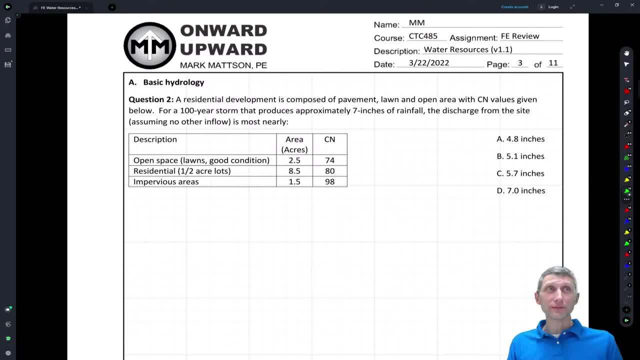 not going to shut off 100 of it. it's going to shut off 100 of it. it's going to shut off 100 of it. it's going to shut off most of it. okay, and that's okay, right, so that's okay. um, we can. um, take a look. 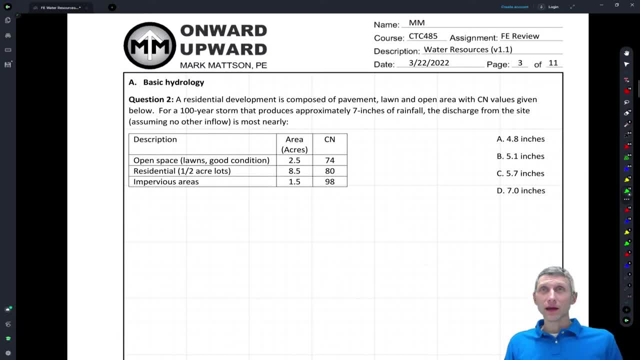 at that and i still still be okay, uh, with it. okay, so, um, just give me two seconds here to fix one thing on my stream, and i think that'll be a little bit better, okay, so, um, what we're going to do is we're going to find- uh, we're going to find- a curve number, a composite curve number for this site. 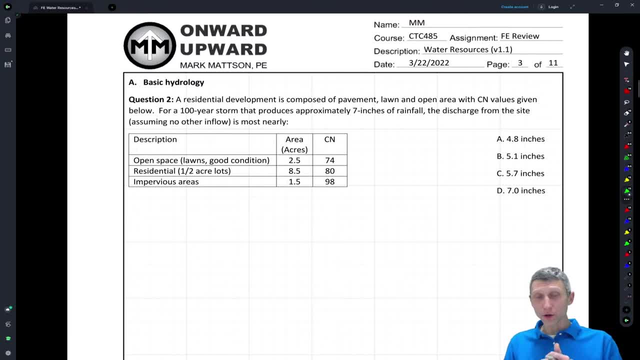 but. but basically what we're given here is residential development. we have pavement, lawn, open area, cn values given, so we have a hundred year storm that produces, let's say, seven inches of rainfall. okay, maybe you live in a part of the country where you get more than seven. 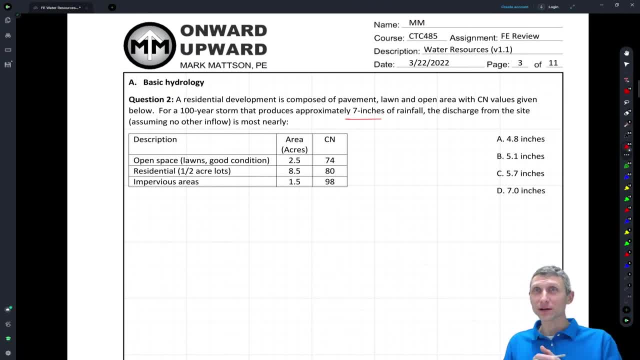 inches. uh, part of the country i live in we get about seven inches for a hundred year storm. the discharge from the site, assuming no other inflow, is most nearly so. what is the discharge? well, what we're going to do here is we're we're going to use these equations right, we're going. 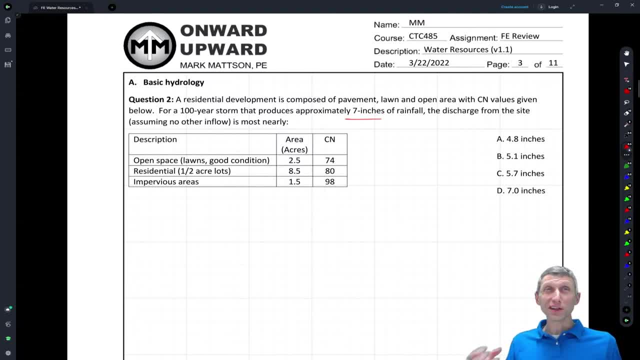 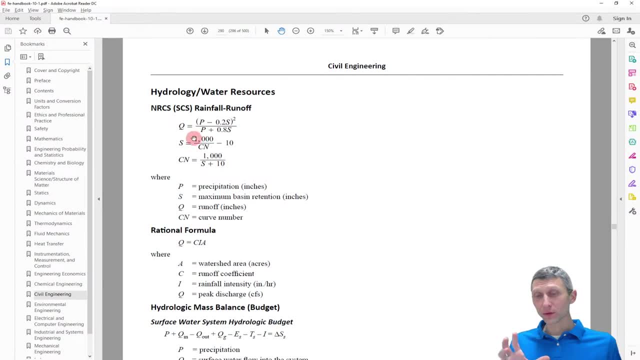 to use these um equations. we're looking for a discharge. we're looking for a discharge. we're looking for inches um. so when we come back to this, we're going to look for inches. which is gonna is another big clue that we're going to use the nrcs method. but anytime you see a curve number, 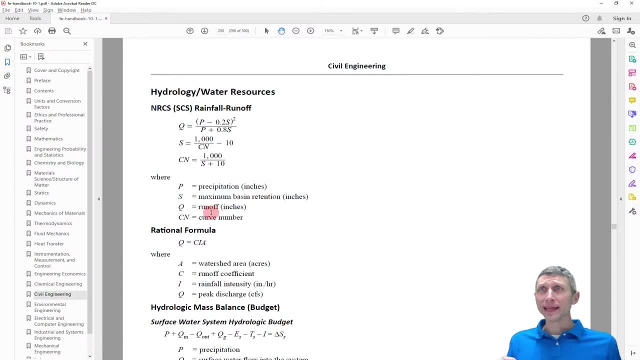 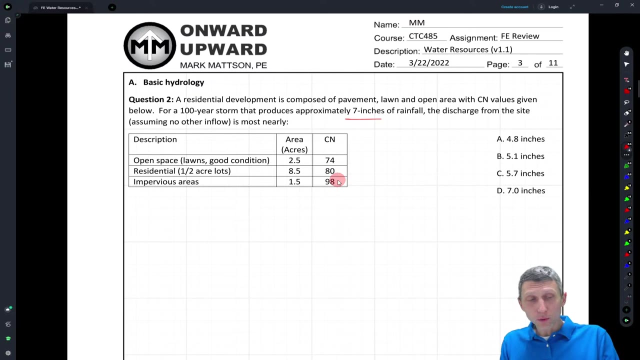 that's where you're going to go, so run off in inches. um, we have to go through this, but but really all of this depends on the curve number, and what you see when we come back to the problem is we have multiple curve numbers. so in order to get the curve number, um what we're going to need to, 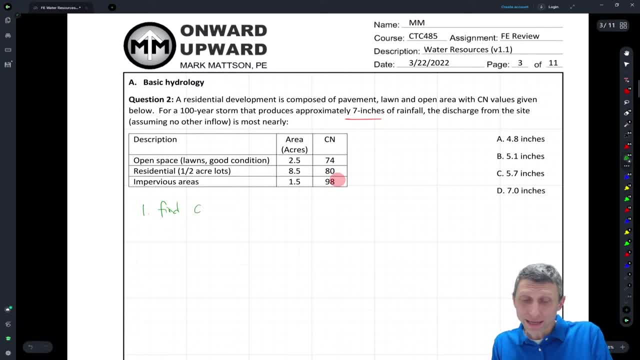 do is we're going to first need to find a composite curve number. so what we're going to do is we're basically going to say we're going to take the site and we're going to say, okay, we've got curve numbers for each of the individual. 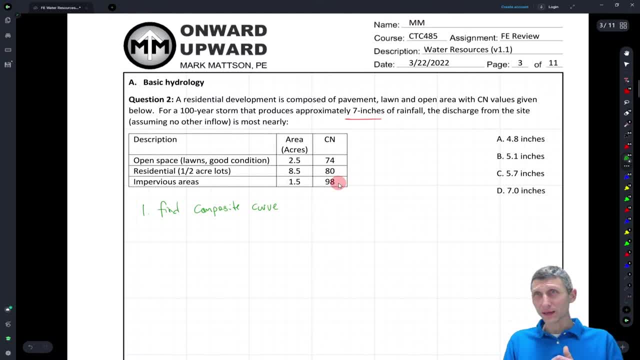 catchments or areas or, you know, parcels of this type of thing. what's the curve area or the curve number going to be for the composite site? so the way that this works is is it's essentially, um, like a weighted average, okay, and to find it, we're essentially going to 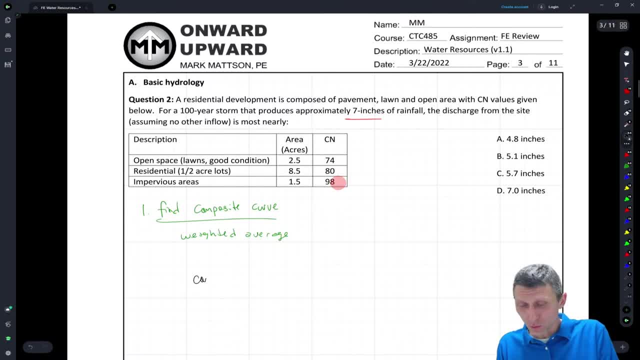 let me write down a formula here. this is not in the handbook, but um, it's just a weighted average. so the composite curve number is going to equal essentially the sum of the areas times the curve number. so the individual areas times the individual curve numbers divided by the sum of the areas. 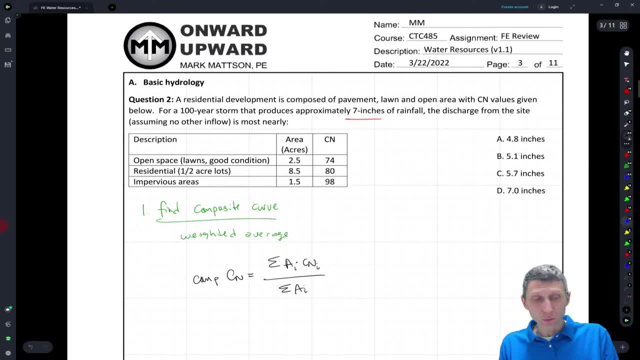 okay. so what we have here is: um, we have our areas, right, these are our areas, um, and we have our individual curve numbers and that's it right. so that's all that's once. we have that. this is pretty good, but what we need to do is we need to come up with essentially a third column where we're going. 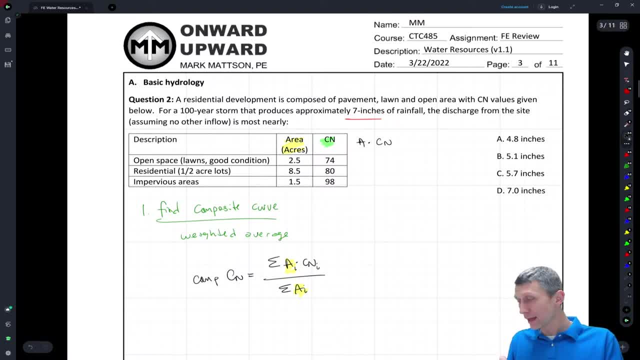 to take a times cn, right? so if we do that out, um, we're going to just get some numbers here. we're going to get 2.5 times 74, uh, i got 185. okay, 8.5 times 80, well, 8 times 80, 640, uh. 8 times 90, uh. so 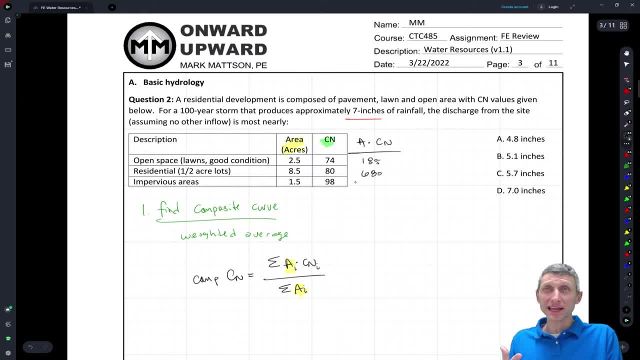 i think this gets to 680 here. uh, 1.5 times 98 again. that's that impervious area and that's going so. now, if we sum these right, if we sum this column, and we sum this column, uh, we're going to get some. 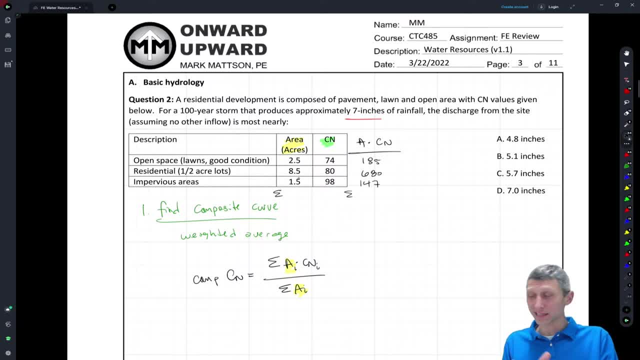 values here. so if we sum all the areas 2.5 and 8.5, that's uh what. 11, and then another 1.5, i think is 12.5, and if we add it, add up 185, uh, 680, 185 plus 680, uh plus 147, we're going to get uh 1012. 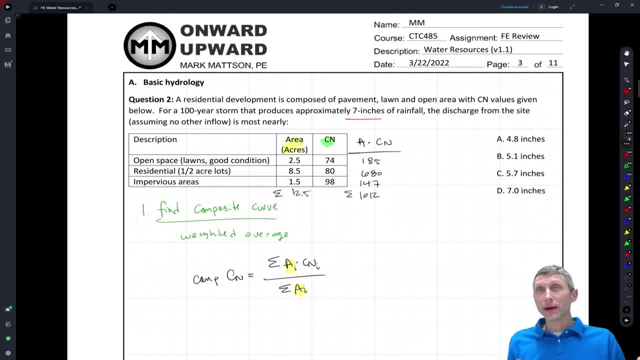 all right. so this is how we get a composite curve number and essentially what we're going to do is, once we have that weighted average um, we'll be able to go ahead and and solve this problem as well. but once you have the 1012 um, we're going to divide that by uh 12.5 and we're going to get a. 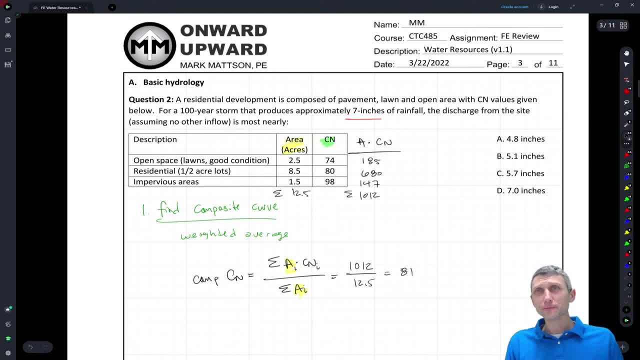 weighted curve number of about 81. okay, so 1012 um divided by 12.5, it's like 80.96, and we're just gonna round that to 81, which is good, because that gives us what we need for these next pieces, right. 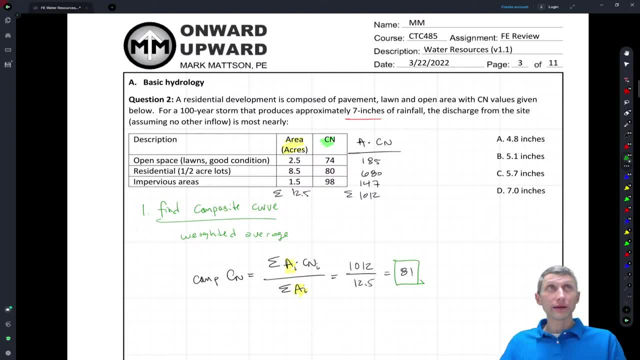 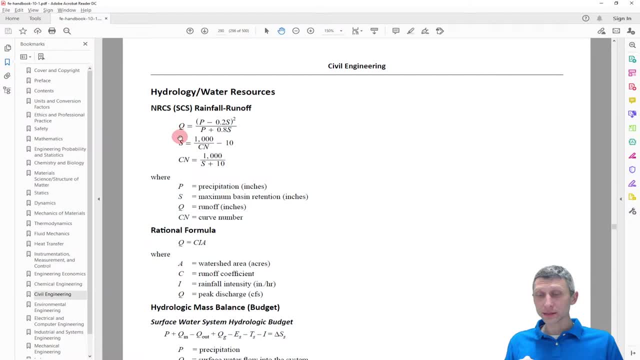 so if we come back to uh, the, the handbook, what we see here is we have two other formulas that we need to um. take a look at uh. the first here is the, the s, the s value, and the second is um, the q value. so let's write those down and solve them, okay. so i'm going to come back here. 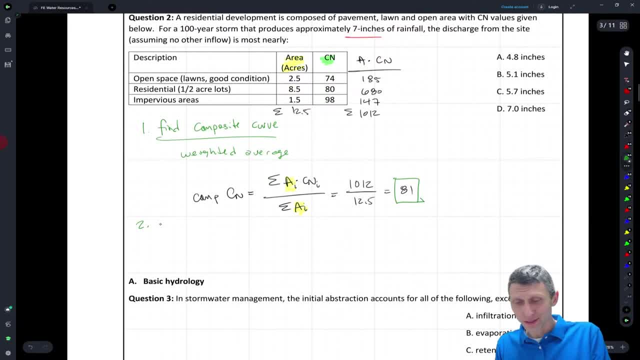 i'm going to do um second step here, kind of, and i'm just going to say nrcs um scs equations. so so we have two equations. the first one was s equals um 1000 over cn- okay, minus 10- and um. what we're getting here is thousand, uh, divided by 81 minus 10, and i get a value if i do. 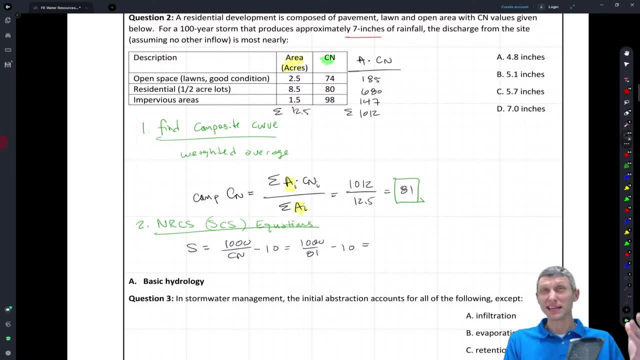 that 1000 divided by 80, point, i'm gonna even go to 80.96, why not um? and then subtract off 10 and i got like um 2.35, roughly right, so 2.35. and then the second formula was the q formula, and the q formula is a little bit. 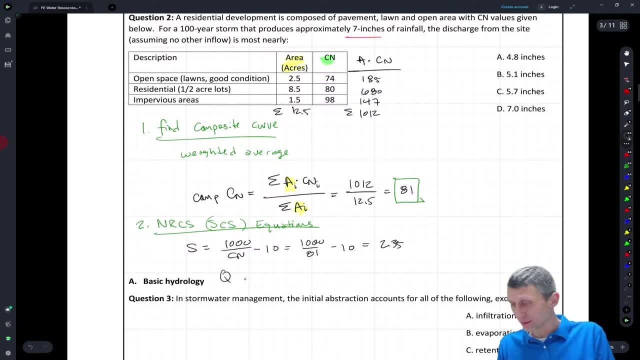 uh, a little bit more. you know it has a little bit more going on, but we're going to say: q equals um p minus 0.2 s, in parentheses- squared uh divided by a p plus 0.8 s. okay, so just two formulas. this gets the plug-in chug, but probably if you see a a question like this: 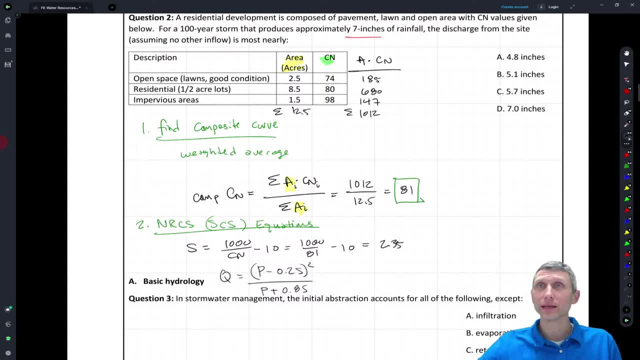 there's going to be maybe some combined uh, combined you know, or composite curve number that you have to figure out. maybe they'll just give you a curve number straight up, but at least this question kind of shows you all the different pieces that i think they could reasonably ask you uh on the fe, because they're not going to get into the other parts of it that. 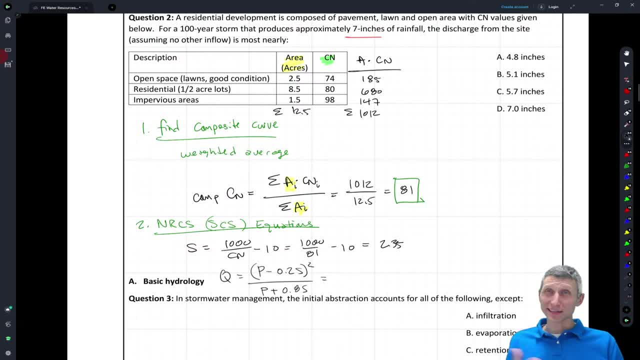 ntr 55, they start using charts and tables and those sorts of things that are not included in the handbook, but this is a legitimate question that i think could could show up. so what do we have? um, our total rainfall here was, uh, 7 inches. so if we plug in, we get 7, you know inches, minus 0.2 times our 2.35 all over. all that has to be squared and we take that all over seven plus 0.8 uh times our. 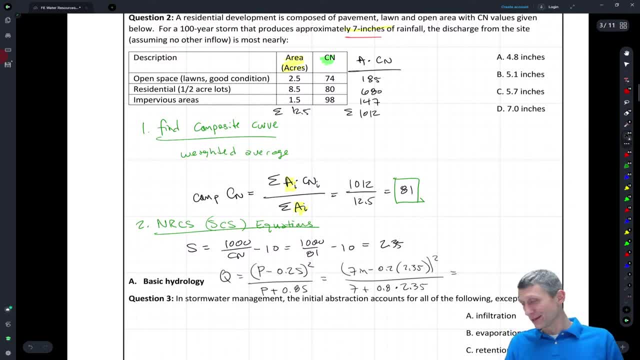 2.35 and that's gonna give us another value. so this is good calculator practice. if nothing else, um, you know, i'd suggest you you work through these or pause this and and take a look at, uh, if you can put this into your calculator quickly and efficiently, because that's going to be. 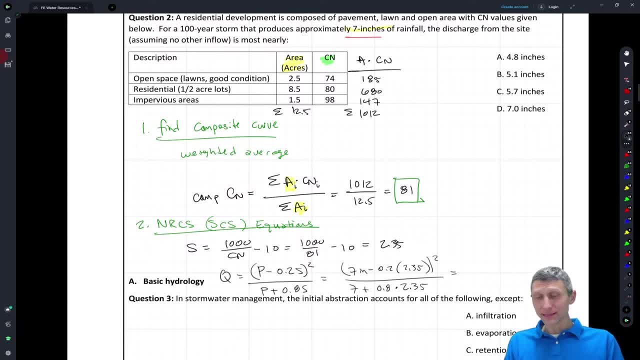 something as well that you're going to have to do on the exam and get it right. So when I put that in I get like four point eight, So four point eight inches, And again our units work out where we have inches, inches, and we end up with four point eight inches of runoff from this site. So 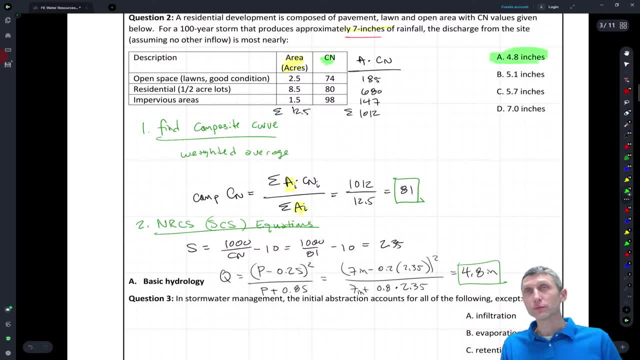 even though we have seven inches total of rainfall, right, so we have seven inches total of rainfall. two inches is either getting infiltrated or retained or somewhere. It's not going off the site, OK. it's getting soaked up and staying on the site, All right. So question: 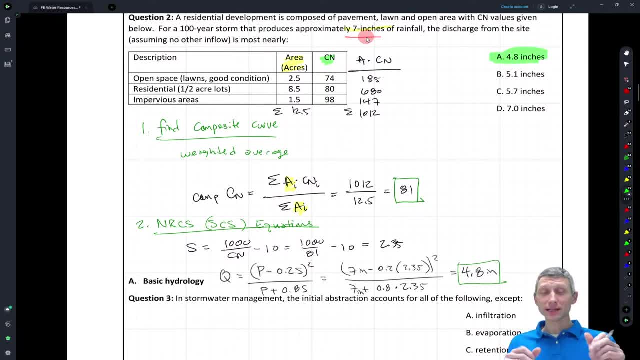 number two is done, All right. So if you have questions on it, definitely drop a comment, But hopefully you've seen some of this stuff before and hopefully it makes a little bit of sense. As we're going through this. I'm going to move this up just a little bit to make a little bit. 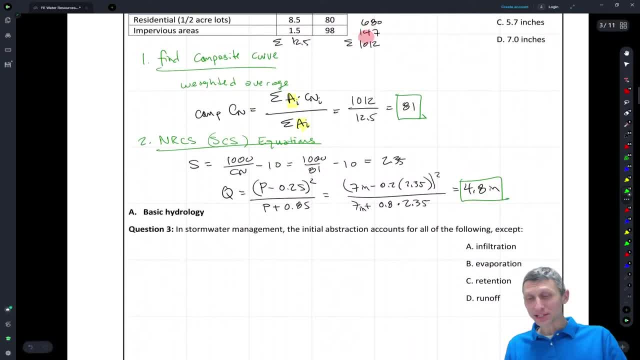 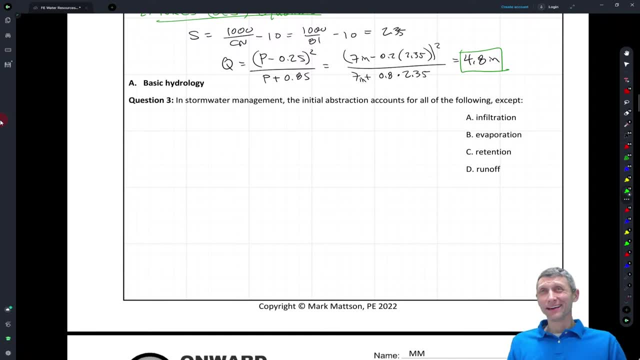 more room here, All right. Next question is a conceptual question. This kind of gets to what we were starting with in the first place has to do with the idea of runoff Right And in stormwater management, the initial abstraction. So this is kind of the key word that we're looking. 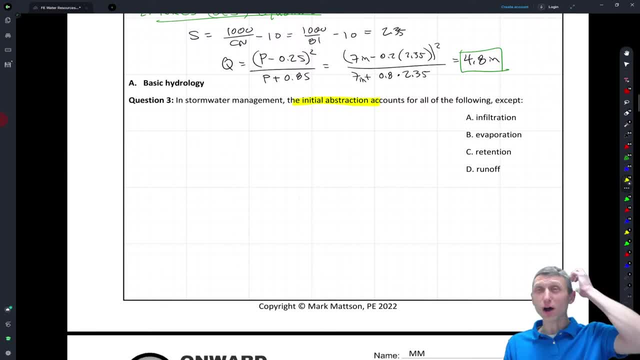 for here. The initial abstraction accounts for all of the following except- And maybe you never took a hydrology class in your undergraduate career or set of courses or program of study that you had to do, But this is one of those concepts in basic hydrology that 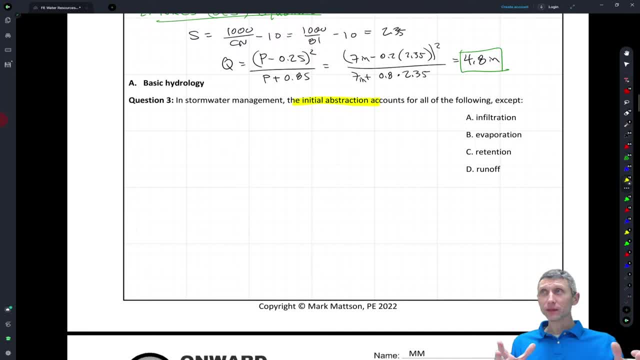 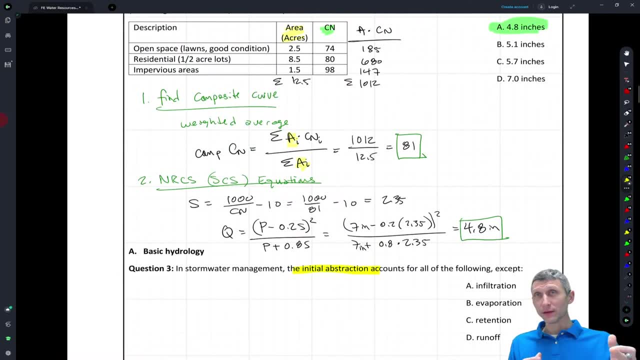 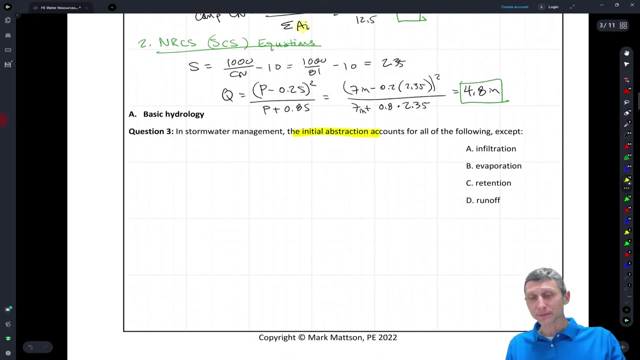 is going to make a difference. So, just like you're going to have basic kind of curve numbers that have an impact of or have that account for that initial infiltration, the initial abstraction is the same thing. So the initial abstraction has to do with the idea that when water hits, 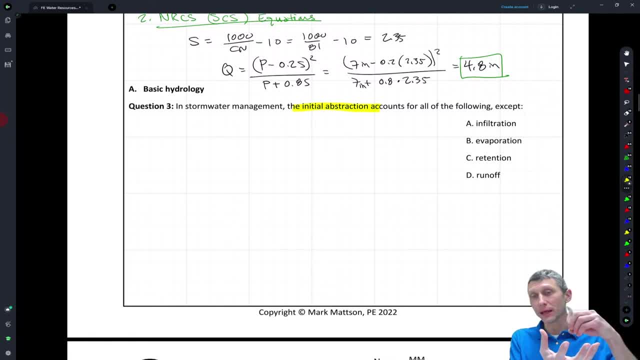 this site, there's an initial amount that gets soaked up, that that doesn't actually go off the site Right. So that's, that's going to be your initial abstraction And with that in mind, now we're looking for. OK, well, that initial abstraction you know you have. 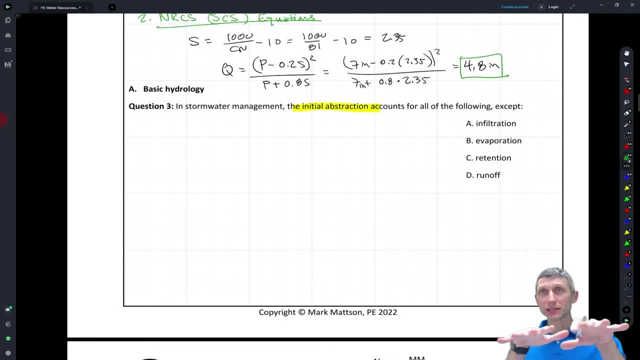 a dry site, you get it wet. There's some of that water is just going to get the surface wet. It's not going to go anywhere. OK, And that's the the initial abstraction. So infiltration, that accounts for that initial abstraction. evaporation: Right, You have a really hot surface. You hit it, You're going to get some. 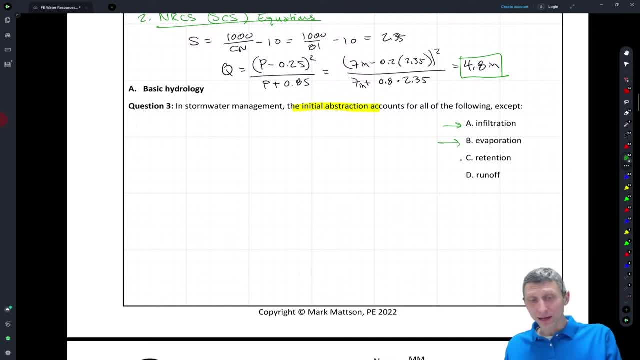 evaporation right away. OK, Retention, retention, Again that's going to be. you got little pockets and divots, even an asphalt- Right, Even an asphalt. or you have some little pockets, divots that are going to hold on to water. So these all hold water Right, These all hold or retain. 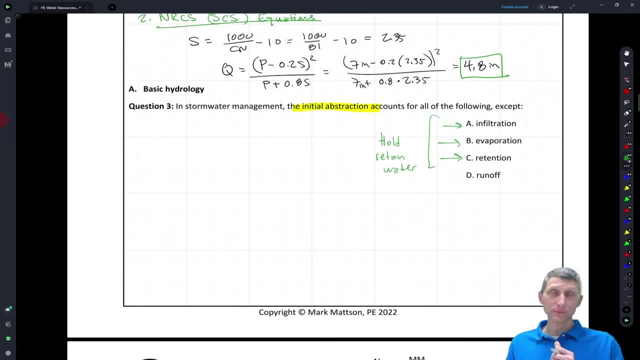 water. That all accounts for part of your initial attraction. And obviously you could have a retention basin where you're retaining a whole bunch of water, Right, But that's, that's not the initial abstraction. The initial abstraction is just: you have the surface roughness. 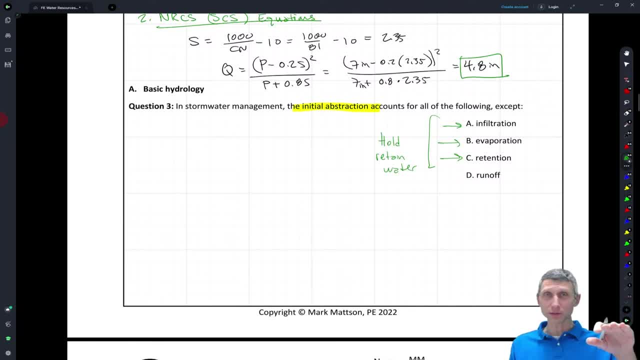 even in like pavement for example, you got surface roughness, little divots, little holes, little pockmarks that are going to hold little drops of water, So you don't get 100 percent of that water running off And obviously in soil you're going to probably have a little. 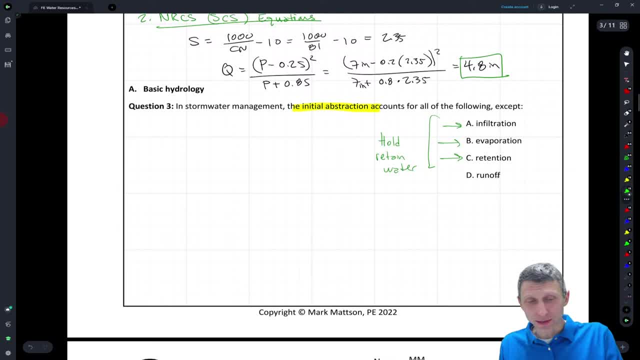 bit more. OK, And what's left off of what's left here is runoff. So the initial abstraction is not runoff. Runoff is the opposite of the initial abstraction. All right, So concept question. I can see concept questions like this. I mean, have you taken a hydrology class, You kind? 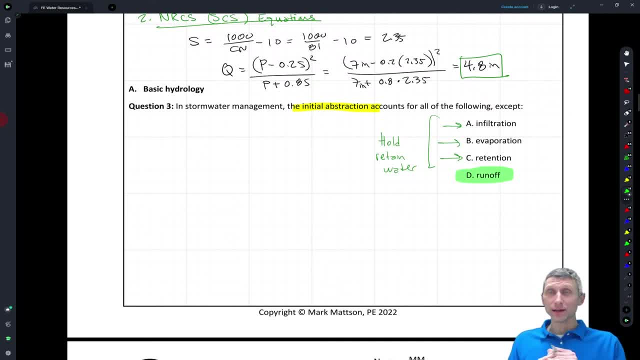 of have an idea of what that looks like and how it's going to play out, So I don't know. We got a handful of conceptual questions on this And some of it comes from when I was working- consulting full time- and I worked for a. 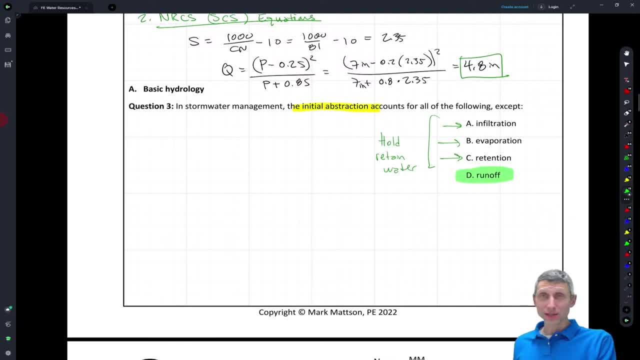 OK, A water resources dam engineering firm. So we did a lot of different things, from stormwater through dam design and all that sort of thing. So some of that's going to come out in some of these concept questions that I throw out here to you. But hopefully they help broaden. 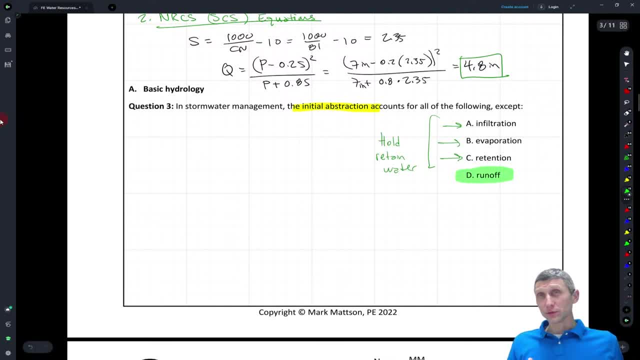 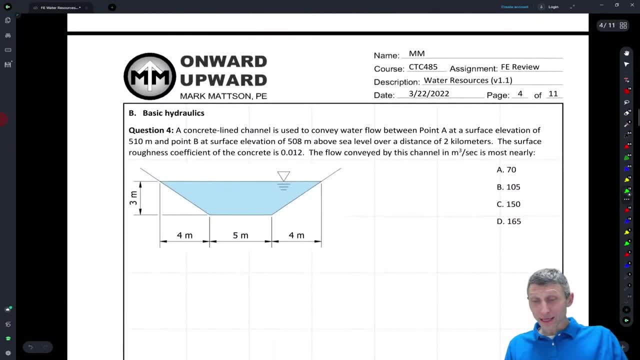 your knowledge, And that's kind of one of the things that I'm trying to do with these review sessions is hit all the topics, but hit them in a way that broadens your knowledge and perspective. So let's keep going. So, question for concrete line change. 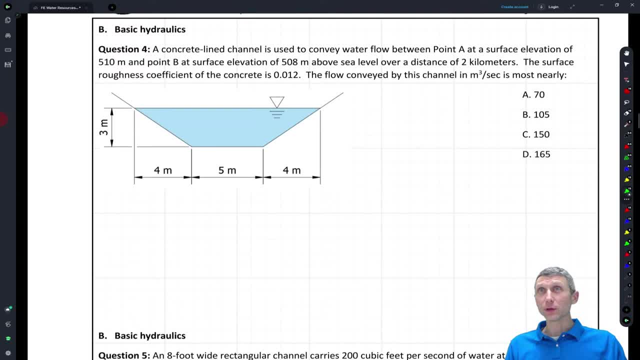 This channel is used to convey water flow between point A, at a surface elevation of 510, and point B, surface elevation of 508 meters above sea level, over a distance of two kilometers. The surface roughness coefficient of the concrete is 0.012.. And this 0.012 is one of those those 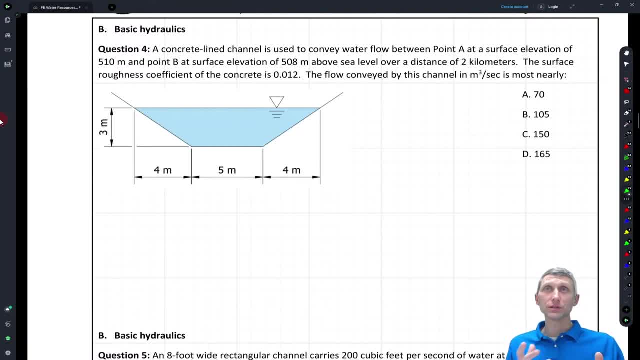 values that should set off kind of triggers in your mind as to what you need to do here. Because what the question then it goes on to ask is the flow conveyed by this channel in cubic meters per second. Most nearly So we got to get flow, But that surface roughness coefficient screams and 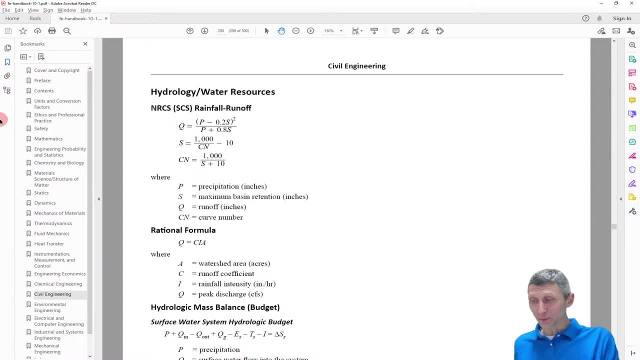 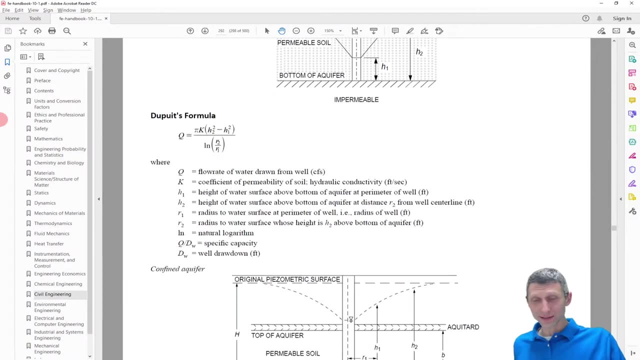 hopefully you're remembering it screams a certain formula. But if you don't know what formula it is, you can come in here and start to look and say, oh, I don't know, Where is it? There's Darcy's law. No, not Darcy's, not Dupuy. You know, we got some things going. 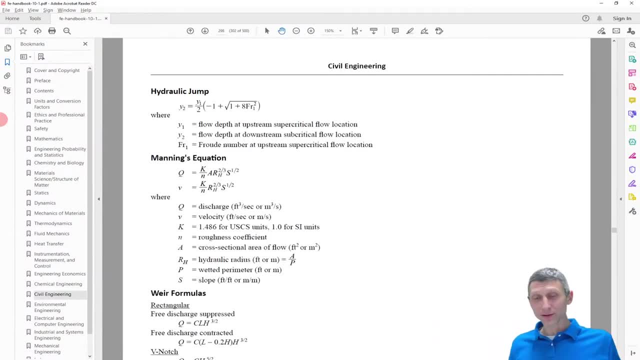 on here. Where is it? It looks like right there Manning's equation. OK, we have a, An end value here, a roughness coefficient, This coefficient that we're going to be using. So this gives us a formula, And I'm actually 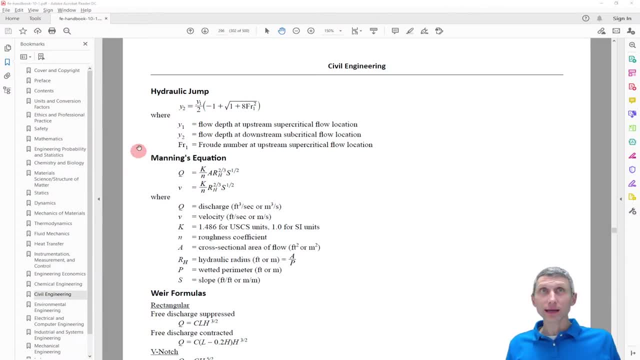 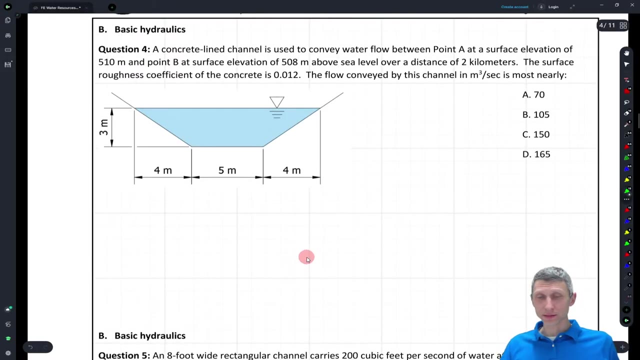 just going to copy this formula over. Why not? So if I copy that formula over, let me just do that quickly and we will maybe make this work a little bit better here. But let's take a look at this formula and I'll come back and hopefully this will make it kind. 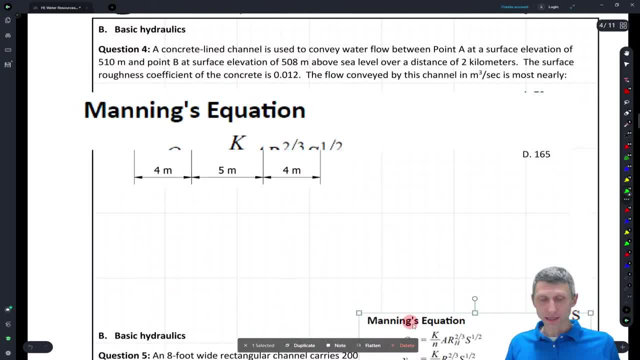 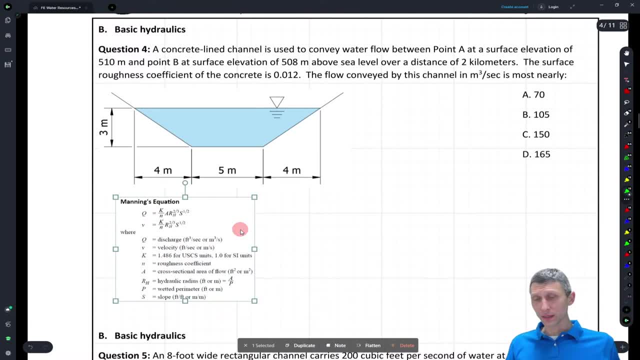 of nice for us, so that we can put it all together and see what the handbook says all at the same time. OK, so here's our Manning's equation And this is what we need to solve for. So that's a little small, but hopefully it's readable. So we need to solve this right And we have 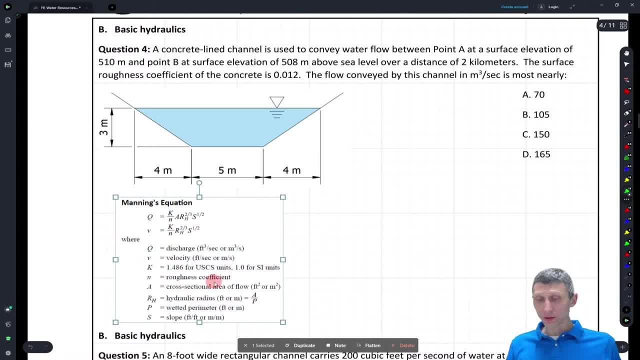 a few different things we have. We're given, and that's good. We know that's point zero one. two: We know this K value we're using as imperial or SI units. I'm sorry, we're using SI units, So this is going to be one point zero for SI units. What else do we need? 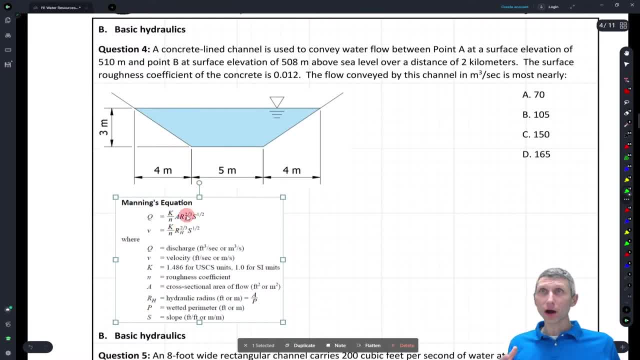 We need a. so we need the area of this thing, We need our age, which is going to be the hydraulic radius of it, And then we need the slope. So let's just work through each of those pieces, Right? So let's start with. let's just start with each of those pieces, So we 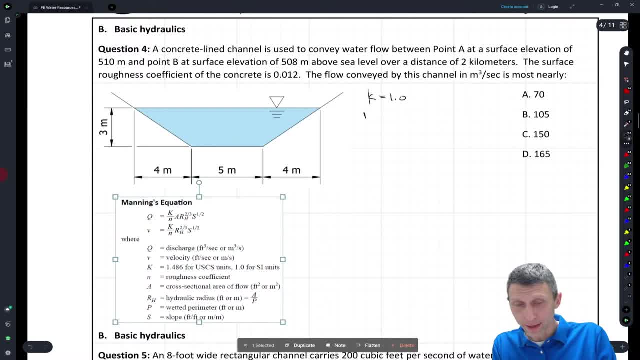 know that K equals one point zero. We know N equals zero point zero one two. What's next? We're looking for flow, So we're going to need the area And the area is going to be the area Of flow. So I'm going to just highlight this here. So if I highlight this area, right. 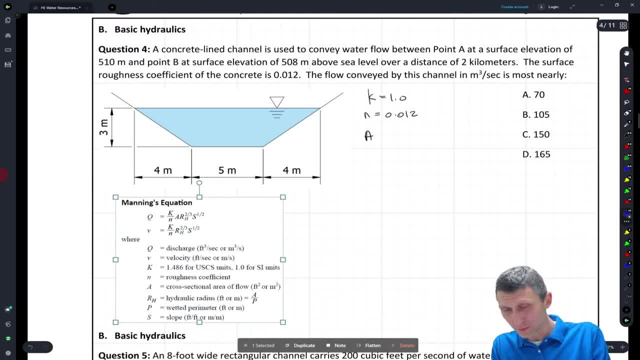 this is going to be the area of flow that we have to deal with, Right? So that is our area. So what is that? That's just going to be. well, this is a trapezoid, It's it's so. we're going to do one half of the bottom height, which is five meters Plus the top height. 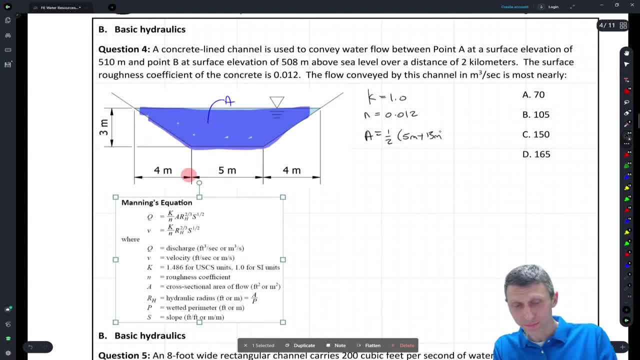 So five plus eight is going to be 13 meters. So that's our average height or, I'm sorry, average width of this thing. And then our height we know is: is this three meters? So if we multiply by three meters, what are we? 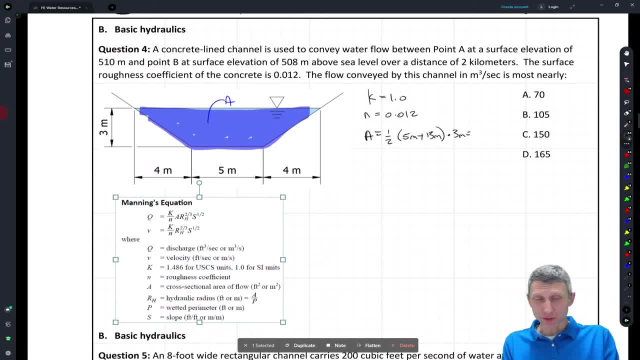 going to get? We're going to get one half of what's this? 18?? That's nine times three is going to be twenty seven square meters, And what's what's our age? So the next parameter that we have here is our age, or the hydraulic radius, which is just a over P. So they tell. 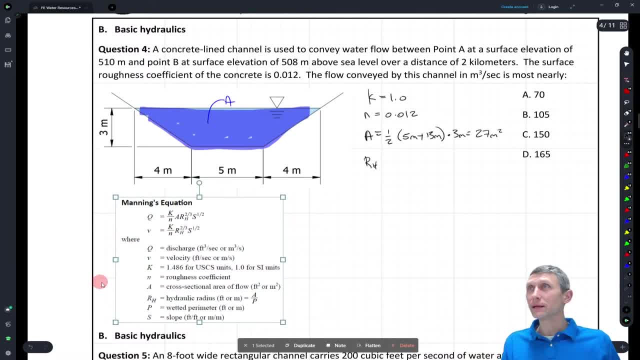 us. this is a over P, And this is where P is The- The wetted perimeter- Right. So P is the wetted perimeter And what that looks like here is- I will highlight this too- But the wetted perimeter is the parts that are wet Right. 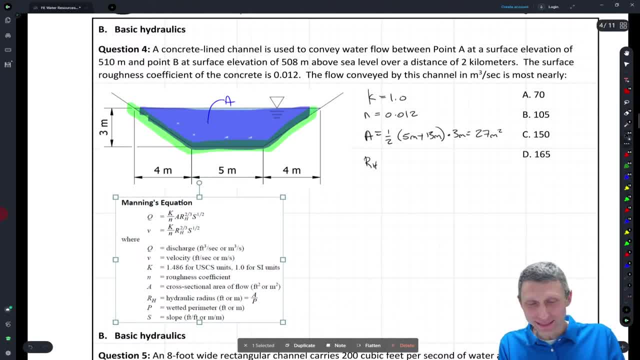 So the parts that are wet. So we can just add these distances up And if we know we have three and four, we're going to get a three, four or five triangle, And I mean you could use Pythagorean's theorem there. but each side is going to be five meters because 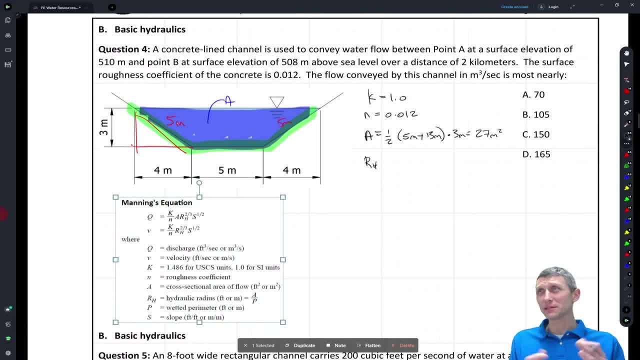 it's, it's, it's consistent. I don't know. I mean, I don't think that if he's going to try to trick you a ton with like crazy dimensions or anything, it's more so. you know the concepts Right. So what do we have going on here? The perimeter is going to be what? Five plus five. 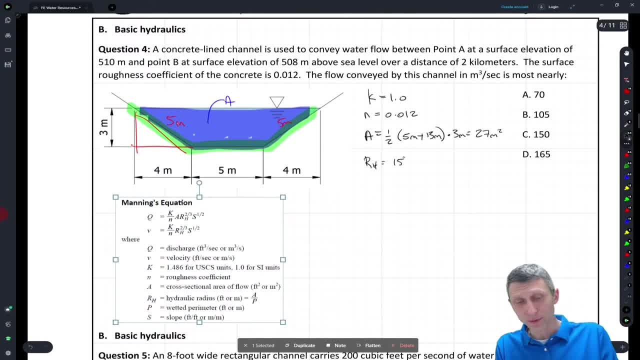 plus five is going to be 15.. I'm sorry, That's the perimeter, So let me start over. The hydraulic radius is the area over the perimeter. So we've twenty seven cubic meters- I'm sorry, Square meters, Man, it's early- divided by the perimeter, which we said was 15 meters. 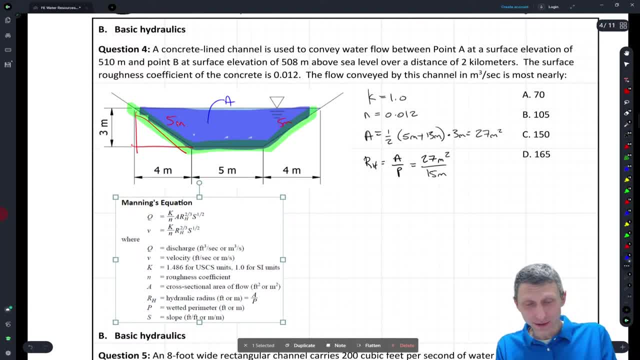 Right, That's the area. This is the area Right Divided by this perimeter, And that's going to give us what Twenty seven divided by 15.. I think that's it works out to be one point eight meters. OK, so what's our next? what's our next coefficient? here is S for the slope. 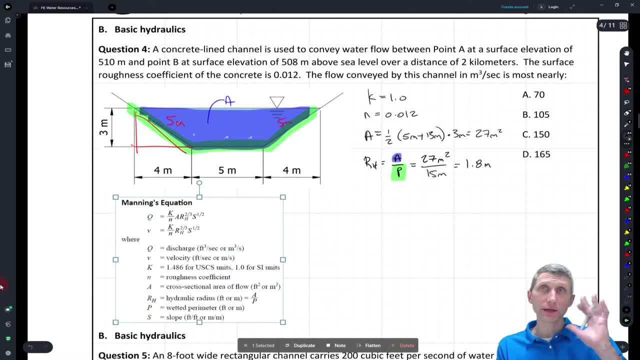 So this is feet per feet or meters per meter. So again, just looking at those units, understanding those units, is huge. on this test, Just knowing what the equation or what the units are in each equation is going to be super important. So we get a slope here. equal to well, we essentially have the fall, which is going to be we go from. 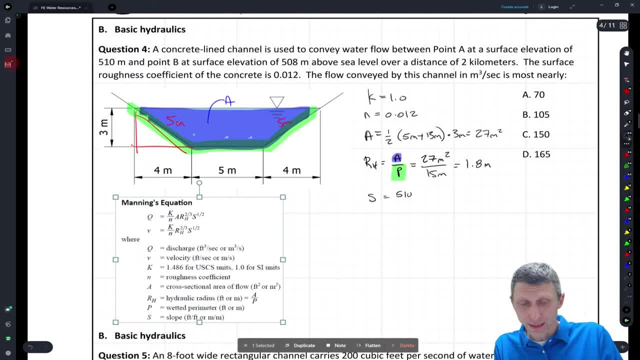 five, ten, down to five to eight. So that's, you know, five, ten meters minus five or eight meters, And this is over a distance of two kilometers. So two kilometers Times what One thousand meters per kilometer. So what do we essentially get? Two divided by two. 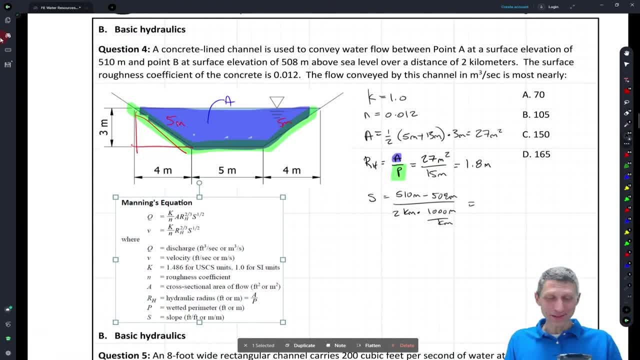 thousand, And if you're not super confident with your decimal division here, it's OK, You can put this in your calculator and there's no shame here. I get point zero zero one meters per meter. OK, Once we get that right, these are all our variables. 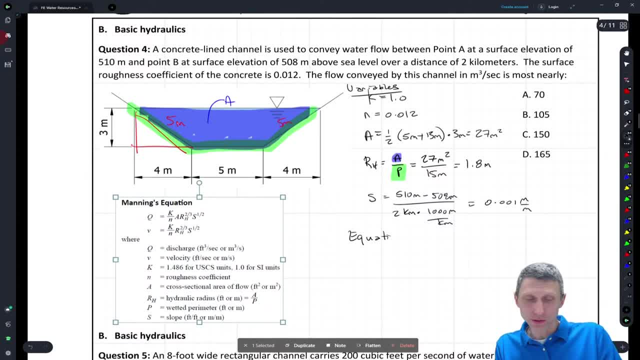 Once we have all our variables, we can just start to plug and chug here into the equation. I've also seen some problems. you know where it's like. it might not be a full Manning's questions, It's just find the hydraulic radius. 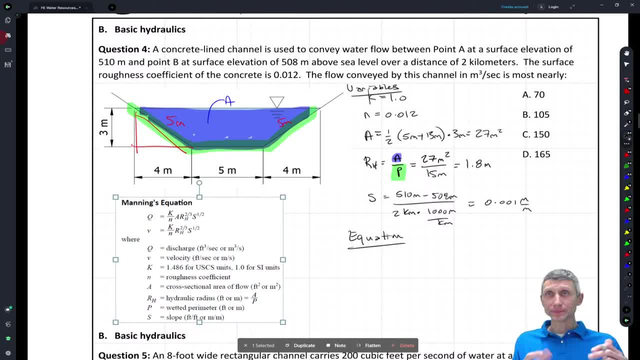 And again, with that, you're just looking at the area divided by the perimeter And that's what it's looking like. So what do we get here? We get Q equals one divided by zero point zero, one two times Times. what was next? 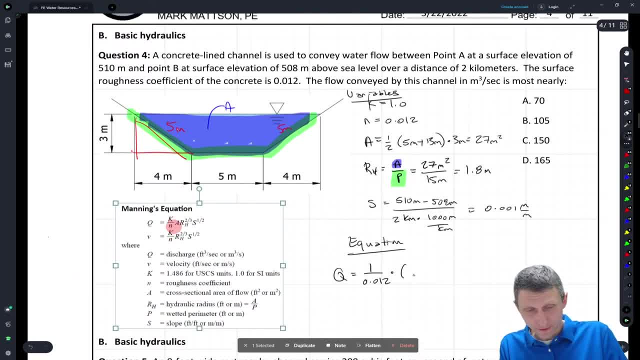 So times a, So the A here was twenty seven meters squared, Sometimes the hydraulic radius of one point eight Meters to the two thirds power. So make sure you know how to do that one on your calculator. It's not just a square button. 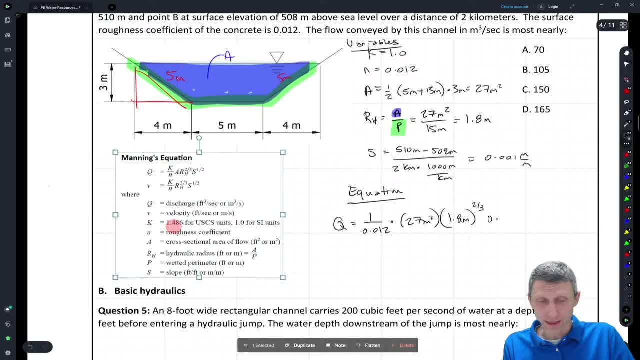 You have to put the two thirds in there. Make sure you get it in parentheses, unless your calculator is in the mode that doesn't need parentheses. But the good thing here is, all the units work. So we have meters, squared meters and the slope in meters per meter. 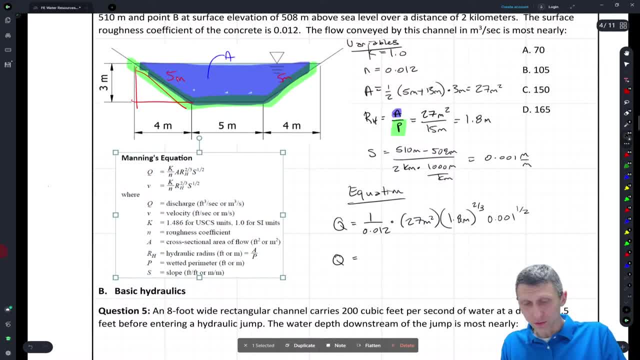 So all our units are consistent And when we solve this, hopefully we get the right answer. That's all. It's always good when you get the right answer, But one divided by point zero, one, two times twenty seven times one point eight. 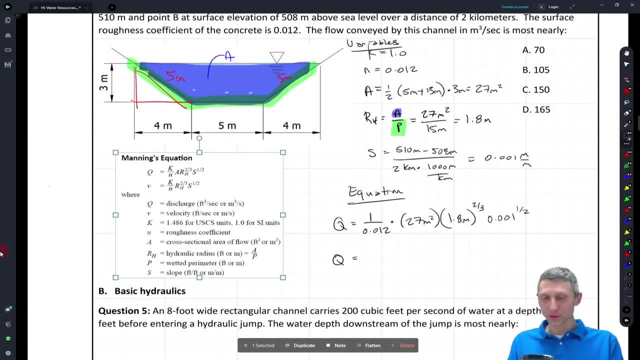 And then what I do here is just to the two thirds power. You can put two thirds directly in to the calculator, But make sure you hit that over button to get down again from the calculator times. point zero, zero one to the point five, I get about one hundred and five, point three or most nearly one hundred and five. 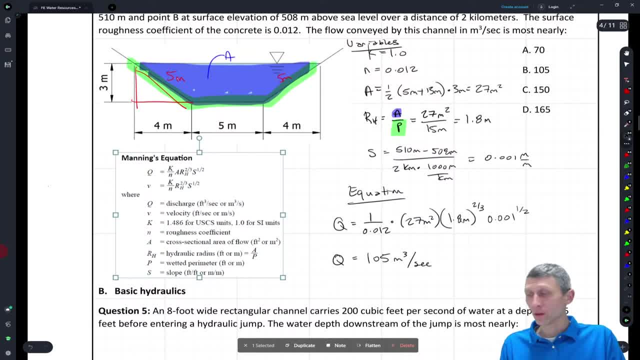 cubic meters per second. OK, So just use a manning's equation. But this brings up a bunch of a couple of different topics. One is just a hydraulic radius, Two is a slope of a channel, and three is kind of this, this idea of how to calculate the flow. 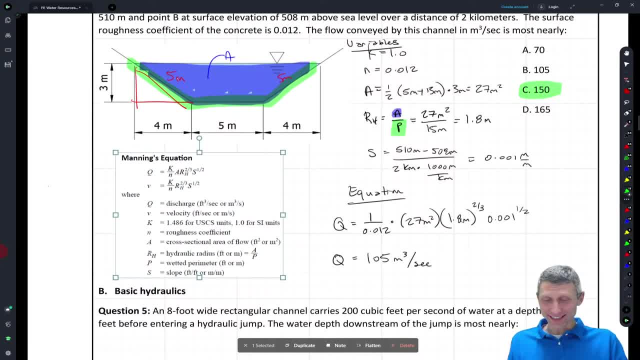 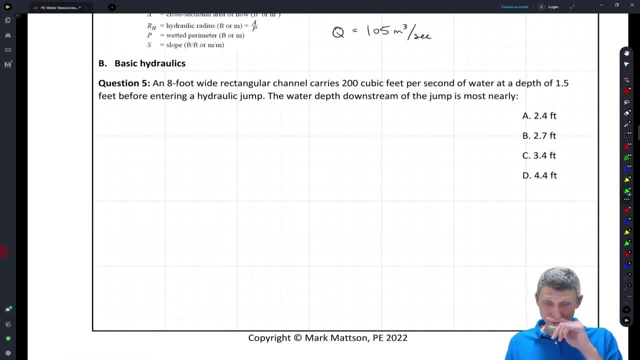 All right, So question four is done. All right, Got that back to question five here. So we've got an eight foot wide rectangular channel, Carries two hundred cubic feet per second of water at a depth of one point five feet before entering a hydraulic jump. 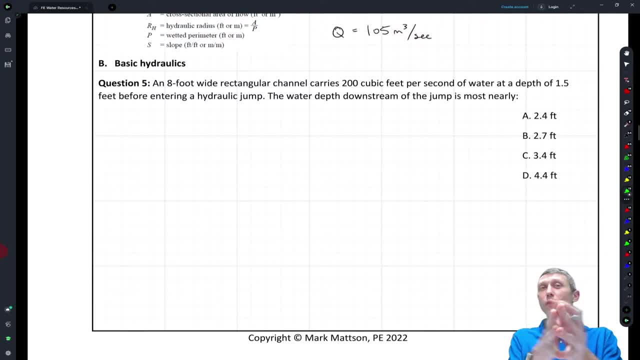 So what's a hydraulic jump? I guarantee every one of you is probably seeing a hydraulic jump today. Do you know where? If not, you'll you'll never wash your hands again the same, because when you're washing your hands, let the water go for a second. 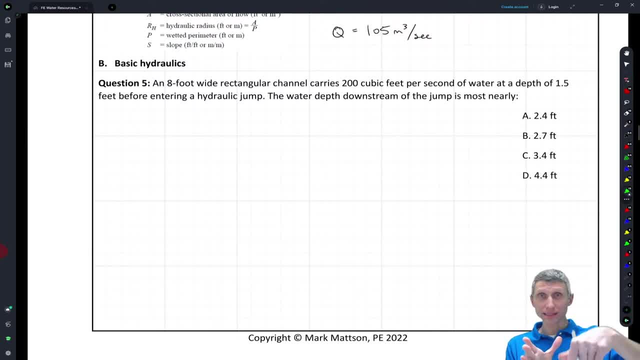 Just look down and see what happens, Right. What happens? that water hits the sink, the sink bottom Right, And it splays out, And then, all of a sudden, It's some radius from the center, It jumps up Right. 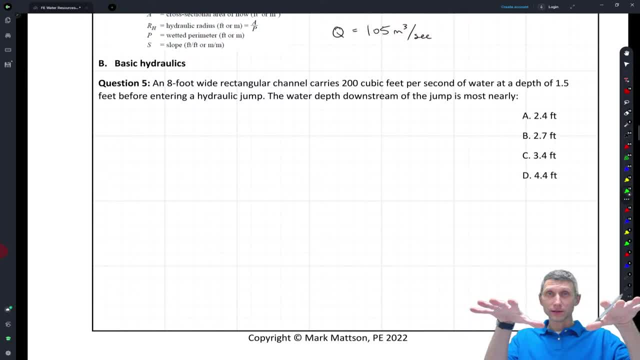 So it goes from this fast smooth flow to a jump kind of you know smooth flows, But it's that's a hydraulic jump, And you'll see that any time you wash your hands, hopefully. But but where does that occur? 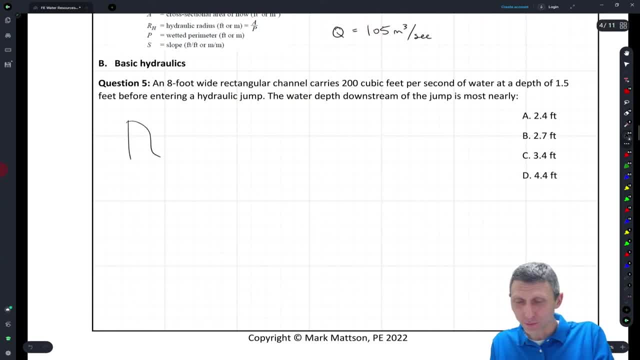 A lot of times it occurs like, for example, if you have a spillway, Right, So we've got the spillway and let's see what happens with the spillway. Well, what's going to happen with this spillway is we're going to come down with water. that's fast and furious kind of off the spillway. 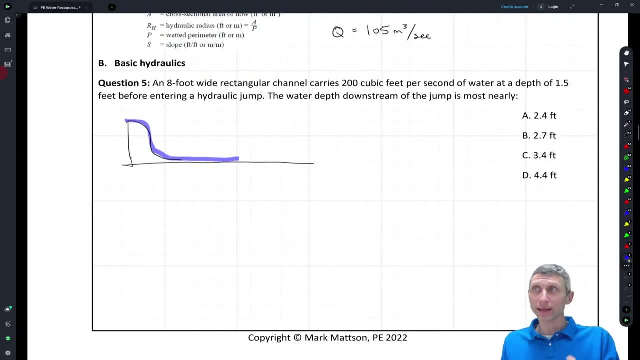 It's going to go down Right, And then the slope is going to kind of flatten out a little bit. It's not going to be a steep and it's going to, you know, jump up here in. the velocity is going to slow way down. 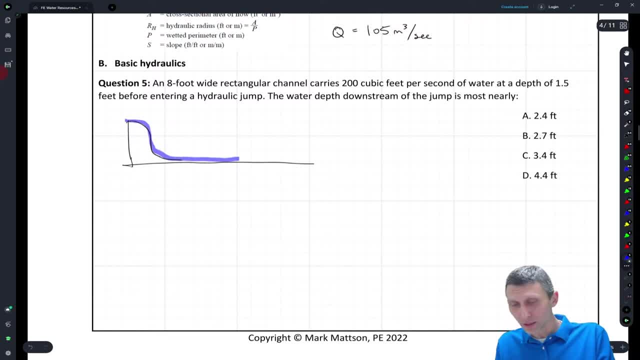 OK, the velocity is going to slow way down, So there's going to be this jump here, And what we're trying to do is we're trying to find essentially This height. Right, So we're trying to find this height here. 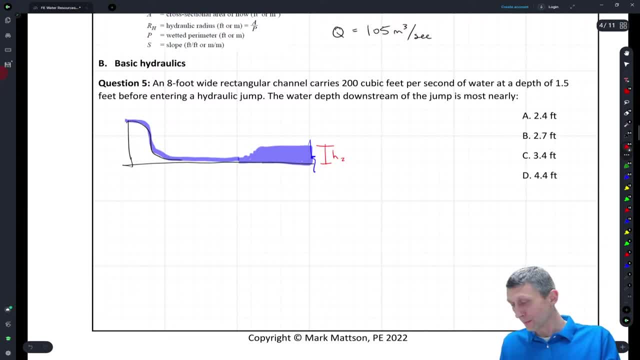 This is going to be. I'm going to call this like height two, OK, Or actually, to be consistent with With the notation in the reference handbook, I'm going to call that Y2.. Well, where's Y1?? Y1 is just this value here, which is going to be the supercritical value. 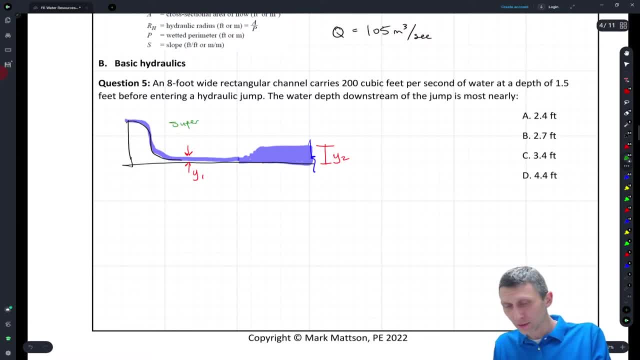 Right. So this is: there's supercritical flow And there's subcritical flow, and those are two kind of concepts that you need to understand a little bit, But we got this really fast: water It's going to. it's going to go supercritical. 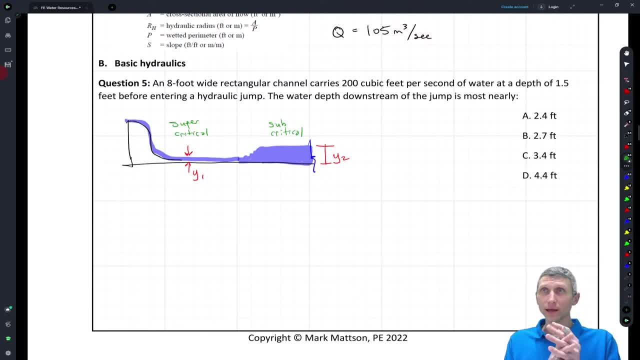 And then at some point, if the Slope, you know lessens and you know, especially downstream of a dam, you see that- or downstream of the spillway, you'll see that work goes to where there's all of a sudden this jump and it goes to subcritical. 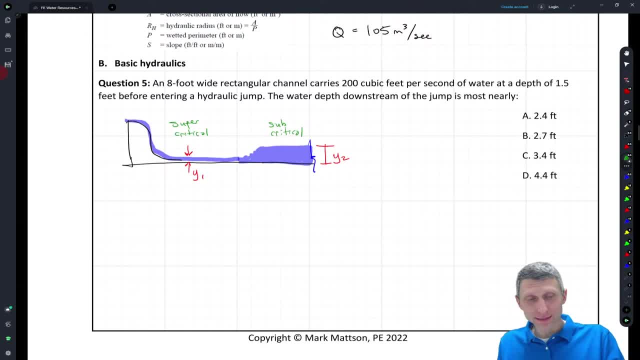 So what we want to do is we want to find that in this, this- this brings up a couple of ideas that I think are worth talking about, in kind of this hydraulics section, But what we're told is we're told that we have an eight foot wide channel, 200 feet per second, a depth of one point five feet. 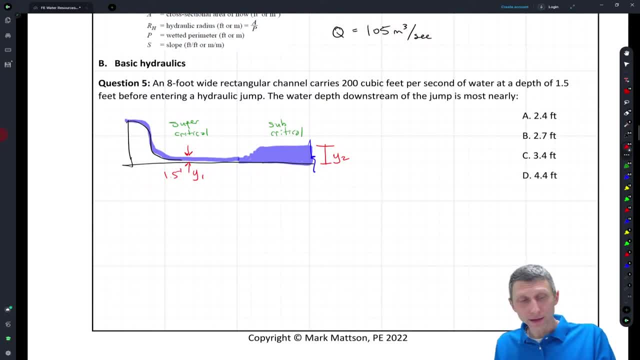 So up here we have one point, five feet. We've got a queue here of, you know, a queue of 200 CFS cubic feet per second, And so what we want to do is we want to find our hydraulic Well, we want to find an equation for this hydraulic jump and we want to go and calculate what that looks like as well. 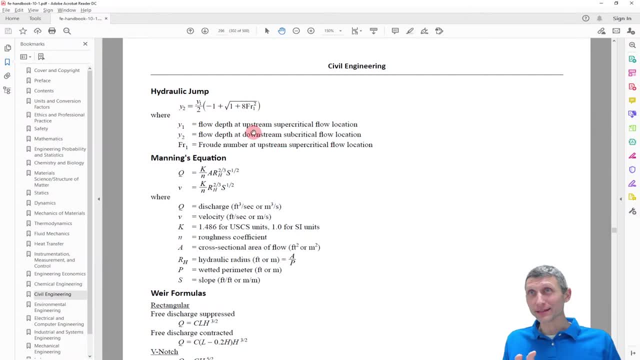 So we're going to come back and what we see here is we're on the same page. So we've got a hydraulic jump formula here. Why don't I sniff that too and bring it in, Just To make our lives a little bit easier? so we have less jumping back and forth. so we have a little bit less jumping back and forth here. 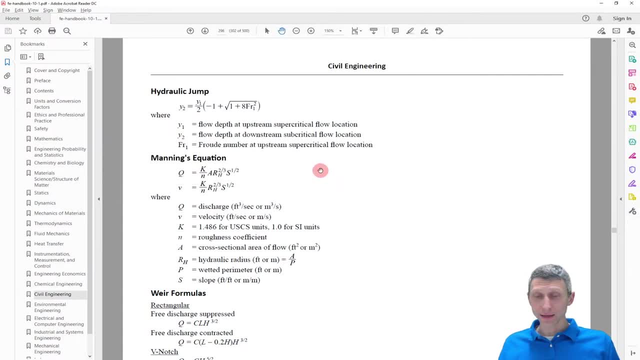 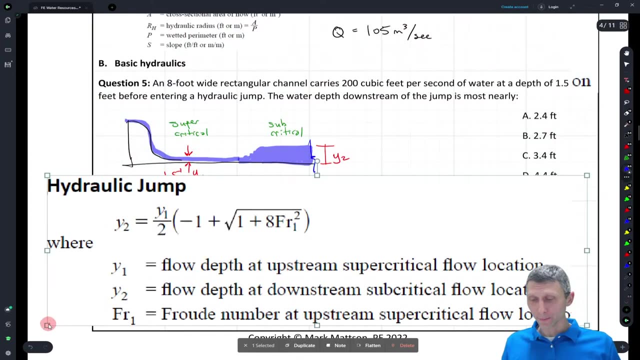 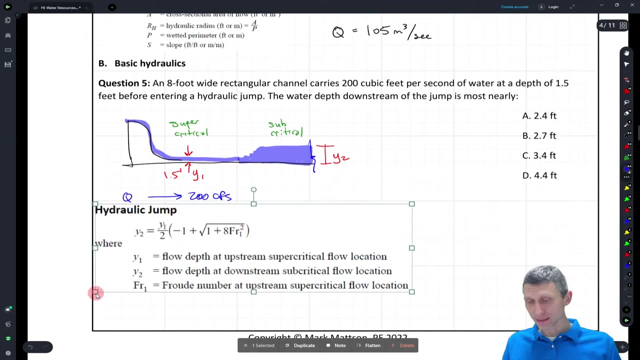 So if I bring this over and come back, We're going to use this formula now and bring it in here, OK, so this gives us a hydraulic jump and it's it. it's a little bit more complicated than what we just did with. 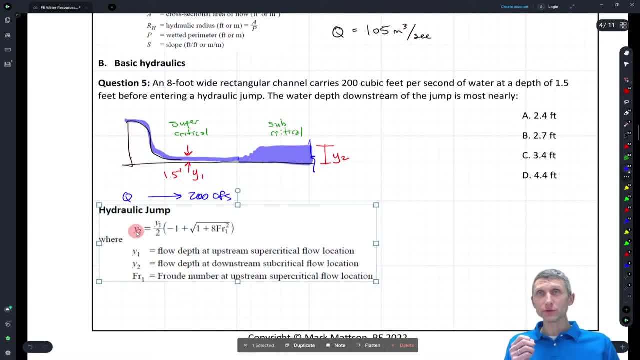 Manning's, because the hydraulic jump, it gives us this Y2 value, which is great. We found our equation, We know what to do, except it brings us to this, to this idea of the Froude number, and the Froude number is is, it's a character. 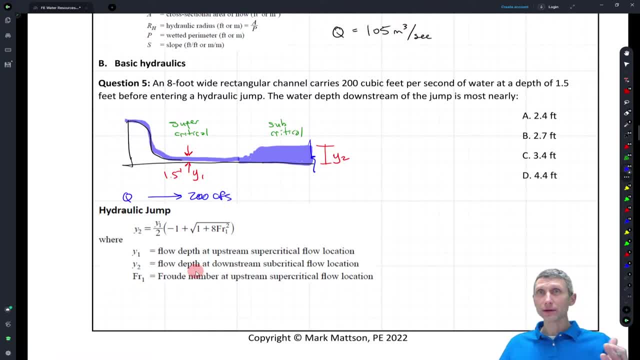 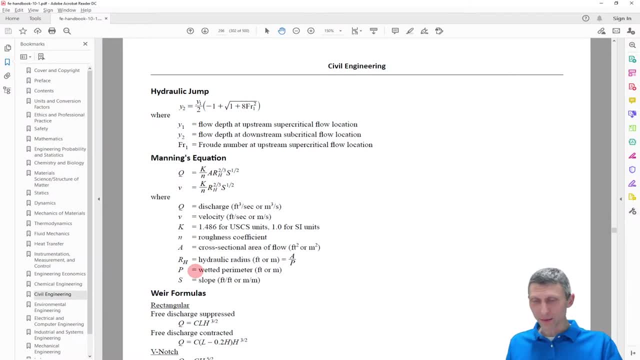 It's a, it's a number that you can calculate to basically figure out whether or not something is super critical or subcritical, And I mean, that's a kind of a simplified version of how to say it. But but here in that reference handbook we're given a Froude number. 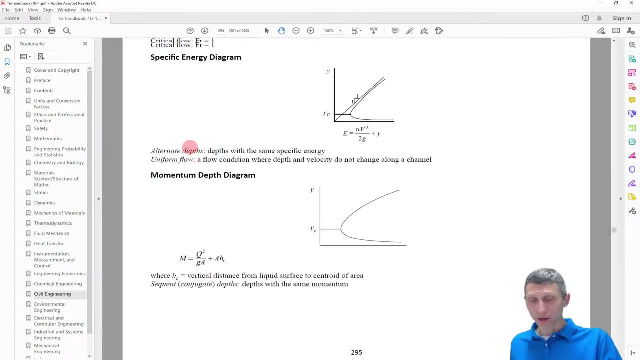 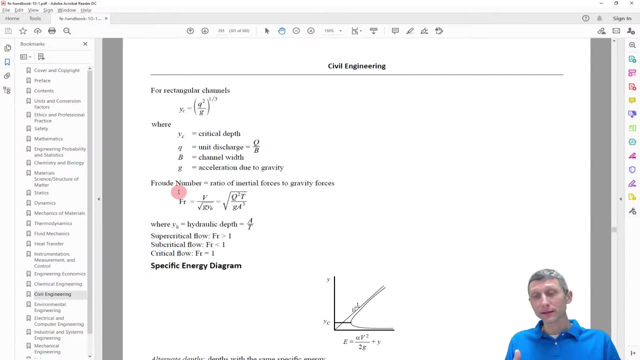 But we have to come back to find out how to calculate that Froude number. And in here it is So. for rectangular channels we have a critical depth. We can calculate the critical depth, but we can also calculate the Froude number. 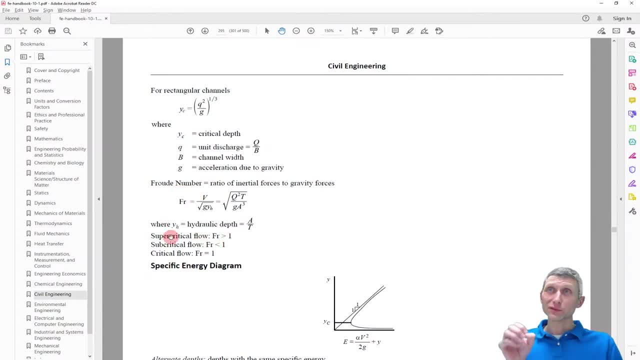 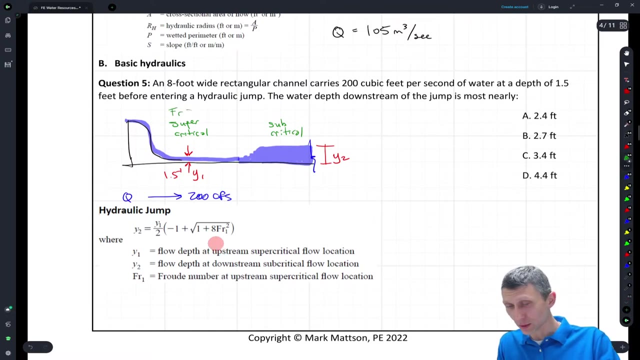 And what we see here is, if the Froude number is bigger than one, we're going to have super critical flow, And if it's less than one, we're going to subcritical flow. So what we would expect is what we would expect is, you know, on one side here the Froude number is is greater than one. 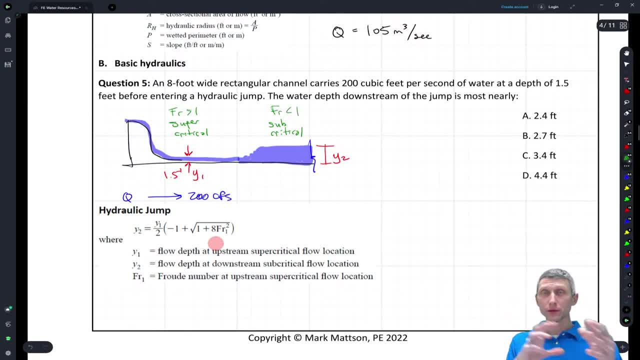 And on the other side, the Froude number is less than one, Right. So we go from. you know, we transition here and we have to go find it. So what I want to do is I want to calculate the Froude number so I can go and calculate my depth, because that's what the problem is asking. 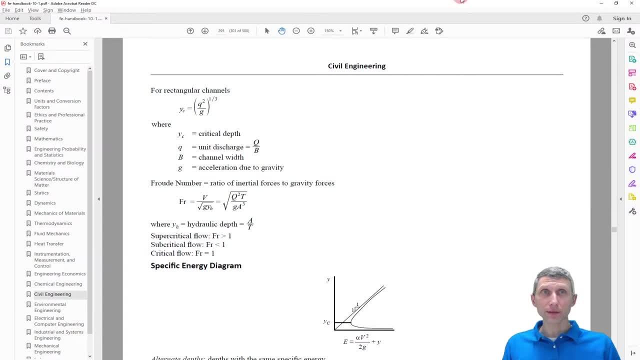 OK, so I'm going to take my Froude number back here as well, And let's let's pull that one in as well. So if I slip that one in and on the test you're going to have both. you know both. you're going to two screens here. 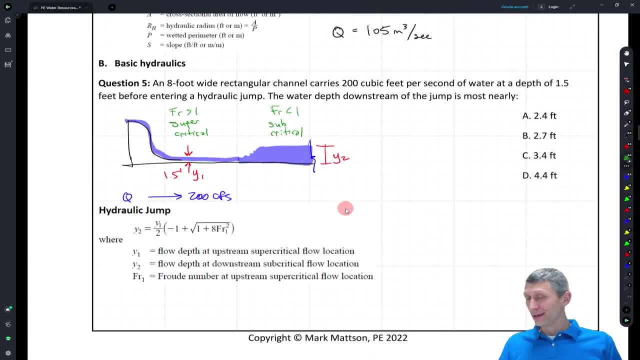 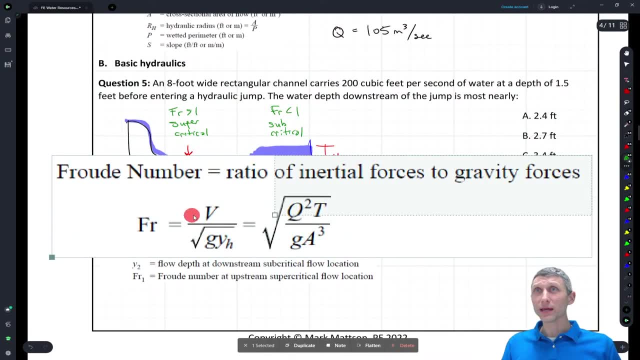 I don't have. I have that luxury as much with what I'm doing, and hopefully this works for you as well. So I'm going to bring this down here because I want to get this equation right and I don't want to screw it up. 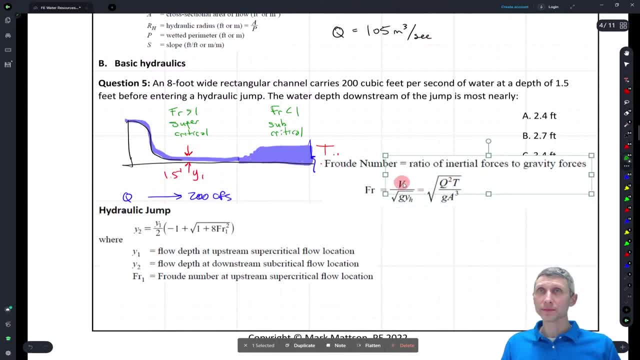 OK, so I'm going to bring my Froude number equation in and let's solve for the Froude number and then we can solve for our depth downstream of the jump. So step one, you know, we're just going to solve for Froude. 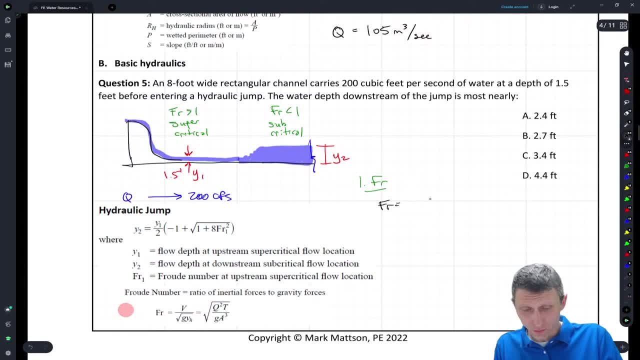 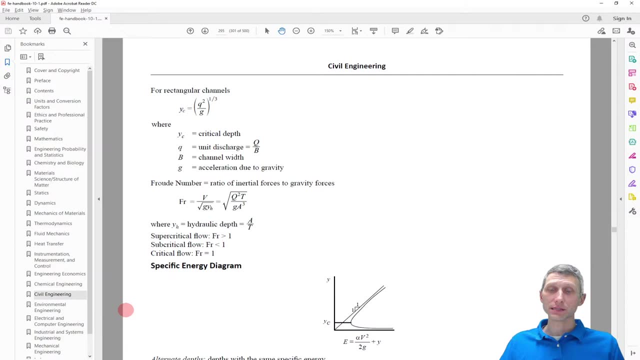 And that's going to look like this. So we're going to have. What do we have? We have the square root of Q squared, So Q here was 200 cubic feet per second times T, And I do have to come back to the handbook for a second here because T is where did it go? 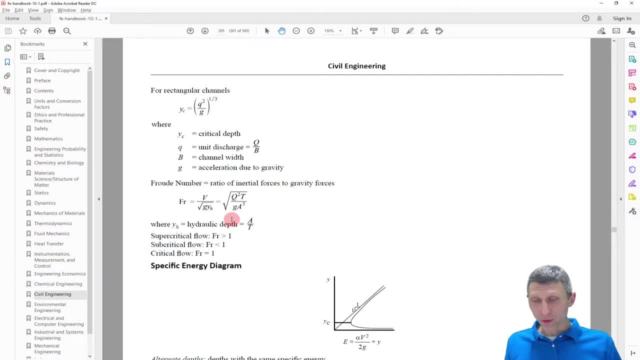 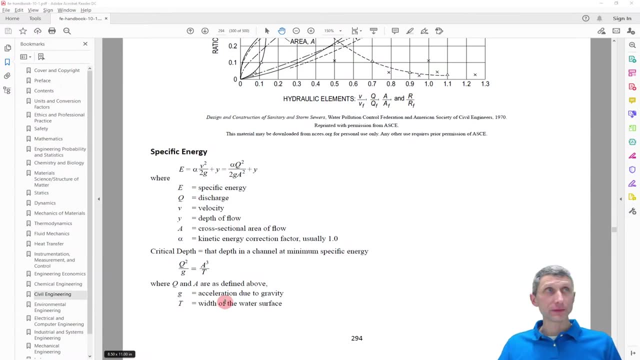 Where's T? Here's the hydraulic depth over T And we actually, I think, if we come back one page where the T is the width of the water surface, So T is going to be the width of the water surface And we're told that that width is is eight feet here. 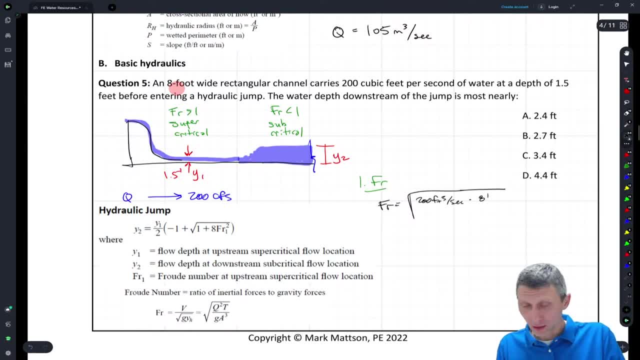 So we're going to use times eight feet Divided by what do we have? We have G, So G for English units is thirty two point two feet per second squared. OK, so if you don't know that number, you probably need to memorize it. 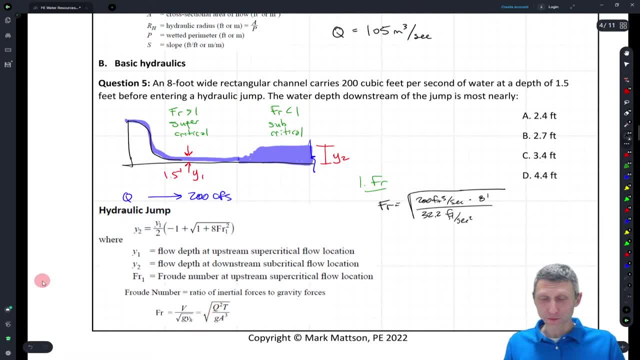 It's like nine point eight, one meters per second, squared for four, for metric. OK, And then. But then what's next? We have times the area cubed, So upstream the area is going to be eight times eight times one point five feet. 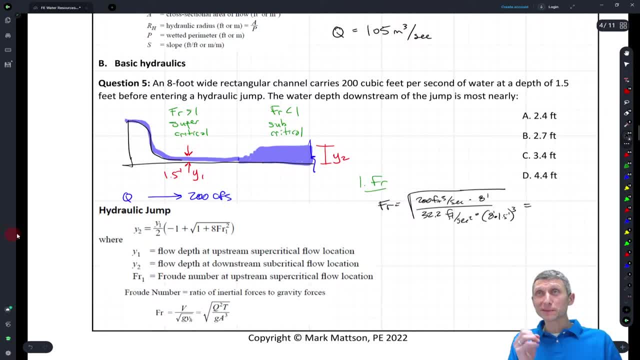 And we have to keep that. So we do all this. what we're expecting is that Froude number is going to be bigger than one, meaning it's super critical, And hopefully the problem was was written correctly. You know, sometimes when you're writing your own problems, you don't necessarily make everything right. 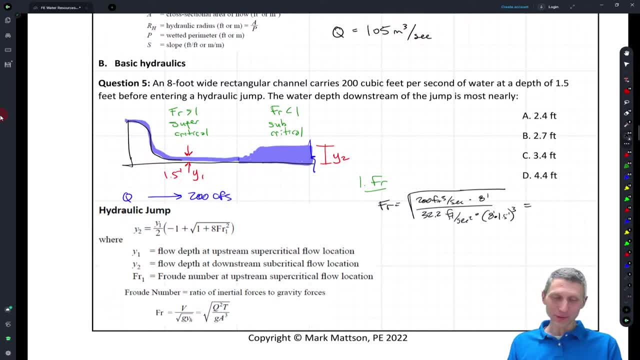 But I think I got this one right. So two hundred times eight divided by thirty, Two point two divided by what do we have? Eight times one point five in parentheses to the three, And I think I screwed something up. so what did I screw up? 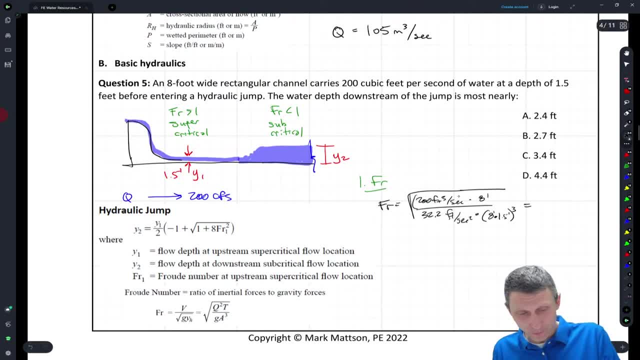 Oh, I forgot to square my flow. There it is. so it's good to put things in your calculator and not just trust your notes. but yeah, so if we put that square in and let me go back, Um, how did I know something was wrong? 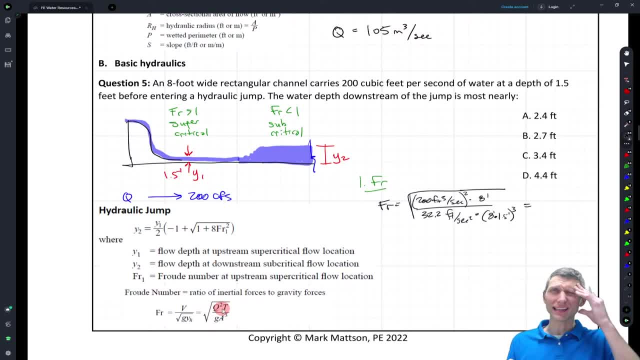 Because when I calculated it I got like a fruit of point one six. I'm like, wait a minute, point one six is less than one. I don't like that. What did I screw up? And that helped me to understand where my mistake was in this right. 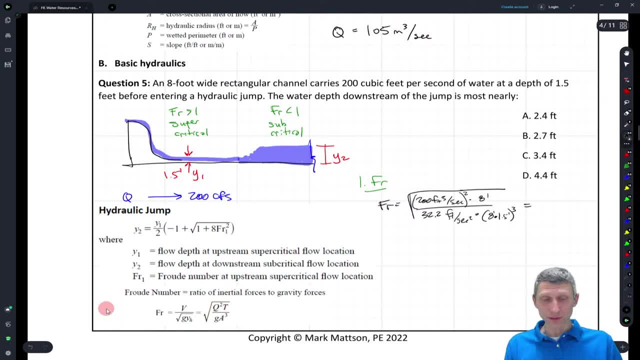 So I knew I did something wrong and I forgot that square. So so you know you have to look at the formula, but you have to write the formula correctly. And I got a value of about two point four, which is greater than one, which means you know it's it's the fruit is greater than one. 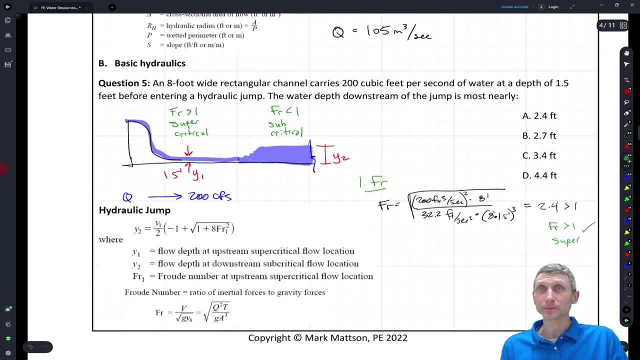 And that's super critical. So that Checks right. Once we have that, all that we need to do now is is is find our wide to depth And that's just again that becomes kind of plug and chug here, because we have the equation. 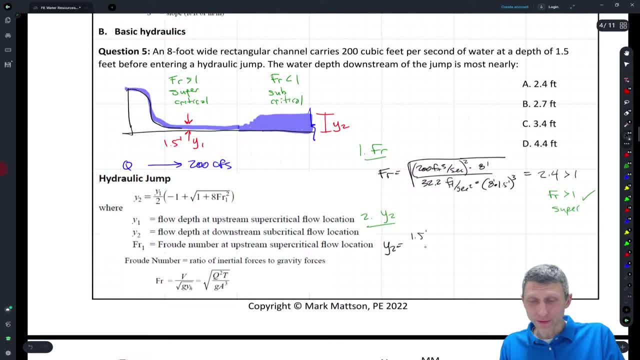 Why two equals one to one was the one point five feet divided by two times minus one, plus the square root of one plus eight times the fruit number. So two point four squared, And if I wrote down all my squares correctly, I think why two is going to equal. 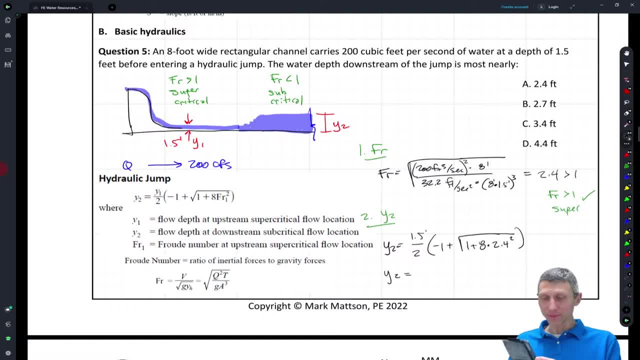 Well, let me just double check. So one point five divided by two times minus one, plus the square root of one plus eight times this. two point four, three, nine, eight, depending on how how much you want to get in there, That needs to be squared. 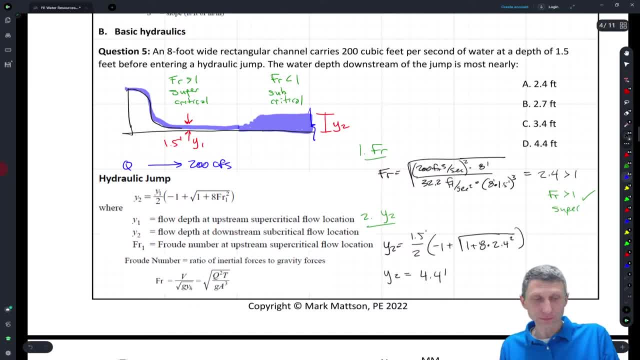 Yeah, so I get about four point four, So hopefully you're able to get that as well. But the reason I wanted to bring this question up is it is it kind of: are you going to get this exact question? I don't know. 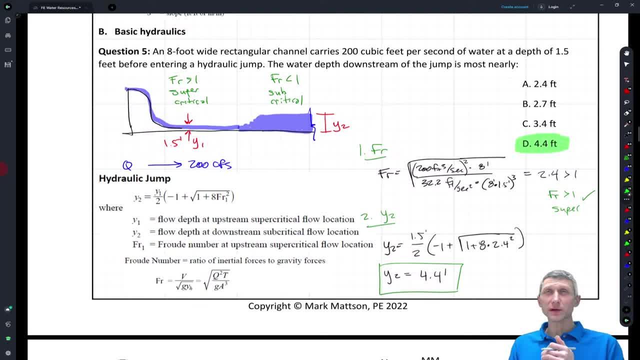 Maybe, maybe not, But the idea is super critical. Subcritical flow is one of those ones that I think could show up for sure. So just the idea of you know velocities and flows and that sort of thing, And I think it's, it's something that can show up because whether you see the free number here or maybe in a different place, I think, I think it could. 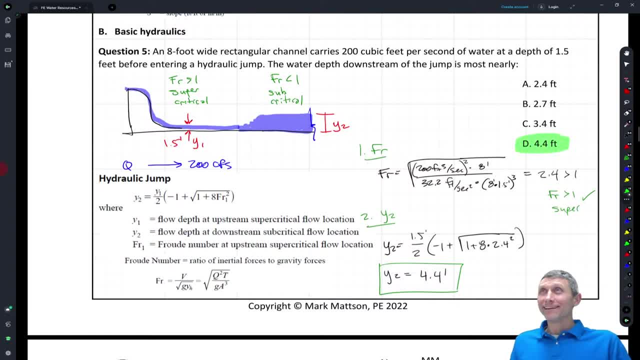 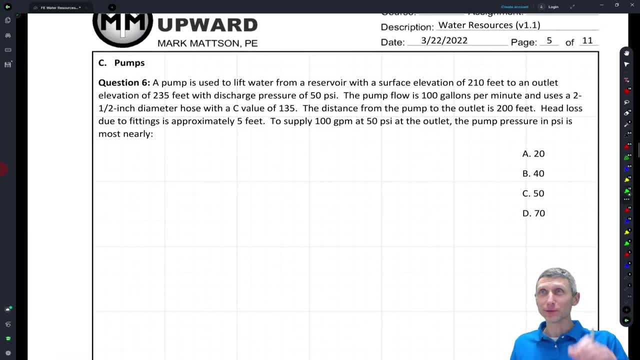 Could potentially show up. All right, you guys are quiet today. no, no major comments, but if you have any comments, let me know how we're doing and you know we'll keep going. So if I make mistakes, let me know, or just put your answers in the chat box and we'll see if, if you guys get the same thing as me. 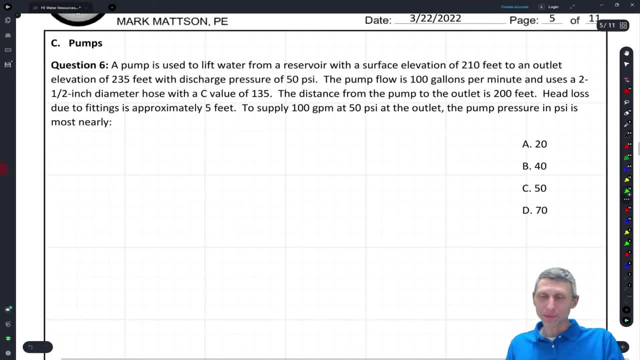 All right. So here we go. So we have a pump right And this is a pump equation. So so last time when we did fluid mechanics, we were looking at, We were looking at, We were looking at the Bernoulli, and now we're going to take a look at the energy equation. 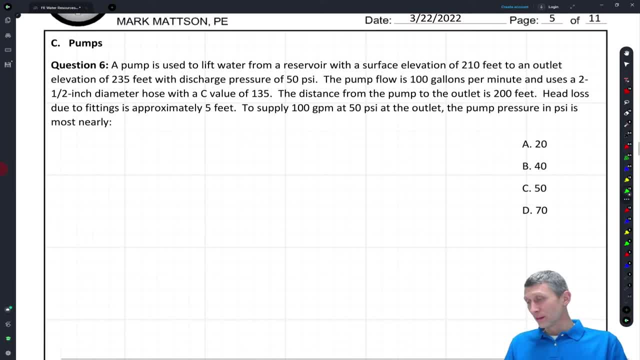 So the energy equation has to do with With energy, energy losses. but let's take a look at this question. see what it says. We have a pump is used to lift water from a reservoir with surface elevation of 210 feet. So let's draw our reservoir down here. 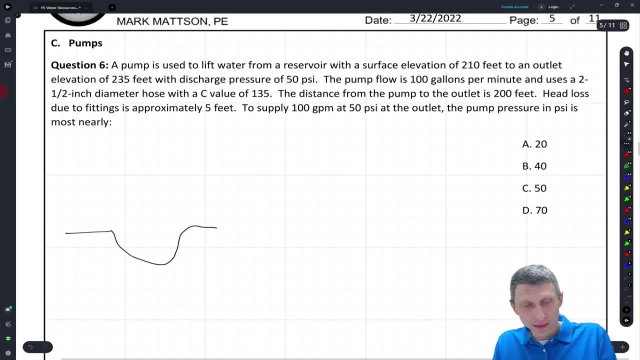 So we've got a reservoir. you know we got a reservoir here and maybe we have some, you know, water level. OK, so this is open atmosphere and this is our reservoir Full of water. OK, and what we're going to do is- I mean, this is one of those things where maybe you're doing an agricultural thing. 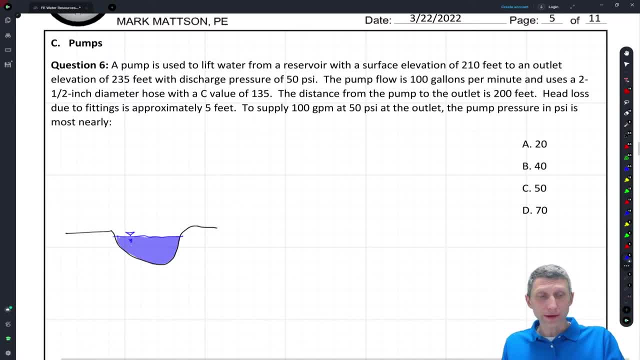 You need to lift water to something- Maybe it's a fire application- but you're going to put some pump. you know some pump, you know. sit in here and you're going to put a hose in, a hose out and you're going to go up to discharge point up here, which is at an elevation. 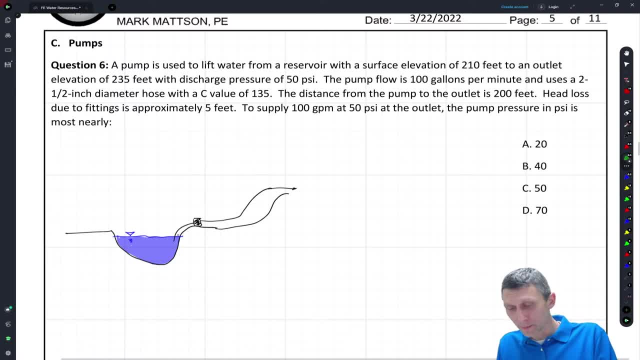 Let's take a look at what our elevations are. So we start at an elevation OK Of- Actually, I think the way that I said is the pump elevations 210.. So we're going to, we're going to, maybe, let's, let's, maybe, move this pump down just a hair. 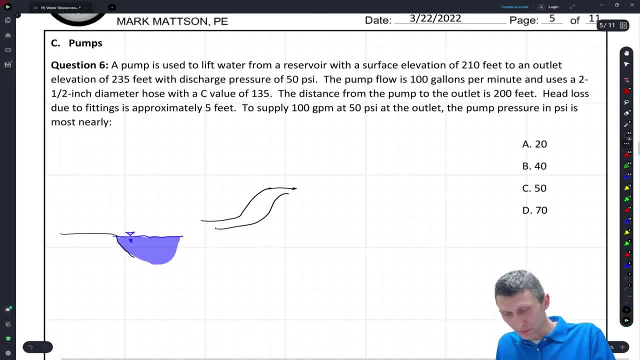 Oops, let's, let's move the pump down, and just a hair here. So we'll move the pump down so that it's at the same elevation as the water surface, And we're not going to introduce like anything too crazy here. OK, so we're going to basically stay there and then we're going to come up to a discharge point. 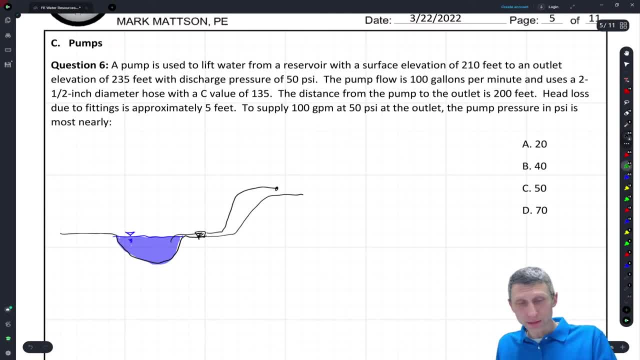 Somewhere, you know up at this point. OK, what elevations do we have? Well, we start a reservoir surface elevation at 210 feet. So we've got, you know, 210 feet here and we have a discharge of 235 feet. 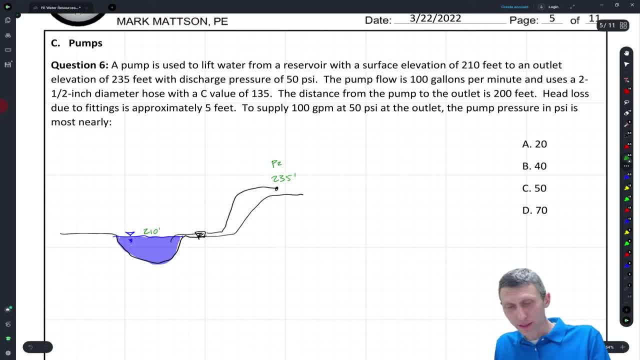 OK, we want a pressure at this point, a pressure at point two of 50 psi. So whatever application they're doing, we need to pressure 50 psi. The pump flow Right. So you got some flow in this thing. That's 100 gallons per minute. 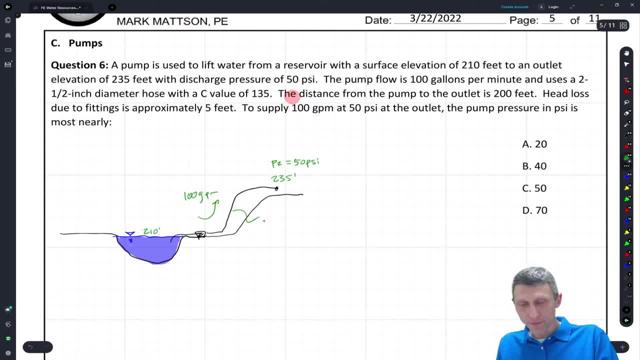 OK, and what we're going to do here is it's we have a two and a half inch diameter hose With a C value of 135, and when you see that C value, that's going to- that's hopefully going to tell you that we need to look at friction in this pipe or this hose. 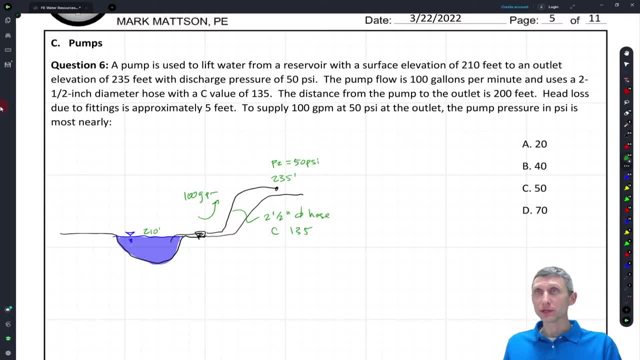 We need to look at friction and hopefully you know that we're going to look at using the Hayes and Williams friction friction factor. Now there's a couple of different ways of looking at friction. There's there's a ton of different ways. people have been trying to come up with good, good equations for friction for a long time. 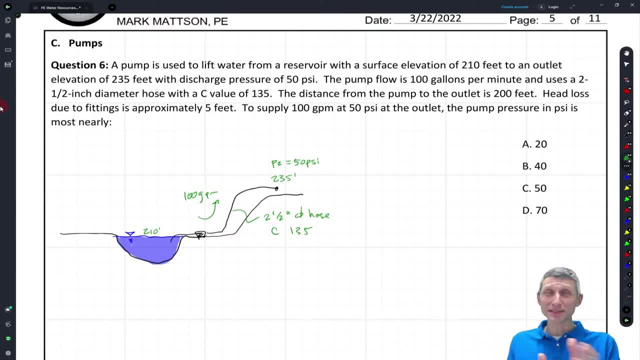 But? but when you see that C value, we're going to use Hayes and Williams and a lot of times in the civil industry the Hayes and Williams equation is a good approximation for typical water applications. You know, 40 to 75,, 80 degrees Fahrenheit. 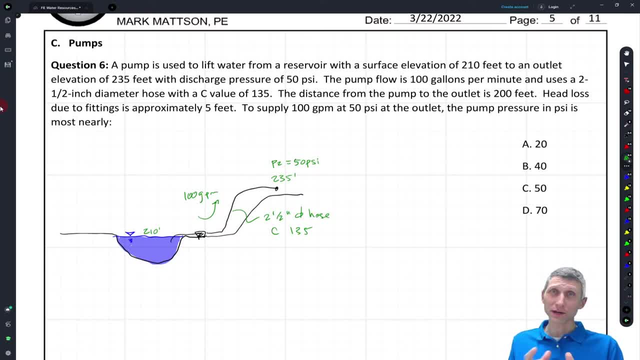 Hayes and Williams is used in the civil industry quite extensively for that. Darcy Weisbach gets gets used as well, But that's typically for non water fluids. It typically gets used for different temperatures. It's a little bit more robust, but Hayes and Williams is a good approximation that gets used a lot in the civil industry in the water industry. 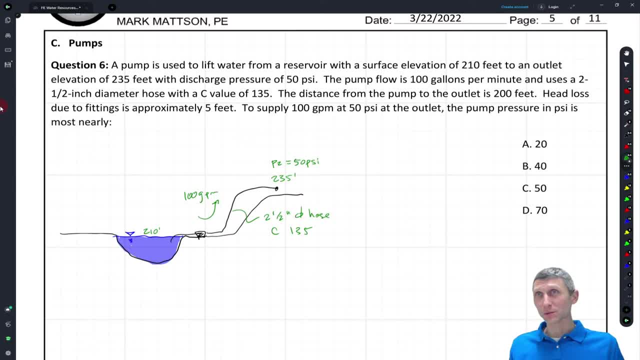 So that's so I chose that one. I mean, we could do another problem with Darcy Weisbach, but I didn't for this session. Maybe another session in the future I will. So this is where this is where starting, and basically what we want to do is we want to find, you know, to support. 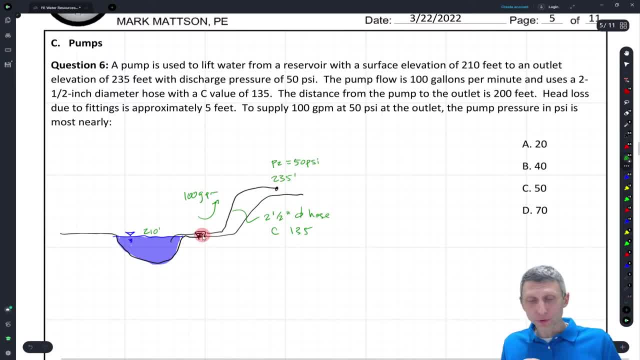 We're going to apply 100 GPM at 50 PSI up at this point. What pressure do we need at this pump? So what pressure are we outletting at this pump in order to get to 50 PSI up here? So we have some elevation head we have to deal with. 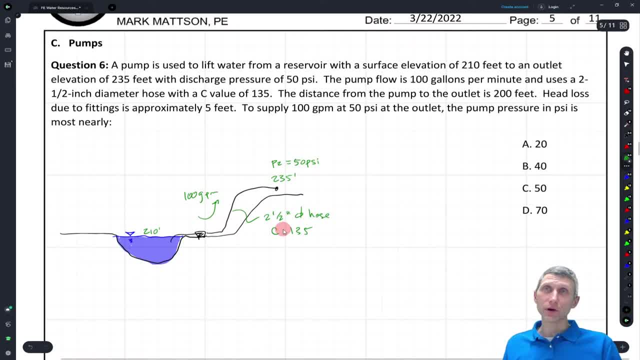 We're going to have some friction losses here, like two and a half inch diameter hose. That's typically one hose that could be used in like firefighting applications, for example, or agricultural applications for sure. So we're going to use you know, this is that. 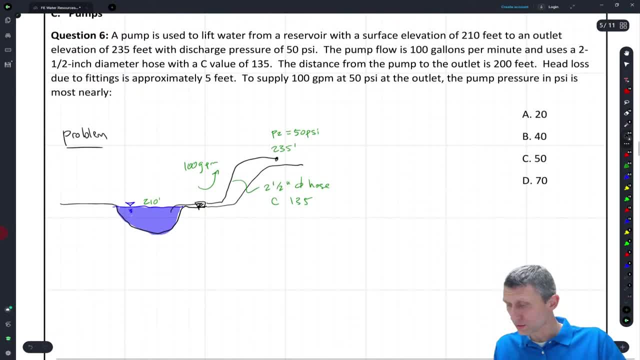 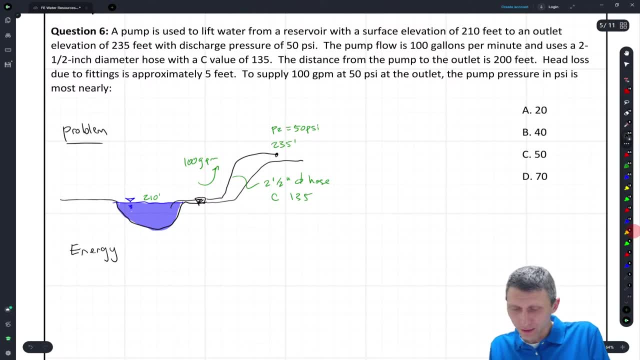 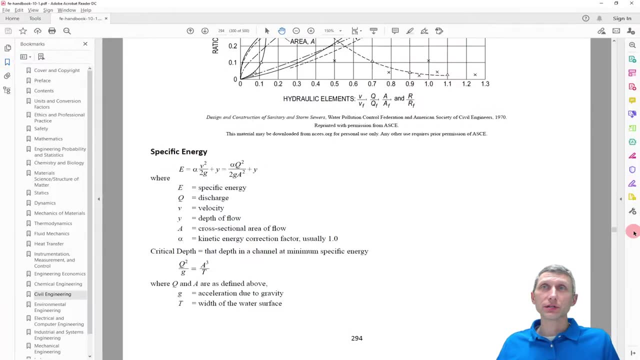 This is our problem. What we're going to do is we're going to use the energy equation here to solve it. So the energy equation- I'll write it here. Energy equation is in is in the manual, But interestingly enough, when we come back to the energy equation, I'm just going to do a search here. 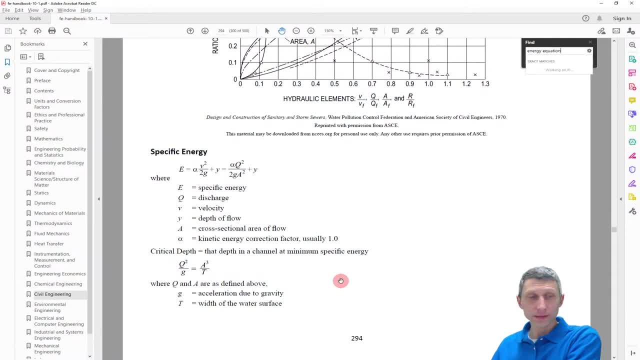 Energy equation. I spelled it right, And is it going to find me any? any matches? Maybe Let's look It's. it's, I thought it was in there, Maybe it's not. Maybe it's. maybe it's just being slow. 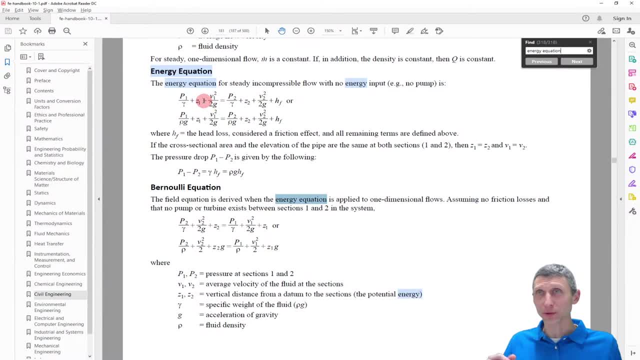 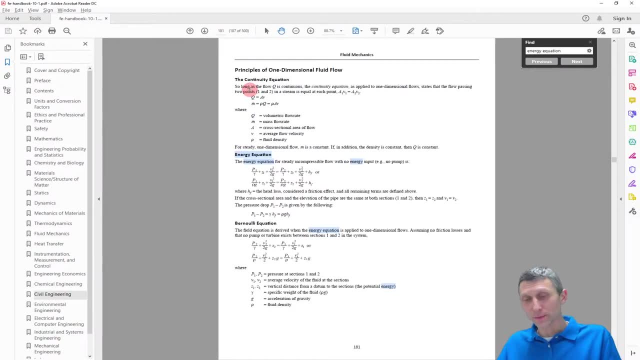 There it goes. And well, actually it's not there. It's not. Oh, there, it is Energy equation. It's interesting to note that this goes back into, essentially, the fluid mechanics section. So this goes into the fluid mechanics section. 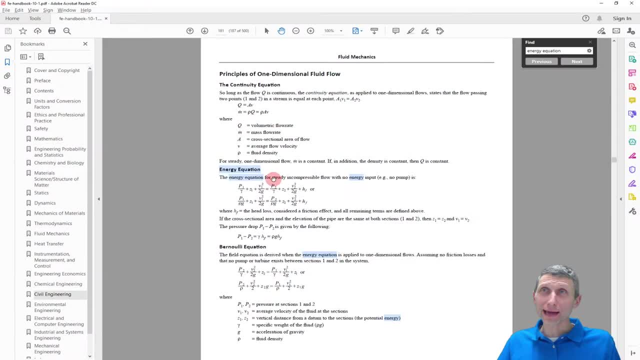 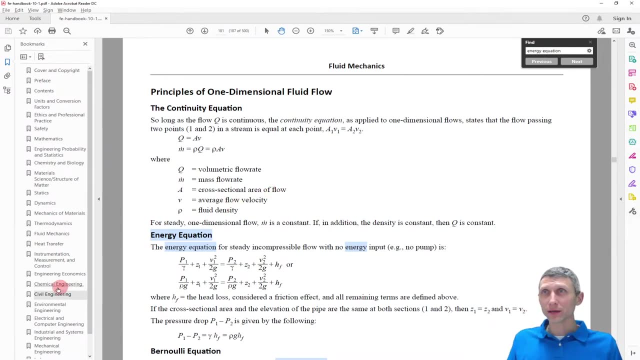 You can see up here, it's fluid mechanics, So it jumps back from, you know, from water resources, And this is where you again, If you're looking at that reference handbook, you got to understand some. some sections are civil engineering, Some sections are going to be fluid mechanics and you kind of have to know where some of these pieces are. 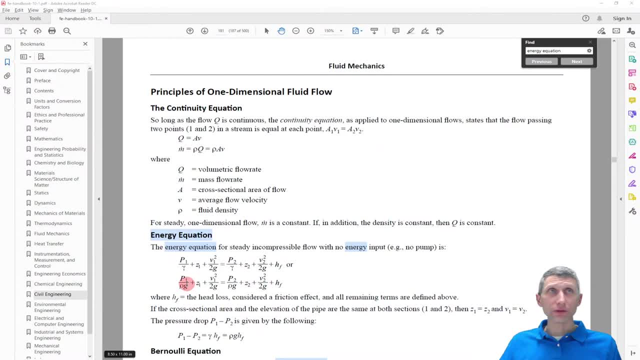 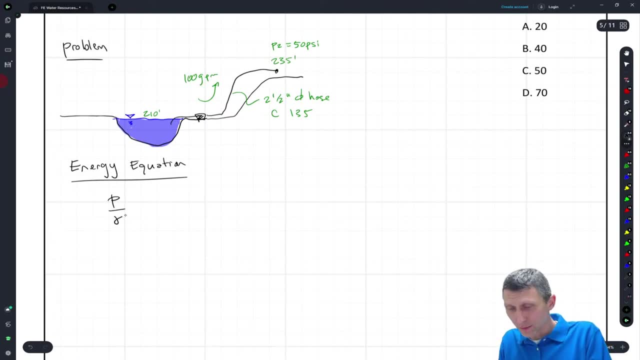 So we're going to take the energy equation and we're going to use it. So let me come back here. What's the energy equation say? The energy equation says essentially that we're going to have P1 over gamma plus Z1 plus V1, squared over 2G plus the pump. 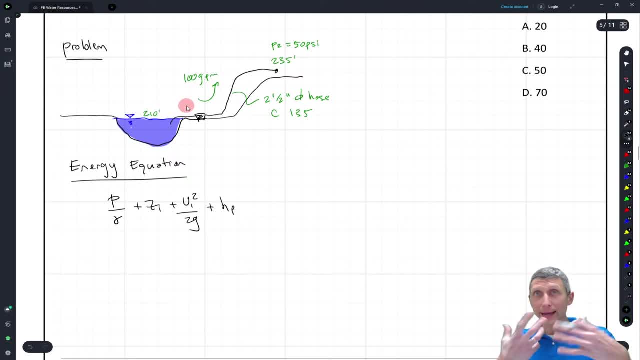 The pump pressure. OK, so that's the pump pressure. So we're adding energy into this. We're going to say that is going to equal to P2 over gamma Plus Z2 plus V2, squared over 2G Plus the friction losses. 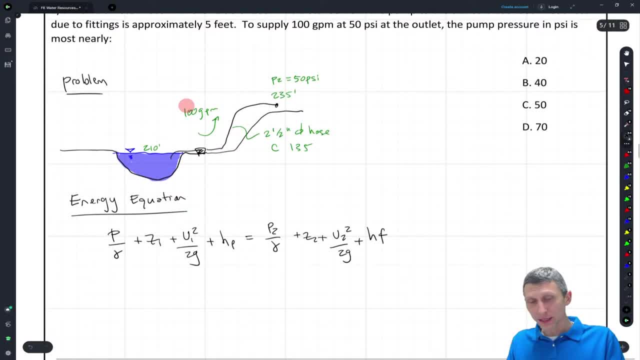 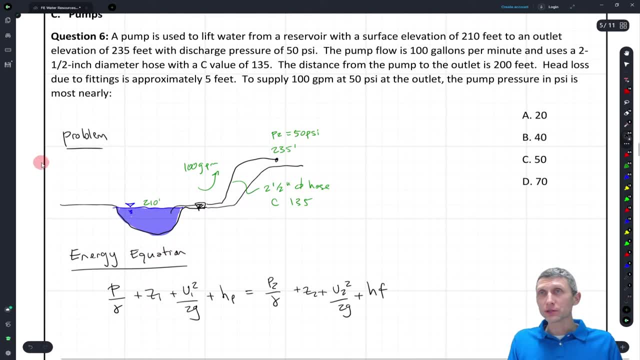 OK. so this is where we kind of have to understand the problem and understand what we're getting into to solve it. But once we know that we're going to use the energy equation now, we can keep going To solve for what this pressure is at the pump. 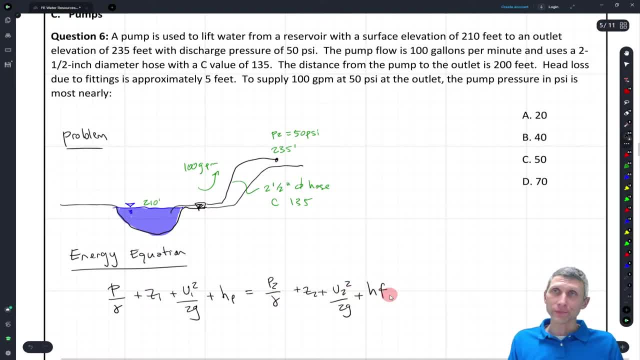 But we also, in order to do this, have to figure out what the friction losses are in the pipe. So let's take a look at each of those in turn. The other thing that we're going to do here is we're going to take a look at: 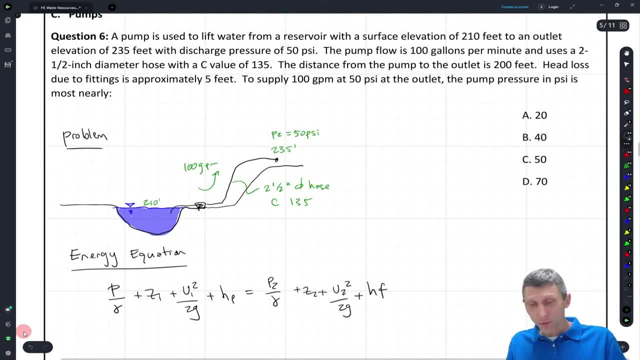 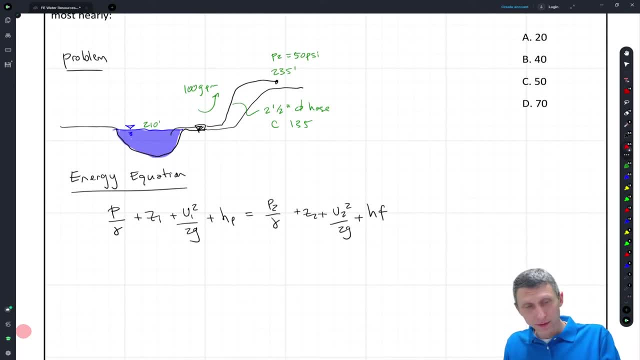 At elevations. Well, actually, let's just let's jump in. What we know is we essentially have: Let's see, Let's see what we can cross out first. So we're going to. I think I forgot, Got a one here. 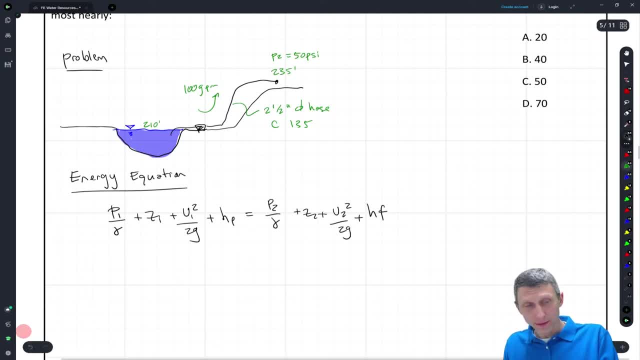 So P1. So if we have point one, kind of like down at this level, Right, So this is point one and this is point two. OK, we're going to go from point one to point two and basically a P1.. We have. we have essentially zero pressure. 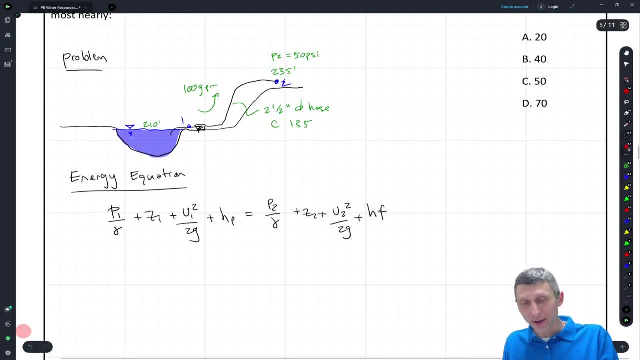 Right, So we have zero pressure. We're at atmospheric pressure. I'm going to cross out P1.. I'm going to call this one zero, OK, P2.. We know we want to be at 50 psi. OK, so we want to be at 50 psi. 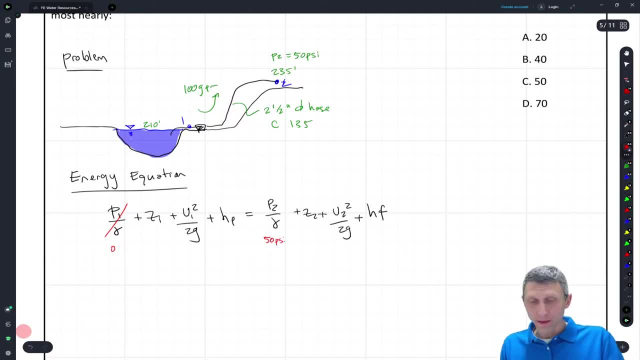 So we're going to have, you know, our 50 psi at P2.. Z1. What do we know? We know Z1 is going to be 210.. Z2 is going to be 235.. And then, what do we do for velocities? 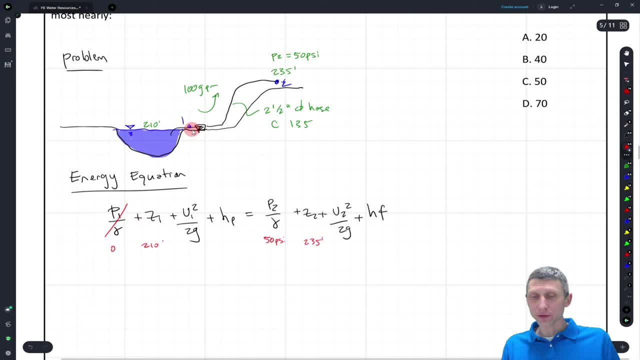 Well, what we're seeing here is we have essentially continuity equation that says: you know, we have a Q is AV, QAV. All of this is two and a half inch diameter hose, So the A doesn't change, The B doesn't change. 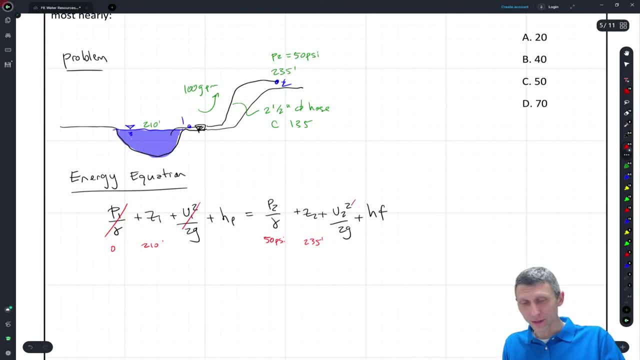 The Q doesn't change Essentially by continuity. we're going to say V1 equals V2 and just cross those out because we're not worried about the velocity head at this point for this system. OK, so what we're left with is: is we really need this? 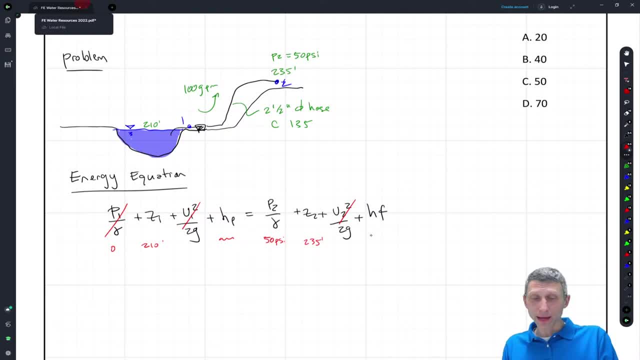 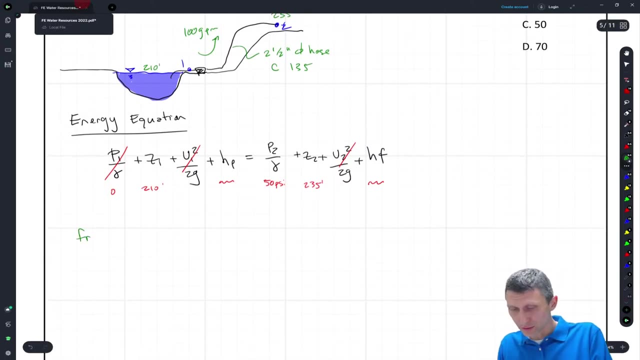 We're trying to solve for this pump pressure, But in order to do that, we're going to have to solve first for the friction losses. So what are the friction losses going to be? Well, the friction losses. Let's just take a look down here and we'll say: the friction losses, friction. 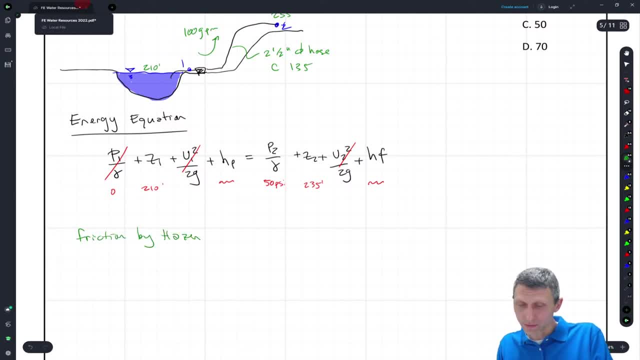 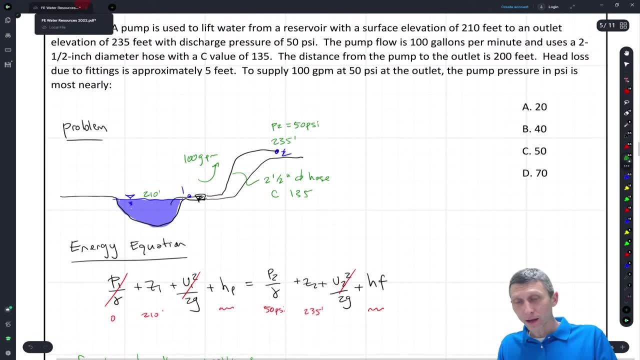 You know, by Let's go to the Hayes and Williams equation, Right, so friction by Hayes and Williams. and why do I know it's Hayes and Williams? Because I'm I'm given the C value and you might need to go look up that C value. 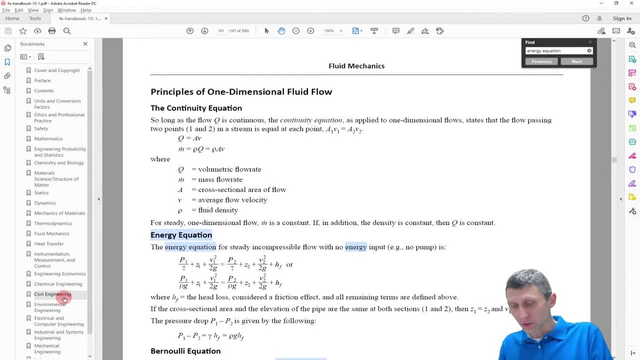 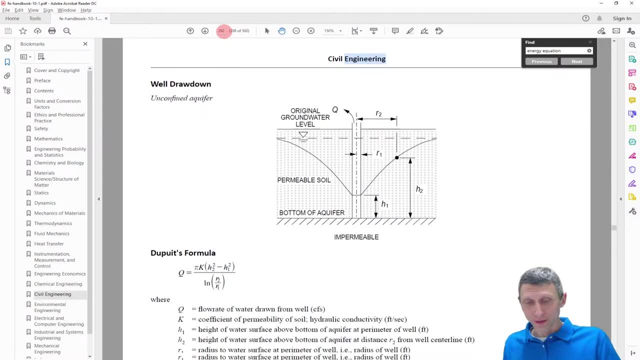 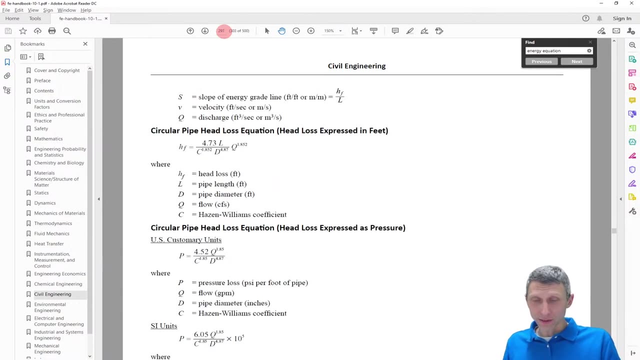 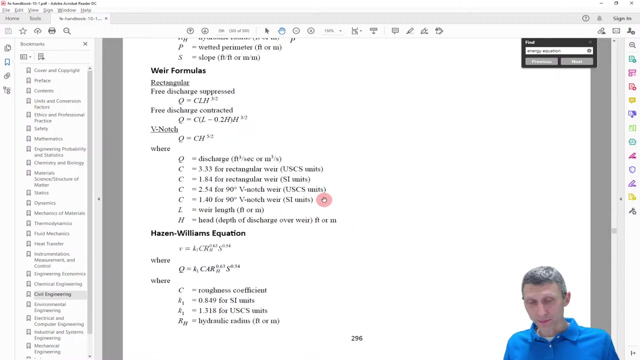 Let's come back to the reference handbook and come back to our civil engineering section, which I think is maybe around like two, ninety two or so somewhere in there, And if we keep coming down we will see Our our friction had lots of circular. circular pipe head loss expressed in feet and a circular pipe head loss expressed as pressure. 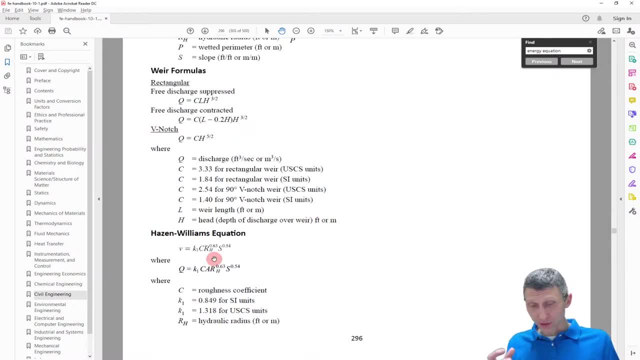 But here's the Hayes and Williams equation. OK, so this is a general Hayes and Williams equation. We got some different things going on, But the nice thing is you don't have to use a general equation because the handbook gives you, gives you, this equation down here. 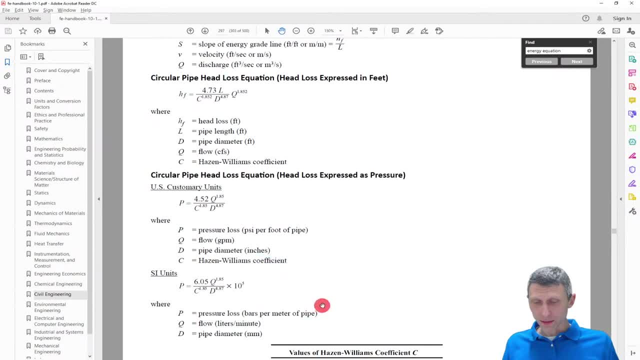 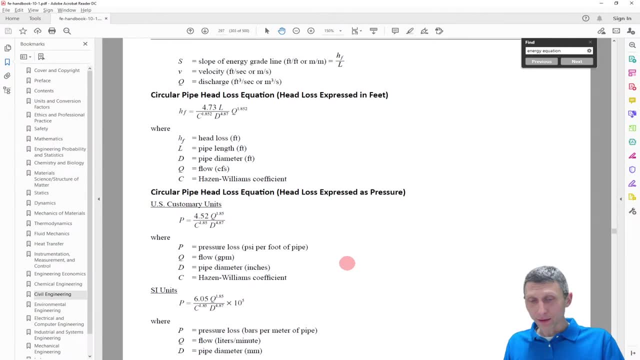 Did I go on page too many? I think I did. So let's take a look at this and see What we have. So we're looking at circular pipe head loss expressed. Well, we can either do feet or pressure, But what I'm going to do here is we're taking our elevations in feet. 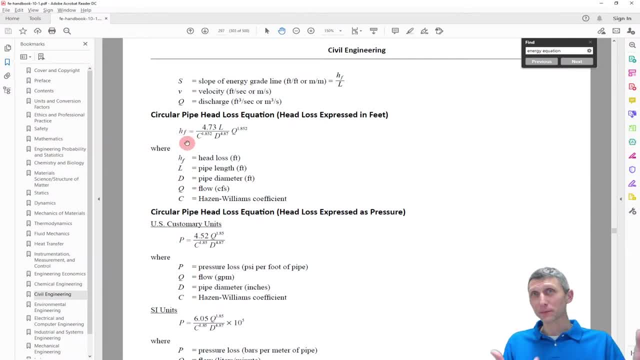 So I'm going to convert everything to feet first. You could convert everything to pressures first, but I'm going to start with with feet. So I'm going to take this equation and and use it. So, actually, why don't we snip it? 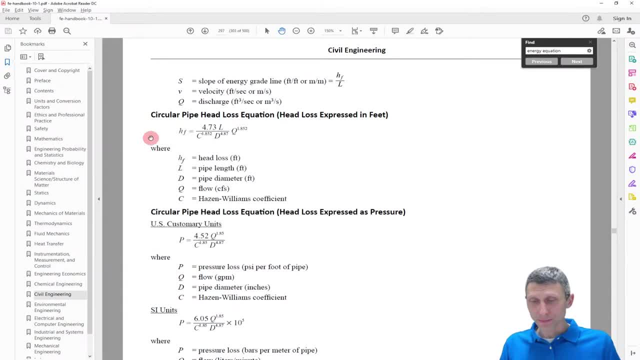 Why not? It's the worst that happens here, So let's snip this in and take a look at it as well. So I'm going to take this, This equation, Bring it over so we can use it for our- our head loss. 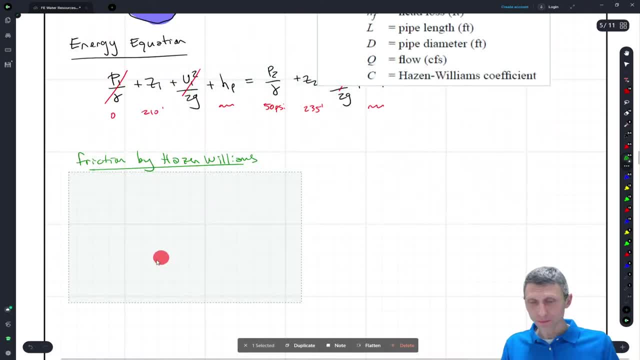 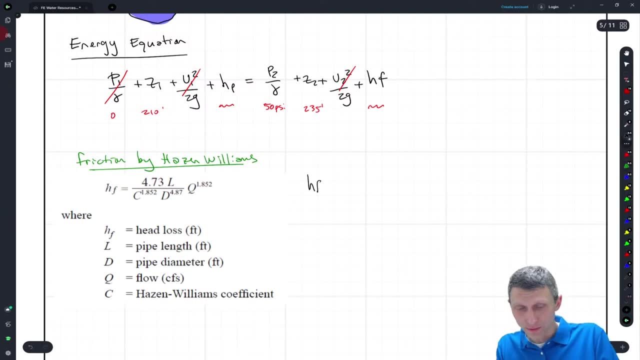 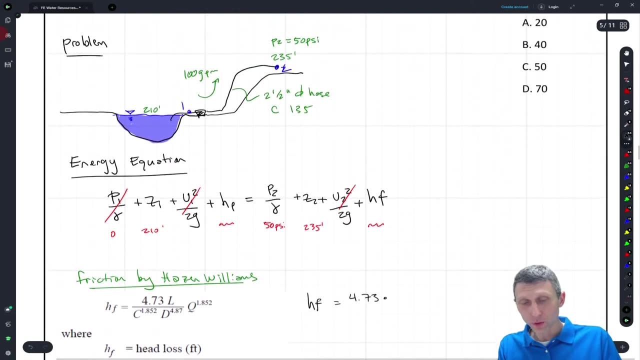 OK, So What do we get? We're going to, we're going to find this, this head here, and we're going to say that the friction Right, It is going to equal four point seven, three times L. We're told, I think, in the problem statement that we have. 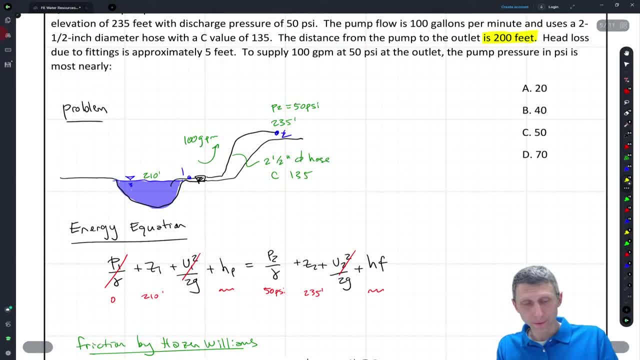 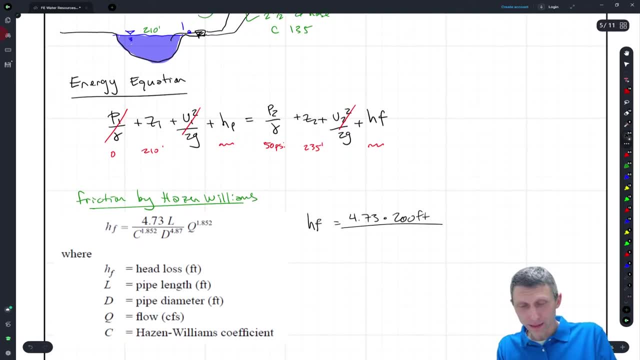 Distance of this 200 feet, hose Of 200 feet: OK, So that's good. So times L times 200 feet: OK, Divided by C, Our C was 135 to the one point. eight, five, two. Again a weird exponent. 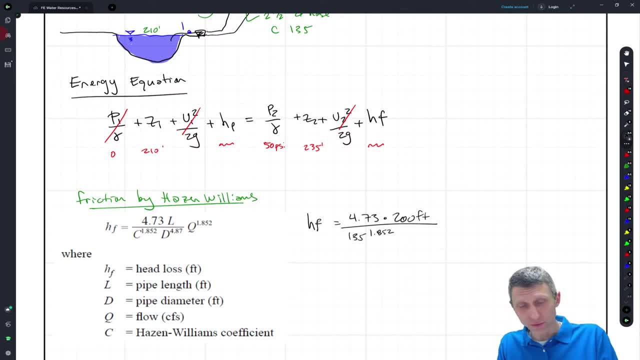 But it's. you just have to know how to type one point eight five, two in your calculator. Times the diameter, So the pipe diameter. Be careful here. The pipe diameter is in feet, So we're going to do two point five inches per twelve. 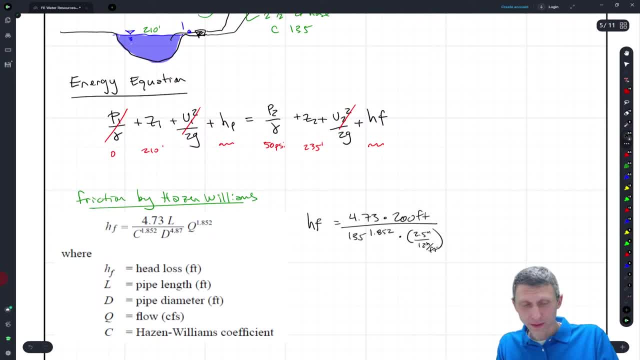 Inches per foot And raise that to the four point eight, seven power. OK, Then we have to multiply all of that times Q, which is going to be a hundred gallons per minute Times, or, I'm sorry, to the one point eight, five, two power. 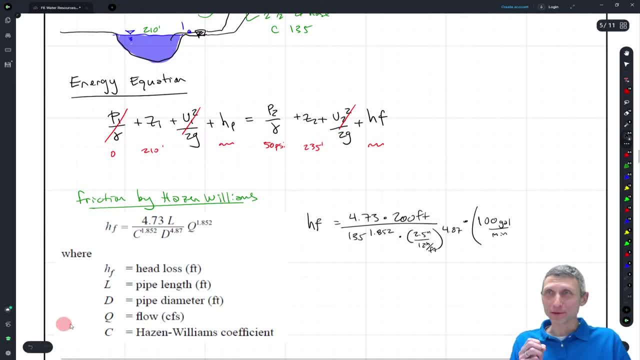 But I left a little bit of room here because we have. we have to be careful because our flows in CFS are forgiven gallons per minute. We have to multiply, We have to multiply. Oh boy, Well, we know that we have sixty sec. 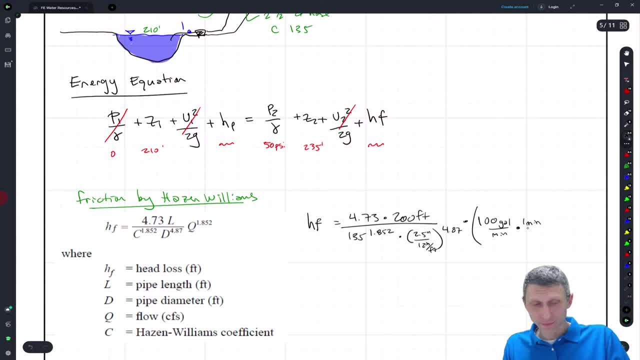 I'm sorry, Wrong way. So we have one minute Per sixty seconds And we know we have a certain number of cubic feet or a certain number of gallons per cubic foot, Right, So if we have one gallon, or how many gallons per cubic foot, 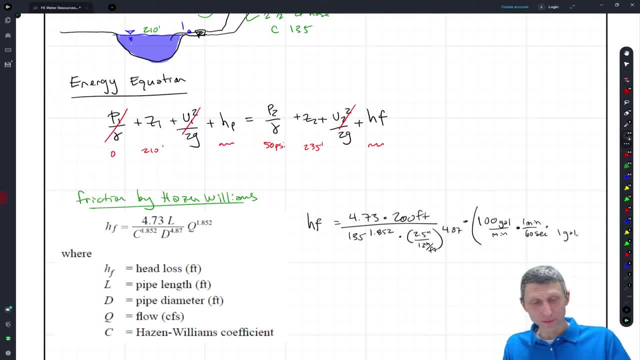 OK, So if you don't know this off the top your head, um, you might not know it off the top of your head. right, How many gallons are in a cubic foot? Cause this is where, uh, we need to do a unit conversion and and then raise all that to the. 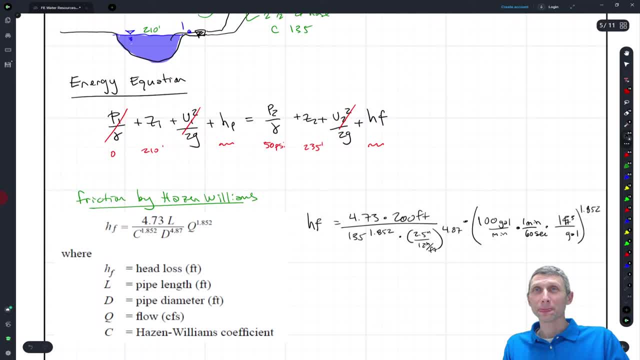 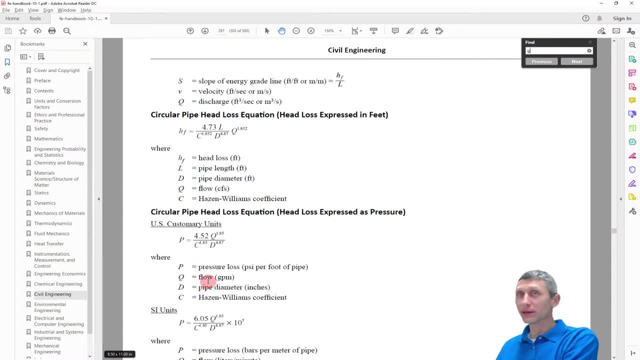 1.8 to five to power. Hmm, So, um, back to the reference handbook we go. Okay, So this is where, knowing, you know, gallon, uh, is is gallons in there. I think it is right: Million gallons per. 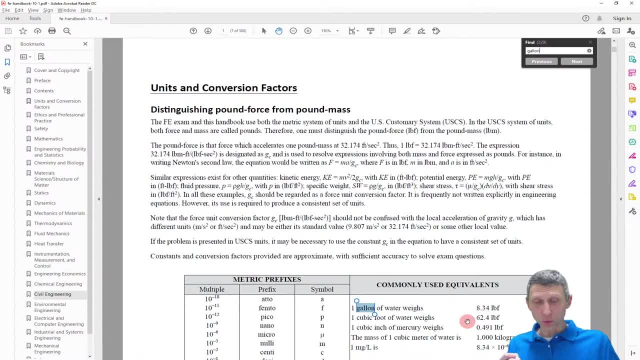 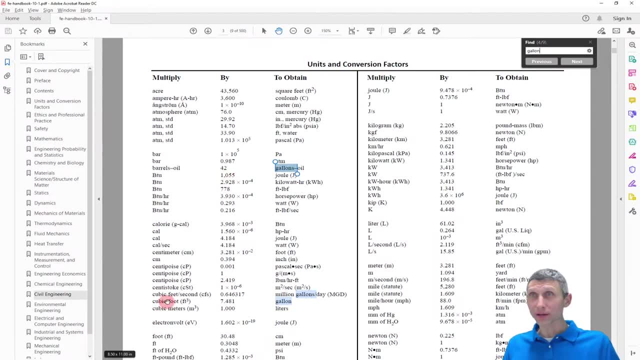 day that gets us into fate and transport. but here, one gallon weighs 8.34 pounds, So we're in the right spot. maybe, Um, and what we see is 42, you know, but we're down here, Look, look, we got. 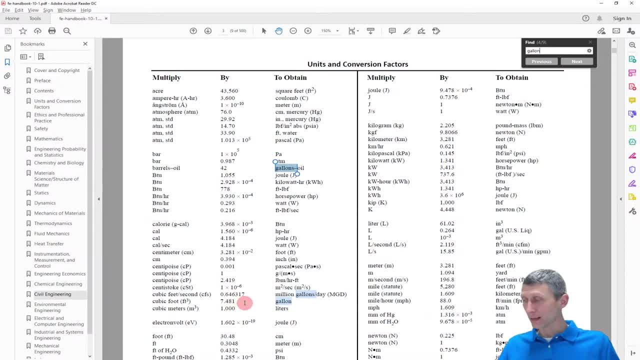 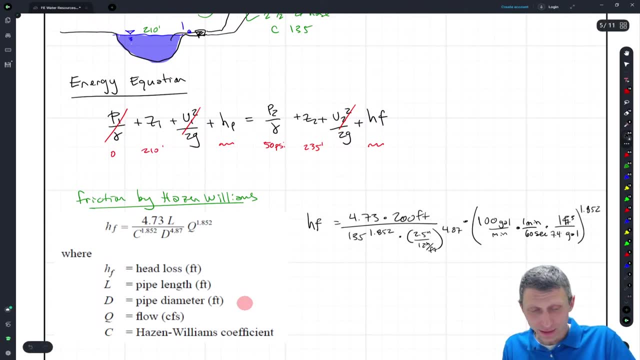 cubic foot: 7.481 gallons. Okay, One cubic foot is 7.481 gallons. So the good news is we can find that. a search and find um didn't take us very long to find it, But what we see is we can cross. 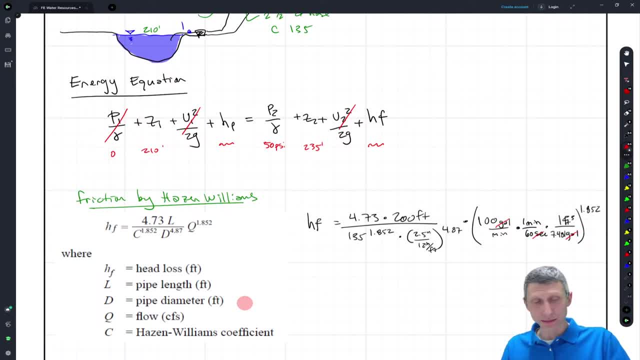 out our gallons? Um, we can cross actually. no, we, we want to keep our seconds. We cross out our minutes and we're left with cubic feet per second. plug all this in And? um, hopefully we get the right answer with all those funny exponents. Um, the number that I got in. 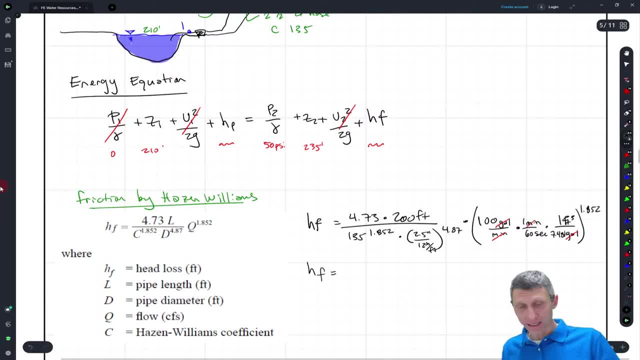 here was about 13.8 feet, So 13.8 feet, So hopefully, um, that that was done right, but let's select those. So 4.73, uh times 200, divided by 135 to the 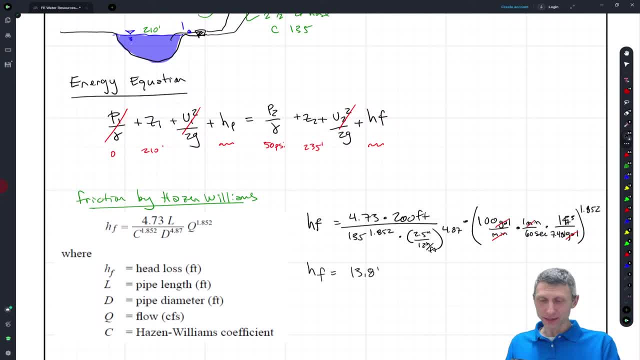 1.852.. And hopefully you're trying this as well, Cause the the you know, using your calculator can be weird on this, Um, especially when you have you're dividing in parentheses and all that sort of thing, But um, but hopefully you can get this right as well, Okay, And then 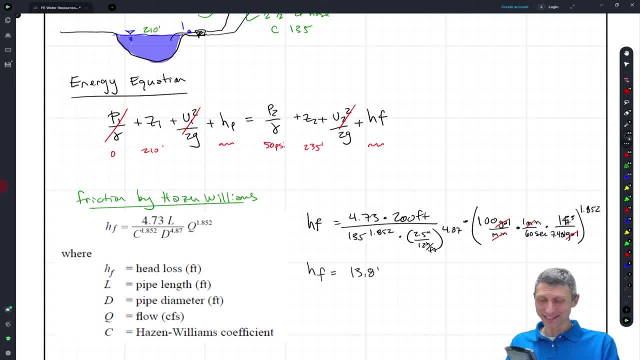 let's see, divided by 60, divided by 7.481, and erase that all to the power of 1.852.. Did we do it? Yeah, I think at 13.8,, 13.82, maybe um 13.82 feet. Okay, So that's the friction loss just in the, the, the from the. 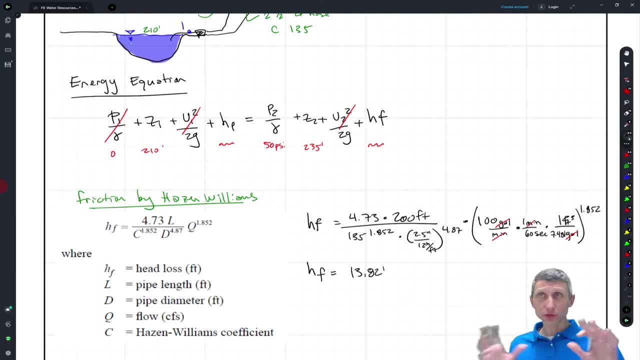 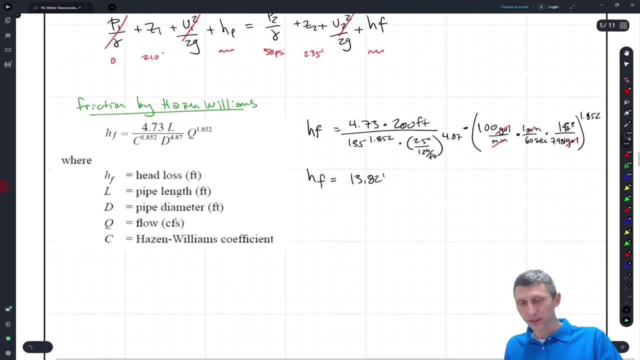 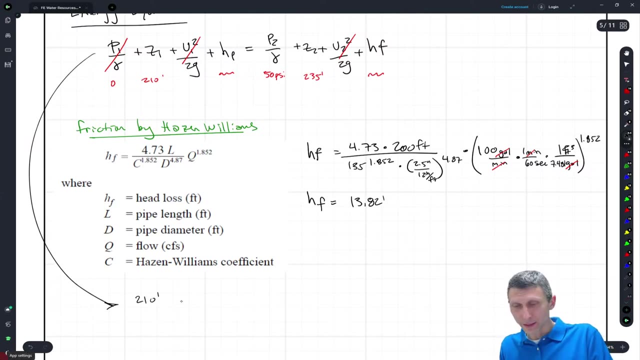 water flowing Okay So. so the good news is we have everything now kind of to plug into our energy equation, So we can do that and we can solve. So let's, let's bring this back down um solve it all out And hopefully, um, this makes a little bit of sense. So we have 210 feet. 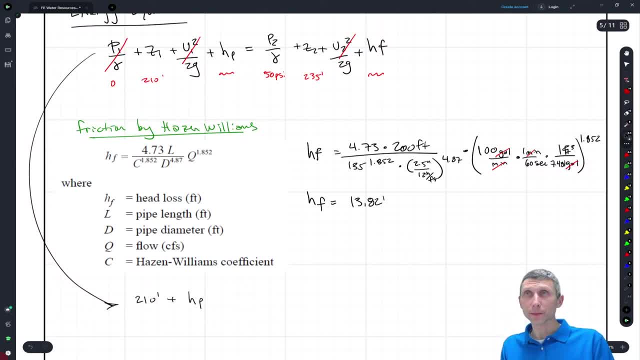 plus HP. That's what we're trying to solve for the head of the pump. um equals the pressure at two right, So we have um 50 pounds per square inch. That's what we know. We have pounds per square. 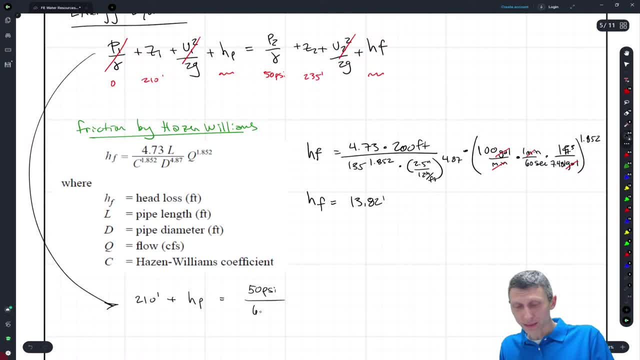 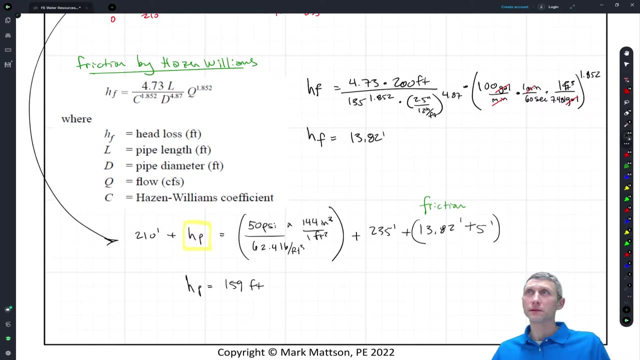 inch divided by gamma, which is the unit weight of water, or 62.4 pounds per cubic foot. But do you see a problem here? Units are huge. All right, Jeff, you back. I think I just got something that said: my, my, my stream got. 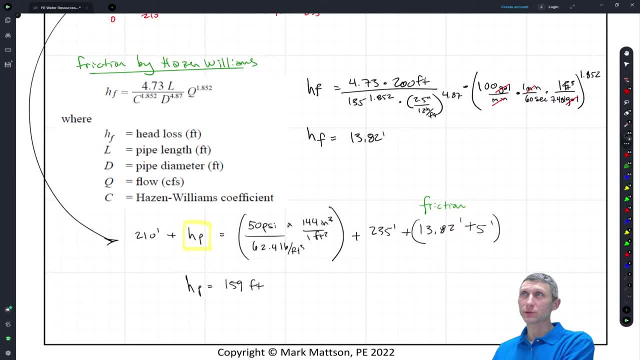 reconnected. So, um, I apologize for that. I'm not sure what happened. Uh, that hasn't happened in past sessions, so hopefully it doesn't happen again. Uh, and I apologize for that. Thanks for your patience. That hopefully this, uh this, keeps going And if we have more issues, I will um redo the session. 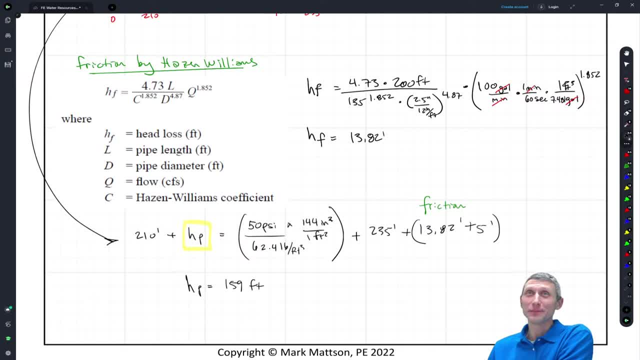 and repost it. So I don't know what to say with that, Uh, but if, uh, you're still there, maybe you can just keep putting something in the chat. So I apologize for any any weird latency that's going on, Um. 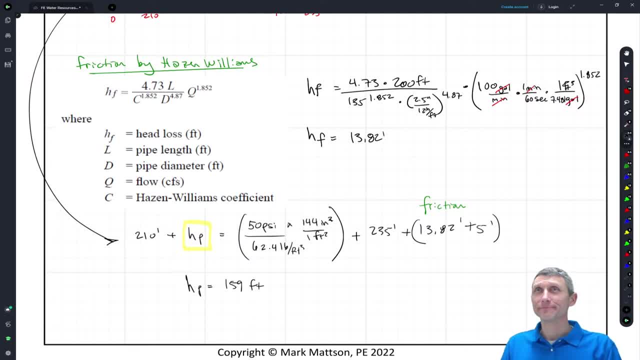 you. Okay, I think we're good again, Um, and so I'm going to keep going here and hopefully, uh, we didn't lose too much, So I apologize for any uh, weirdness that went on with the um stream. 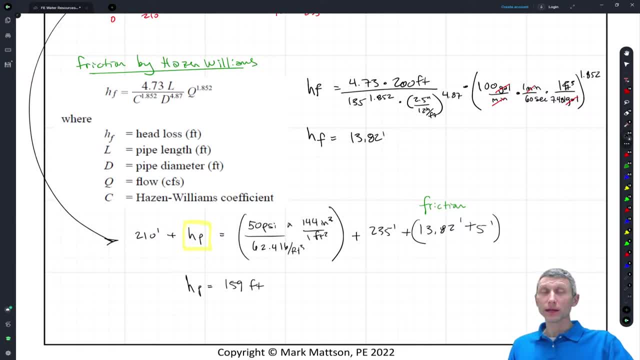 getting disconnected there. but we will, uh, keep going and hopefully not have any more issues. So, if we do, I will do a repost of this and hopefully, um, make it work. but, um, sorry for any technical issues, They're not exactly sure. So I'm going to keep going, Um, and so I'm going to. 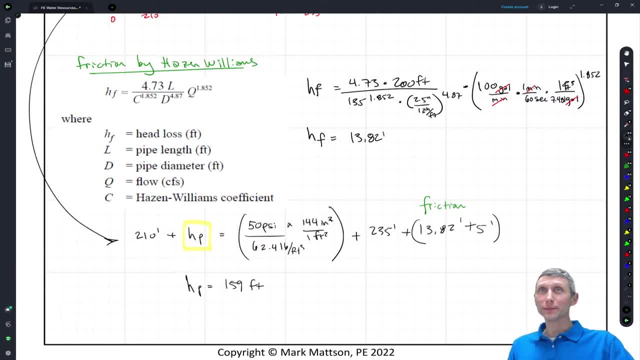 make sure, uh, what happened. So we'll keep going. Okay, Thanks for your patience and let's keep going. So, not sure exactly where we left off, but, um, the biggest thing that we're doing is we're just plugging and chugging into this, into this, uh, into the energy equation, right? So, as we 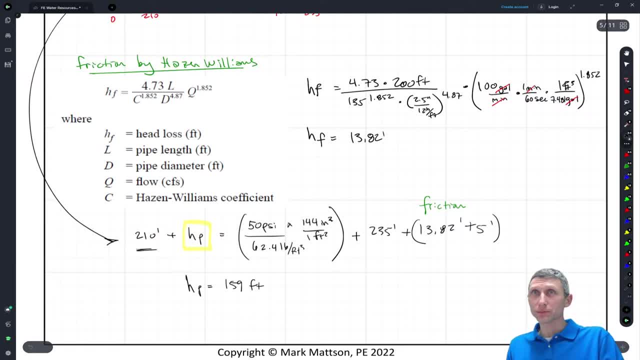 plug and chug. we have the elevation at the first point, Um, we have a pump pressure at the second point, or the pump, the pump pressure that we have to provide, right. We have the outlet pressure that we want. This is at the outlet, now, right? Um, and then we're. this is our outlet outlet head, the, the. 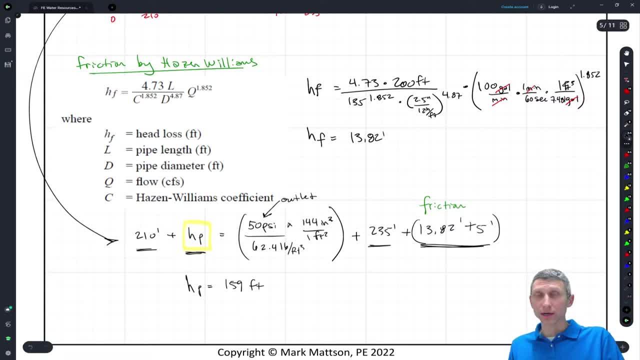 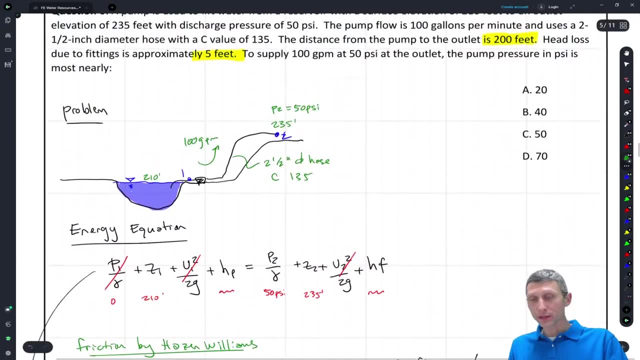 um the elevation, And then we have our total friction here, which is a sum of the friction loss in the pipe right. So the friction loss in the pipe uh, plus the friction loss in the fittings, And if not sure where we got cut out, but um, the friction loss in the fittings is. 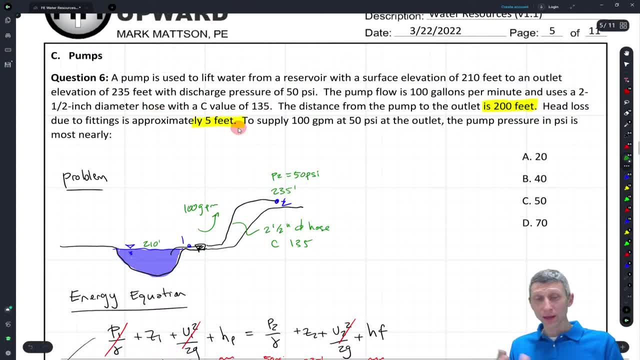 given in the problem statement as as five feet. So, um, that's going to be, um something that we have to also add in there, right Cause sometimes those nozzles of contractions and maybe you know, whatever there is there, there's going to be. 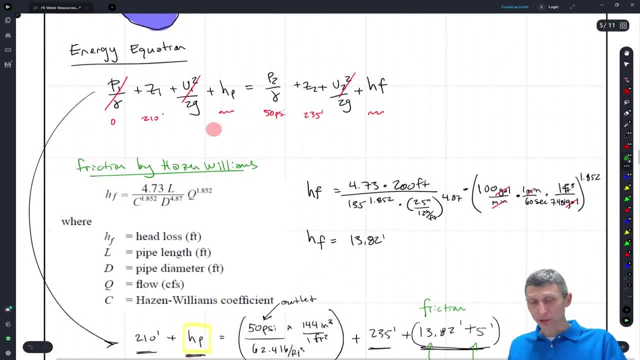 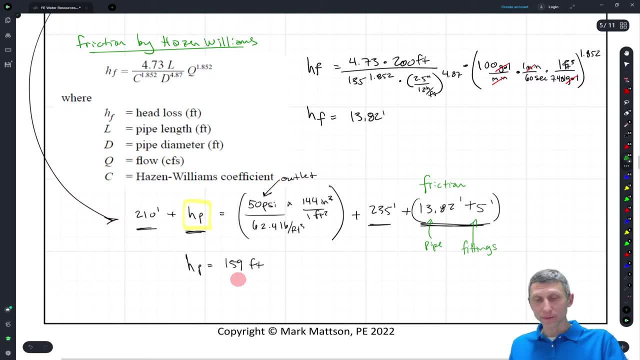 some, um, you know, 90 degree fittings. you're going to lose some pressure that way. So when we plug all this in, we get a total head of 159 feet. but um, the the problem actually asks for a PSI. 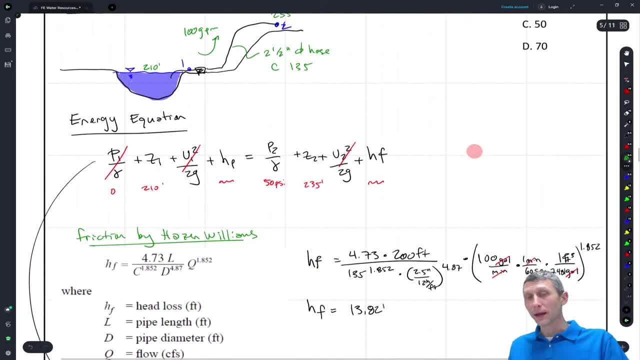 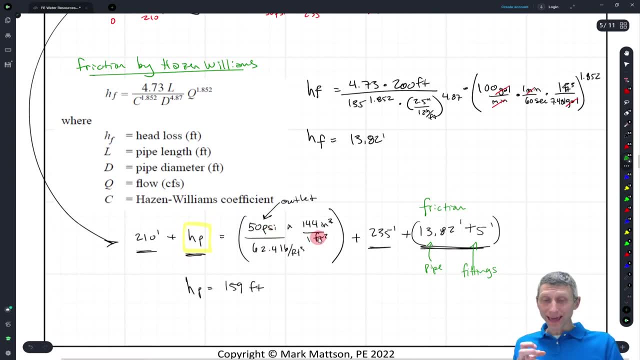 the pump pressure and PSI. And that's where we need to know how to convert back to PSI. And we did that once already, right? So to convert from PSI to um to head, we had to multiply by 144 and divide by 62.4.. So to go the other way, um, we're just going to reverse that process. So, um, what? 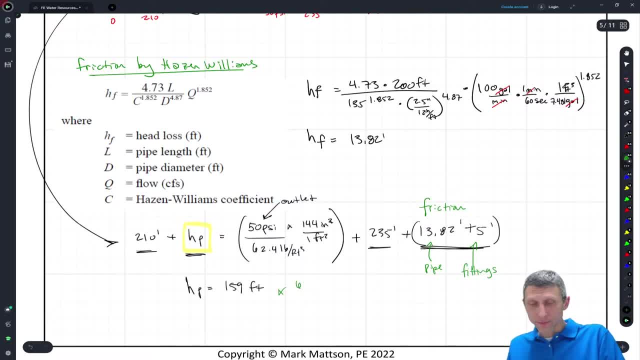 we're going to do here is we're going to multiply you know times um 62.4 pounds per cubic foot, um divide by 144 inches squared per- I'm sorry, Yeah, Per foot squared, And what we'll end up. 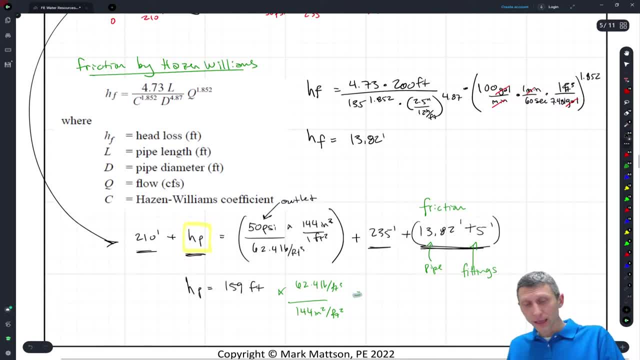 with here is: this is going to give us a pressure in um pounds per square inch And I believe when we do that out, um, what we get is 159, uh times 62, uh 0.4, uh divided by 144.. And that's like about 69 PSI, 68.9, uh PSI. 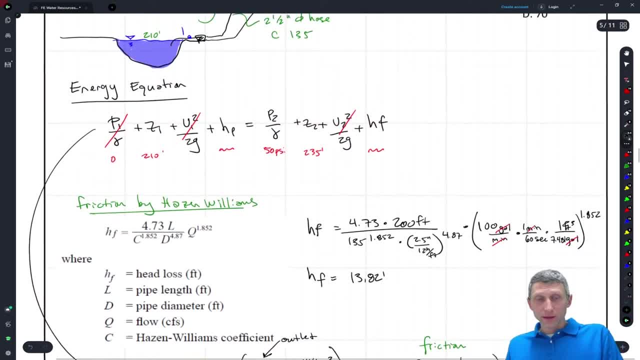 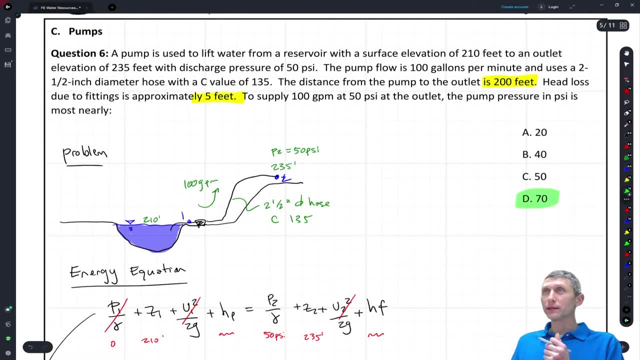 um, which is going to be um, most nearly, uh, most nearly 70.. So sorry, I don't know what happened with uh the stream getting dropped there for a second, but it looks like we're back live. 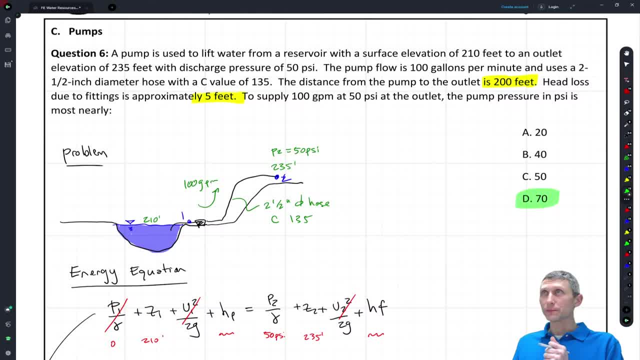 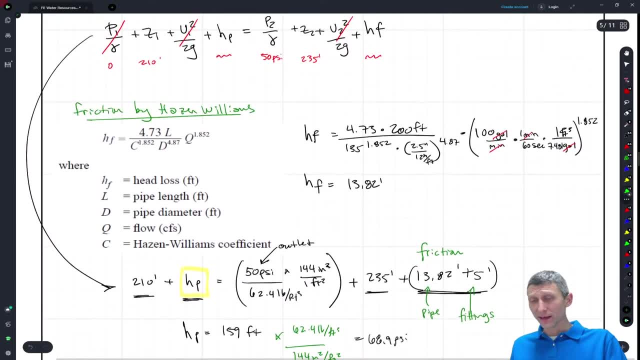 And we'll. we'll keep going with that. So thanks for your patience, But, um, hopefully, um, this makes sense. We're using the energy equation. We're finding friction, in this case by Hayes and Williams. Um, could you use Darcy-Weisbeck? Yeah, you could use Darcy-Weisbeck, Um, if you did. 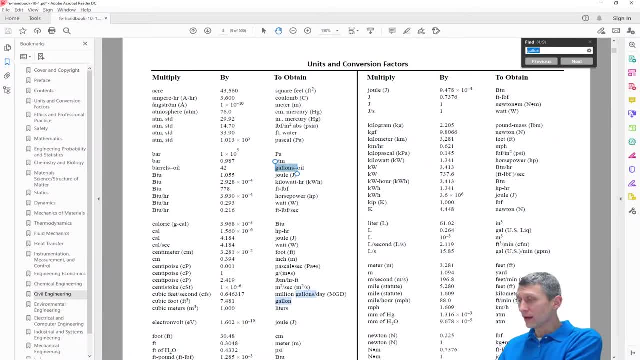 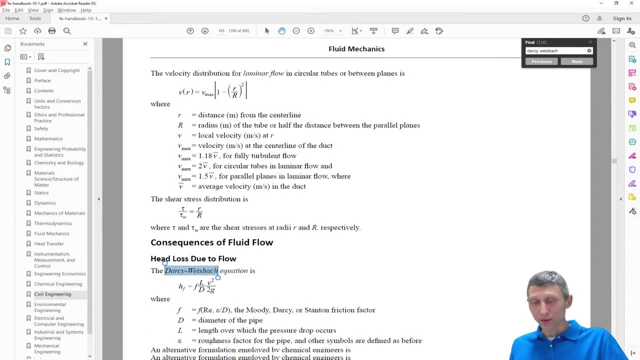 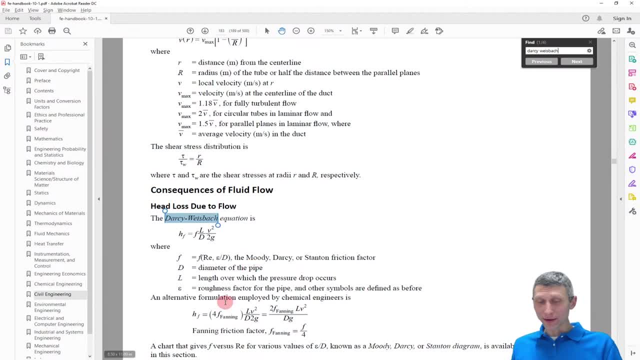 value friction factor: the the Moody diagram is given, right, So you can. you know, the the Moody diagram is given if you have to go there. Um, so that's another possibility, but, um, hopefully, uh, if you do, you can plug and chug there as well, Okay, So, um, you know. 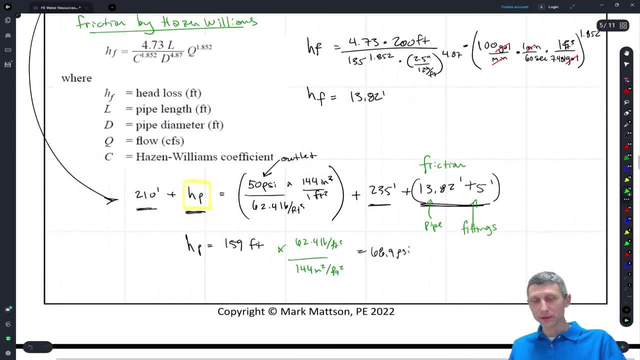 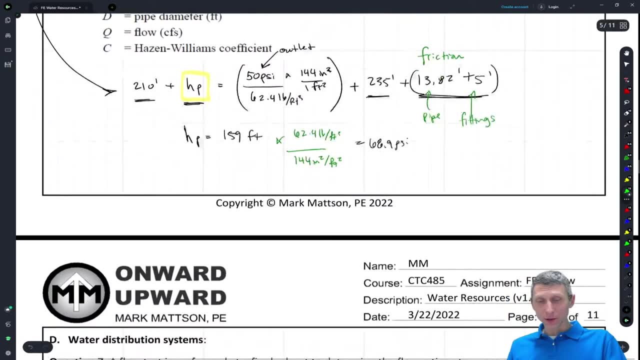 as we come back to this, though, again, knowing that energy equation, knowing how to put those, those losses in uh, is going to be key to solving this type of a problem. All right, Well, let's keep going and hopefully, hopefully, the rest is smoother, Um, and what we do here is: 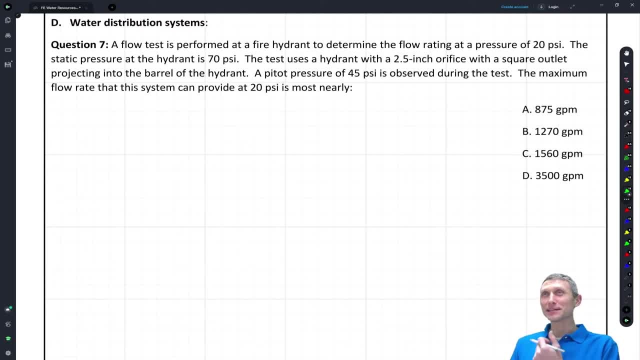 a flow test is performed. We're on water distribution systems. Flow test is performed by hydrogen during the flow rating at a pressure of 20 PSI. So the static pressure, the hydrogen, 70 PSI, has to use a hydrogen two and a half inch orifice with square outlet projecting into the 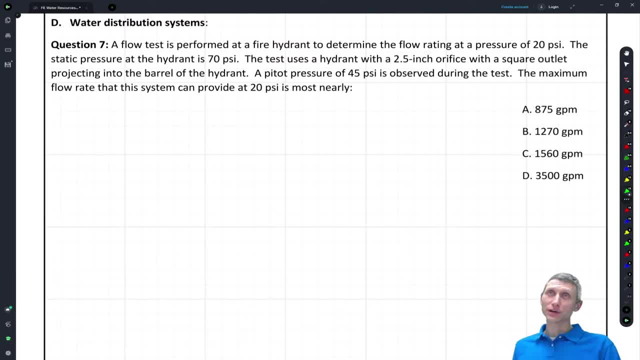 barrel of a hydrant Um a pitot pressure of 45 PSI is observed during the test. The maximum flow rate of this system can provide a 20 PSI is Almost nearly So when I was in consulting one of the things like full-time consulting. 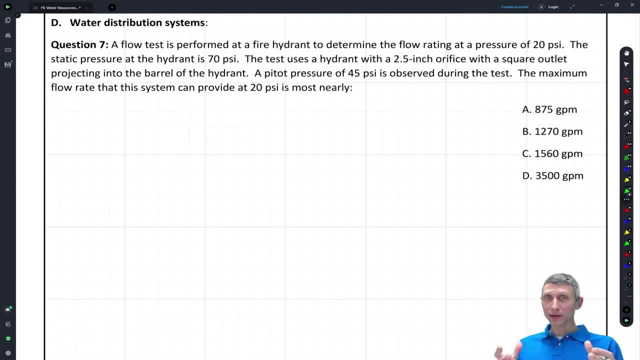 one of the things that we had to do is we're putting a site together and we have to work with the fire protection engineers to make sure that there's enough fire flow at the site before the building. So, um, one of the things that I was doing is, as, as I was looking through, 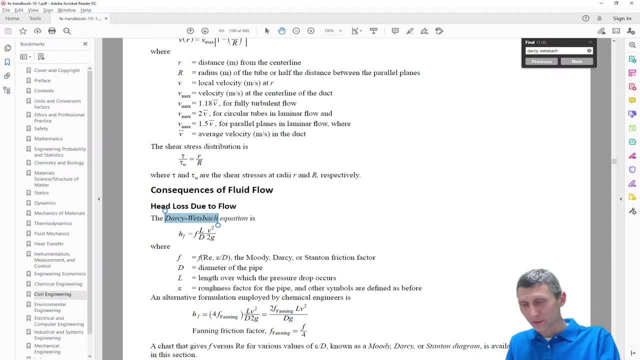 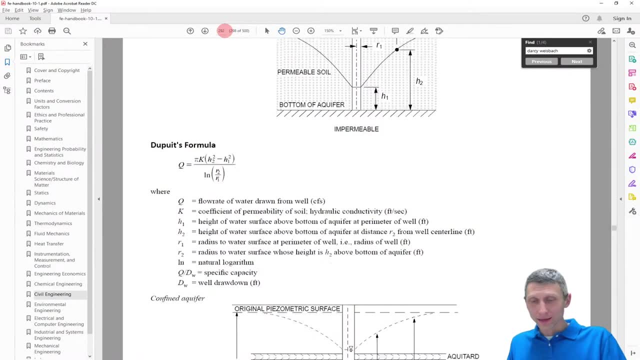 this, the, uh, the, the reference handbook, um, right, And we come in into this right, Um, and I I come back into, like you know, the, the water resources section, Uh, what we get into here. 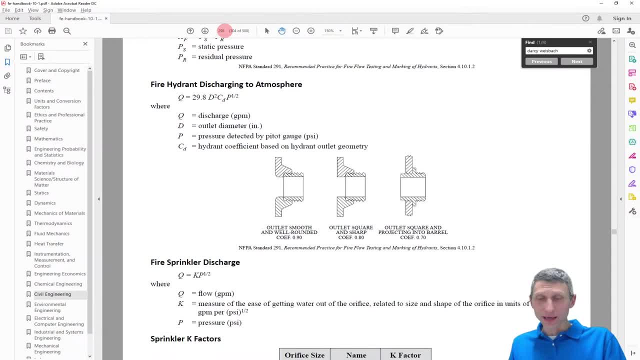 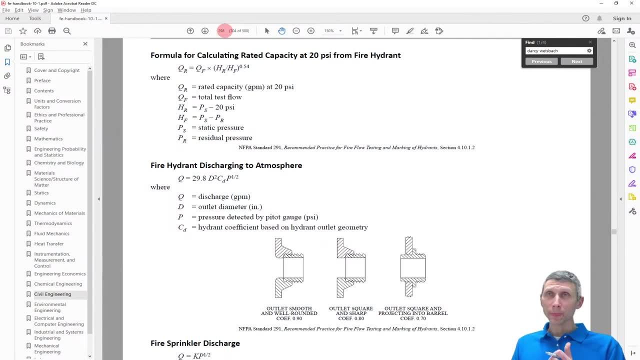 is all of a sudden we get to some fire hydrant calculations And one of the big things for civil engineers is you might not be doing the fire protection system. that might fall on your mechanicals. Um, but one of the things as a civil engineer is you're dealing with the water. 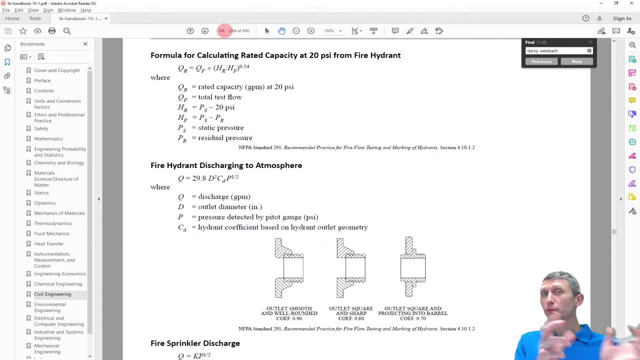 distribution outside, So you have to make sure that you have enough flow for the fire protection engineers. So, um, when I saw this, I was like you know what? that's one of the things that I actually we had to do in the real world. We had to go to get fire flow tests at our project sites. 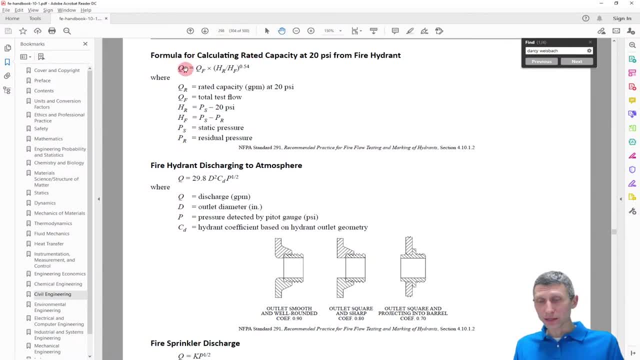 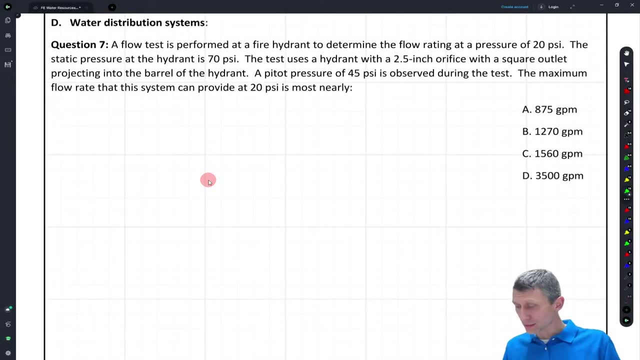 make sure there'd be enough flow at the site. So we're going to use these two equations here, uh, to solve this question. So I'm going to come back and take a look at it, Right? But, um, basically, the flow test is what we need to do. So the first thing that we're going to do, 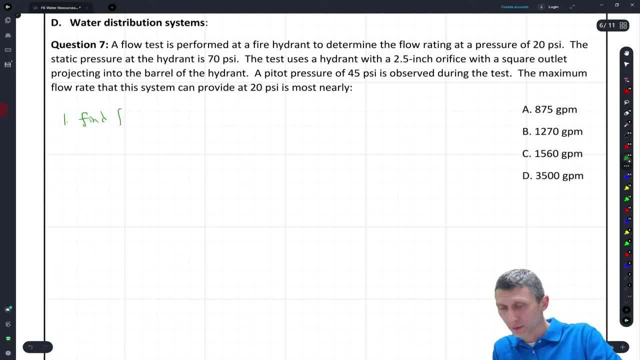 is, we're going to find, um, the flow at the hydrant Um. uh, so we're going to find the flow, um, at the hydrant Um, at the test pressure. So this is kind of step one here, And with step one this is kind of a two-step process, You might. 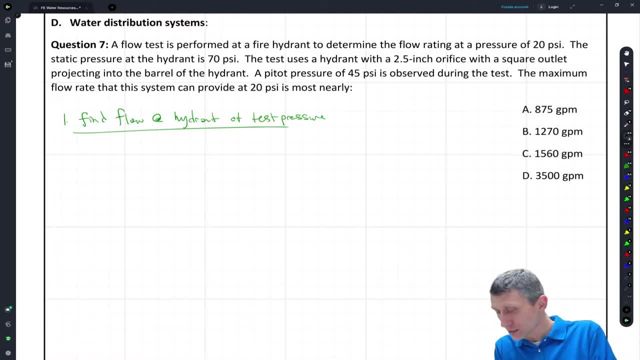 get just only one of these, but at least, um, you're there. And the equation for that one was just: Q equals 29.8,, uh, times. This is an empirical formula, It's calibrated, but times, if you. 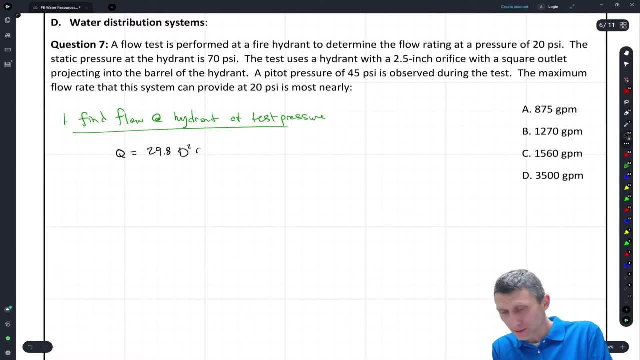 if you're looking at your reference handbook, it says D squared and times CD, uh, times P. this is going to be Yeah To the one half. Okay. So the nice thing is this: 29.8, it has some conversions in it already, but 29.8 D is going to. 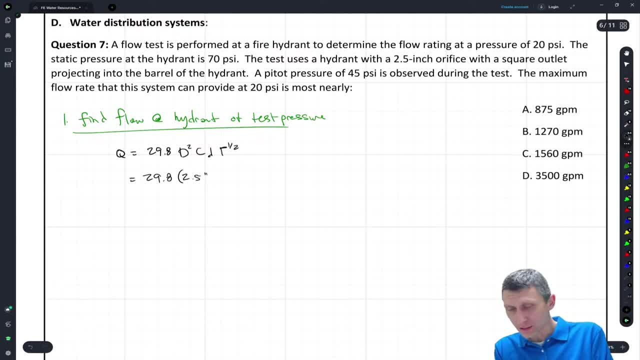 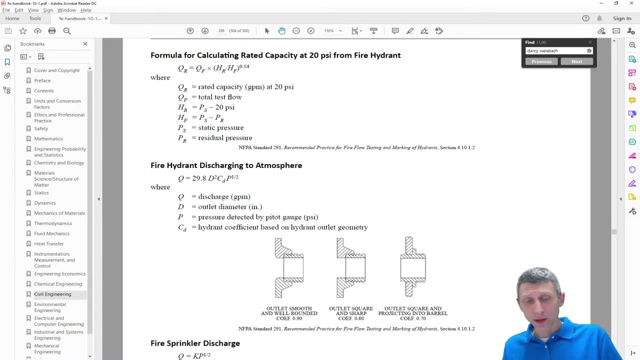 be our outlet diameter. So we have a two and a half inch orifice in. D is an inches Um times CD, which is a factor for the hydrant coefficient. So if we come back to, We have a square outlet projecting into the barrel. 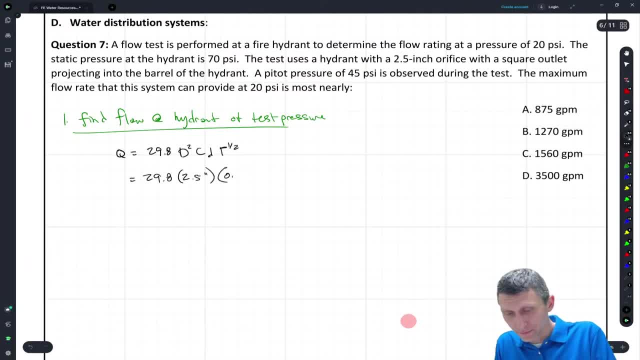 That's going to be our 0.7.. Okay, So 0.7.. Is that right? Right serum times our p, which is our pressure detected by the pedo gauge. so the pedo pressure of 45 psi is what we're going to use. so 45 psi, so our flow at the test pressure. so this is our q, maybe. 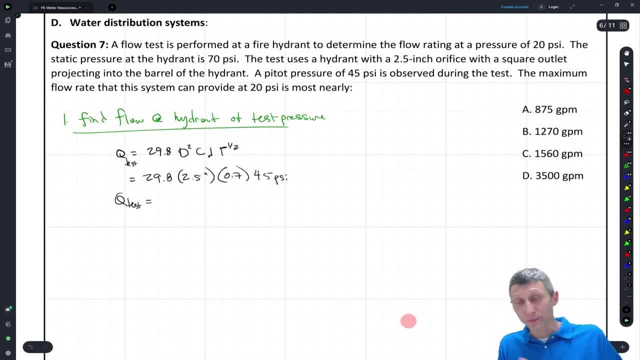 test. all right, this is our q at our test is going to be some value here, right? so if we, if we plug that value in, we get 29.8 times 2.5, and i gotta keep remembering those squares, 2.5 square times. 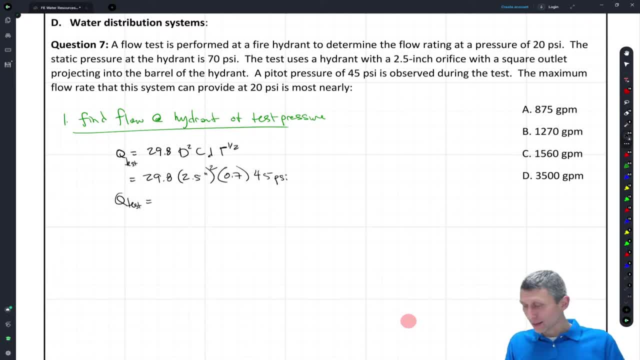 0.7 times 45 and i get like, uh, something wrong because i didn't take the 45, i didn't square, take the square root of the 45. so let me do that one more time and i get about 875 gallons per minute. 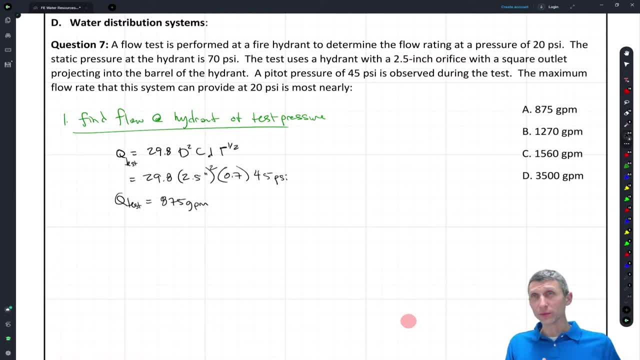 so that's the flow during the test. so what do they do? um, at the test, they go they. they open up the hydrant, let it rip and they take a pressure reading and figure out how much pressure is is coming out. you convert out the pressure reading and figure out how much pressure is is coming out. you convert that. 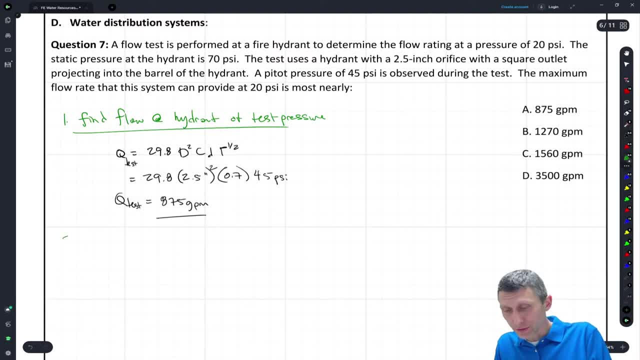 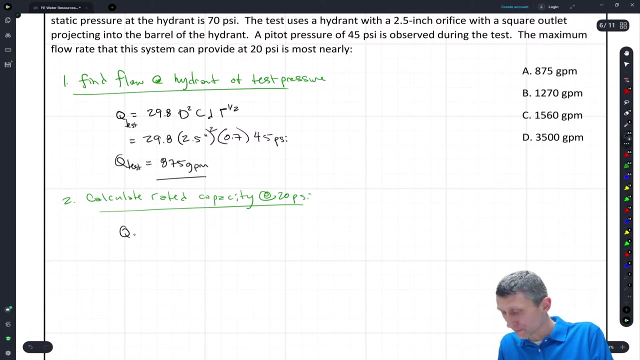 pressure, uh to a flow. so that's step one. um. step two is you calculate, uh, the rated capacity at um at 20 psi. okay, so this is about as low as the pressure you want to go and still have pressure to fight your fire. so what do we do here? um, this is just another equation. so qr equals qf times hr. 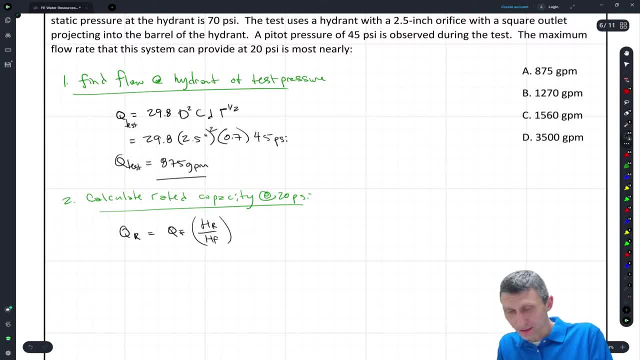 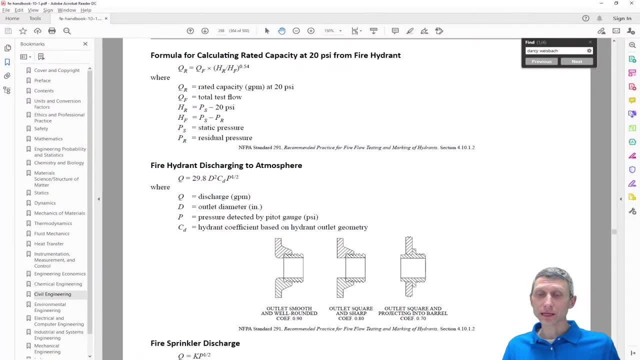 over hf, uh to the 0.54. you gotta love these empirical equations with all sorts of crazy uh exponents. but what does this look like here? um, essentially, what this looks like is that we have the test flow. the rated capacity at 20 psi is what we're looking for. um, we have this hr, which is ps. 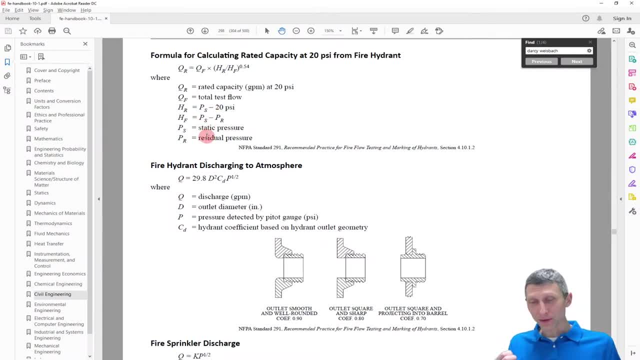 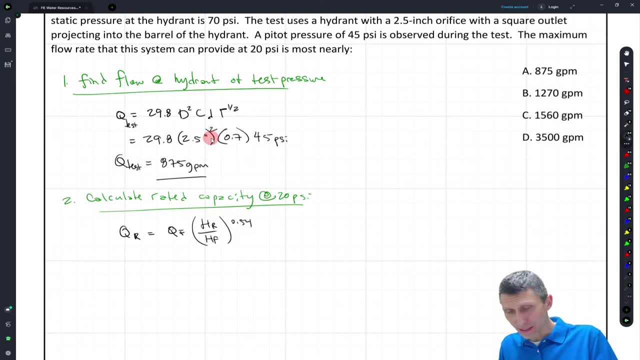 minus 20 and ps minus pr. so you know, we have a static pressure and our residual pressure and once we have all those pieces, we can come back in here and plug in um. but essentially this equation looks like: um, we're going to have our 875 gallons per minute. 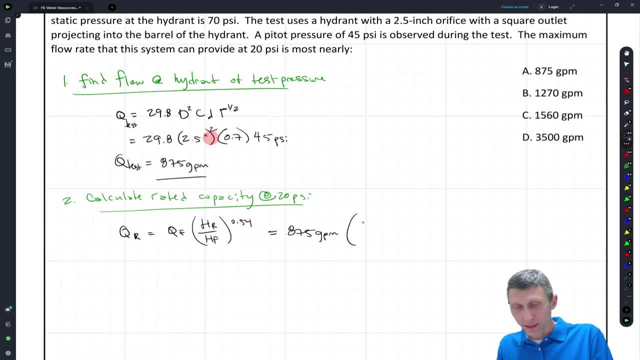 times our hr, which was uh, hr um was, was ps, our static pressure, minus 20 psi, that's the the lowest we want to go, and then hs or hf, i'm sorry, is our um, our static pressure minus our residual pressure at our test. so pr um okay, so we can, we can plug those in, but we get set. 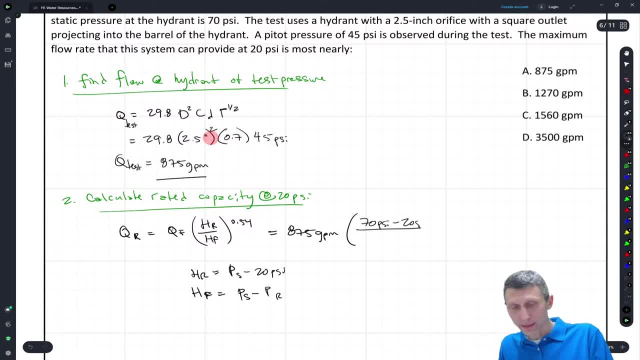 bindi, which is our static pressure minus 20 psi, um, divided by our static pressure, 70 psi minus 45 psi and um, we raise that to 0.54 power and we get a value of qr equals about 1272 gallons per minute. okay, so this would be the maximum amount of fire flow available at that site. uh, and. 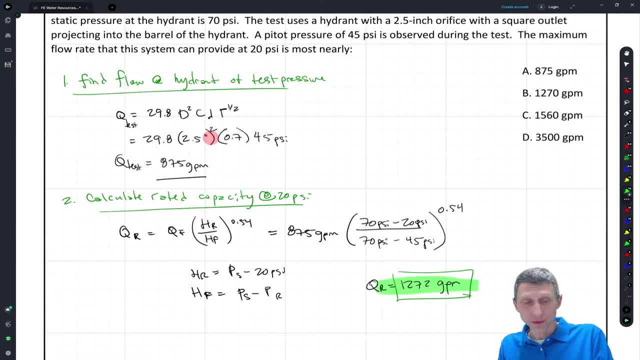 you know for for where we are at 20 psi. okay, so 1272 is close enough to 1270 that we're going to go with it all, right. well, no hiccups there, hopefully. uh, our stream is back and and not screwing up here. 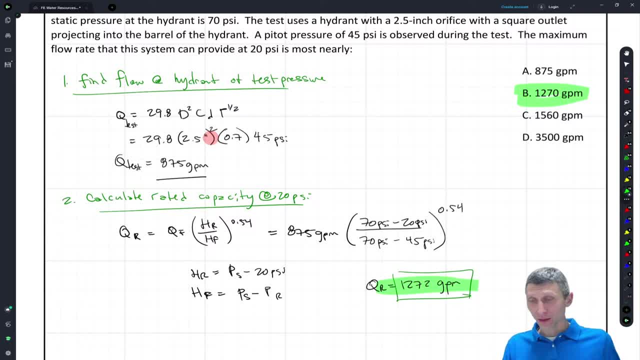 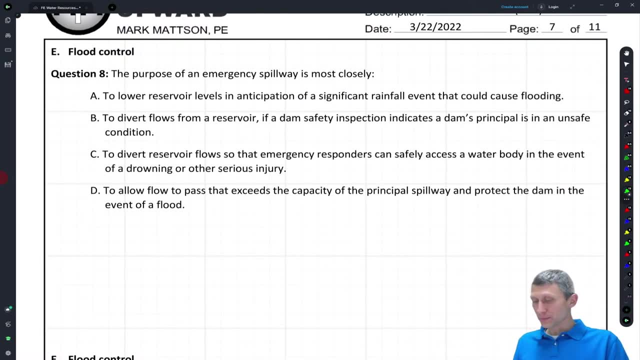 so let's keep going and uh see where we go. okay, the next couple questions are: are um concept questions, so purpose of an emergency spillway? what's an emergency spillway? it sounds like it's used in an emergency. so, um, don't take the bait and don't say that it's for first responders, okay. so emergency responders? no, that's, that's not what. 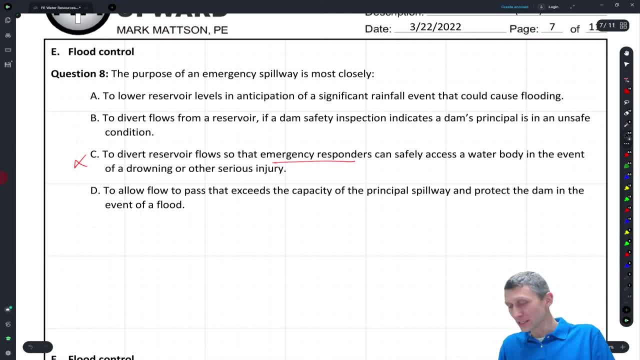 it's for emergency spillway is not for that um. what is an emergency spillway? well, at a dam, typically you have some um, so you should. at a dam, typically you have some normal spillway. sometimes you'll have some, uh, some gate structures right. so where you have maybe a couple gates and then you 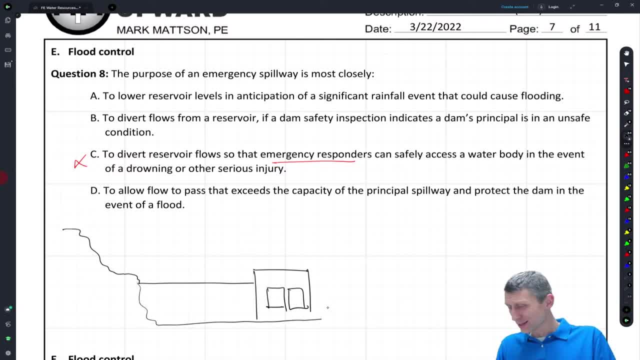 know. so you're going to come down here and this is your dam, uh, and then, as you go up from there, maybe you keep going up and you have a, maybe you have like a uh, a little bit of a um, a little bit of a, an earthen section of this dam, and then at some point you keep going up. well, at some point, right. 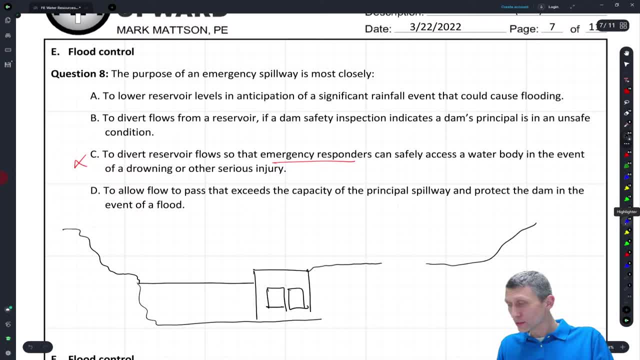 the water level starts to rise. so what we don't want to have happen is: we don't want to, we don't want water to over top our earthen dam, right? so? so this might be our like, right, so we might have, like, a spillway, all right, we might have a gated dam, a gated section. 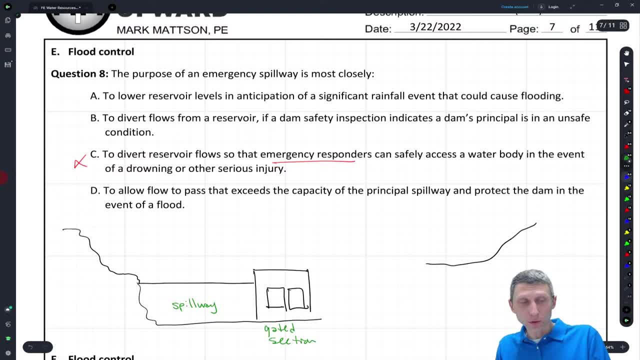 right, so the gates can get opened up so we can pass a whole bunch of flow. um, you know we can pass a whole bunch of flow through those gates. you know we're going to have some flow coming over the spillway. but what we don't want to have happen is we don't want water to flow over, um, like if this: 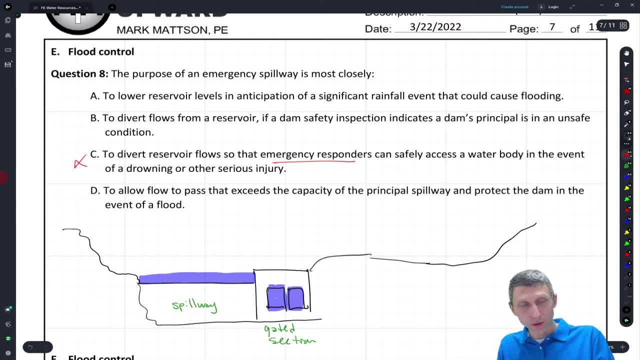 is our. you know, this is our, our dam here, our earthen dam. we don't want water to flow over our earthen dam. why not? because water erodes earth. okay, we don't want water to flow over an earthen dam. so what we're going to do is we're going to knock out a section. 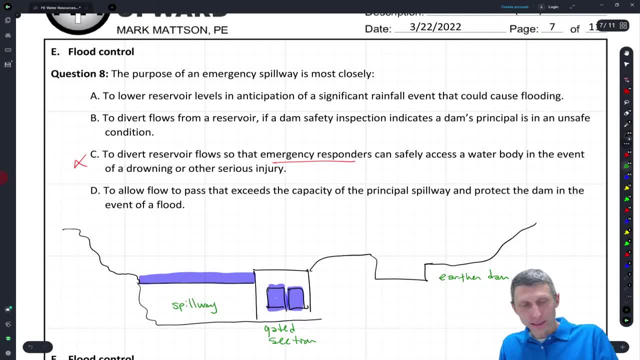 of that dam and we're going to put in a spillway so that, as the water level rises, right, we're going to, we're going to, we're going to pass enough flow here so that we never end up, uh, going over our earthen dam. so this is going to be like our emergency: uh, spillway, okay, and that's going to. 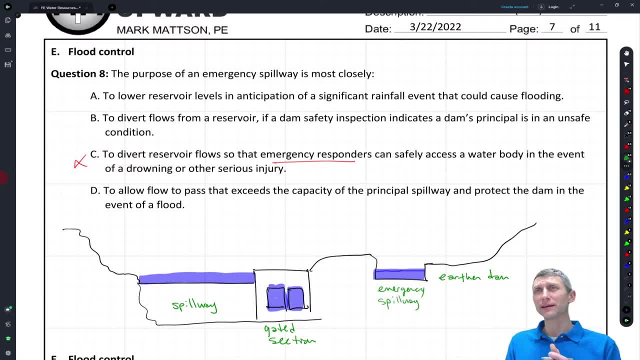 be used to control the flood levels, and whether it's an emergency spillway in a dam or it's a water control structure that has a weir to pass flow, which will be used to control the flood levels, be in a couple problems. we'll do that. what this is doing, we're we're allowing this to to pass flow. 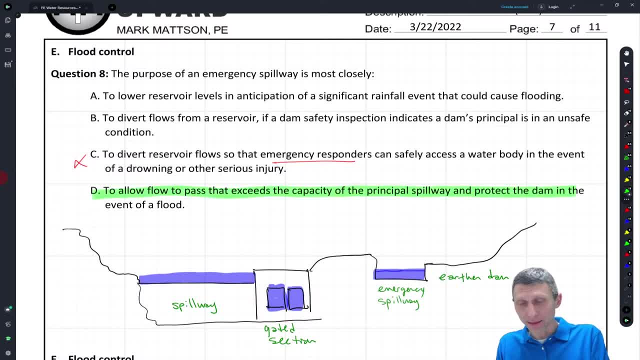 that exceeds the capacity of the principal spillway and protect the dam and the event of a flood. so that's what the emergency spillway is doing: it's it's allowing us to pass enough flow that we're not going to overtop, uh, the earthen dam. okay, we're not. um, we're not, we're not here. 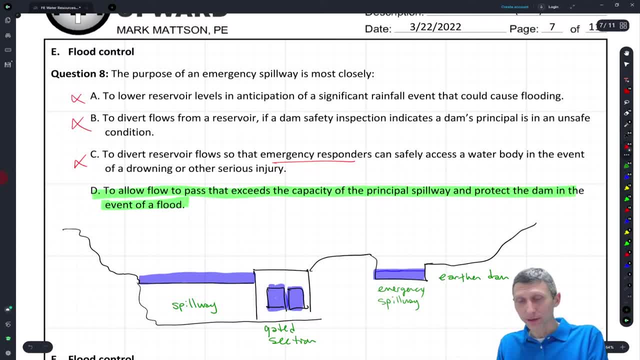 diverting flows from a reservoir. we're not lowering the levels of a reservoir in the anticipation of a rainfall event. right, this is, you would use gates, you know, potentially to lower the reservoir level. um, divert flows. uh, you would again use gates to go into, like some secondary channels or something. 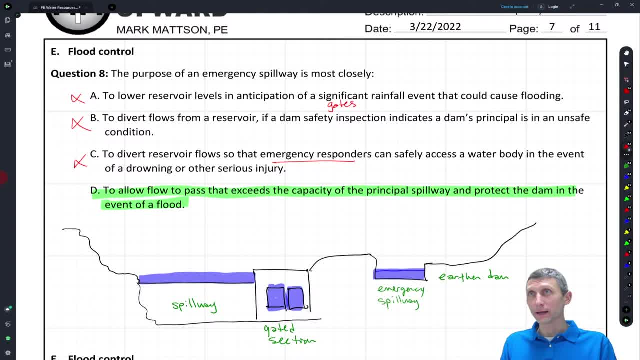 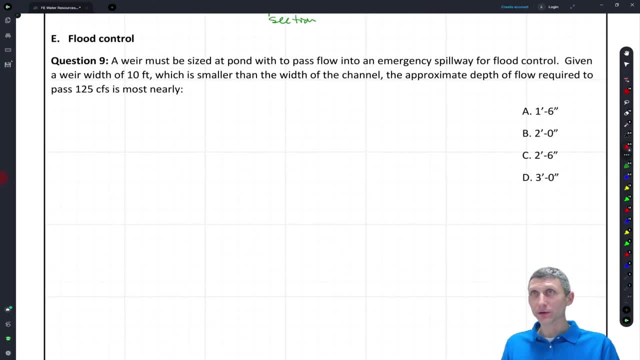 like that. but this is um, this is flood control. uh, kind of 101. so hopefully that question makes sense. um, in this kind of is a spin-off of that question. right, we have a weir. it must be sized at a pond, um, at a pond, i thought i added that, but i must not have um. 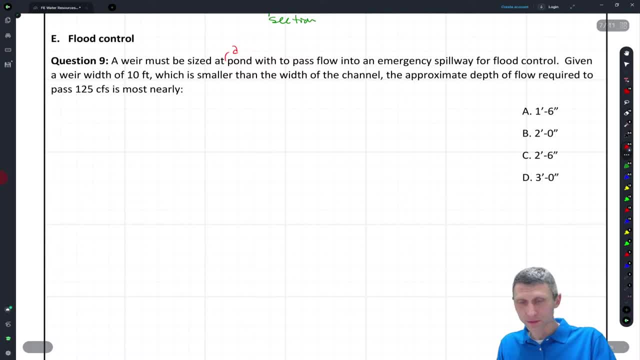 a weir must be sized at a pond to pass flow into an emergency spillway for flood control. given a weir width of 10 feet, which is smaller than the width of the channel, the approximate depth of flow required to pass 125 cfs is most nearly so this is going to get us into a weir. 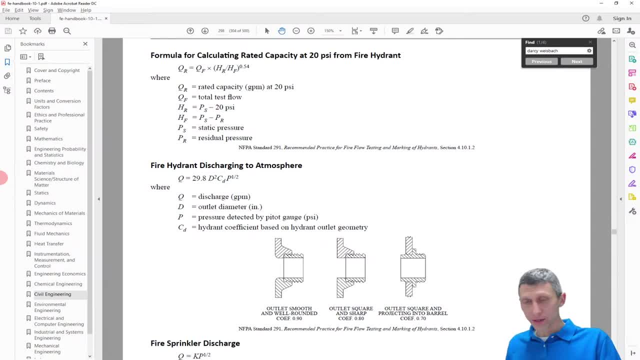 equation, right? so, um, this is going to get us into a weir equation, and uh, let's come back to take a look at what that looks like here. so, this is going to get us into a weir equation, right? so, um, this is going to get us into a weir equation, and, uh, let's come back to take a look at what that looks like here. 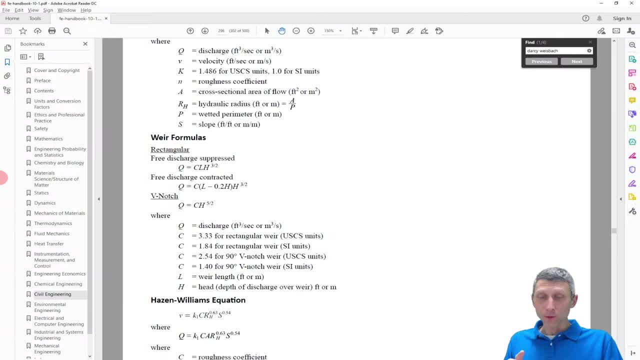 and here we have some weir formulas. um, we have rectangular, we have free discharge suppressed, we have free discharge contracted and we have v notch. so, ah, which one do you use? well, the good news is they're not. they're not crazy different, for even the suppressed and contracted. but um, let 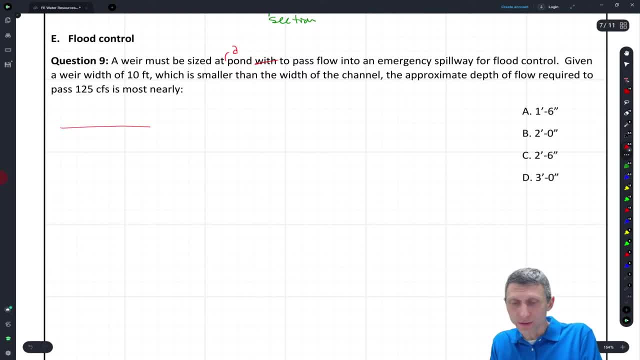 me just show you what those look like real quick. but basically what we have is again, we have this um emergency spillway where if you think of you have a dam, you're going to have some channel that's blocked out here to pass a certain amount of flow, right. so in our case, we're going to have 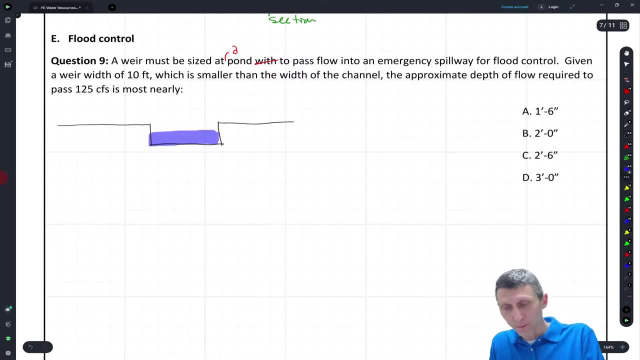 90 cfs. right, so our flow, our q um is 90 cfs and we have a width of, we know our, our channel width. we've got 10 feet for it and, uh, you know, behind this we're going to have this water level. that's. 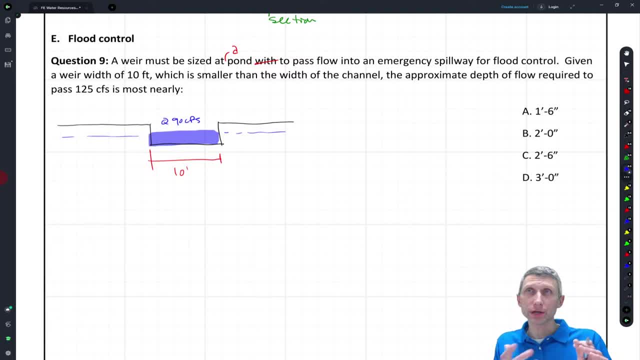 being held back by the dam. because that's what we're trying to do. we're trying to figure out how to pass 90 cfs, what this depth of flow is going to be right, so that's the depth, um, or in this case i'll call it h, right? so the types of weirs that we're going to be passing are going to. 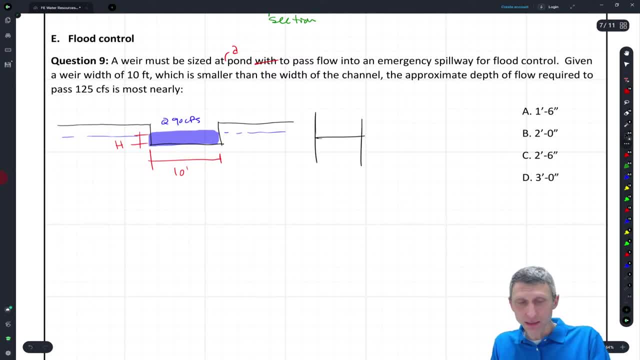 be in the same length that we have. we have a suppressed uh, which means essentially, um, the whole thing, or uh, the the water flow is over the whole channel width. okay, so this is um, this is one version of that uh. we have a contracted. okay, an equation for contracted. contracted looks like this: 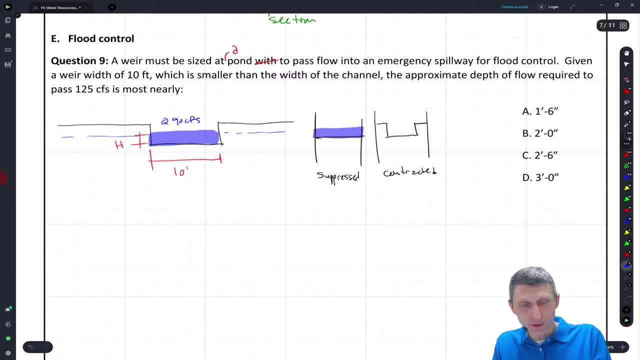 where we have, uh, a weir that's less than the full width of of the pond. so in this case, we're going to, we're gonna have contracted, because this reservoir- right, this reservoir- is bigger than just the spillway. okay, so we're gonna use the contracted formula. I'm the 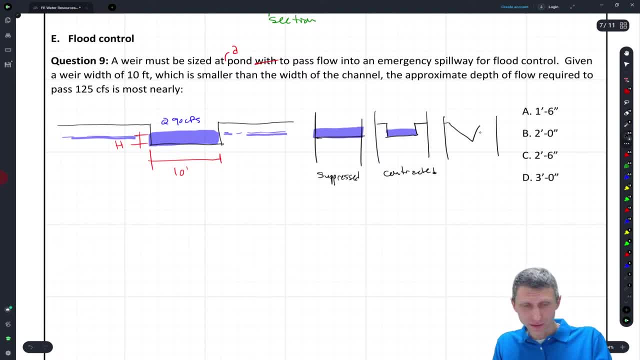 last one here I'll just show for completeness is: you could have like a v-notch, right, so we could have like a v-notch. we are, and those are. those are useful because, as the you know, flow gets higher, you can pass more flow and less flow as the flow is lower. so this is like a v-notch and the equations for 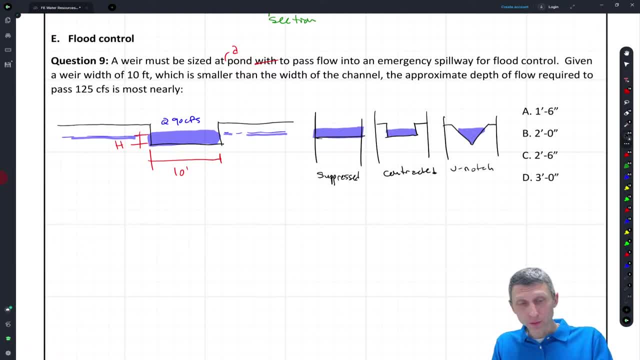 each of those are in the manual, but the the equation that we're gonna use here is: we're gonna go with a contracted, because our pond is typically going to be bigger than the little spillway that we're going to pass this flow on. okay, so if we look at that equation, we're gonna have Q equals C times L minus 0.2 H times. 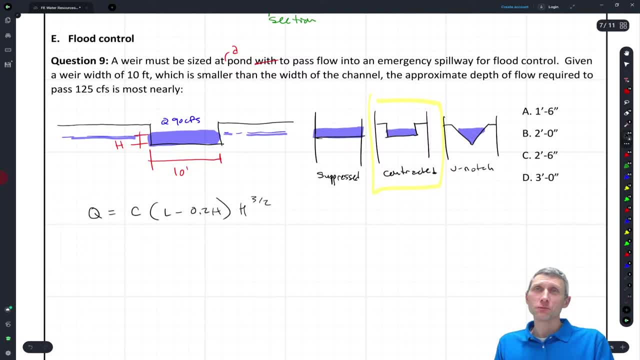 H to the 3 halves, at which point you say I don't want to solve for H because that's just a mess. honestly, it's a mess. um, there are some approximations. right, there are some approximations. this is not in the handbook, the this you know. there are some approximations that show up, like in: 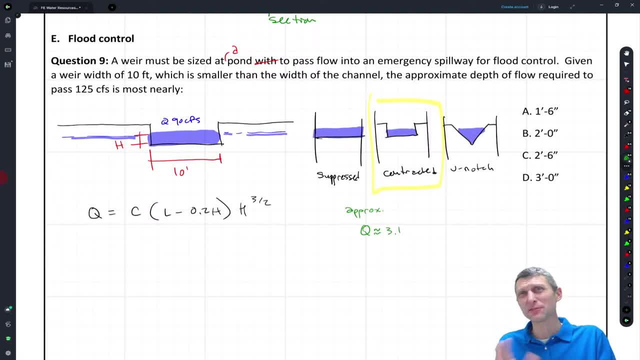 the New York State so on, or management design manual that just says we'll see for a contracted we're maybe, as likes you know, 3.1 times L, H to the 3 halves. so that's a good approximation. but if you don't know it, where do you go? where? 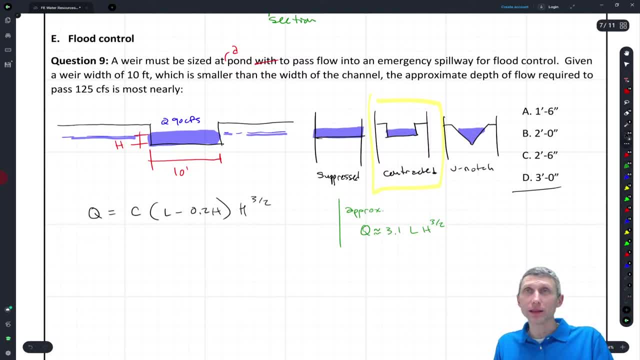 I go, is I just I? this is where I try to cut my losses. I got, I got four answers and I've got a calculator. okay, so I'm just gonna plug in, because when we come back, when we come back to the handbook, right, what do we have? we have C for a. 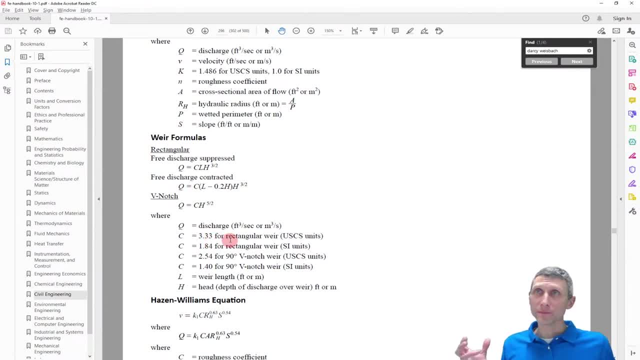 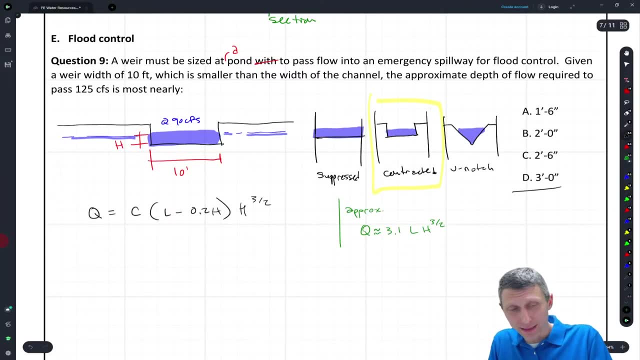 rectangular weir. this is sharp crested rectangular weir. it's gonna be 3.33, okay. so what we can do is we can. just you know, we can plug and chug here. I mean honestly I think that's gonna be the easiest, but plug and chug, okay. what I'm 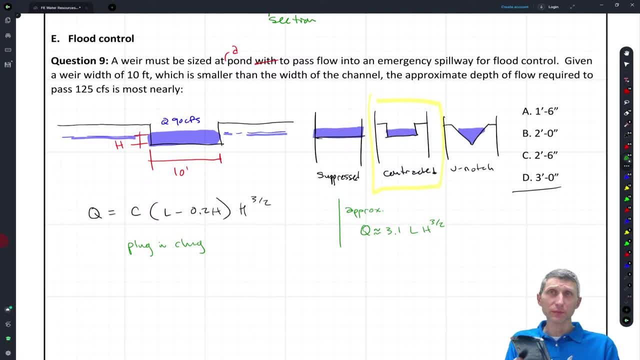 gonna do is I'm just gonna stick it in my calculator once. so I'm gonna say 3.33 and times. what do I have? I have um, so this is gonna be: Q equals 3.33 times 10 feet minus 0.2 times H, times H to the 3 halves. so what I'm doing is I'm just 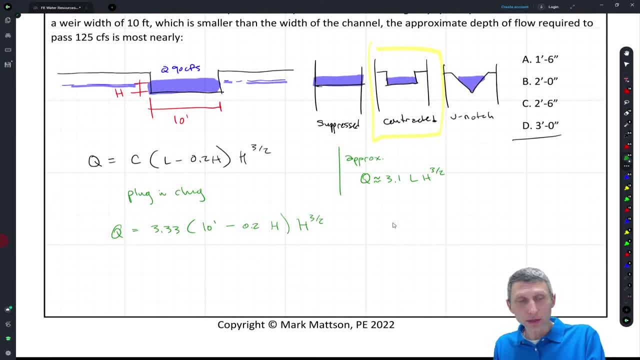 gonna plug this in. so I'm gonna plug this in, I'm gonna say okay, for I'm gonna say, well, what Q do I get for each of these Heights if I plug them in? okay? so that's the. that's gonna be the easiest way, I think, to do this, because you have 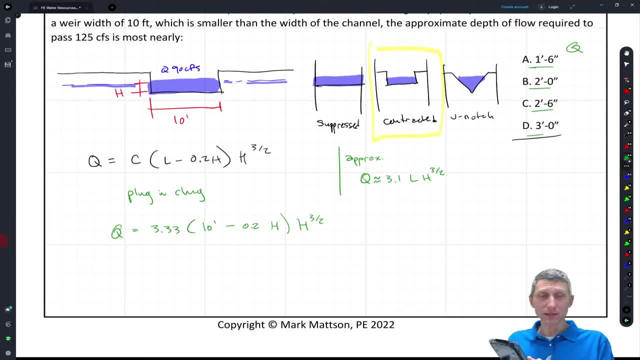 a limited amount of time and solving for H is just a bear. but if I just start like, and I do 1.5 feet times 1.5 to the 1.5, you need like about 59 CFS. okay, and then the beautiful thing of. 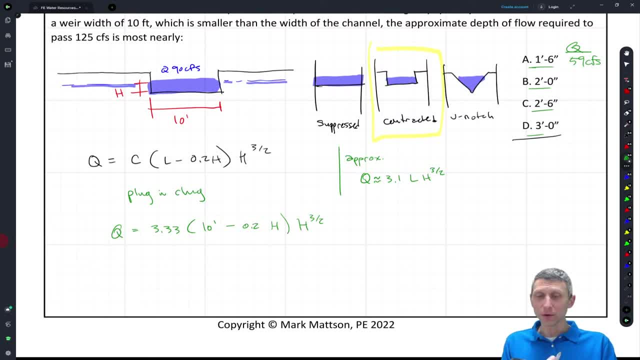 the calculator is, you can go back. I mean you can put the function in your calculator and look at a table, or you can put each one in individually. I mean you just hope it's not the last one, because then you just waste all the time. but but even so it's not wasting that much time. I get 90 CFS. I'm getting closer. 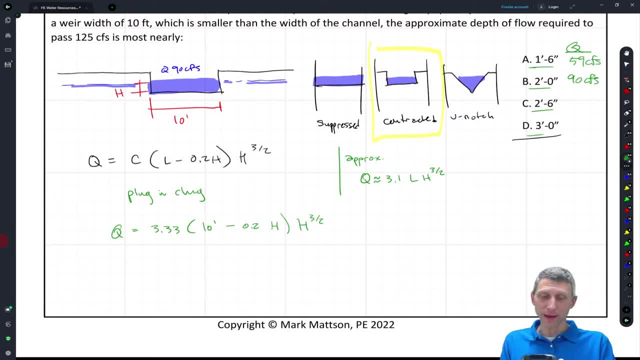 and then we can just start calling each of those in one by one, so, and then we can just sort of get there together literally and do each one along the way. that way, the rest of this thing where, far as I go to 2.5, I think we're going to be spot on. So what do I get with that? I get about 125 CFS. 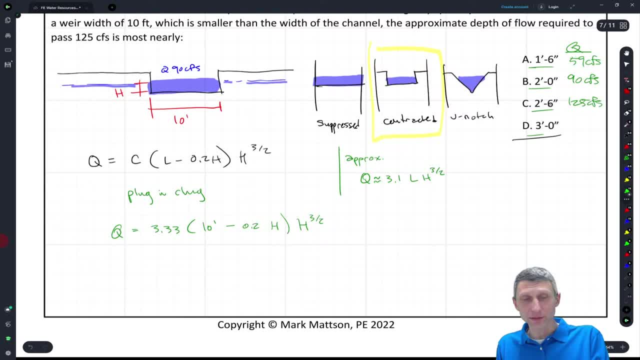 Okay, And I can go to the next one too. At this point, though, I would stop, and I would, just I would, I would highlight it in. I'd say that's good, That's going to give me my 125 CFS, So this. 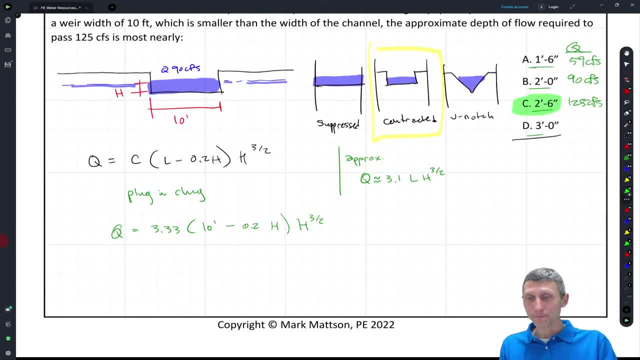 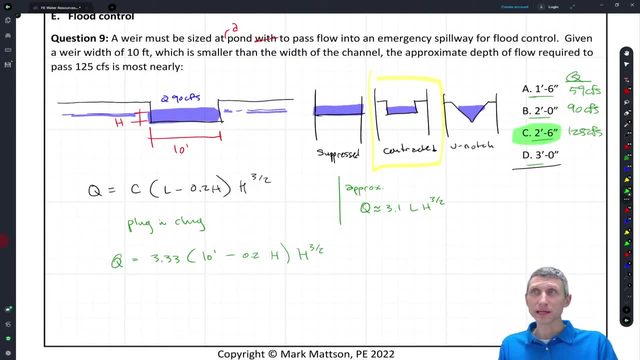 is kind of a brute force approach, but sometimes, um, that's what we're looking for is is, uh, trying to find how we're going to get 125 CFS with this. Okay, So, even with this approximate formula three, so we, uh, we can go back and check this, but with this approximate formula 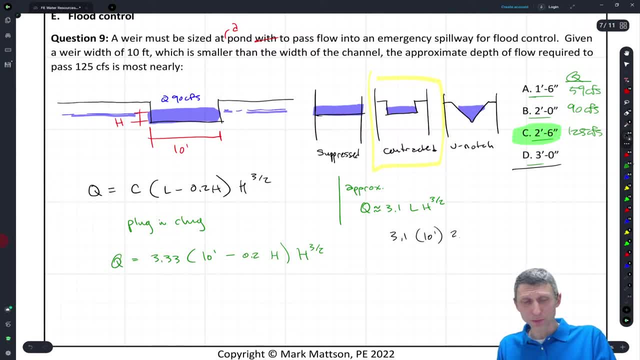 3.1 times 10 feet, um times what- 2.5 feet to the three halves- this is going to give us an approximate flow. Again, this isn't in the manual, but it's a. it's a reasonable approximation. 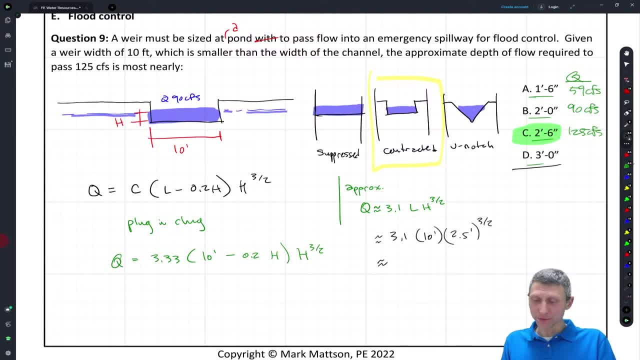 um times 10 times what 2.5.. Five to the uh, 1.5.. This is going to give us about, you know, one, 23 CFS. So again it's, it's really really close. Um, but this, you know, this version of the equation. 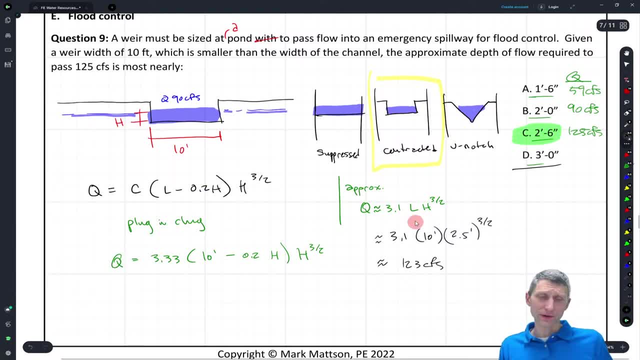 isn't in um, isn't in the handbook. Okay, So this version isn't in the handbook, Um, but it's uh. you know, what I would do here is I would kind of plug and chug this brute force it. 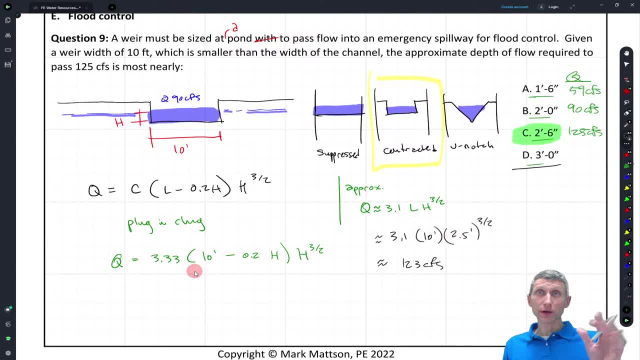 and keep going. All right. So we're equation. I could definitely see that in. I could. I could definitely see it in flood control, whether it's an emergency spillway or it's a water control structure, uh, where you have to limit the or you have to provide a certain out discharge at a. 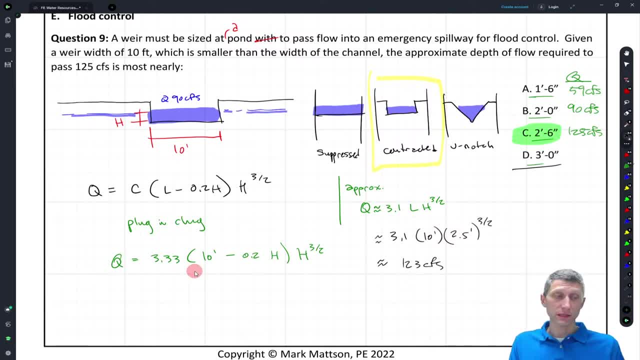 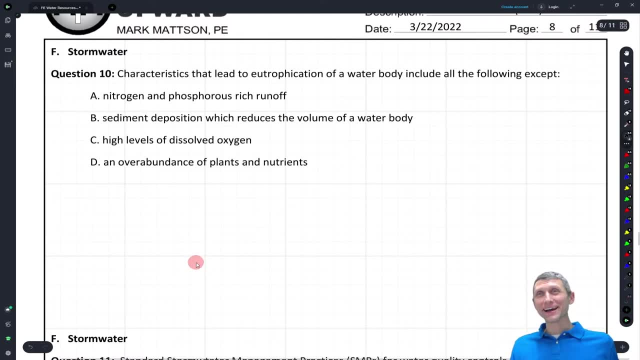 certain flood stage or elevation of a pond or something like that It's. it's one of those basics that I think is is probably going to be tested. All right, here we go. I threw this one in honor of when I took the PE. when I took the PE exam- uh, actually, I had a question that talked. 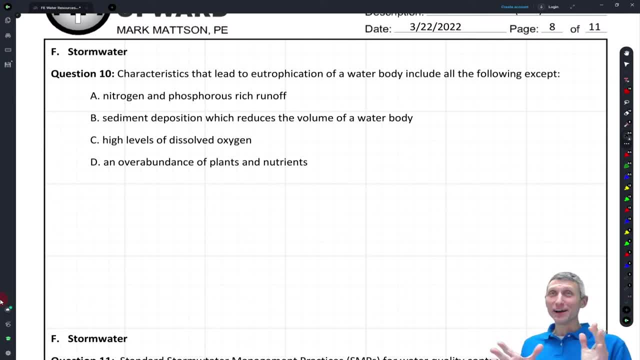 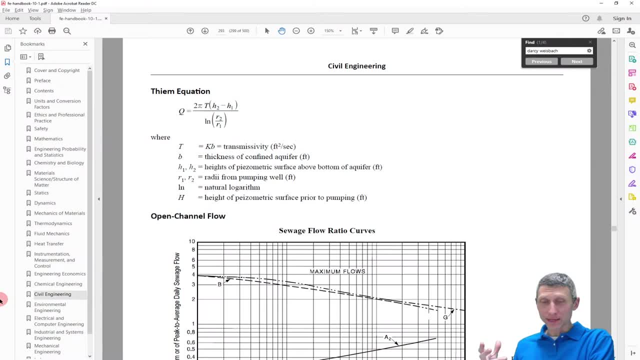 about eutrophic water bodies And I was like, Oh man, Um. but I threw this one in honor of that And also because because it does show up in the FE handbook, but when you come into the FE um reference handbook, 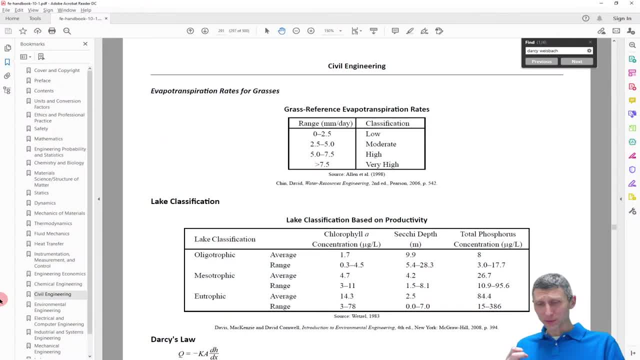 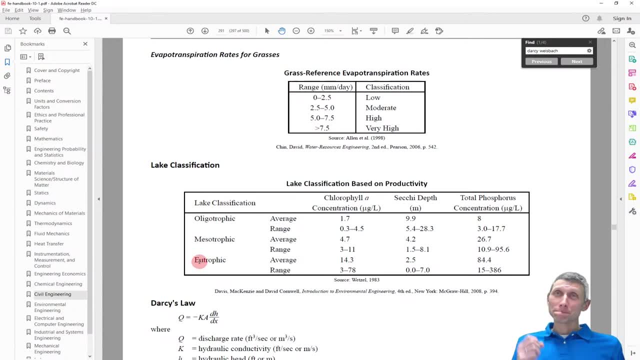 and you come back to evapotranspiration. you know transpiration. you come back to late classification. you get some terms in here like oligotrophic and mesotrophic and eutrophic- right, What do we see with eutrophic? There's a lot of chlorophyll. Okay, So we go from 0.3. in a oligotrophic to three to 78. in eutrophic, Okay, The total phosphorus, we go from eight to 15 to 386.. So, eutrophic, we go from eight to 15 to 386.. So, eutrophic, we go from eight to 15 to 386.. 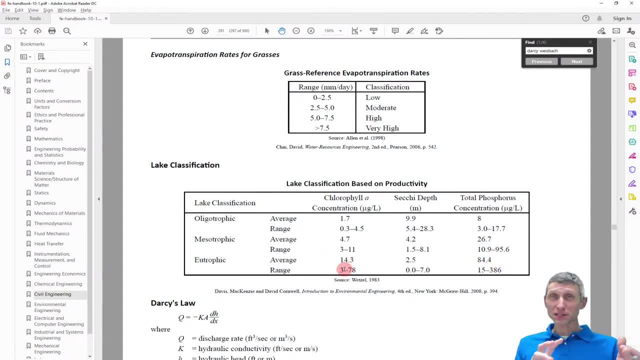 A lot of phosphorus, a lot of chlorophyll, because phosphorus is a fertilizer. It makes things grow really well And especially nowadays, when we have a lot of fertilizer out there and it gets washed into our streams and lakes, it can cause blooms of vegetation and even algae blooms. So when we 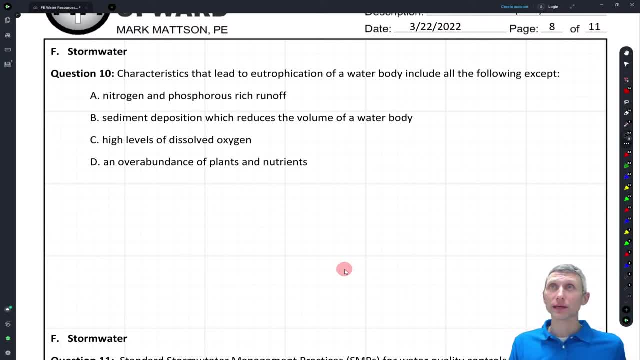 come back to this question. we say characters characteristics that lead to eutrophication of water body include all the following except um: nitrogen and phosphorus runoff. Yes, 100%, That will cause eutrophication, uh sediment deposition. So the so basically eutrophication. 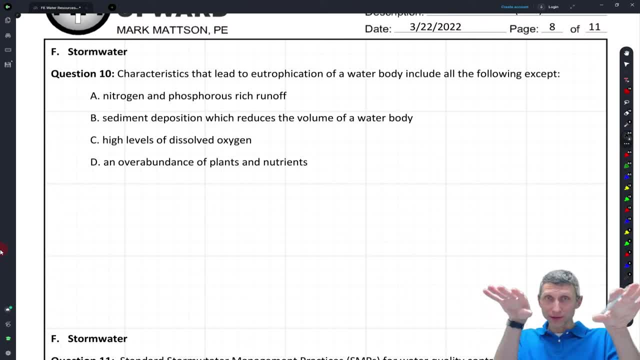 happens when the mineral content increases, right. But if you start depositing soil and filling up a lake, it's going to now have the same mineral concentration in a shallower volume. So you're going to get more minerals, you know, per volume. So that'll cause it to. uh, I'm going to skip. 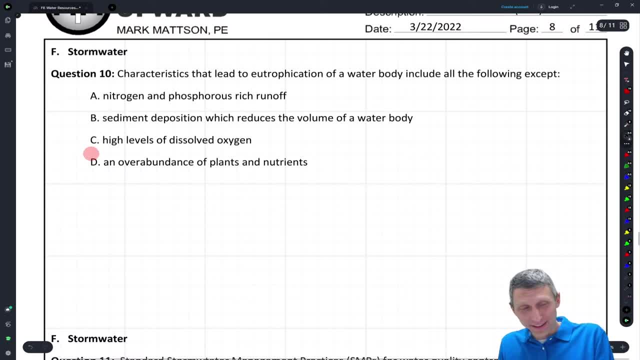 high levels of dissolved oxygen, because that's the answer. Um, you know, I'll just I'll highlight that answer. Actually, high levels of dissolved oxygen Is good. When you think about, um, a lot of, uh, a lot of, like ponds around a building, you'll often 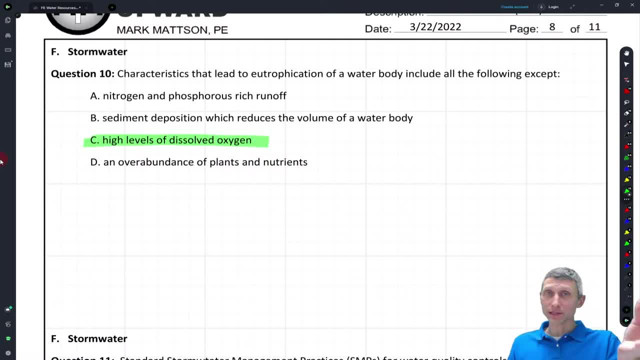 see a fountain in it, and the fountain is decorative, It looks nice, but it also adds a lot of oxygen into uh, into the um, into the pond, which helps with with decomposition and that sort of thing. But again, an overabundance of plants and nutrients. these two go hand in hand, So more. 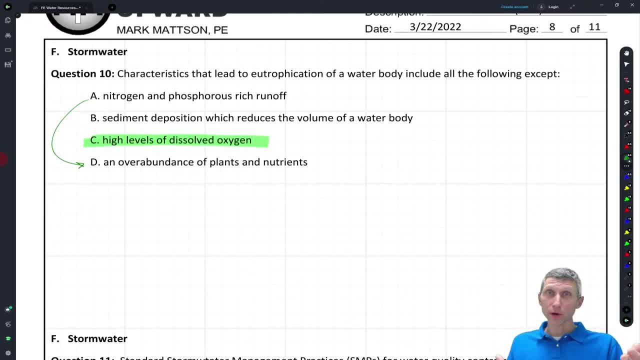 fertilizer into the water, more blooms, a more decomposing mass which eats up that dissolved oxygen, which is better. So that's a good answer. So that's a good answer. So that's a good answer. It's not bad for, uh, fish and and um other aquatic life. Okay, Deutrophication one of those. 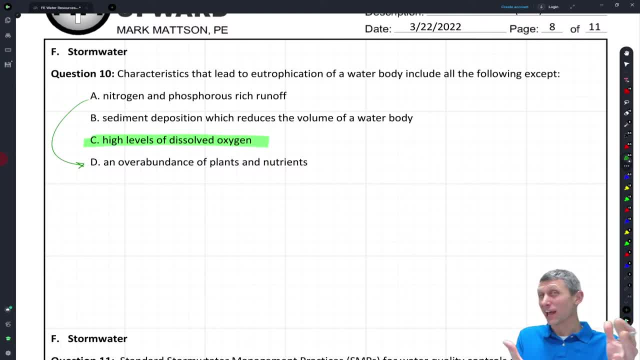 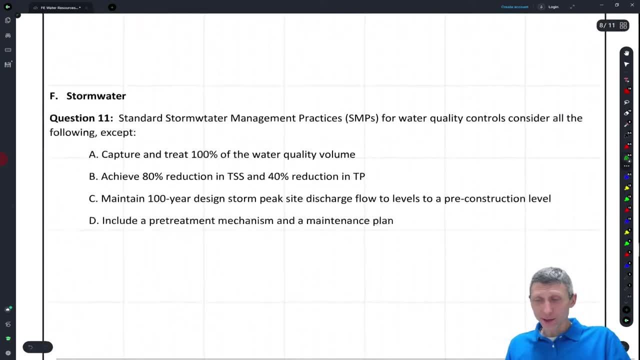 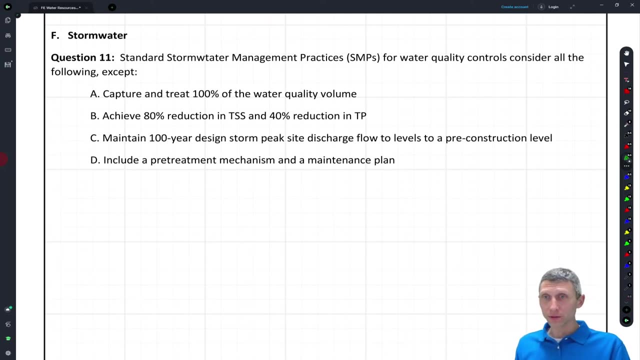 concept questions, but I think um, I personally actually saw that on the on the PE exam, So something like a concept question about eutrophic water bodies. Here's another one Um stormwater management right. Standard stormwater management practices, SMPs for water quality controls are. 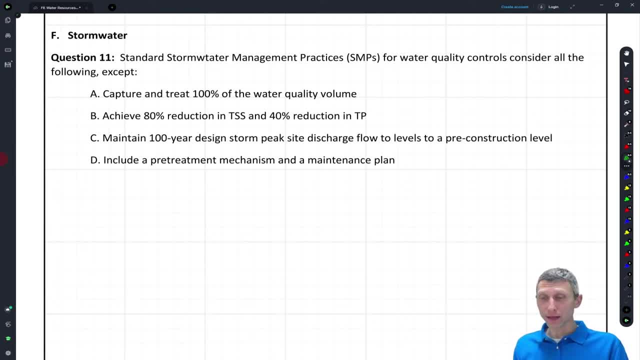 um consider all the following except right. What does it not consider here? Okay, Um capture and treat 100% of water quality volume. That's that's water quality. Okay, That's that's good. Um achieve 80% reduction in total TSS. 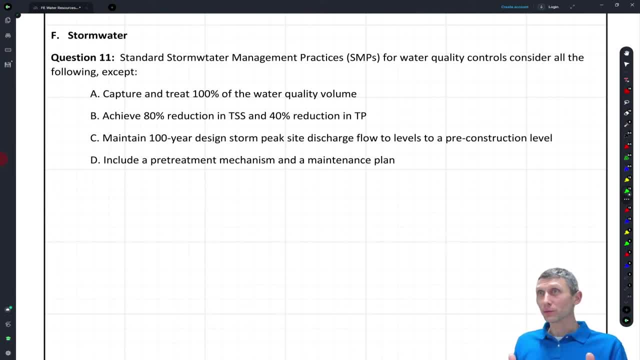 What's total total suspended solids? All right, So that works as well. Um, and then reduction in total phosphorus. Yeah, Reduction, total phosphorus is good, because, uh, that's what we're looking forward to. So, and then here's? here's another question: Maintain hundred year design storm peak. 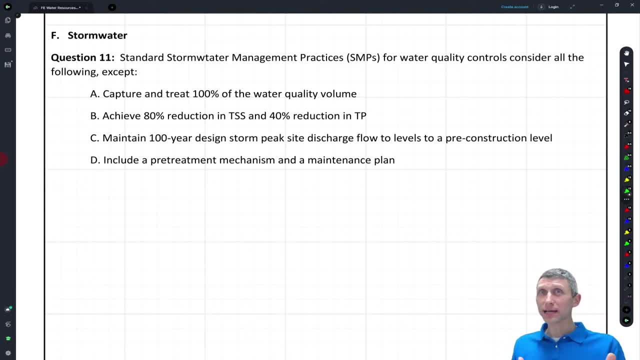 site density. So what does that mean? Um, so that's, that's, that's good. Um, so that's that's good. Discharge pre-construction levels: a hundred year design storm is not water quality Once you get. 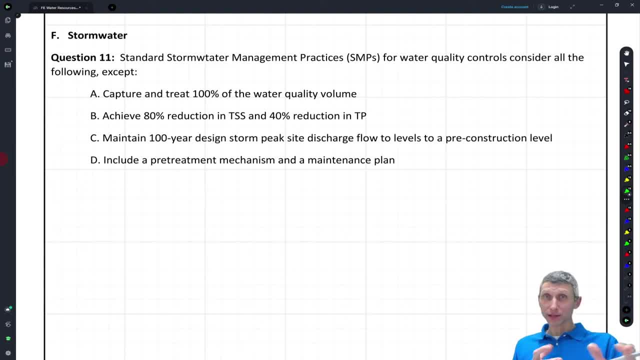 to a hundred year design storm. everything's turbid, turbidity. That's another one. a lot of sediment in the water and it's it's, it's cloudy, right, So that's another one where this becomes um water quantity, right, This is, this is a quantity control. Um, this is, this is flood. 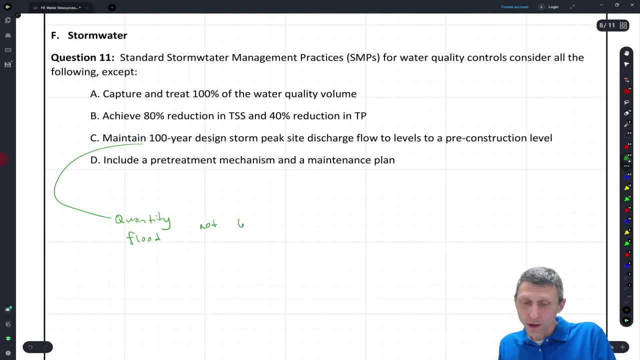 control. This is not water quality volume, That's water quantity volume. Okay, So this is quantity. Um, and that's going to be our answer, uh, for this question. pre-treatment mechanism, That's what one of the requirements for storm in the storm water management design. 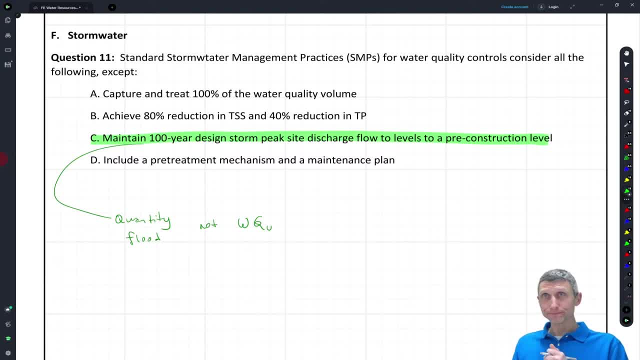 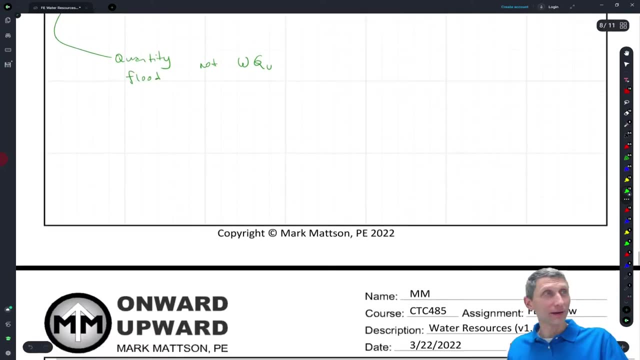 manual for water quality as well, So hopefully that helps. Garrett, just saw your question. Yes, this is the time and day I'm typically streaming these sessions, So glad to have you along. Hopefully we can keep going without any more hiccups. So, um, so, let's keep going. We've got. 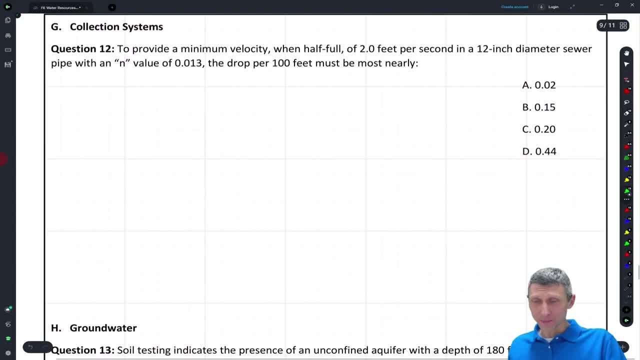 a few more questions here. Hopefully we can get through all of them. but um provide a minimum velocity when half full, two feet per second. a 12 inch diameter sewer pipe with an end value of 0.013 drop per a hundred feet must be most nearly So. this goes back to Manning's equation. So we've 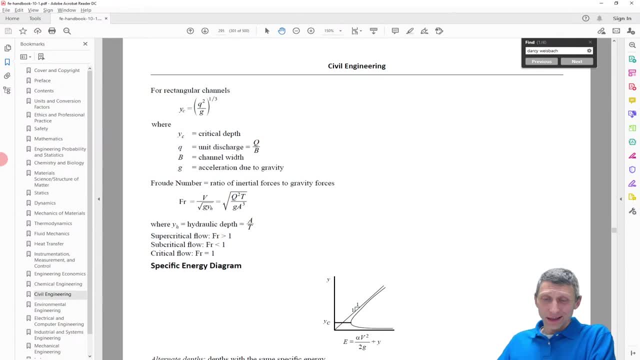 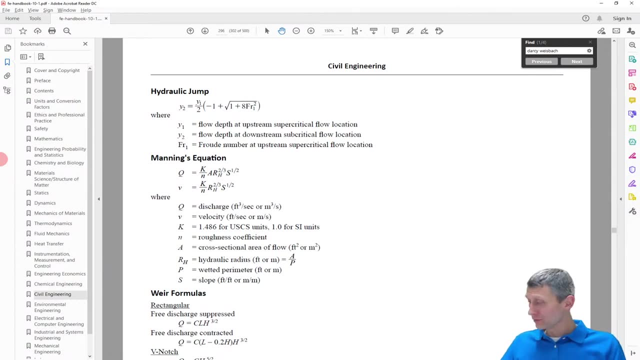 used Manning's already. Um, honestly, uh, this equation isn't isn't much different, So, but but here we're. we have velocity instead of flow. So let's write down our Manning's equation, um, and then see what we need to solve. 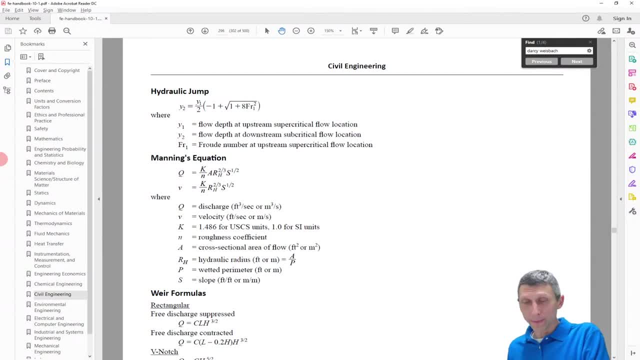 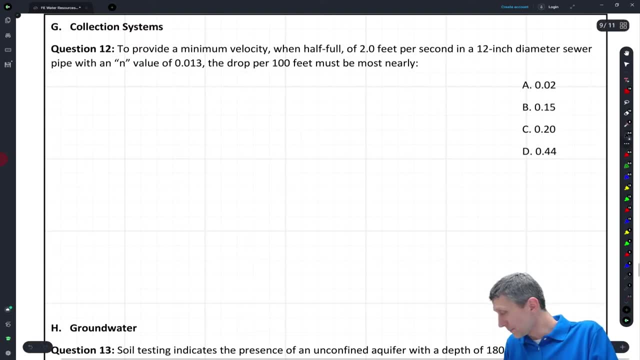 For and make sure that we can do it. Okay, Um, so what we're going to do here is is we're going to come back and we're going to say the velocity in this pipe based on Manning's, um, Manning's- sorry, let me try to write this better here- Um Manning's, um equation. 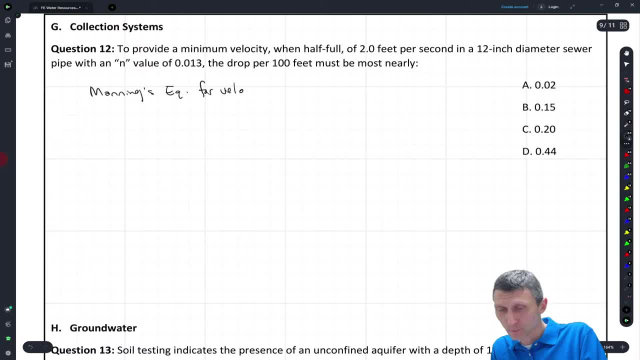 uh for velocity is going to be what um we're going to have. V equals K over N, So it's going to be V N times the hydraulic radius, uh to the two thirds, uh times the slope to the half Um. so what we're trying to solve for here is this: the drop per 100. 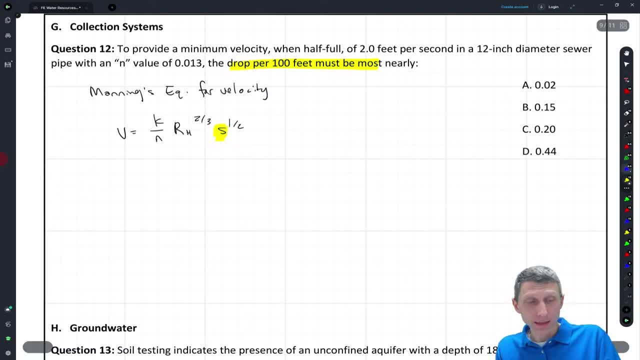 So we're trying to solve for this slope. Okay, In here we're going to. we can plug and chug um two feet per second. um equals this K value. Now that we're going to use um is. 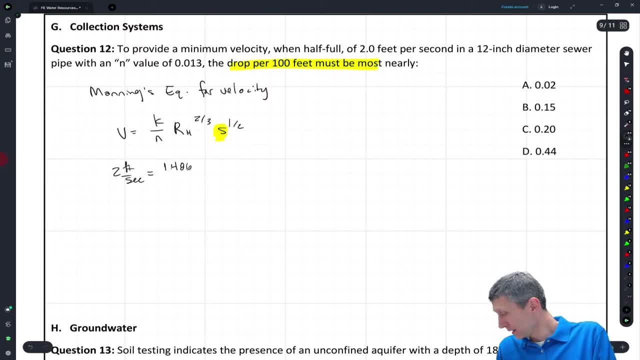 going to be 1.486 and that has a bunch of units in it, but that's what we're going to use for us. So we're going to use the estimated units um divided by our end values: 0.013, uh. 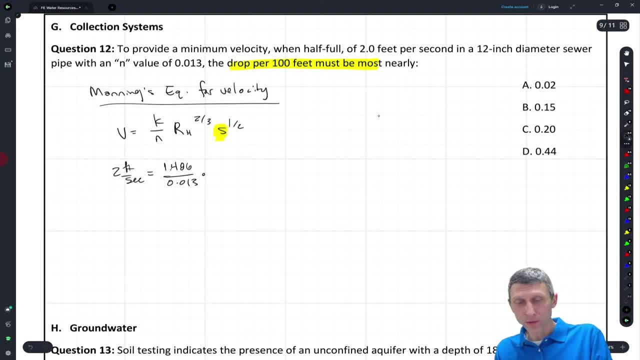 times the hydraulic radius. So what's our hydraulic radius? Well, we have a pipe that's going to be half full of water. Okay, This pipe is half full. And um, again, when we're looking at this, we're going to look at the perimeter, the area, and we'll solve this. 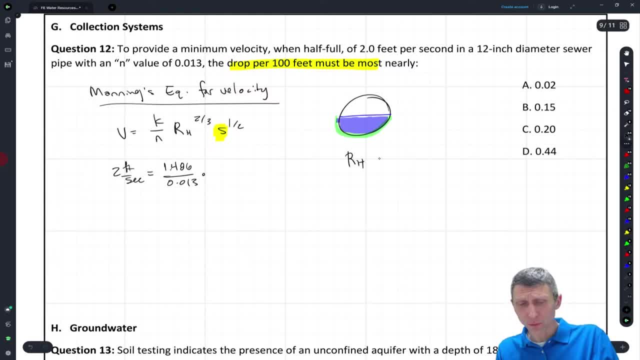 So if we look at the hydraulic radius of this thing, what are we going to get? Well, we're going to have one half. We're going to have one half of PI D squared over four. right, That's the area, but it's. 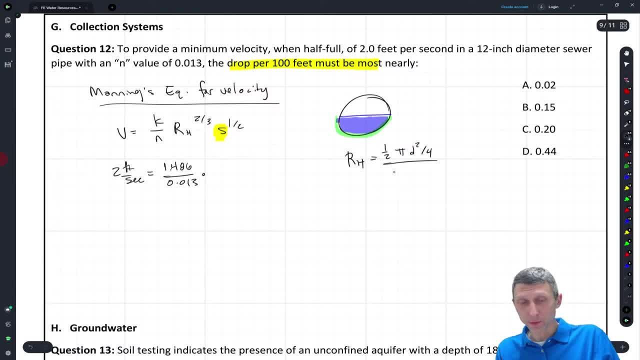 one half of it, because we only have half the pipe. Um, and then what's the perimeter? Well, the perimeter is going to be one half of what PI D, because PI D is the circumference. So we get a bunch of things that cross out. The one half crosses out, the PI's cross out. 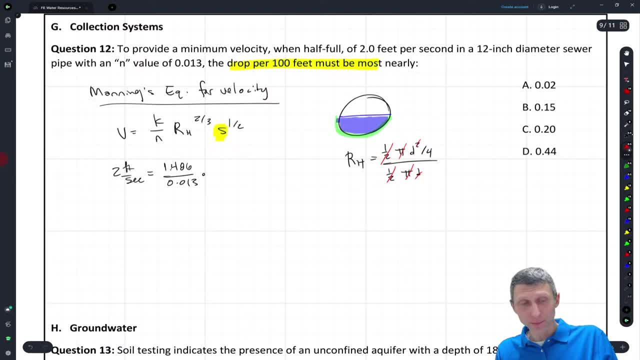 uh, the one of the D's cross out and we just end up with, essentially, D over four. So in our case, the hydraulic radius equals what we have, a 12 inch diameter pipe. Okay, And I'm going to say, um, you know, 12 inches divided by four equals three inches, which 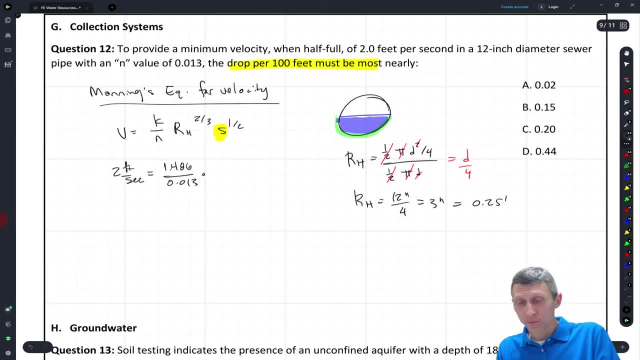 is going to equal a quarter of a foot. Okay, So then I'm going to come back in here to my hydraulic radius: one quarter of a foot to the two thirds and we get S to the one half. So once you have all that, you have to rearrange a few different things, but you're 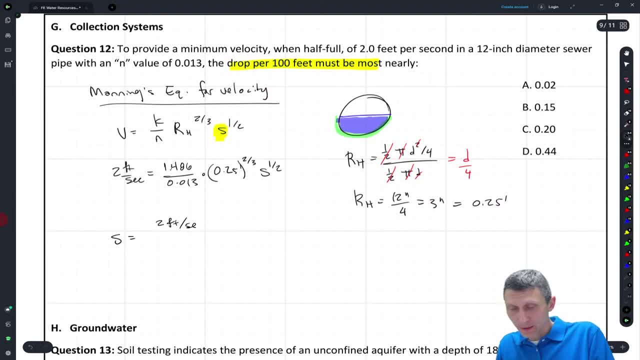 going to get? S equals what? Two feet per second. Uh, what Divided by all the rest of the pipe? Okay, Divided by all the rest of this, 1.486, uh, divided by the 0.013 times 0.25 to the two. 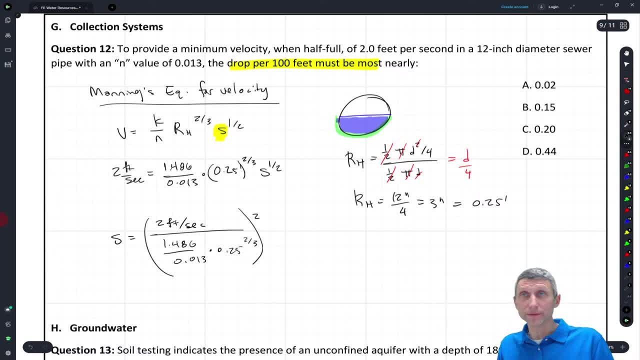 thirds, And to get rid of the square root, we have to square all of it, Okay. So when we saw that, I think the answer that I got was 0.0, uh, zero two, and the units on the slope are feet per feet. And you look at this and you say, oh shoot, none of these match. 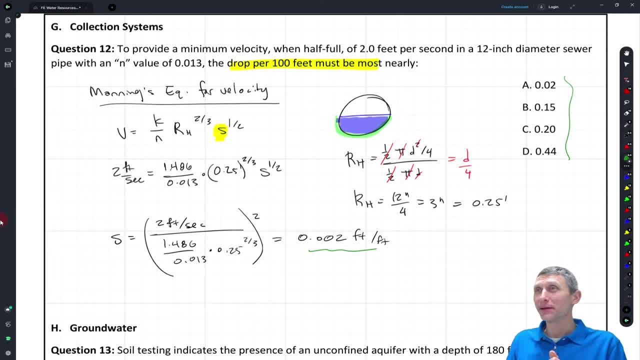 And that's when you look at me. I'd say, Madsen, to just screw something up, Um, oh man, And. and I I'd love to say that I did, but I actually didn't hear. I actually took this problem from the 10 state standard. 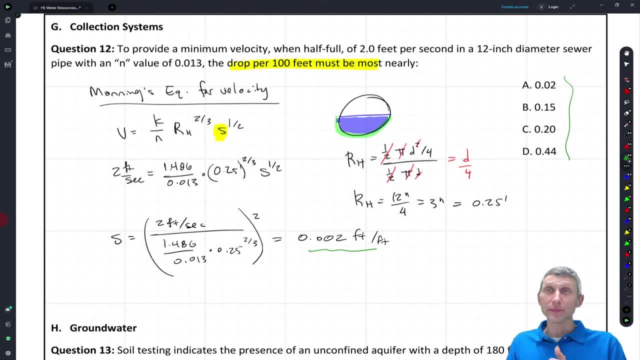 So up in the North East- kind of Midwest Northeast um, the 10 state standards are what are used for sewer design and the minimum slopes are are spelled out in the 10 state standards as I'm using, uh, the Manning's equation. They actually use full flow, but it's it's. 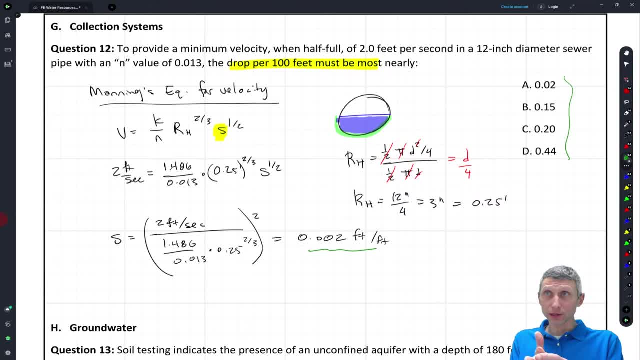 not really um any different here, but w w? w. this is looking at as many Manning's equation for two feet per second with a end value of 0.013.. So this is a foot per foot. What we want is per 100 feet, So, um, we're going to multiply. 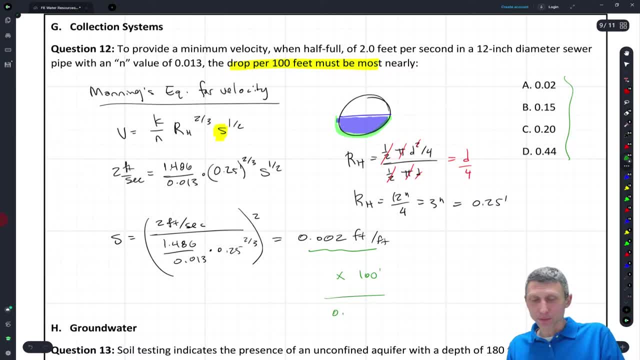 this times a hundred feet to get our answer, which is going to be 0.2 feet per. And that's going to be our answer. So, for every a hundred feet, you're going to drop 0.2, right? So 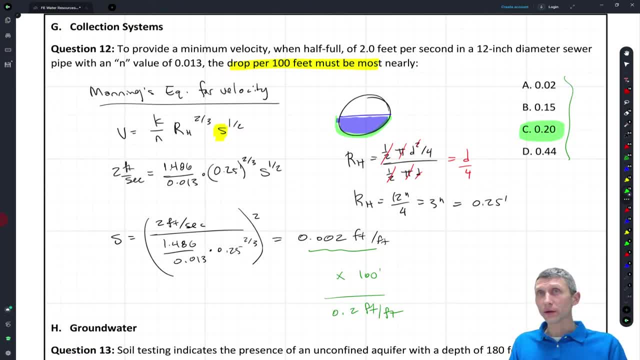 0.2 divided by a hundred is going to give us our slope of 0.002.. Okay, And so I actually, I should say 0.2.. Um feet per per um per 100 feet, I should. I should say it that way, Okay, So that's. 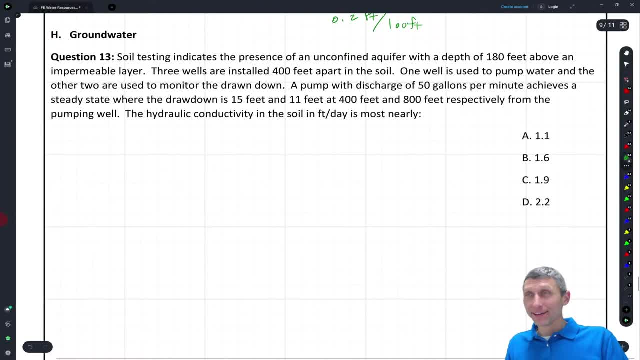 that's question 12.. Let's keep going. Um, we've got a few more here and uh, let's see how we do So. soil testing indicates presence of an unconfined aquifer with a depth of 180 feet above an. 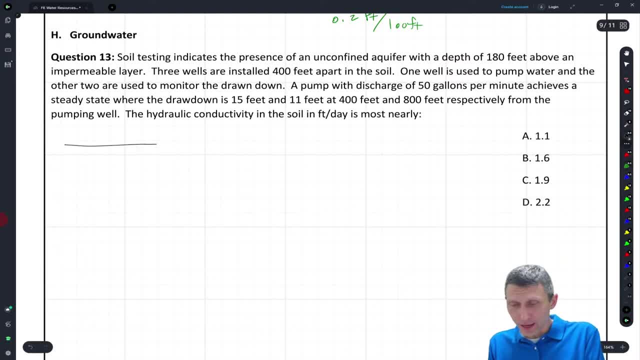 impermeable layer. So we've got some um stratum here and this is, you know, we have some groundwater table, Okay, this thing going on. so this is some groundwater table and what we're gonna do is we're gonna insert, we're gonna drill three wells into here. I chose for 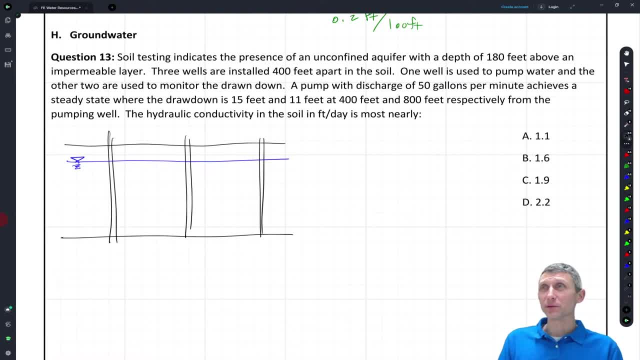 groundwater. I chose a well drawdown problem. there are. I mean, you could get into some other problems here, but basically what we're doing is I'm out of this one. well, we're gonna pump out a Q equal to what I say. I said 50 gallons. 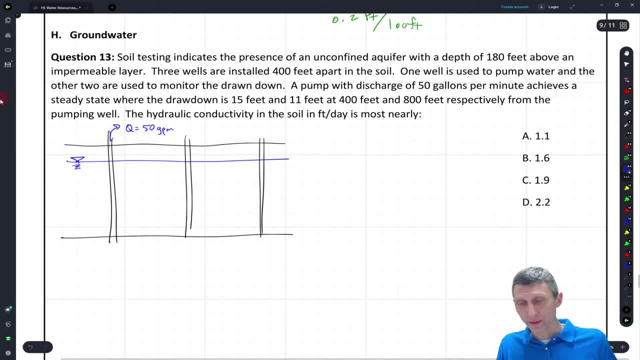 per minute, okay, so we're pumping out 50 gallons per minute and we achieve a steady state. so what we're gonna do is we're gonna start to draw down this aquifer, okay, and we're gonna draw down this aquifer, okay. so we know that this. 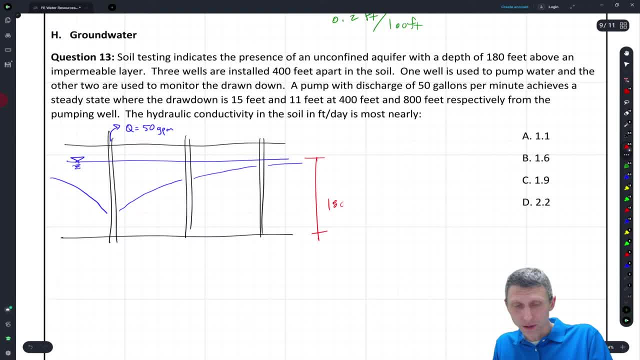 aquifer is 180 feet tall and at this point we're 15 feet down. so this is the 15 feet here and at this point we're 11 feet down and our distances are 400 feet and 800 feet from the well. okay, so you know, our water, our water, is gonna be in here and 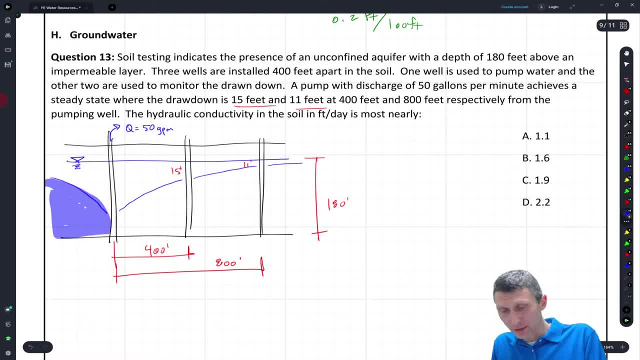 it's getting drawn down, all right. so it's getting drawn down in each of these wells. we'll see that, you know, coming down and that is going to. this is kind of gonna be our well draw down problem, right, and that's what this is kind of kind of look like there. so the question is: how do we solve this? 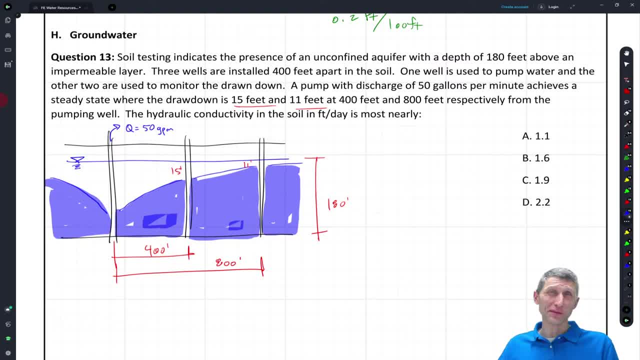 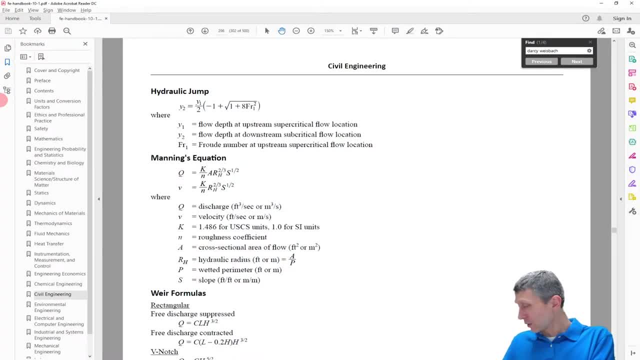 problem? um, this actually is one of those questions that hopefully will be answered in the next video. Hopefully, if you get something like this, you can read the question quickly enough, know where the equation is, quickly enough to go to find it, But our well-drawdown equation is going to be right here. 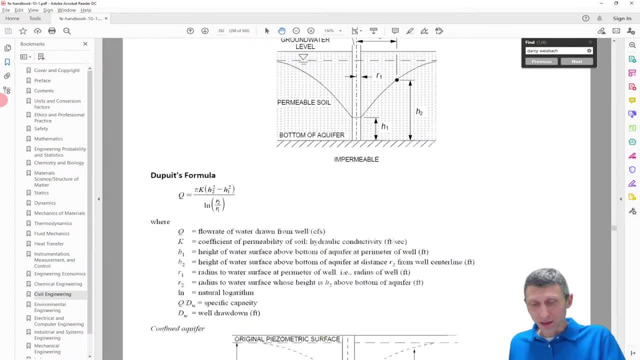 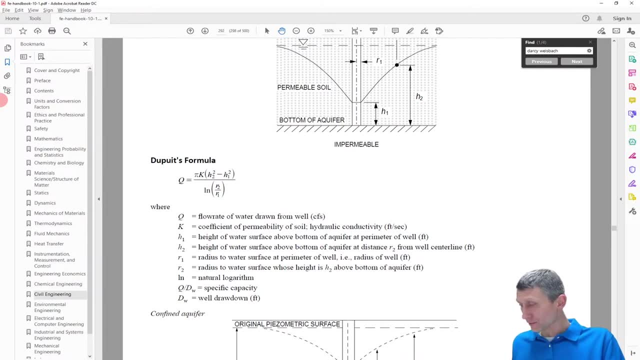 So it doesn't look exactly the same as this, but it's going to be very, very similar here, So we have an equation here that we're going to be able to use to solve this question. Okay, so let's copy this equation over: 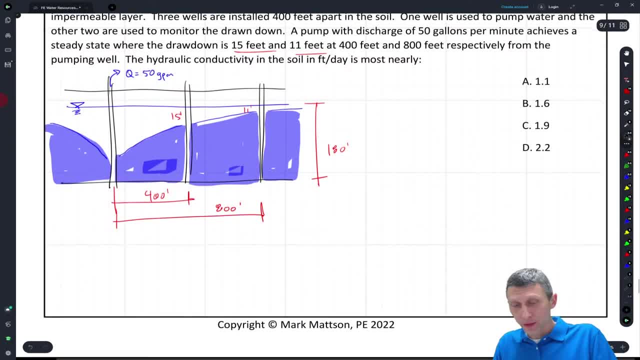 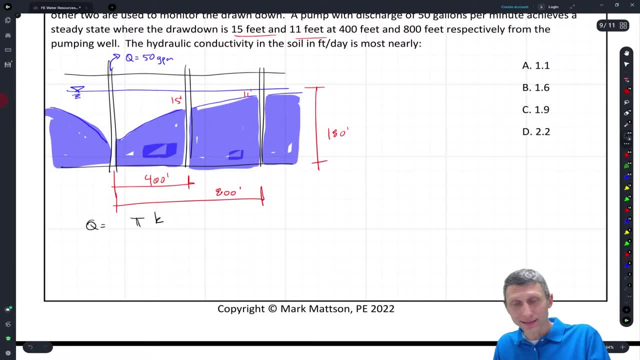 And let's go ahead and solve it. So the equation says: Q equals pi times K, So that's the K. That's the hydraulic conductivity that we're trying to solve, for Pi times K, times H2 squared minus H1 squared divided by the natural log of. 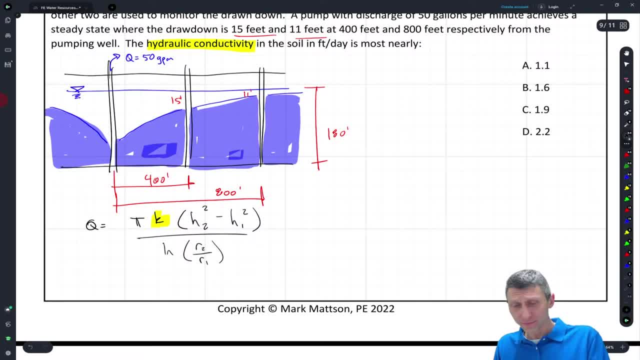 R R2 over R1.. So we have most of this right. What we have is we have- I'm just going to plug and chug over here- So 50 gallons per minute And we have to do our unit conversion here again. 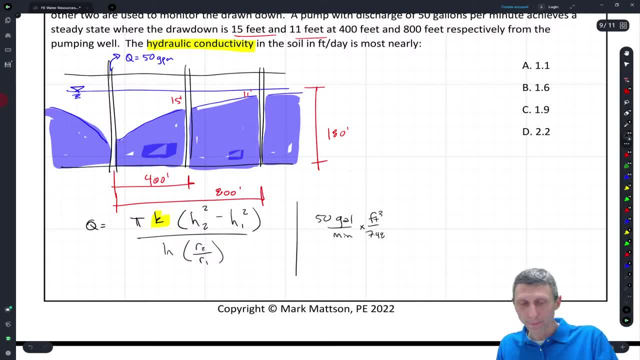 So we have to do one cubic foot per 7.48, you know, one gallons times every minute There's 60 seconds. This is going to equal pi times K Times our height, And this is where you got to be careful with the height. 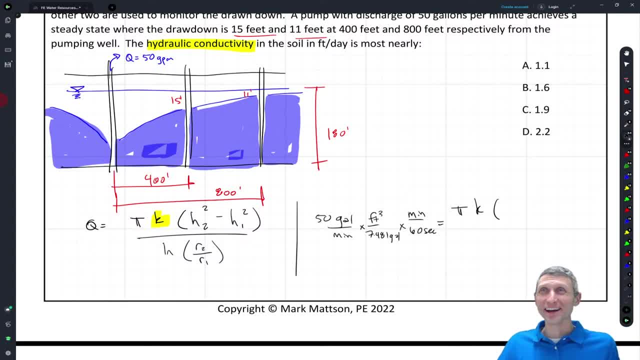 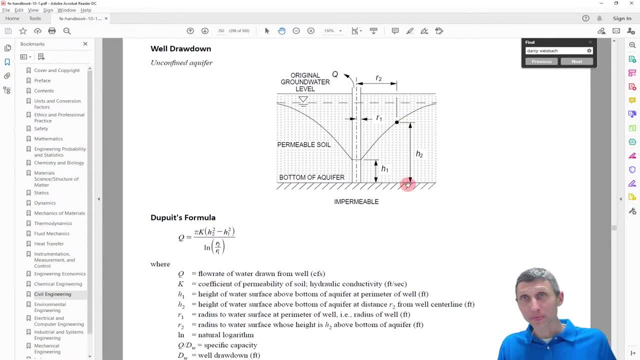 It's so easy just to plug in the wrong number and get the wrong answer. But our height? here we have to look at this. The height goes from the point to the bottom of the aquifer. Okay, so from the point to the down, we have the drawdown, which is from the point to the. 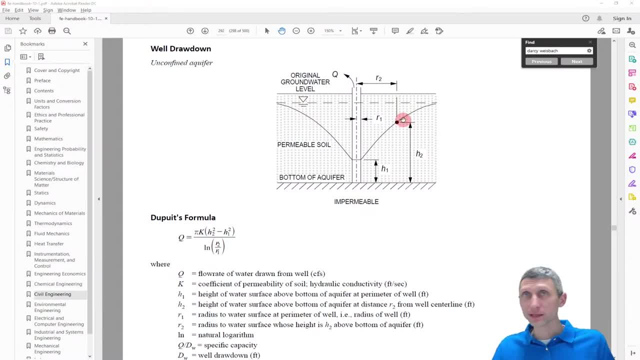 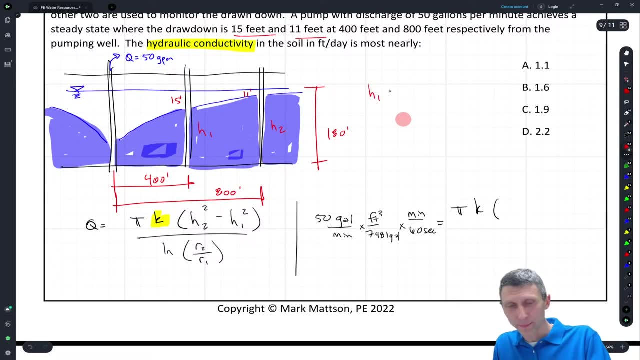 original surface, the groundwater level. So we need to find our height here And we're going to have- this is going to be like height one and this is going to be height two- But height one is going to equal this 180 feet total, minus our drawdown 15 feet, which is going to be 165 feet. 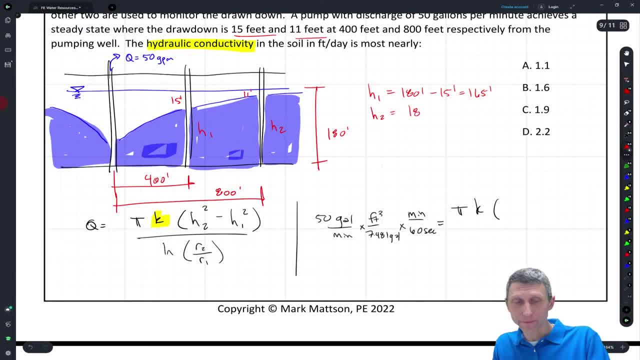 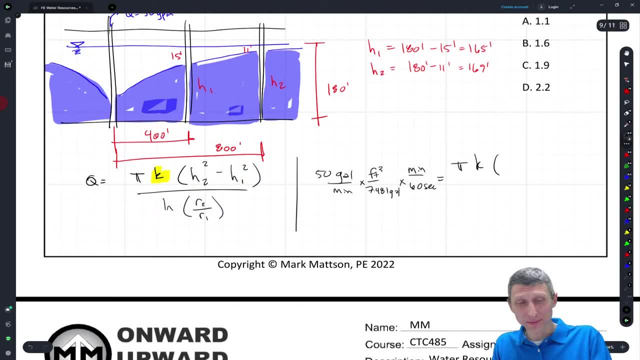 And height two is going to be our 180 feet minus 11 feet, which is going to be 169 feet. Okay, so once we have our heights again, this just becomes kind of a plug and chug thing, where it's 169 squared minus 165 squared divided by the natural log of the radius one. 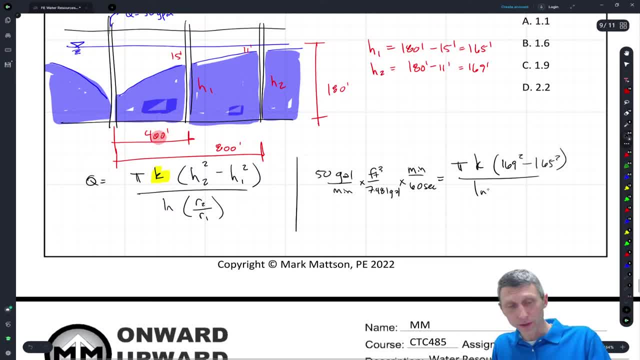 So our radius- I'm sorry, Our radius two, which is 800, divided by radius one, which is 400.. Okay, so you solve all that. You solve all that, You solve all that And hopefully you get a value that makes sense. 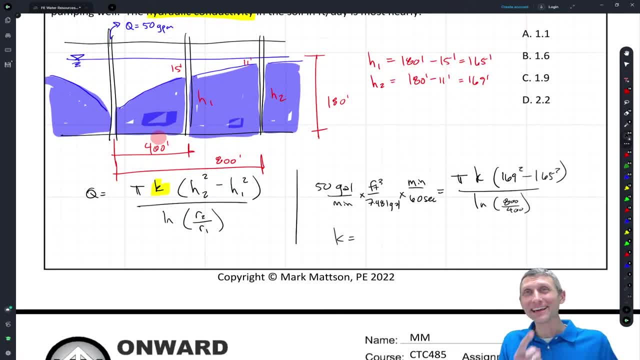 So when you solve all that, we get a value that looks nothing like our values up above right. We get a value that says k equals 0.0001.. Did I miss a zero? I think I missed a zero: 0.000184.. 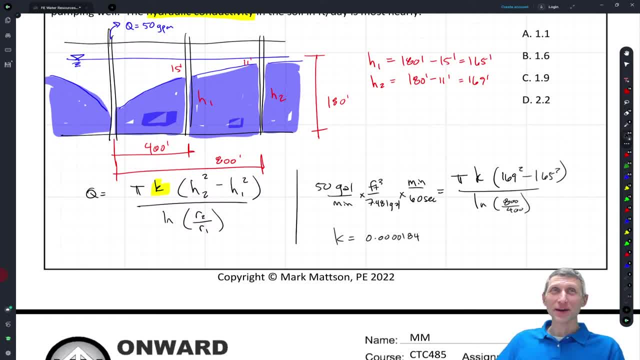 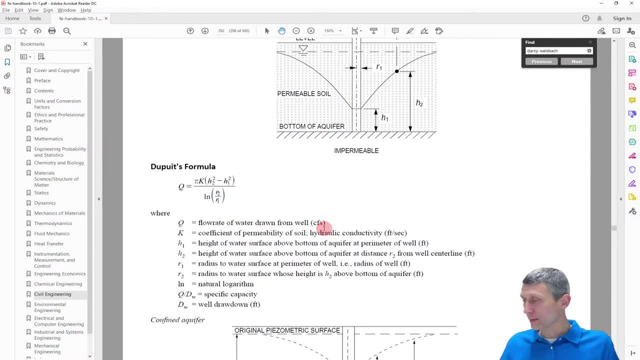 And you're wondering: what did I screw up? Hopefully I didn't miss a square this time in the calculator. But actually what you see here is when we look at this Q value. this is a flow rate in cubic feet per second. 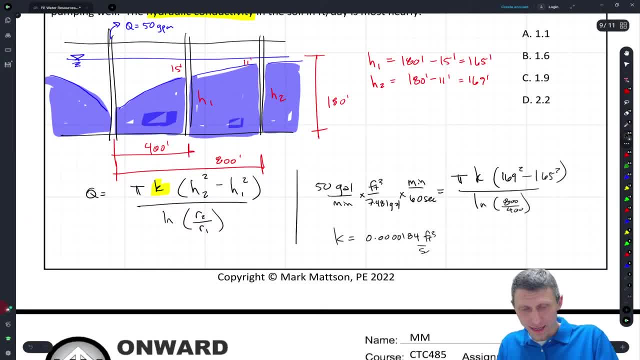 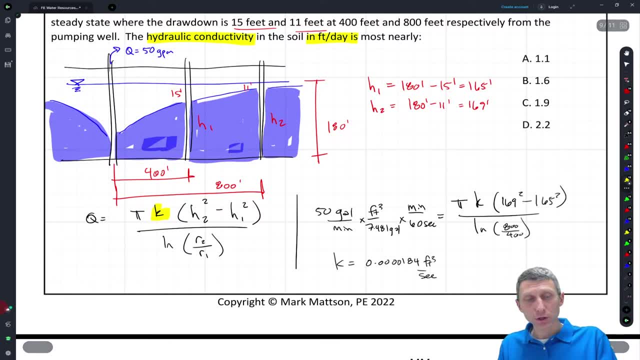 Okay, cubic feet per second. So feet cubed per second. And what does the question ask for? The question asks for feet per day. So that's what we're tasked with here is to come up with Actually hold on. 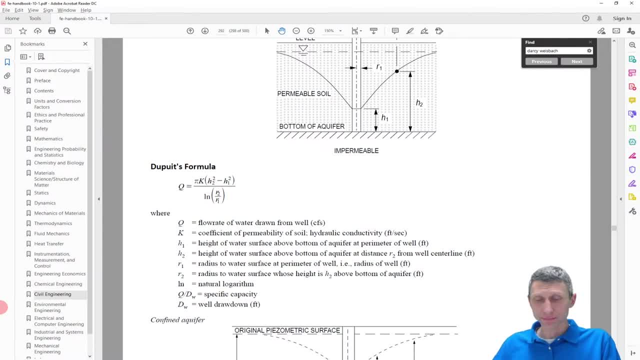 Let me just double check here. Oh right, I'm sorry. No, the K value, the Q value, is cubic feet per second. The K value is feet per second. Sorry about that. The K value is feet per second and we want feet per day. 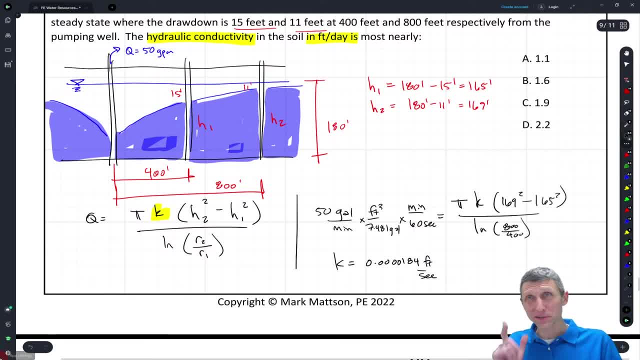 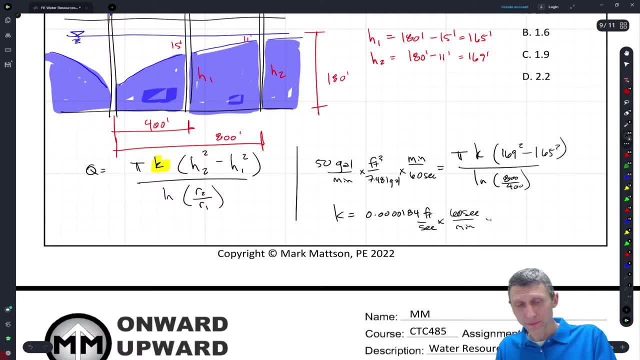 So this is feet per second. I was thinking some of the units were wrong, But this is feet per second. We want feet per day. So how do we get days? Well, there's what: 60 seconds And a minute times 60 minutes and an hour times, 24 hours in a day. 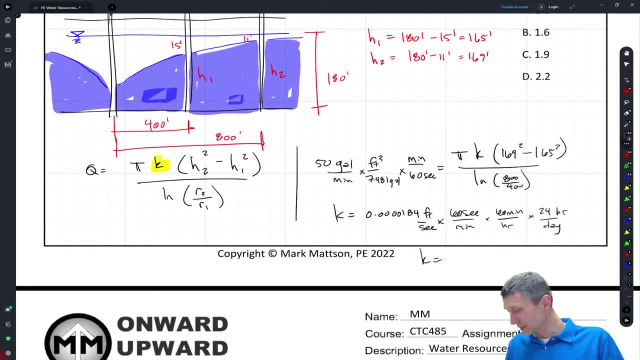 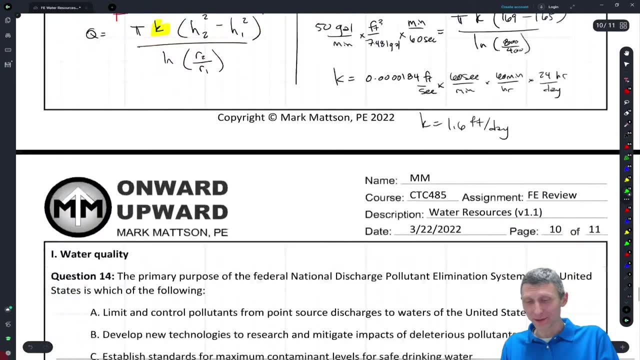 And K is going to equal. I think it works out to be roughly 1.6 feet per day, which is a typical kind of value out there too, So hopefully this works for you. All right, We got a couple more questions here. 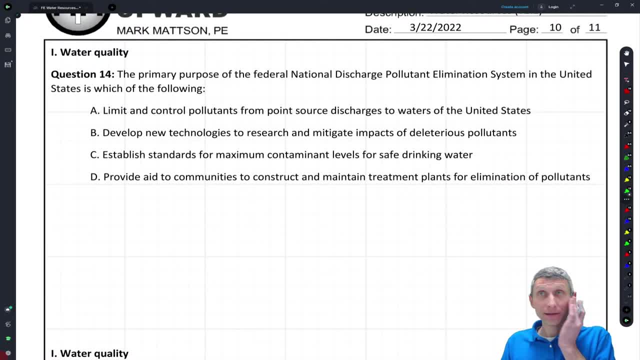 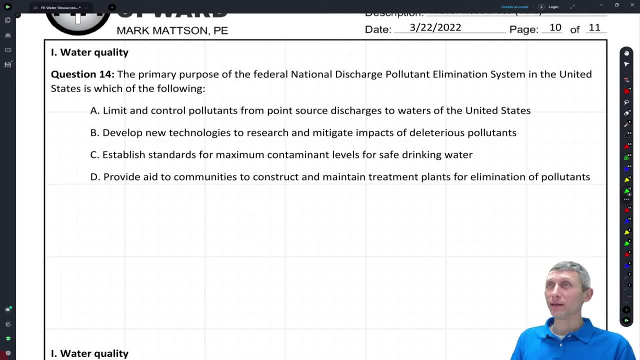 are used to filter water quality. Honestly, I knew this was going to be long anyway and I didn't get that one in there. Maybe for a future one I'll get Darcy's Law in. But primary purpose of the National Discharge Pollutant Elimination System in the United. 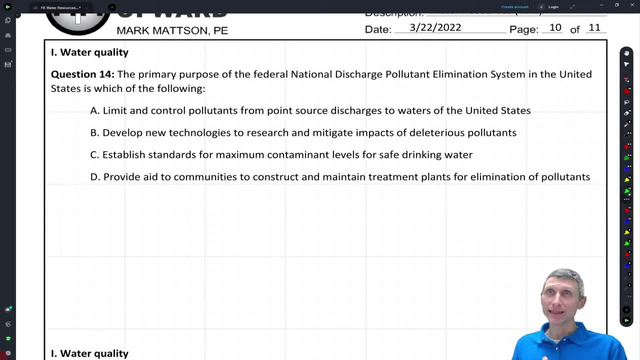 States. So, anywhere you go, you're going to be running to NPDs, Okay, And this is going to be something that you're going to have to deal with. on sites to maintain water quality volume. This is a result of the Clean Water Act. 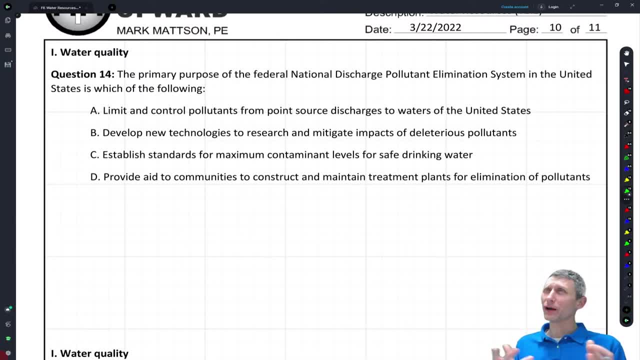 Like back in the 70s, the Ohio River lit on fire, you know, and people didn't like that. They said water shouldn't be lighting on fire And, as a result, that was sort of one of the catalysts that led to the Clean Water Act. 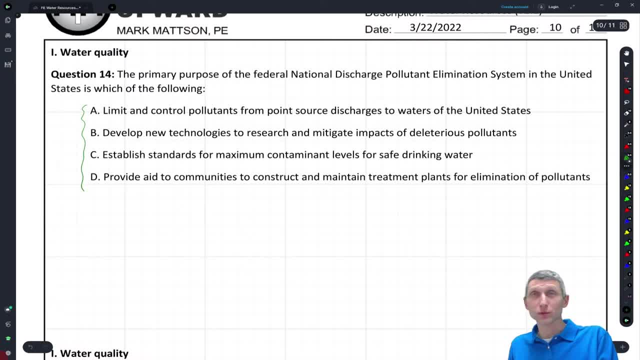 And each of these, you know each of these answers here is a result of the Clean Water Act, But specifically, NPDs is the clean water act. So NPDs is the Discharge. Pollutant Elimination System is controlling point source discharges. 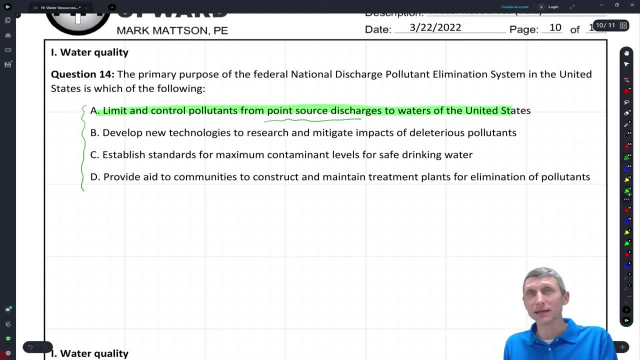 So that's what this permit does in every state. you know some states have their own system. The federal government will regulate that to states like in New York State there's a speedy system, a state Pollutant Discharge Elimination System. 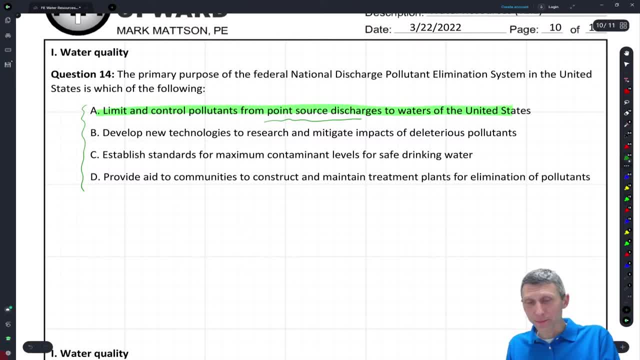 But then the other pieces of these right, the other components of these were all right. so these are all results. So the Clean Water Act, So Clean Water Act was put in place to protect water quality. You see that, even now, even with some of the lead in the drinking water, and you see you. 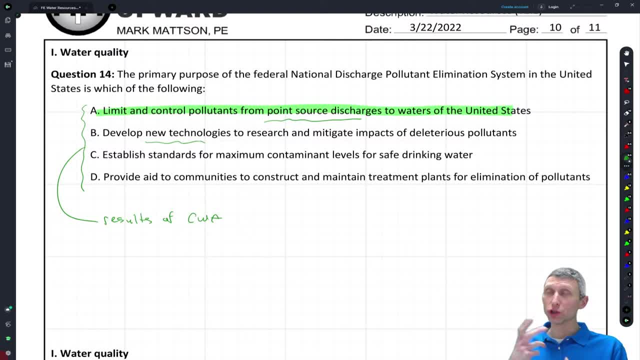 know Clean Water Act stuff going on that's looking to mitigate some of those problems, But new technologies, standards for contaminant levels, communities helping communities construct treatment plants and even now you see federal government reaching in to help communities replace water lines, especially lead tanks. 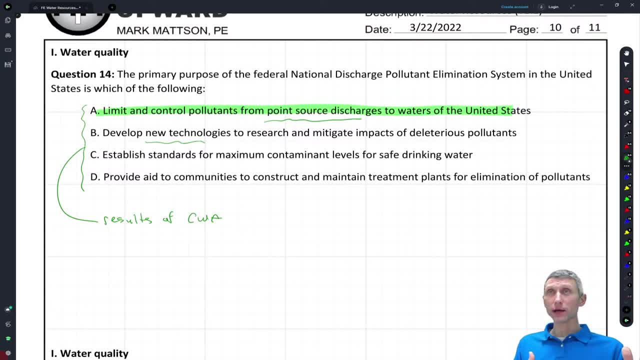 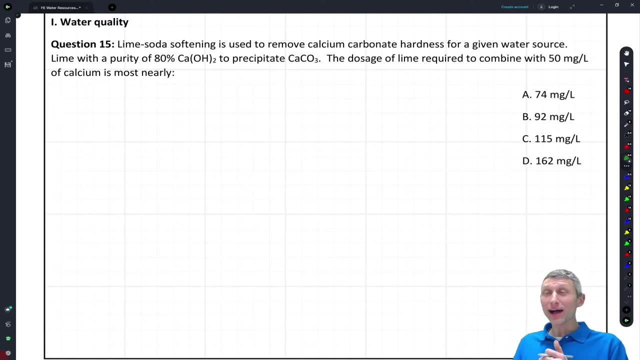 So Clean Water Act covers a lot of things for water quality, but specifically here we're looking to control pollutants from point source discharges for the NPD system. Okay, So let's keep going, and this gets into basic chemistry. So honestly, I'm surprised a little bit that the Civil FE doesn't have a chemistry section. 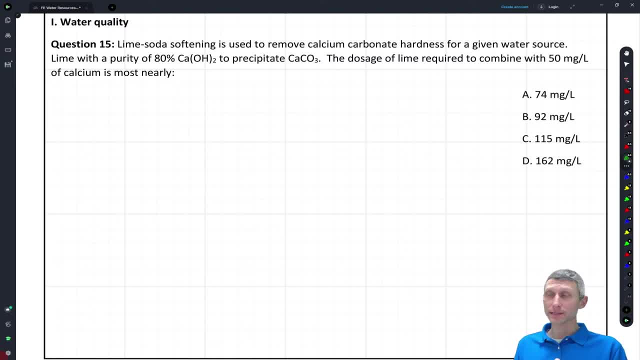 Every civil program needs a chemistry class. you take a chemistry class and this is kind of where I think it'll show up is when you get to kind of water quality. So what we have here is some kind of basic stoichiometry and honestly, stoichiometry is 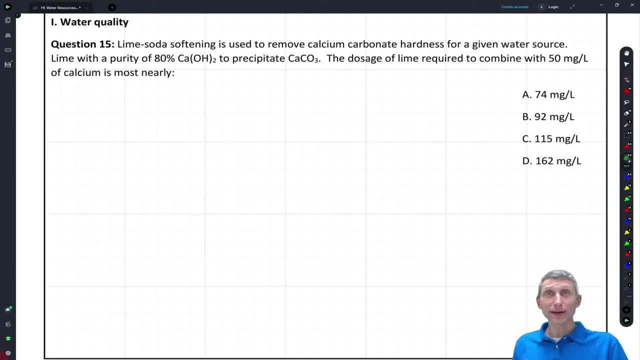 not at the top of my list for things that I'm super an expert on, So if I screw something up, put something in the comments, let me know. But what we have here is lime soda. softening is used to remove calcium carbonate hardness. 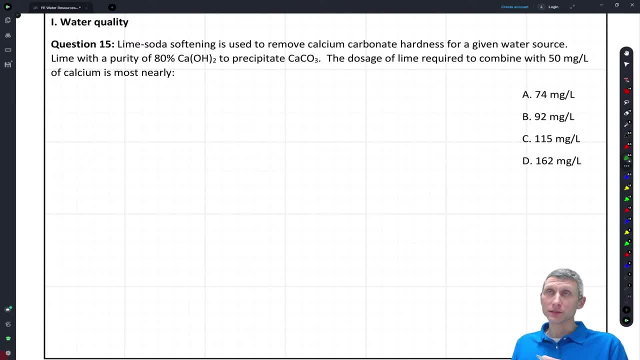 for a given water source. So there's a lot of calcium in this water and you add a whole bunch of lime to it to precipitate calcium carbonate right. So the dosage of lime required- You can find 50 milligrams of calcium- is most nearly. 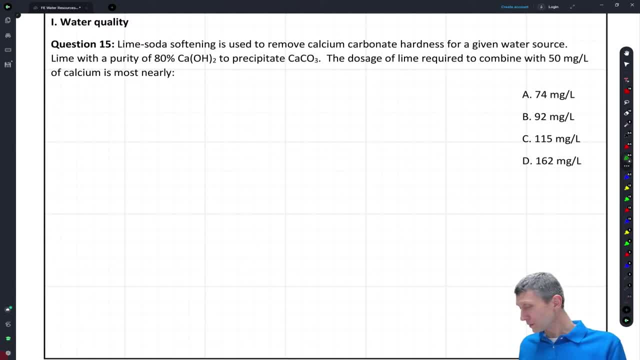 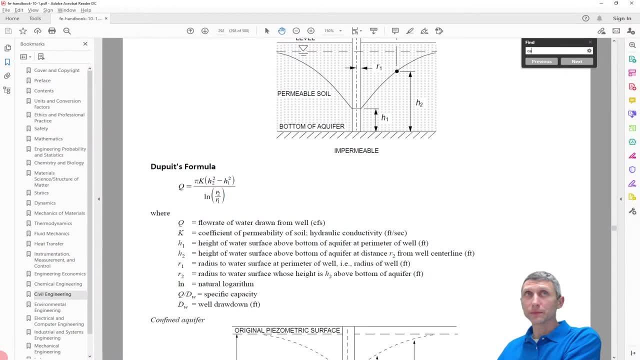 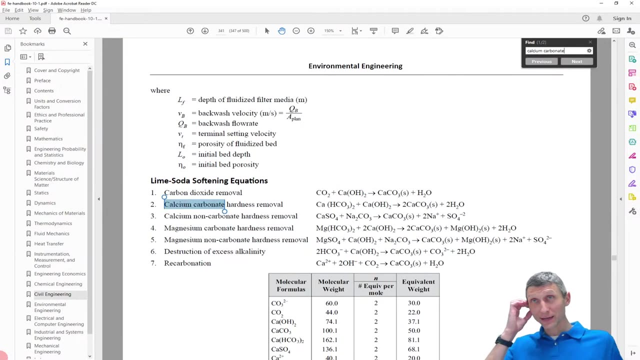 So this goes into stoichiometry and if you remember stoichiometry, what we have to do is we have to look at the reaction and figure out what to do. So you might be like me and wondering: like, what's calcium carbonate? So calcium carbonate, if I look at that, I find something and I search it and magically, 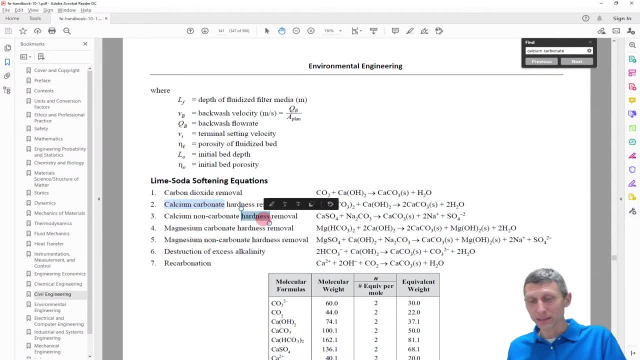 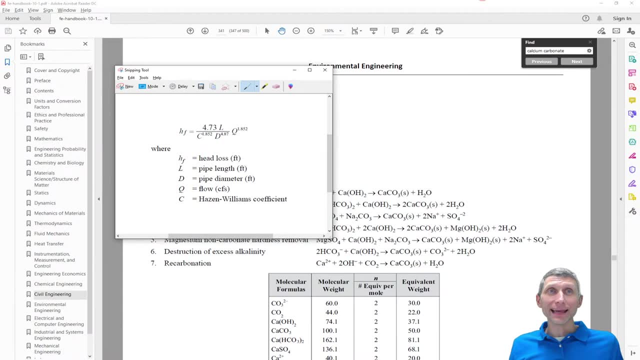 something pops up. So I think, when you get into some of this like basic chemistry stuff, some of the equations are already in Right Reference handbook, right? So we already have this equation and that's going to be a good thing because, honestly, 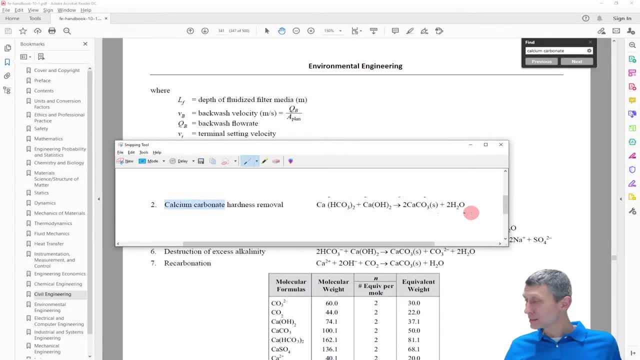 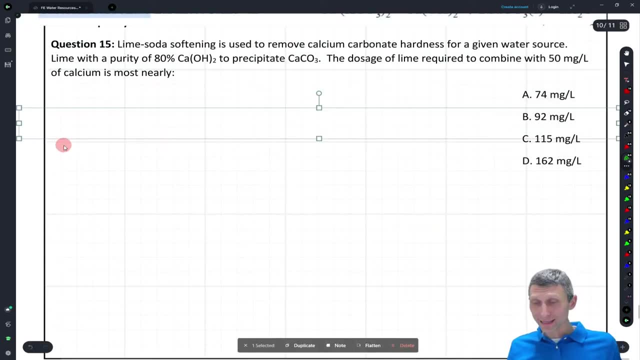 I probably wouldn't remember this otherwise. okay, But this is the equation that we're going to use, and then we have to basically use some stoichiometry to get, you know, go from one thing to the other. okay, So if I bring this over here, basically what we have is we have 50 milligrams per liter. 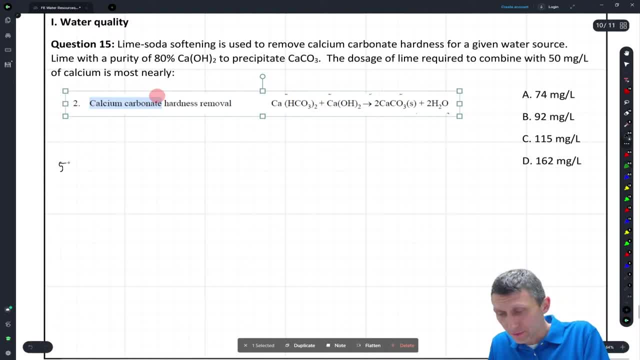 of calcium. So let's just start there, Okay. So what we have is 50 milligrams per liter of calcium. So calcium is just, you know, the calcium ion, and what we're going to do here is calcium, And what we want to do is we want to use stoichiometry to go from this right to essentially. we 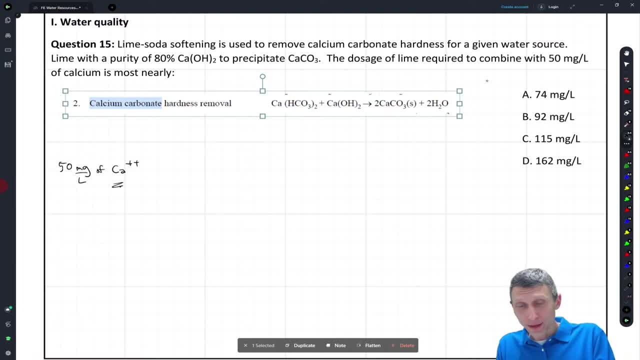 want to get to how much lime we need to add to this. So lime, this is what we're going to do. is we're looking for lime? How much? Oops, that didn't work. Let me come back here for a second. 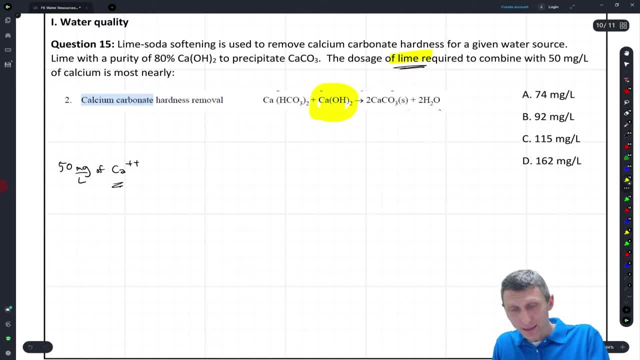 How much lime do we want to add to this thing? And this is our lime. So we want to go from calcium all the way over to lime. How do we do that? Well, anytime we get into stoichiometry, we first have to take this and multiply it by. 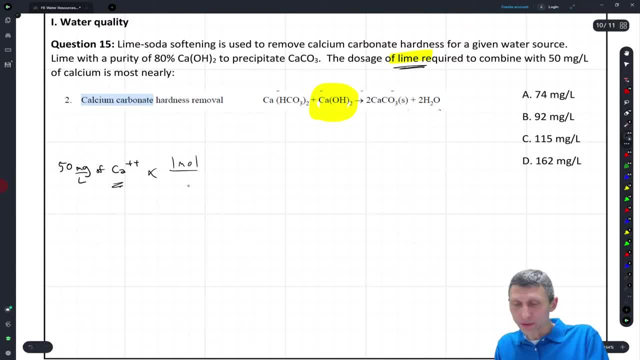 essentially, you know we want one mole of this is equal to what's our molecular weight of our calcium, right? So our calcium has a molecular weight here, Okay, So if we look into our reference handbook, what we see here is we have some basics, right? 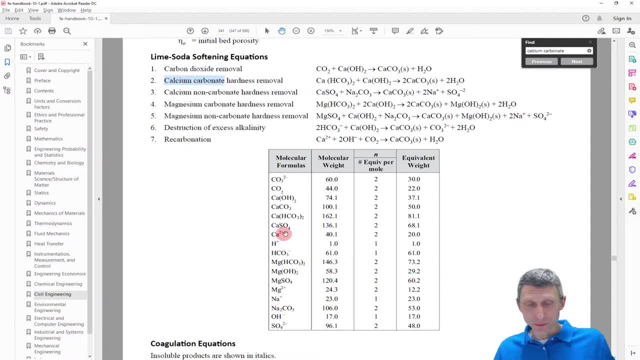 So we have some basics like calcium 2 plus right is 40.1, molecular weight of 40.1 per mole. Okay, So I can come back now and I can say: well, that's going to be 40.1 grams. 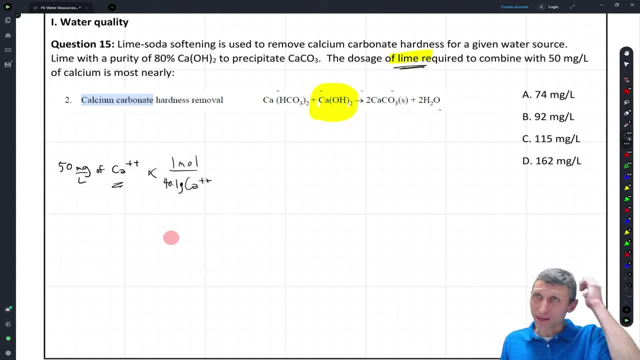 And don't worry that milligrams and grams don't cancel out, because we'll get back there in a minute, But so we know that we have one mole, is this? So we're starting some conversions? Okay, And actually one mole of: let me keep the calcium. let me keep the calcium here as well. 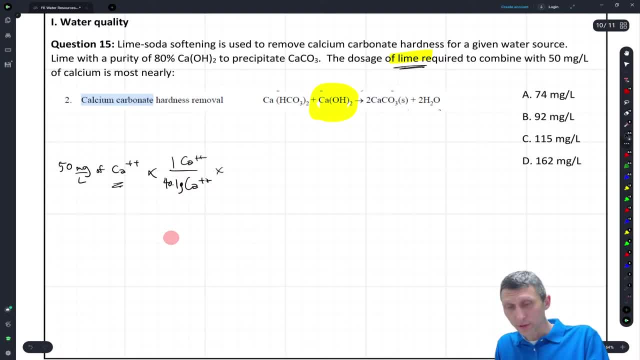 So we have, one mole of calcium is 40.1 grams. So now what are we doing? Well, we're saying, for every mole here of calcium that starts right, we need to add one mole of calcium hydroxide. So what we're really doing is we're saying, well, for every one mole of calcium, we're 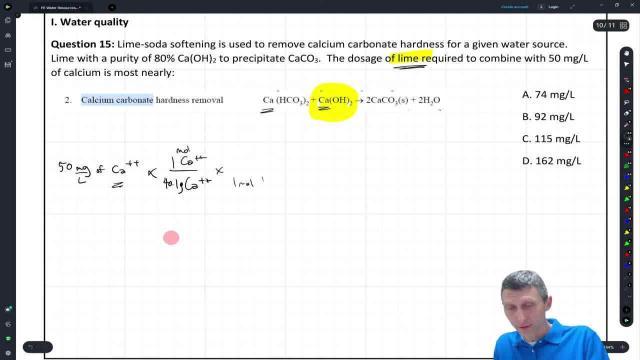 going to have one mole of calcium. We're going to have one mole of calcium. what's this? hydrocarbonate calcium C-A-H-C-O-3-2.. Actually, let me put that on the top right. So for every one mole that we start with, we really have one mole of this hydrocarbonate. 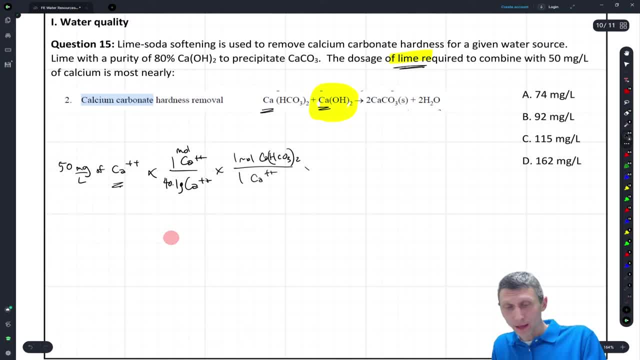 for every one mole of our calcium, And then we're going to multiply this. Well, what we really want, though, is our calcium, All right, Our hydrocarbonate? Okay, So we have our hydrated lime here, So we're going to say, for every one mole of our calcium hydroxide, we have one mole of. 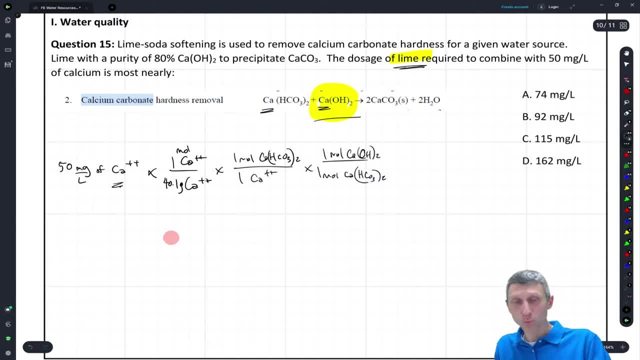 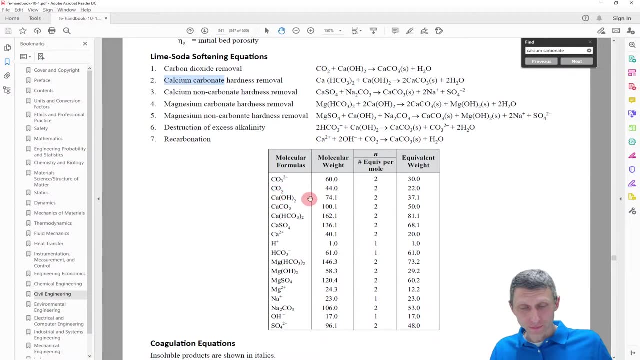 our lime, And then we need to keep going. So now we have: one mole of our lime is equal to what? Well, again we have to come back here and we have to say: the one mole of the calcium hydroxide is 74.1 molecular weight. 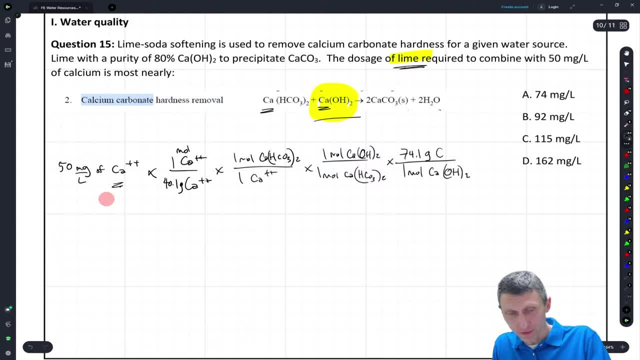 So this is a 74.1 grams for the calcium. I'm sorry for the lime. Okay, Big, long stoichiometric equation, but the cool thing is, everything starts to cancel out. So the calcium goes away, the calcium goes away, the calcium or the calcium hydrocarbonate. 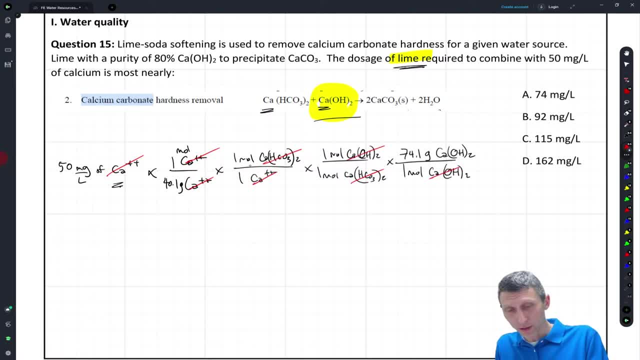 goes away, This lime goes away And we're left with, you know, all our moles here Go away And we're left with essentially even our grams go away. So we're left with an answer here. When we do all this out, we're going to do essentially, it's just, it just works out. 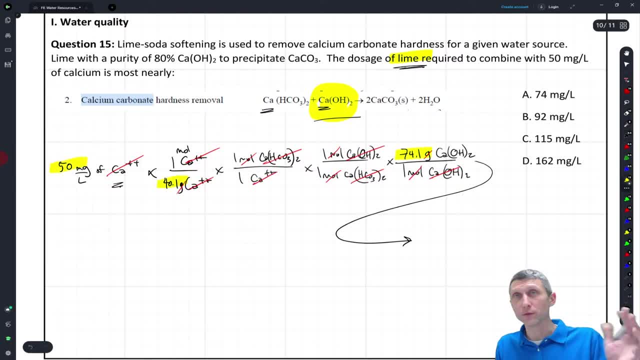 to be essentially like what: 50 divided by 40.1 times 74.1.. Okay, So if that makes some sense, we get 50 times, you know, 74.1 divided by 40.1,. we need an. 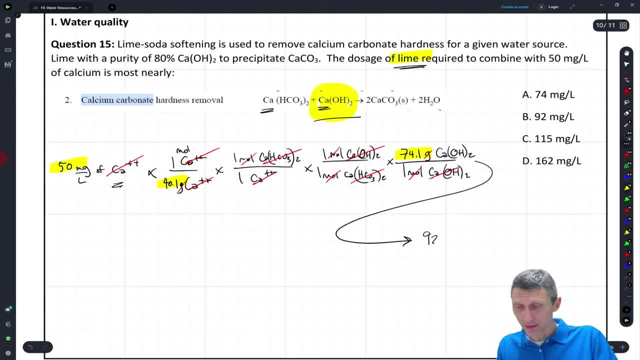 answer of like 92.4.. Okay, So that's the answer. All right, So the answer is 94 milligrams per liter of the lime. But don't pick this answer. And the reason is is because you have to read the question. 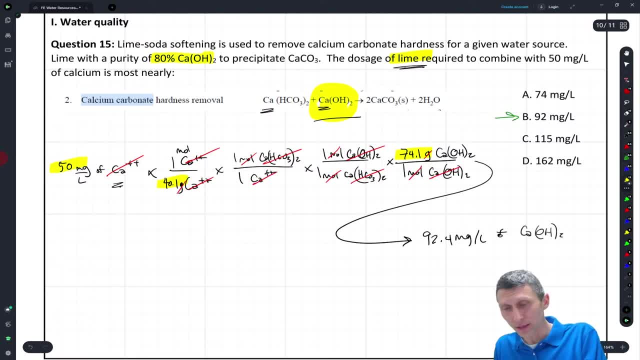 Here we have. here we have 80% purity. So the lime is only 80% pure. So the lime is only 80% pure. let's take the 92.4 milligrams per liter divided by our 80%. Okay, 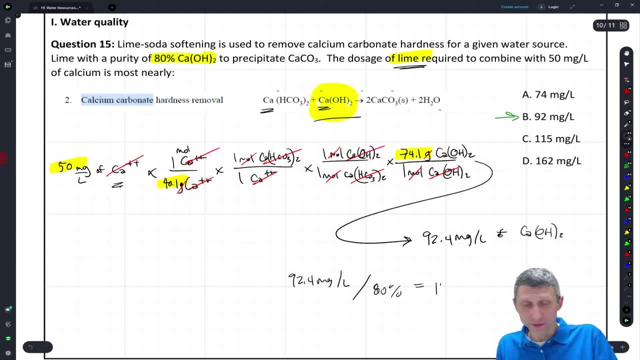 And we're going to get one other value here. That's going to be about 115.5, roughly milligrams per liter of the lime, And that is our final answer for that one. Okay, So again, the stoichiometry. if you don't remember it, go back. and there's a couple. 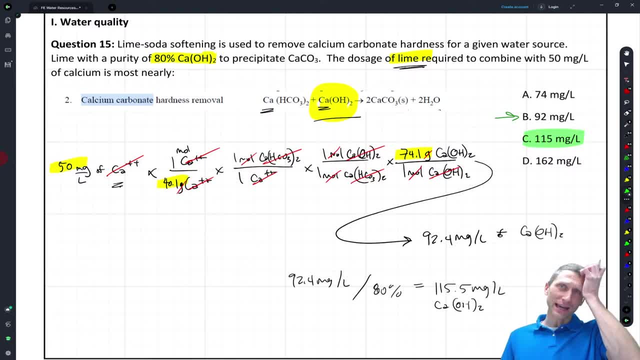 good videos. probably that can explain it better than me on the chemistry side of this. But hopefully some of this this stuff is is coming back to you or you remember a little bit from that chemistry class And if you have some, you know, maybe some ratios here where you don't have a one-to-one. 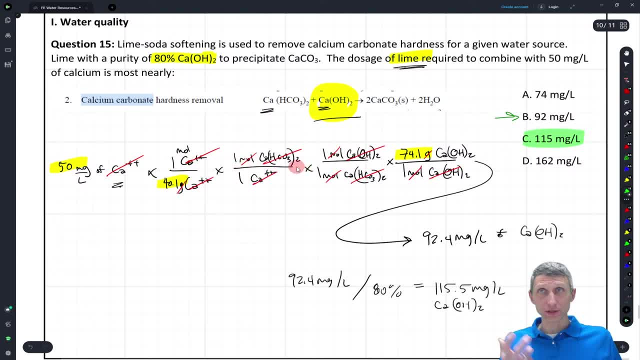 molar ratio of these things. you can, you know, use your conversions to do them a little bit more easily, But I haven't talked to a few people that have taken the exam recently. Water softening, water hardness, these types of things did show up on the exam. 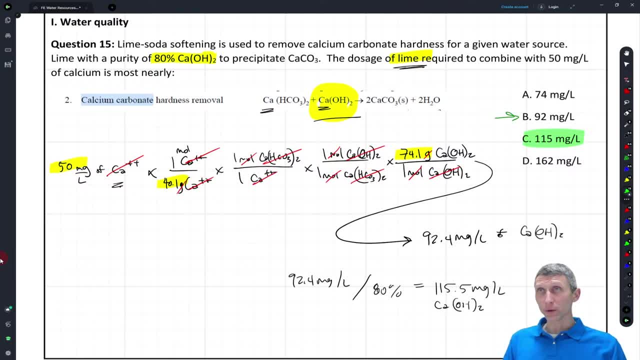 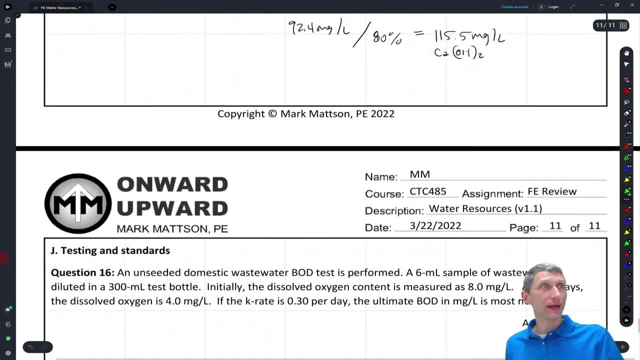 I don't know the specifics of the questions, but those topics were there So I wanted to get them in there and specifically in this section. Okay, And then two questions left and we will send this one. send this one and be done. 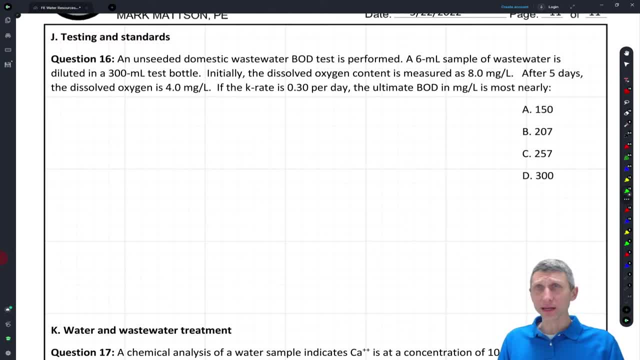 So where do we go today? So so what we have here is BOD. Again, talking to people that have taken the exam recently, they, you know not specifics, but BOD was one of those things that showed up. So so here we have an unseated domestic wastewater. BOD test is performed. 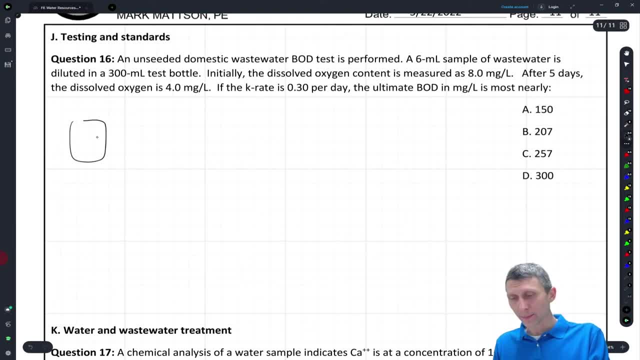 So what do you do? You take a 300 milliliter bottle right And you add a small sample of you know your bad stuff, Your wastewater. you fill the rest of the, you know. you fill the rest of this with clean. 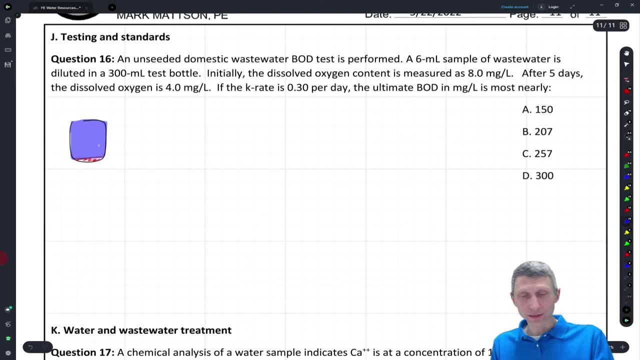 water, You know. so you dilute it and then you start taking some measurements, right. So you start taking some measurements and you know you get some readings here. So what are you reading? You're reading the dissolved oxygen content, Okay. 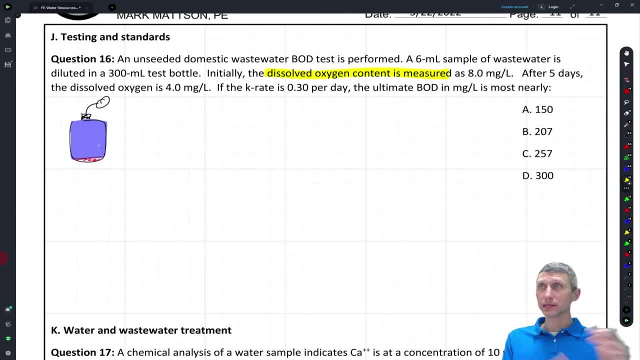 So this is kind of your BOD test. You set it up, you let it sit for five days, you measure it again and you get a second reading. And what we're asking here is: well, what's the ultimate BOD? 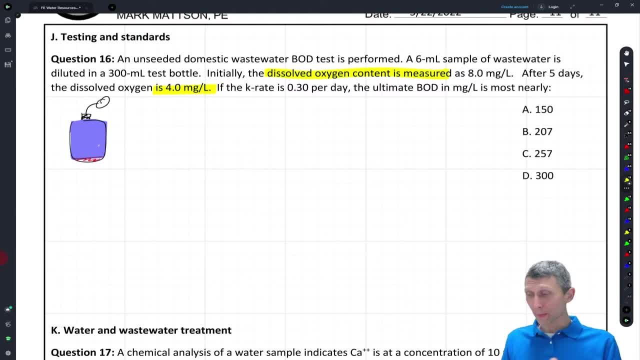 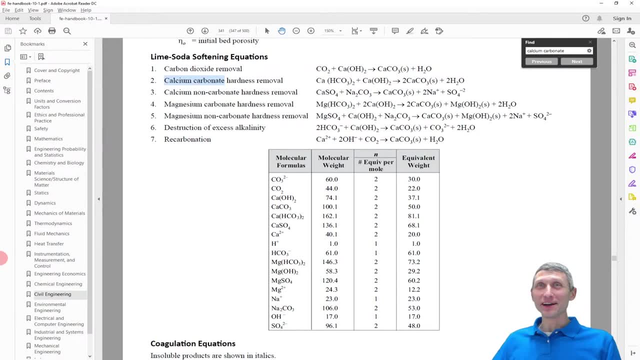 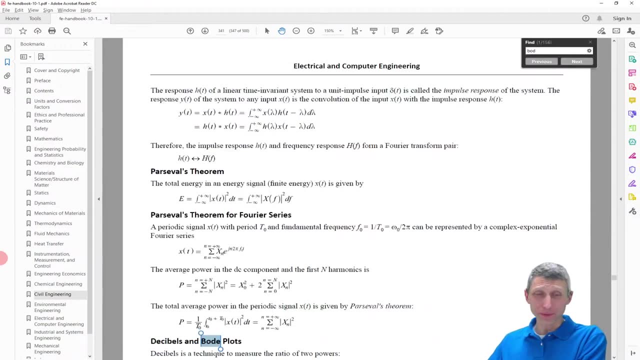 What's the kind of the, the ultimate BOD in this sample. So maybe, again, you don't really remember your environmental class too well, and that's okay, I don't either. I'm just being 100% honest with you. So, but the thing is, some of these basic concepts, you know, can you just look up BOD. 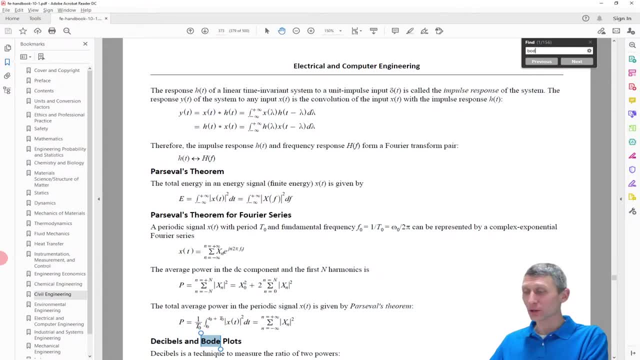 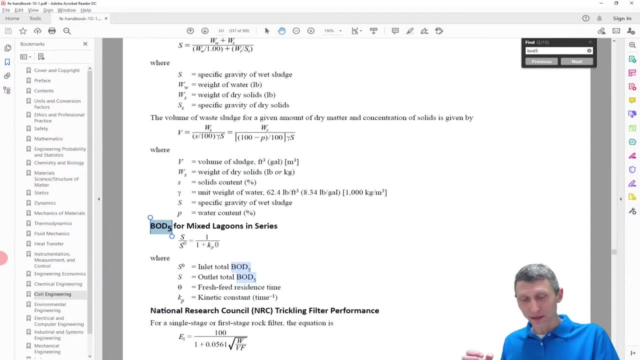 Maybe, but man, there's 156.. So BOD five, does that ring a bell? Oh man, look at that Beauty. So BOD five does start to show a couple of things in here, which is good. So that puts us into the environmental section, which is good. 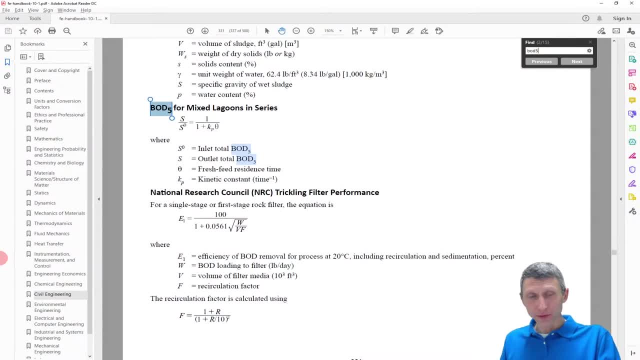 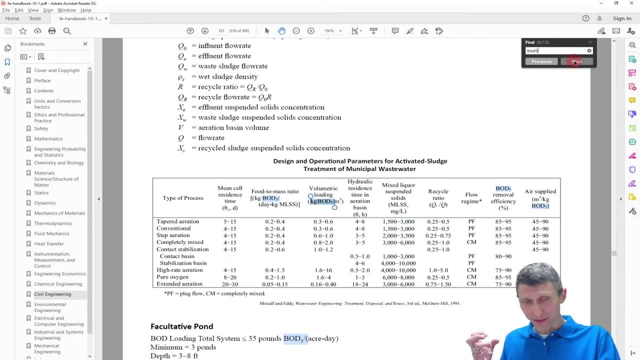 Okay, We don't want to mix the lagoon, We're not doing lagoon design here, but it puts us in the right section. So maybe you don't remember what BOD is. BOD is kind of a measure of biochemical oxygen. 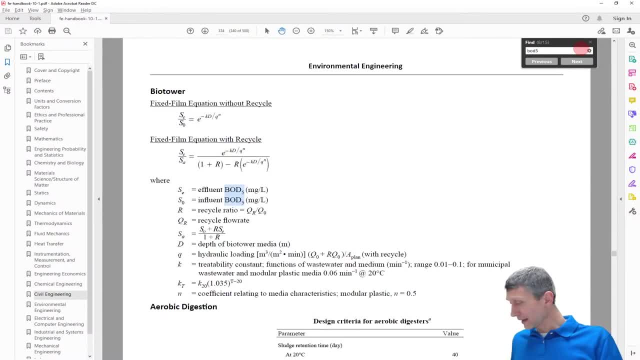 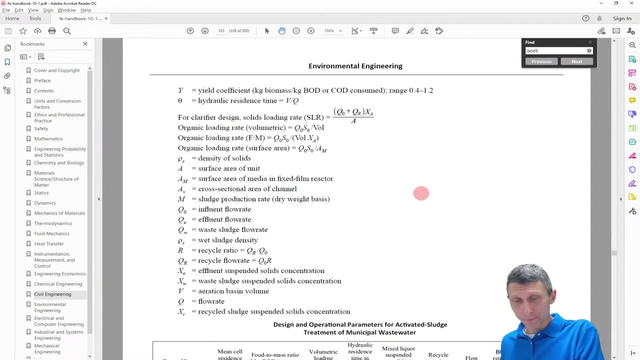 demand: Right, And this is where I wrote down where we need to go here. So I think I went by it already. So let me come back here and let me see where we are. There we go. So the BOD test solution and seeding procedures. 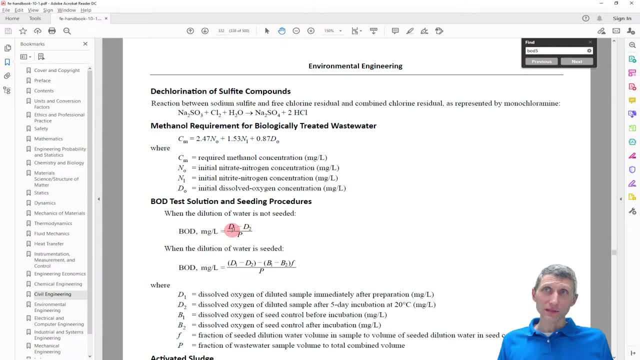 So here we have a BOD and milligrams per liter. We have dissolved oxygen. one dissolved oxygen, two divided by P, which is the fraction of the wastewater sample. Okay. So if environmental is not your first language, that's okay, But you do if you, if you know some of these basics, it will help you on the exam to get. 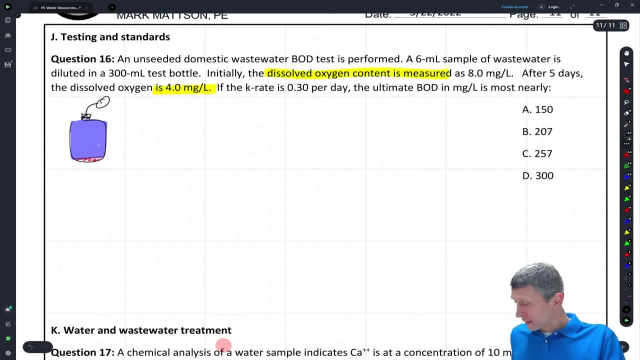 some of those points Right That maybe otherwise wouldn't get. So let's first start with this right. We have the BOD and specifically we're going to do BOD. five here is going to equal D one minus D two over P. So what's this? 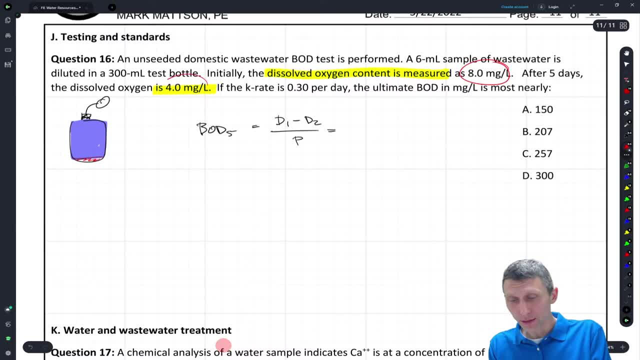 It's the dissolved oxygen you know at. you know one and at the time that we're looking. So what we have here is dissolved oxygen, eight milligrams per liter minus our four milligrams per liter divided by P, and P is the that fraction. 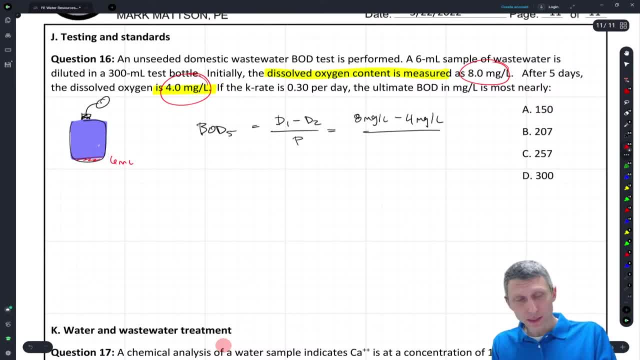 Right, So in this one we have six milliliters of the wastewater. We have, you know, 300 millimeters or a milliliter sample or bottle that we're going to be using. So we take six divided by 300. you know, we could keep our milliliters in here just for. 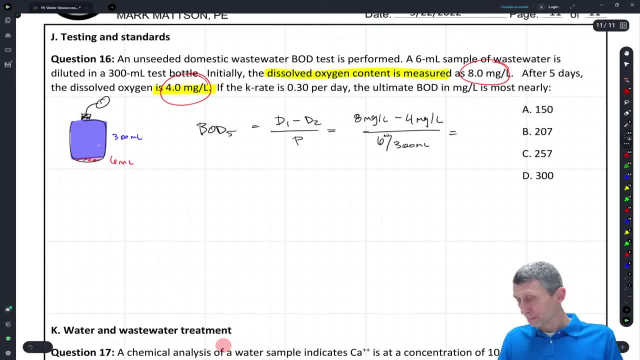 unit consistency. but that gives us our BOD five of I think this works out to 200 milligrams per liter. So you could stop there and say 207.. Great, But don't do that. So the ultimate BOD isn't just the BOD five. 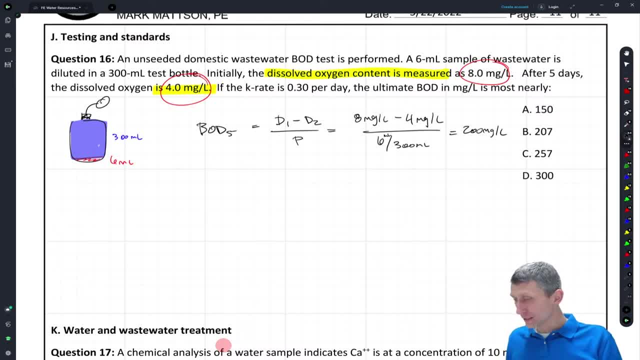 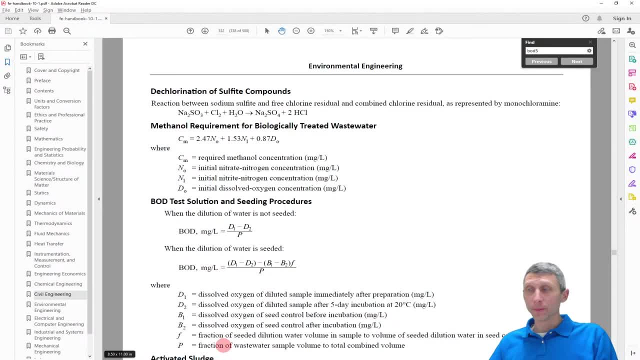 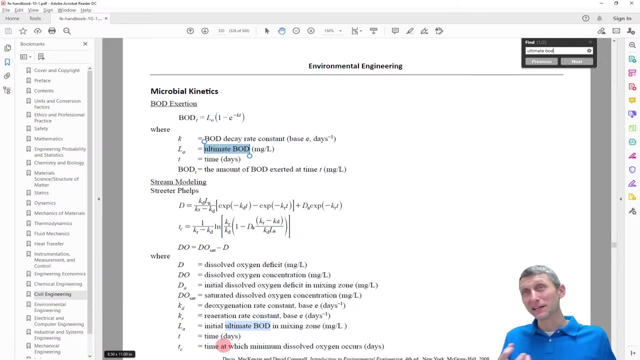 What we want to do is we want to go to the next equation here, which is going to help us as well, And specifically, when we come back to what we're looking at. I'm just going to type in ultimate BOD. Okay, So, ultimate BOD, this gives us a BOD exertion. 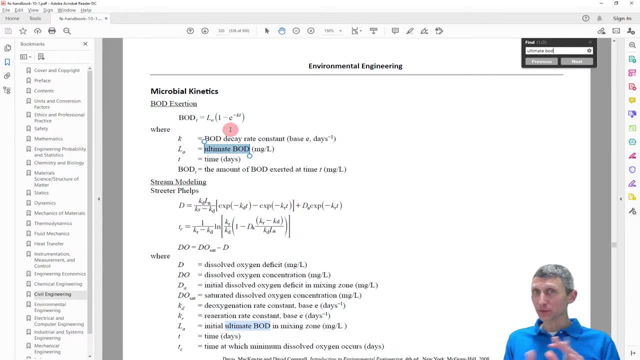 Another formula that is kind of one of those basic formulas is a basic test for BOD. That's why I'm trying to get the. I mean the environmental section. It's so big that there's a separate environmental FE. This is not intended to be an environmental FE review by any means. 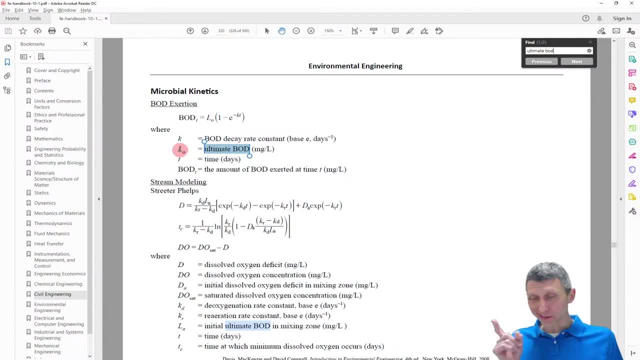 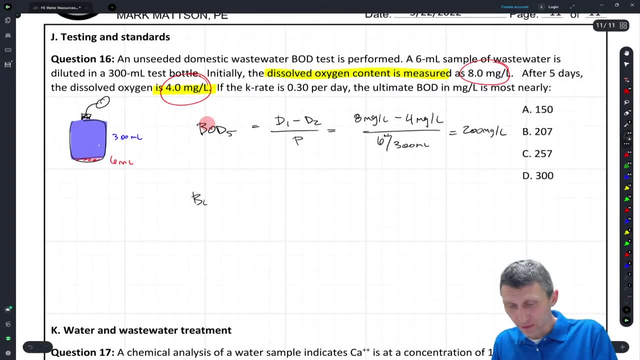 Okay, But hopefully it gets some of the basics. But what we're seeing here is that L a lot. is that the ultimate BOD that we're looking for? So I'm going to come back here and I'll say the BOD. you know, in this case I'm going to 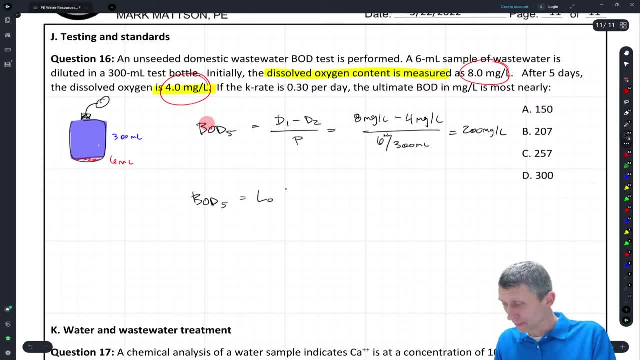 say the time T five equals the ultimate BOD times, one minus E to the minus KT. Okay, And let me put my parentheses in the right spot here. So what I'm going to do is I'm going to take this value that I just learned figured out. 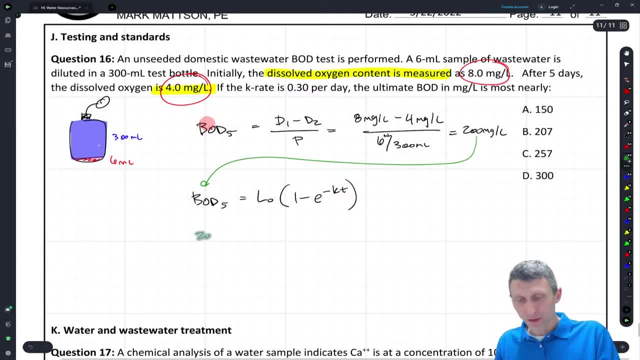 here, I'm going to plug it in. So I'm going to get 200, I'm going to get 200. milligrams per liter equals our L a lot times one minus E to the minus K, And what's K Again. this is where you're going to want to take a look at this. 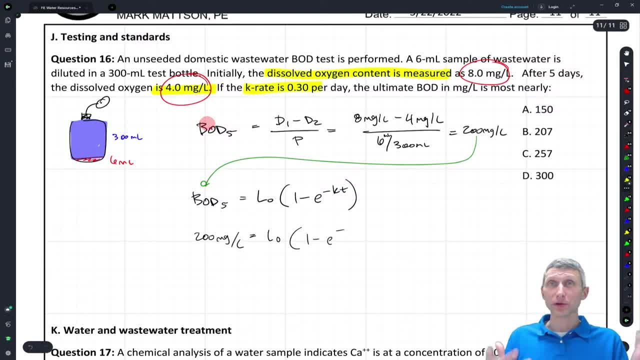 But, but hopefully you've read the problem to see that the K rate is 0.3 per day, So that's good. It is 0.3 per day times our five day tests And the good news is our units work out here. 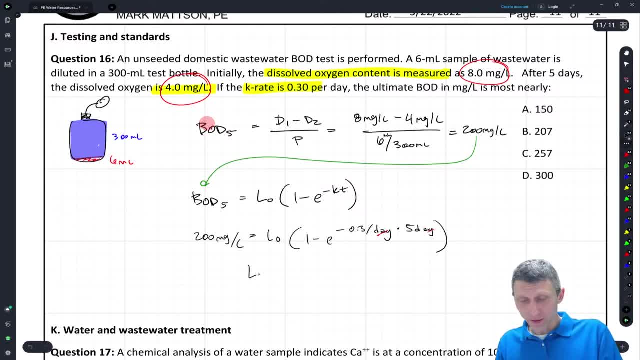 Um, and we end up with coming up with L naught, you divide 100 by- you know this mess- And uh, what she get, I believe, is about 257 milligrams per liter. Okay, So that's the total ultimate BOD. 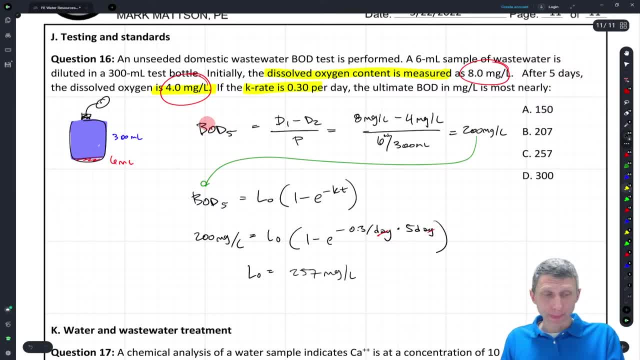 Uh, that eventually gets. um, it's all for man, we're, we're, just, we're fine, Why not, Let's go, let's go to one more. but hopefully that makes a little bit of sense. I mean honestly, um, if I had to pick some, some basic wastewater type things, I think 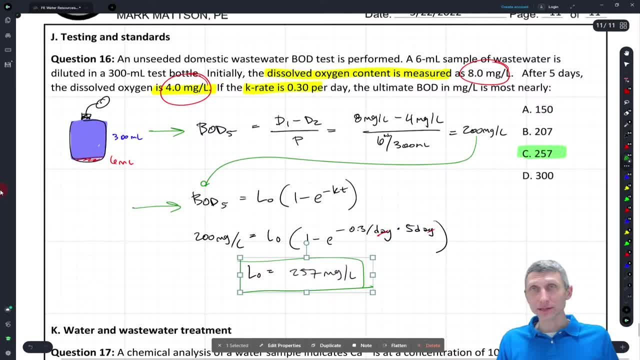 BOD is going to show up. I think you're going to see. you know whether this is fate and transport or it's a BOD test or something along those lines. um, wastewater there's. there's a couple of different topics. 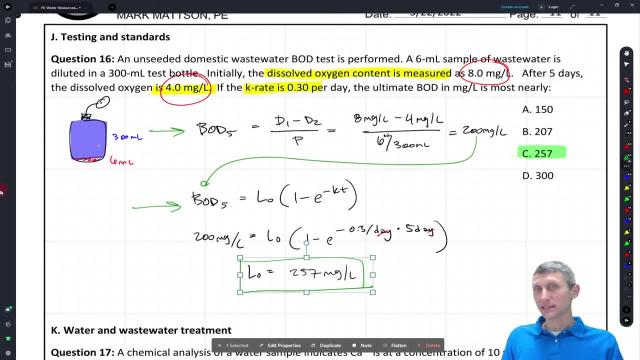 that you could throw out there. It's going to be a couple of questions on the test, It's not going to be overwhelming, but it's one of those things where, if you can get them, that's great. Um, if not, you know, I wouldn't spend a whole bunch of time studying all of environmental. 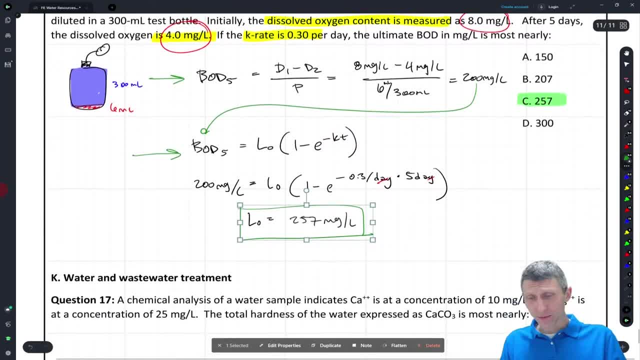 because, like I said, there's a whole test just on environmental Uh. but if you can get some of these basics down, I think that's going to help you. Here's another one of those basics that I think is good. That's useful. 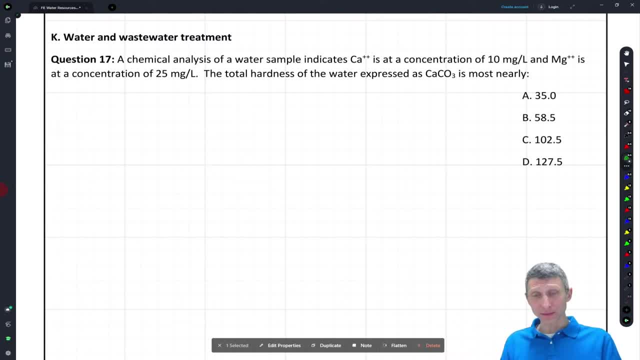 But um, this is the last question. here We have a chemical analysis. Water sample indicates calcium and magnesium. We have Different concentrations: 10 milligrams per liter and 25 milligrams per liter. What's the total hardness of water expressed as calcium carbonate? 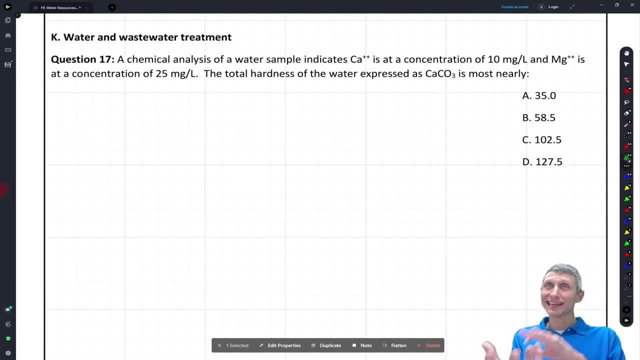 So again, this kind of goes back to the stoichiometry. What we're doing is we're trying to take one thing and convert it into something else, right? So this goes back to the stoichiometry and um, what we see here is um, is is total. 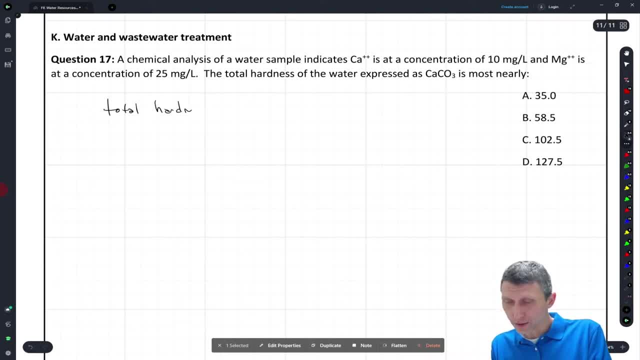 hardness: uh, in in water is essentially the sum of the calcium And um and the magnesium. okay, That is our total hardness, which is what we want to solve for. So, if you get other things like um, you know other other uh chemical analyses that give. 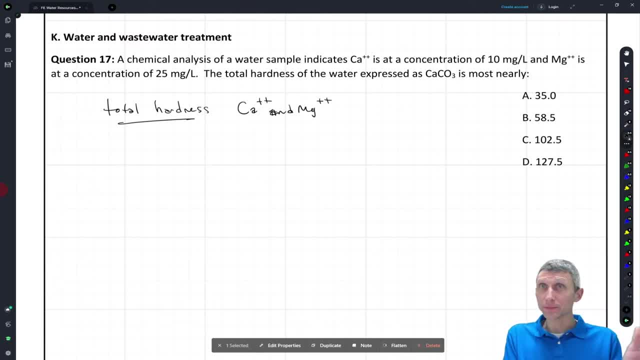 you other other components in there, minerals in there, the calcium, the magnesium. you want to pull out for the total hardness. But to convert this, what we're going to do is to convert. um, what we're going to do is we're going to take, uh, the, the, the grams of, you know, substance. 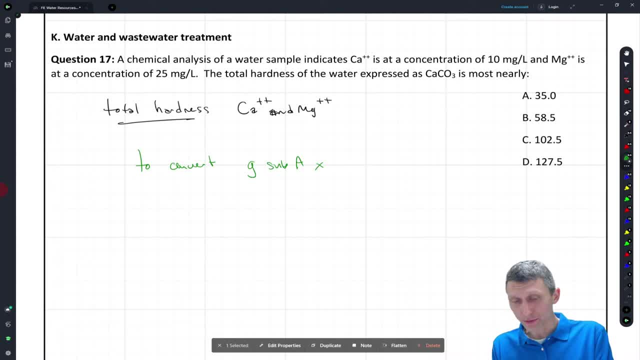 A and multiply it by, or the milligrams, in this case the milligrams for a liter of substance A, and multiply it by, uh, the equivalent weight right of the calcium carbonate, divided by the equivalent weight of the, the, um, the element. okay, 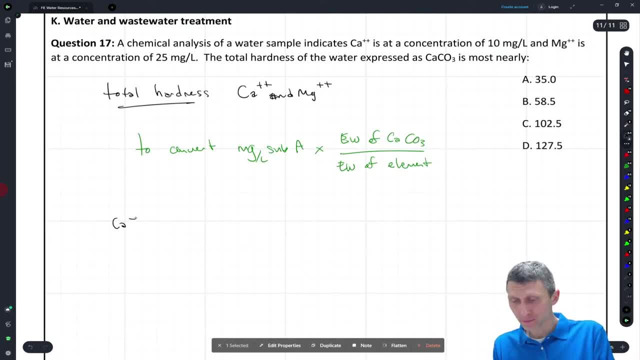 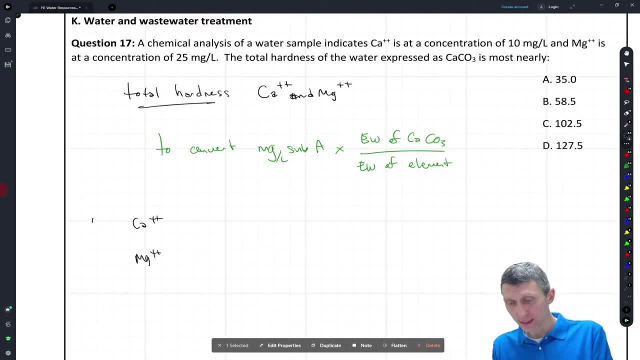 So here we have two things: Um, we have the, the calcium, and we have the magnesium, And specifically, we have, uh, 10 milligrams per liter and 25 milligrams per liter. Don't just add those and say 35 and I'm done. 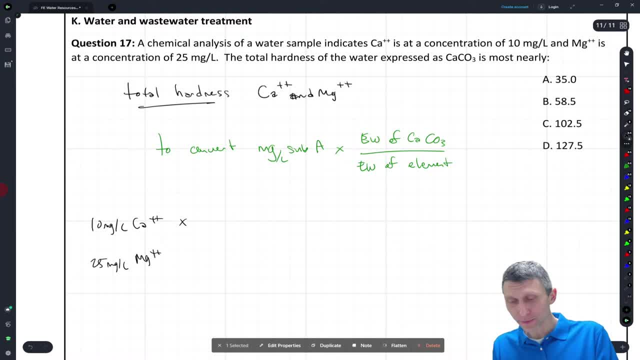 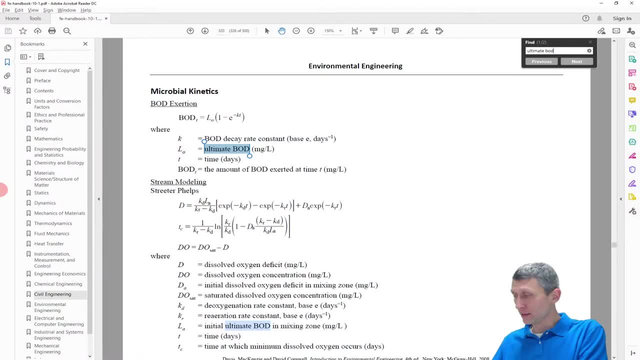 I don't want, you know, I don't want to do that anymore. Um, all we have to do here is we have to multiply by a ratio. So let's go and look at, find our equivalent weights here, Uh, and we can come back and: oh, where's that? 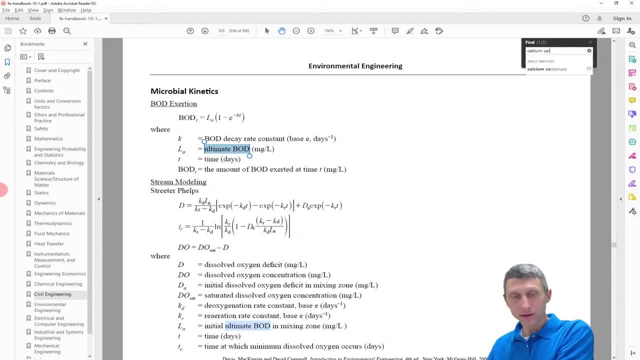 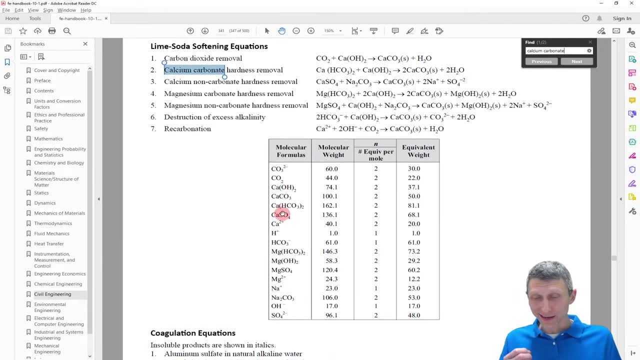 That was a calcium uh carbonate, right? So if we come back to calcium carbonate, If we come back to this table- which is nice because this gives us our calcium carbonate, which we could use the 50 or the 100.1, um and um, and then we can use uh for our 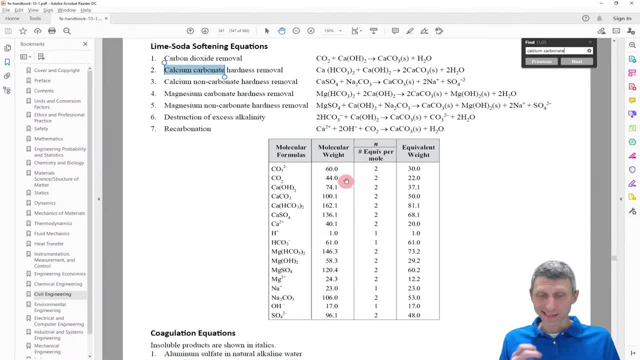 calcium. we can use the 20 or 40.1.. We have to. we have to pick and choose. it's kind of like mass versus versus weight grams. Um, I'm probably saying that wrong, but it's man, we're two hours in, so let's just keep. 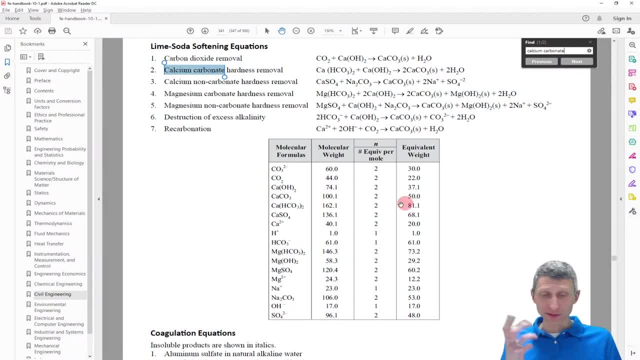 going with it. Um, but you can see the ratios here: 100 to 50 and 40 to 20, they're, they're, they're similar ratios. They make a difference. Um, so, let's, let's go with this. 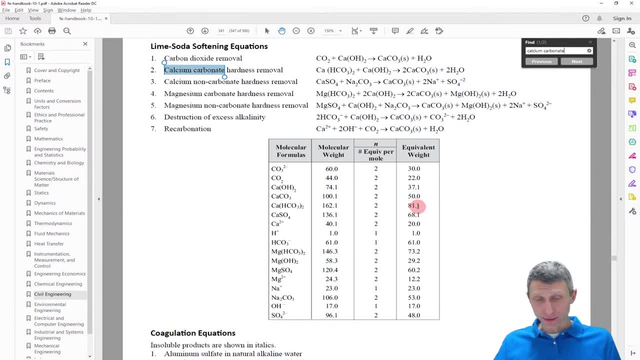 Um, so we're going to pick. you know the. the calcium carbonate is um 81.1 and the calcium is 20.. So, let's, let's. is that something? did I say something wrong? Um, calcium carbonate? no, calcium carbonate is 50, sorry. 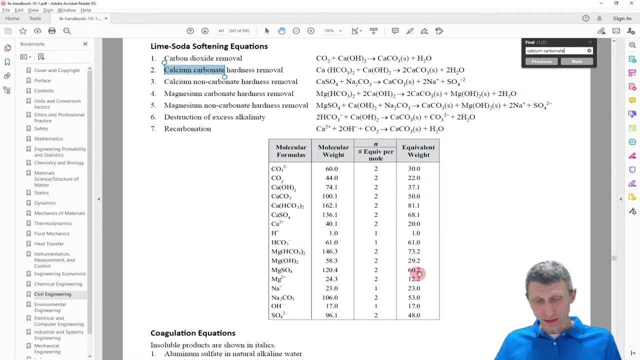 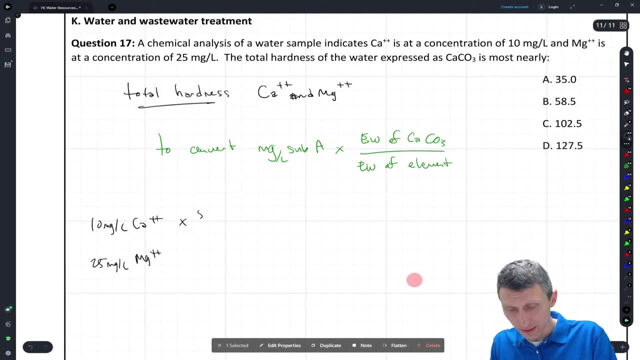 Calcium carbonate is 50 and 20 and the magnesium is 12.2.. Okay, So let's come back and and and finish this one. Okay, So let's go ahead and send it and be done. So we have 50,. um, you know, 50 over 20, this is the 50 of the calcium carbonate over 20,. 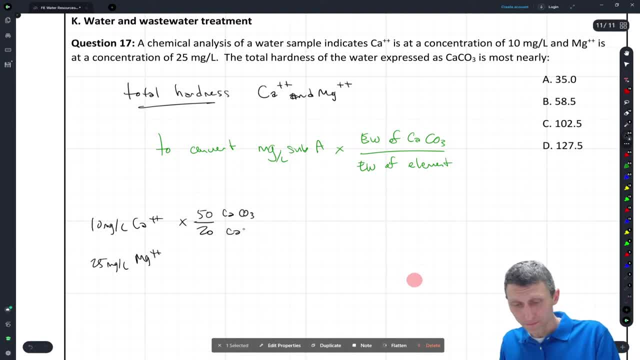 uh, the equivalent weight of of calcium, And we're gonna multiply this one by, I think, 50 of the calcium carbonate, divided by 12.1 of the calcium, And we get a couple of values here. Um, so the values that I get here is 10 times. 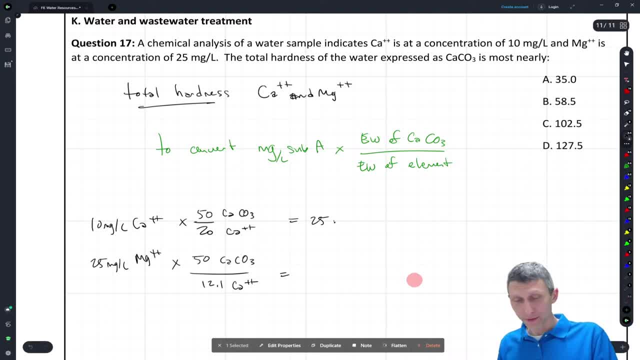 So we get uh- essentially what 2.5 is going to be- uh 25 milligrams per liter as the calcium carbonate And we ended up with uh 102.5 milligrams per liter as calcium carbonate. We add those up to get our total hardness, and our total hardness is going to be about: 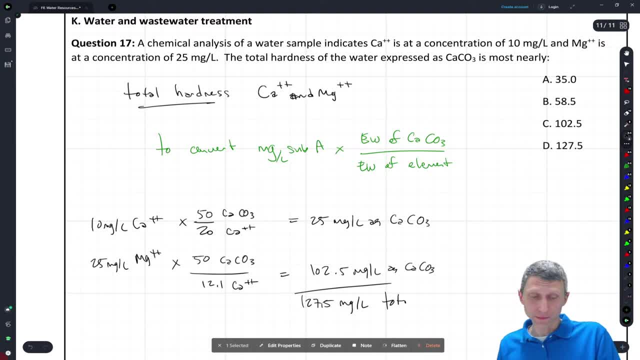 1, 27.5 milligrams per liter, uh, total hardness. and we did it. so we got there. um, there was the. i don't know we'll see how the the recording it does uh with, uh with everything. but hopefully i can trim that middle section out where 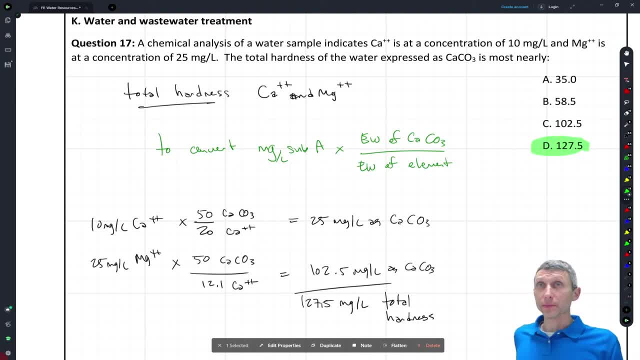 where, uh, the the recording of the stream hiccuped. but, um, hopefully this, this is helpful because there's a lot in here. i mean everything from mannings to hazen williams to we didn't get darcy wise back, but, um, you know, there's, there's some of this water chemistry in there as well. 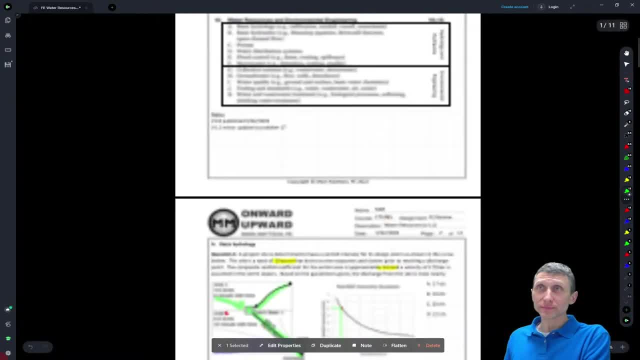 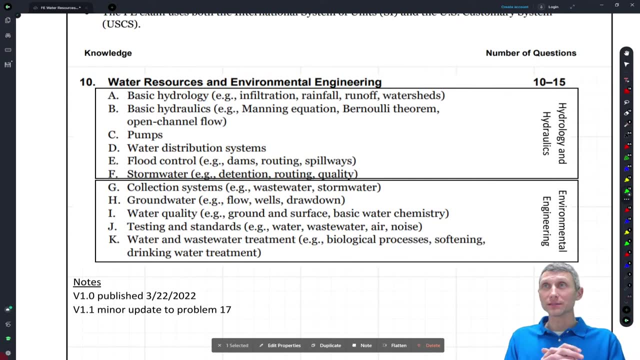 there's a lot in this section and hopefully you know, when you're all said and done, you get 10 to 15 questions in here. i mean there's a through k, is is close to 10 to 15 right there. so if you get one question for each, i tried to, you know, lay out some of those conceptual questions, some of the 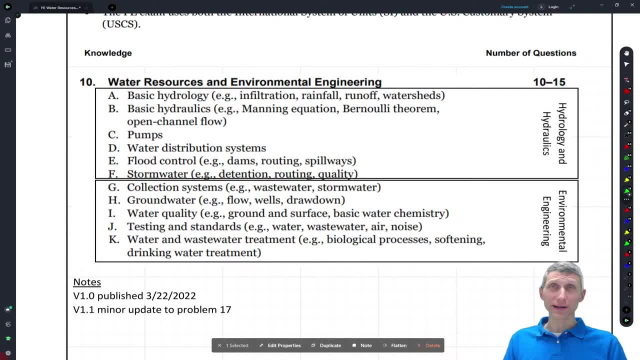 more, more technical questions, some of the ones where you use weird exponents, uh, some of those empirical equations and weird units that you have to work through because, uh, because it can be a challenge. it can be a challenge, but i think you guys can now this section, you can get it down and you can be number one. 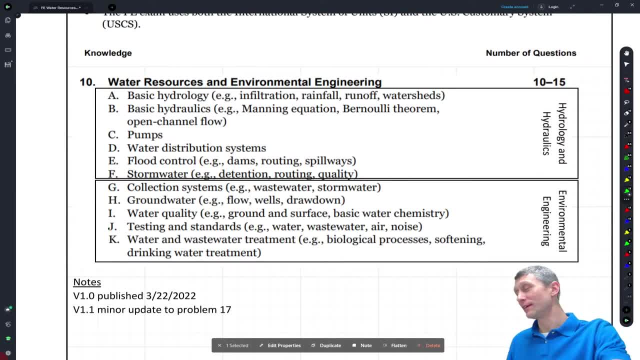 which reminds me, um, that wastewater jokes really aren't my number one choice, but they are a solid number two. sorry, okay, i had to do something just to lighten this up a little bit. and, uh, you know what? i got one more joke here that i i found, and it's not mine, i can't take. 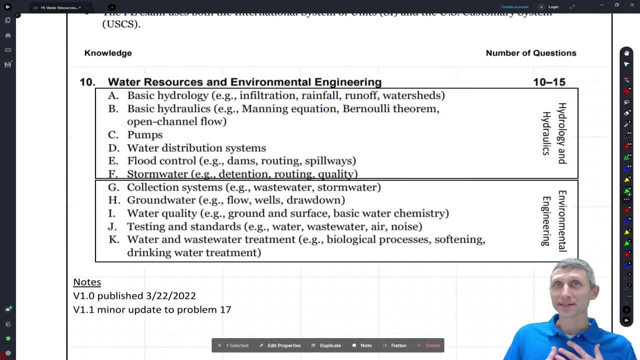 credit for this, but it's funny, so i'm just gonna, uh, i'm just gonna say this one just to send us off with a laugh, hopefully. so, uh, there were passengers on a small plane, um, that were sitting there and then the pilots came in the, but the pilots had you. 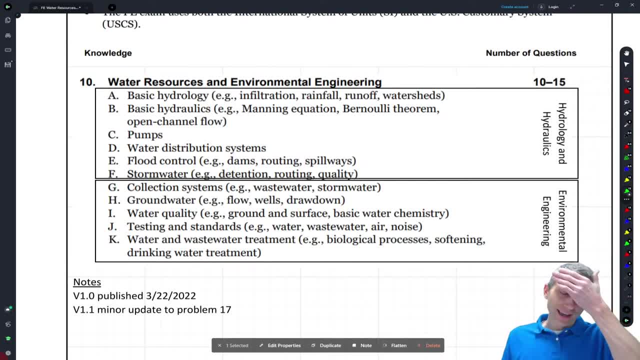 know big dark glasses on. one had a cane, one had a thing i dog- and they go up to the pilot or the- um, you know the cockpit. they close the door and they start taxiing down the runway and everybody starts getting nervous because what they see is a big lake in front of them. 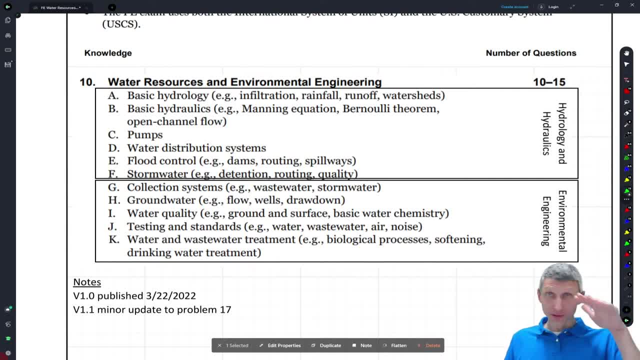 at the end of the runway and so, um, as they're going down, they're still going down, they're still going down, they're still going down. so they start screaming because they just get really mad, because they, um, they, they start worrying for their life because they're going into the pond and 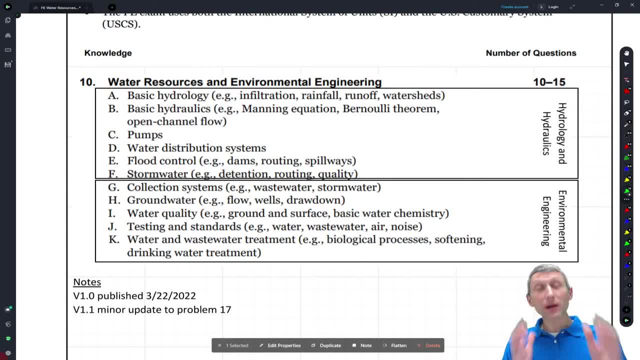 they're gonna, you know they're gonna, they're not gonna do so well, um so, but all of a sudden plane picks up, starts going up, up, up, up, up up, and everybody, everybody breathes a sigh of relief. um, then the cockpit, the, the pilot, turned to the copilot and said: you know, bob? 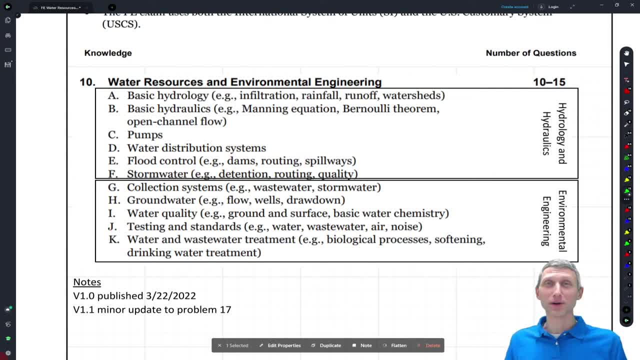 one of these days they're gonna scream too late and we're all gonna die that they couldn't see. yeah, so, anyway, they, they couldn't see the the lake, but at least everybody screamed. so, oh man, not so funny, but funny. um, maybe that's a solid number two joke, who knows? uh, but that's. 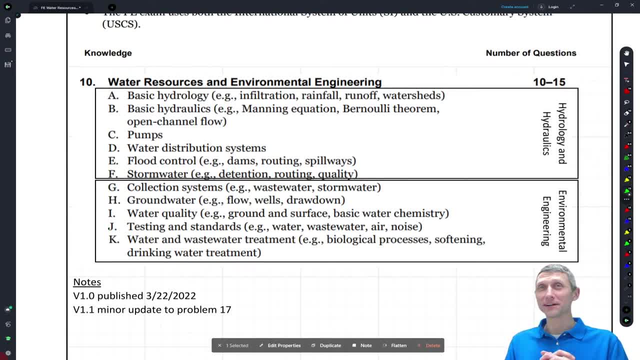 that's it. so, um, hopefully this review helped you. hopefully the problems are are a good refresher on a bunch of things and, uh, you know we can. we can keep going. so next week we'll be on to transportation. uh, i've got some good problems there and, jay man, you, you remember my tests. 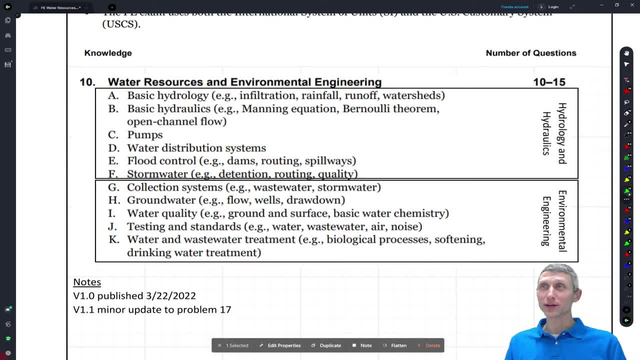 transportation. so this is going to be, uh, my, my transportation analysis test from from i. actually i think i'm going to take problems from your test, so why not? um, this is, uh, this is good, but um, transportation should be fun again. a million equations um about two million variables.